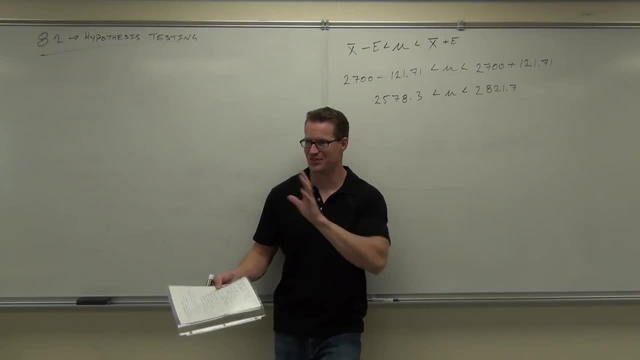 Right, But that's usually how science goes, at least to first deal with hypotheses. You do a hypothesis, you make a hypothesis, and then you experiment, don't you, And you see whether that hypothesis was actually a true statement or whether that was just complete garbage. 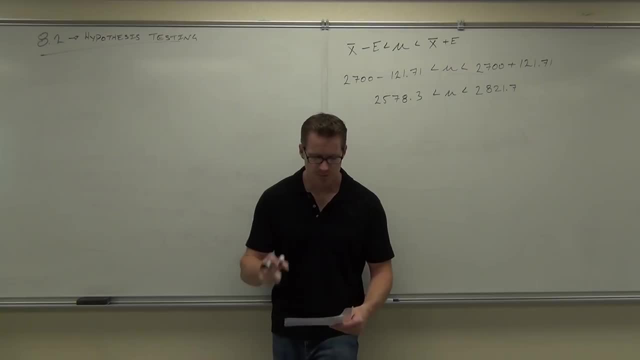 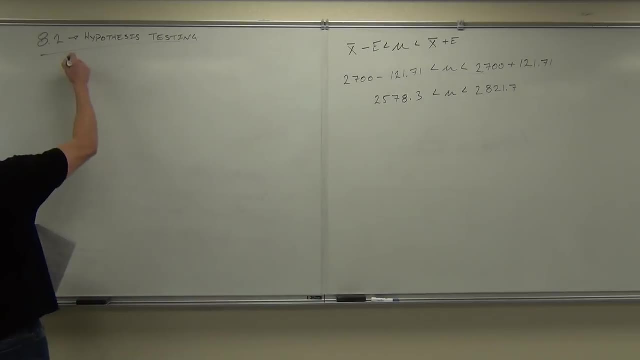 You either prove it right or you prove it wrong. You with me on that. That's basically what we're doing here. This hypothesis testing is testing whether or not a claim is valid. That's the whole idea for this whole chapter: Testing whether or not a claim. what's a claim? 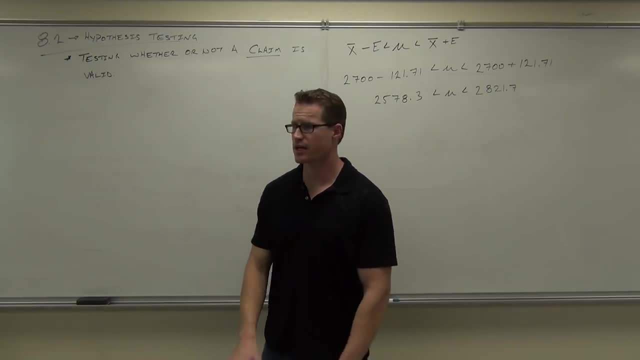 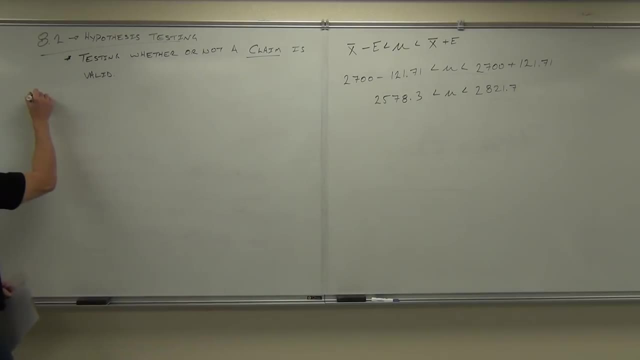 What is a claim, then? Some sort of statement. yeah, you're exactly right. Here's some examples of some very simple claims that we can actually test, based on fact, based on a sample. One example would be- I think I made these ones up- 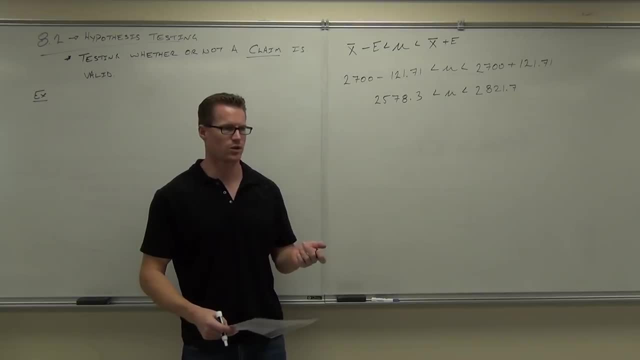 One example would be: most people get their jobs through networking. You ever heard of networking, Networking, that statement: it's all about who you know, Not about what you know. it's all about who you know. You ever heard that before? 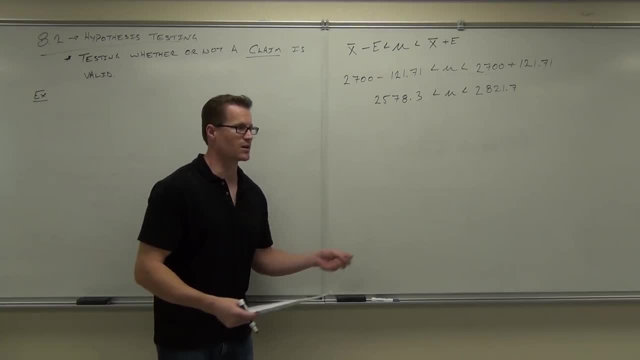 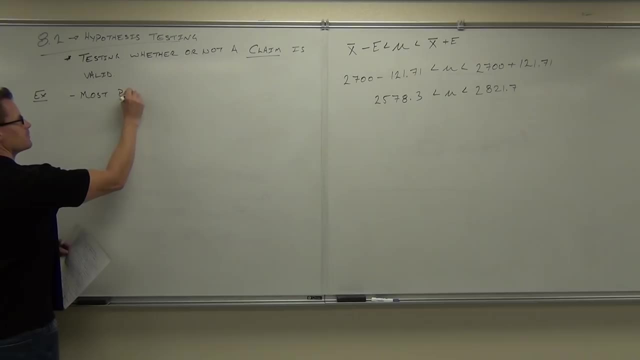 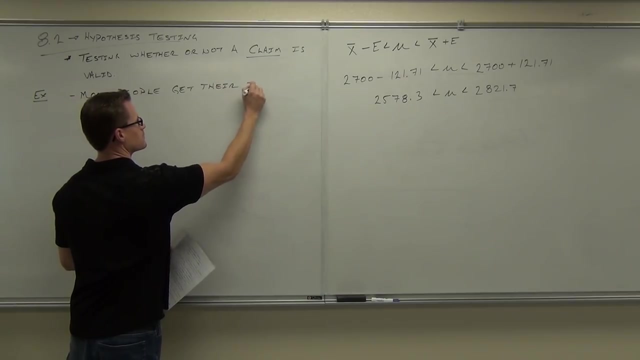 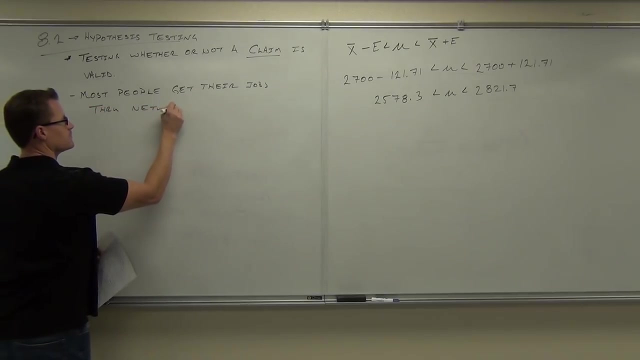 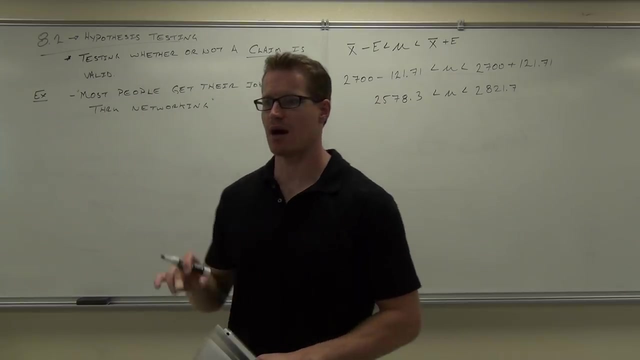 Well, do you believe that's true? Well then, you believe, you get your jobs through networking, And a lot of people do So. if I made the statement most people get their jobs through networking, We could actually translate that into a statement we can now test. 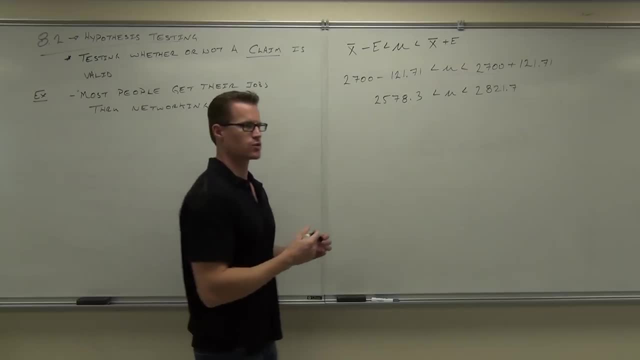 Here's the deal. Firstly, if I say most people get their jobs through networking, are we dealing with a proportion or a maximum? Are we dealing with a proportion or a maximum? Are we dealing with a proportion or a maximum? 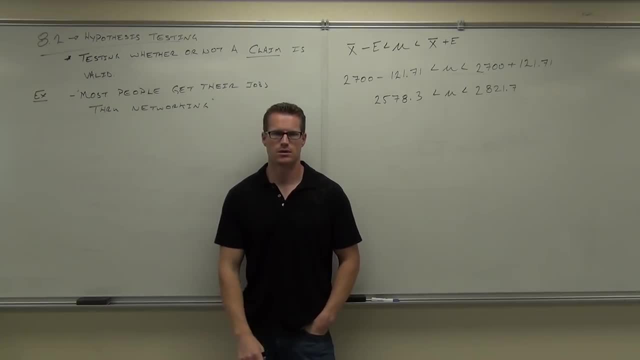 What's the word mean here? do you think, When I say something like most people, That's a proportion? That's a proportion What's most mean to you? More than 50%. Say it again: More than 50%, That would be most to me. 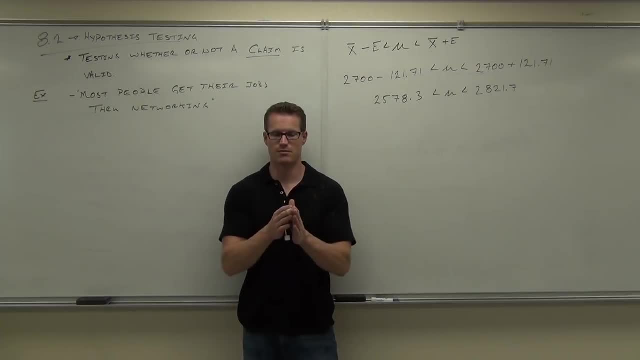 Would that be most to you? If I have most of the pie, I have most of that's, more than half of it. That's 50% or more of the pie. Well, actually just slightly more than 50% of the pie. 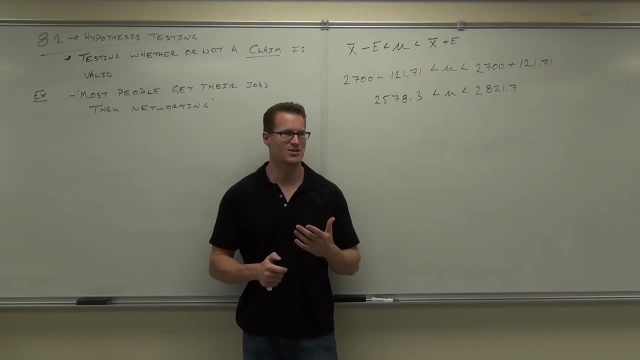 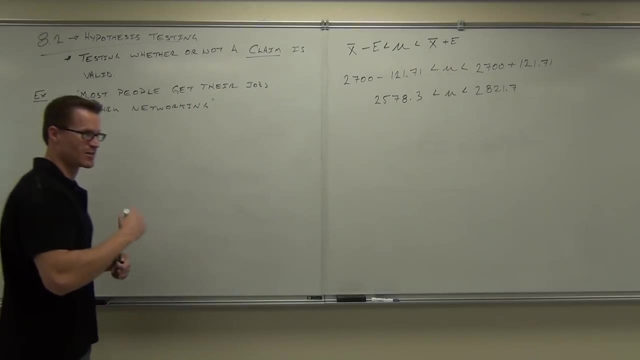 Does that make sense? So I don't know. pie, Oh my gosh. I'm so thankful that Thanksgiving's coming up so I can eat my pie. That's fantastic. I'm gonna have most of the pie. trust me on that. 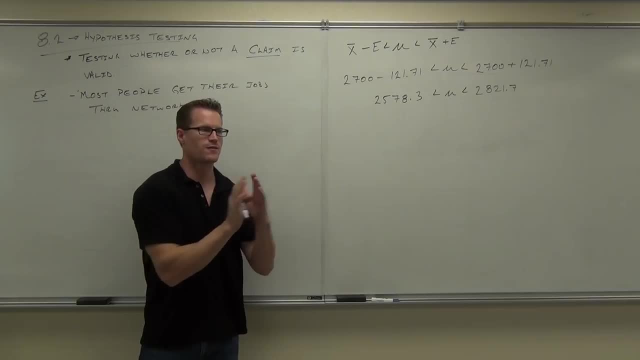 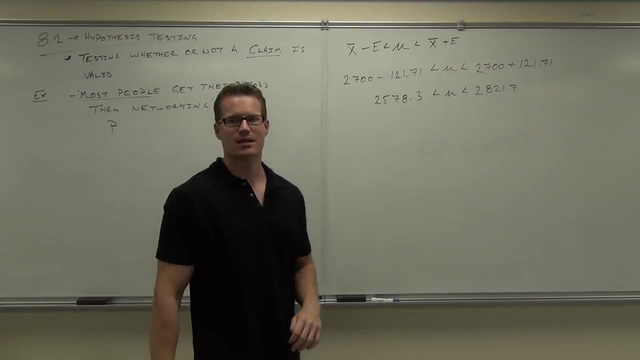 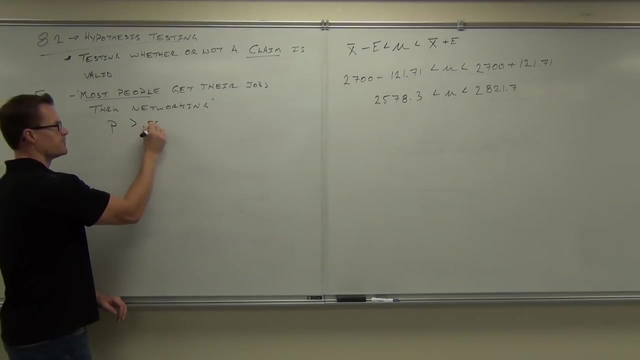 So most is a proportion. it says more than 50%. So if I'm talking about most people, of course that is a proportion. We use the letter P for proportion. We'd be testing the claim that most people the proportion is more than 50%. 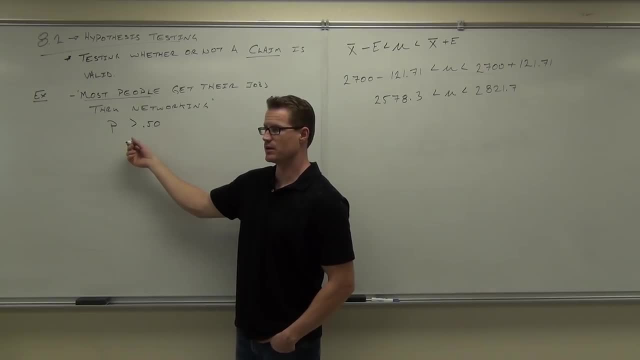 Do you see how we can translate this claim into that statement? Yeah, you have to identify whether something's a proportion or an average. Now, if it's an average, it's gonna say average. If it's a proportion, it's gonna give you something like most. 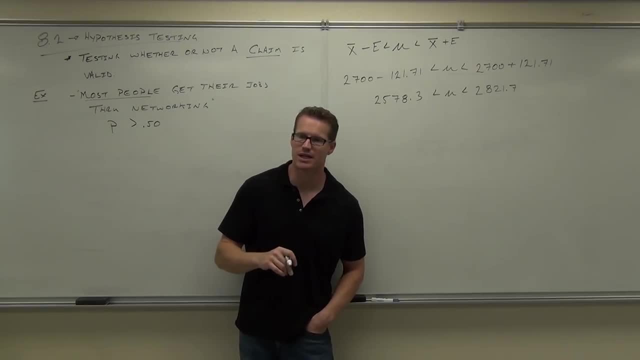 or more than 60%, or less than 20%. It's gonna have a percentage, or it's gonna say most- You with me on that, It gives you a proportion. So we'd say, all right, the proportion. or most people get their jobs through networking. 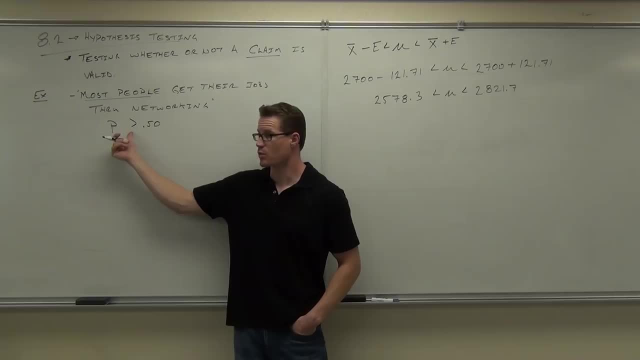 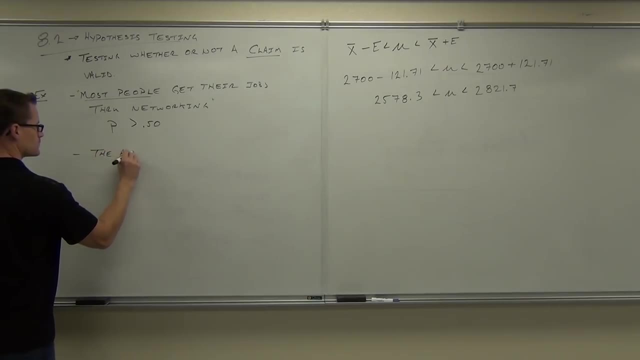 that would be a proportion's more than 50%, or P is greater than more than 50%. Here's another example: The average pay load of trucks on the 99, that's a freeway. in case you didn't know that, The same, the same. 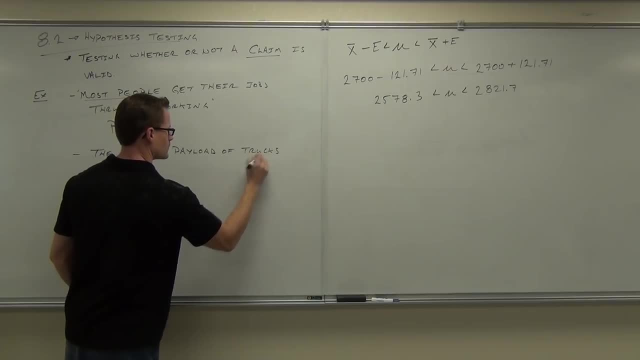 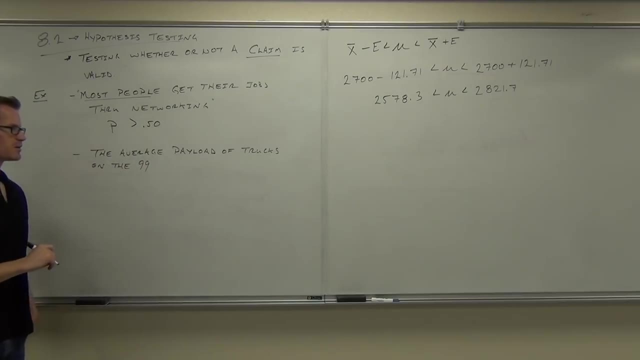 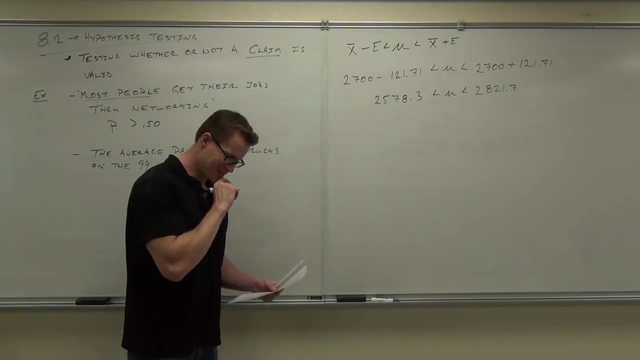 Just an adventure. We want to have a form that says thatiggies get paid and the ramp and that territorial damage All right. Now let's delete these. That means if it's a freeway and we can't get our job. 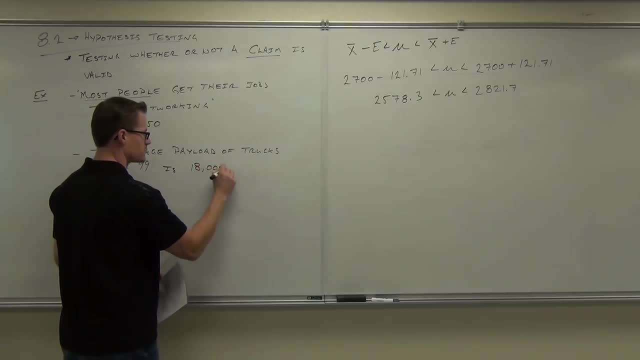 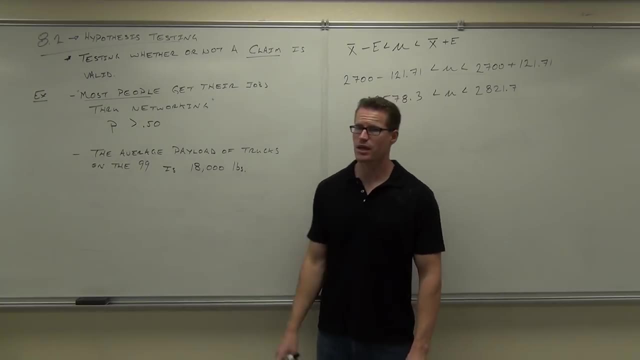 18,000 pounds. Is that a claim? Sure, I just stated that claim. I just said: okay, here's what it is. I said the average payload of trucks on the 99 is 18,000 pounds. Now are 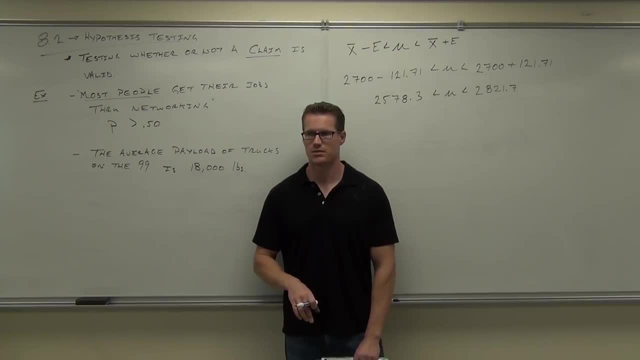 we dealing with proportion or means here? do you think Means Why It says average? Notice how I'm using a population parameter here. I'm not using p hat, right? I'm trying to say something about the whole population We're going to figure out in just a moment. 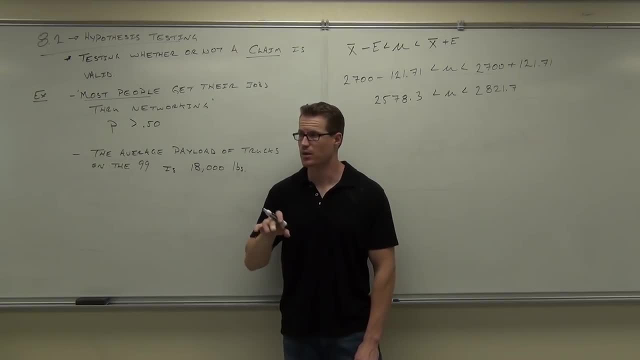 how we can use sample data to do that. It's a pretty interesting thing. We're going to find that out. I'm saying something about the population. This is a claim about the population. Do you see that It's not about a sample? We'd be certain about a sample. 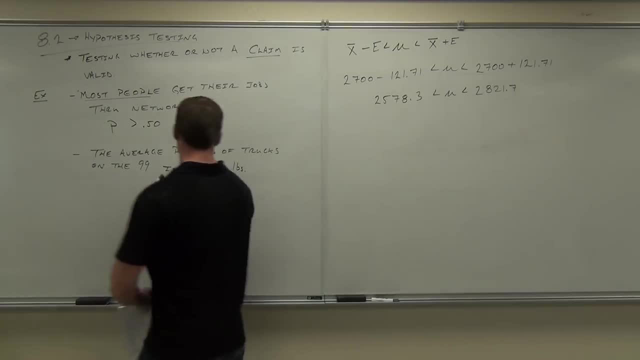 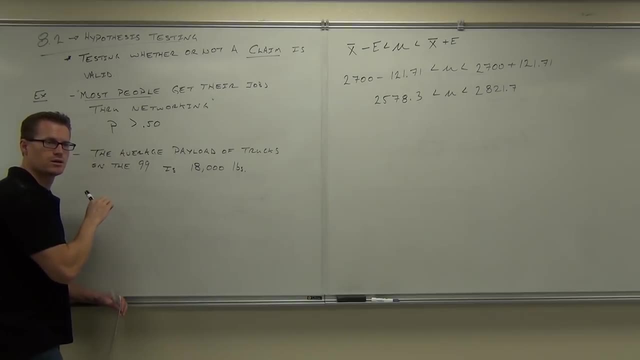 We're going to be testing claims about populations Instead of average, payload of trucks. instead of a proportion, here I have an average. What symbol am I going to use? if it's about a population, Definitely mu, X, bar or mu. What do you think? Mu? 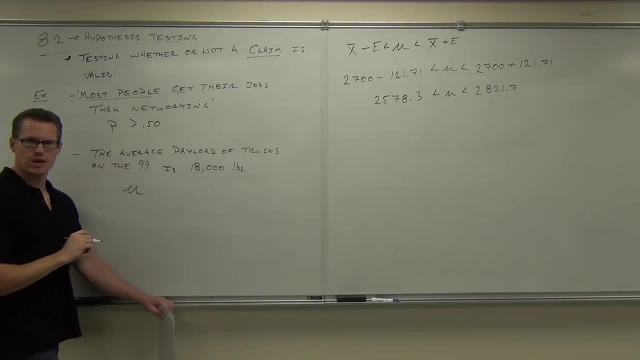 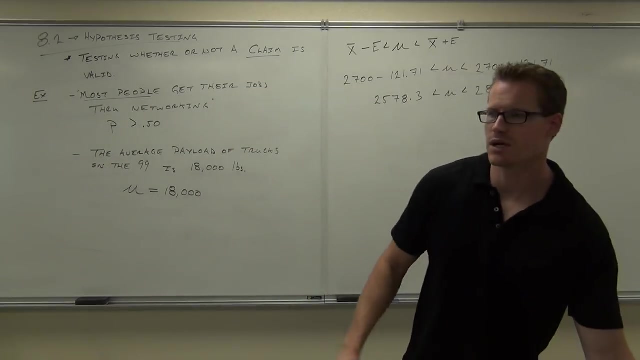 Mu. What am I trying to say? Is it greater than, less than or equal to, Equal to? Why? What says it's equal to? Can you get from here to here on your own? Can you determine that the average is 18,000?? 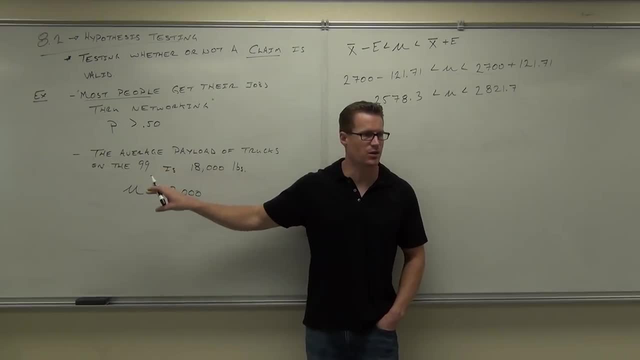 You see, what this chapter is about is translating into a claim and then testing that claim. You see, anybody can make these up. I could say: the average payload of trucks on the 99th is 500 million pounds. That's a claim, right? Is it a true claim? No, But you'd have to find out how to prove me wrong. 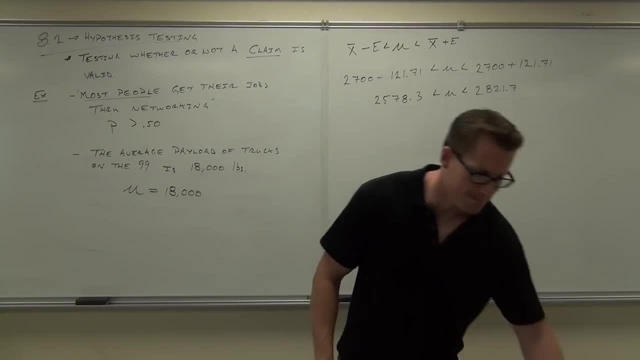 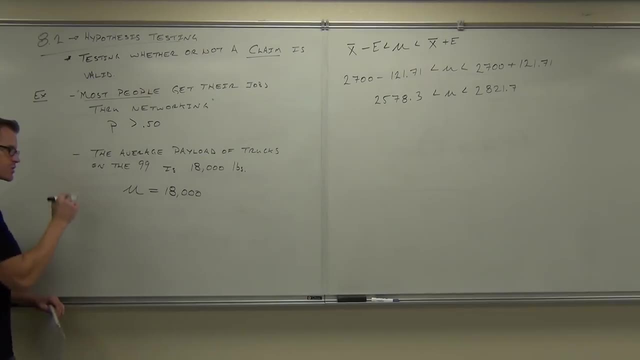 And that's what we're going to do in this section. In order to do that, we've got to talk about something called the rare event rule. Now, we've talked about it before, but now we're going to be more specific. 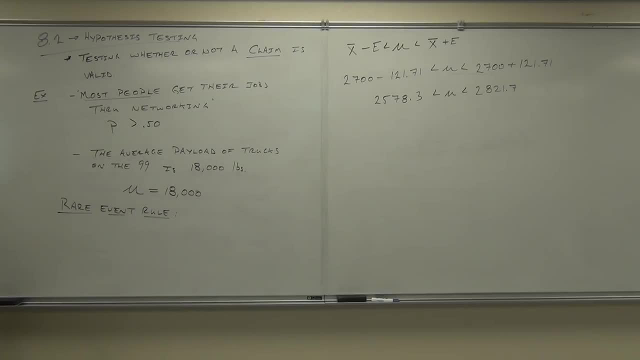 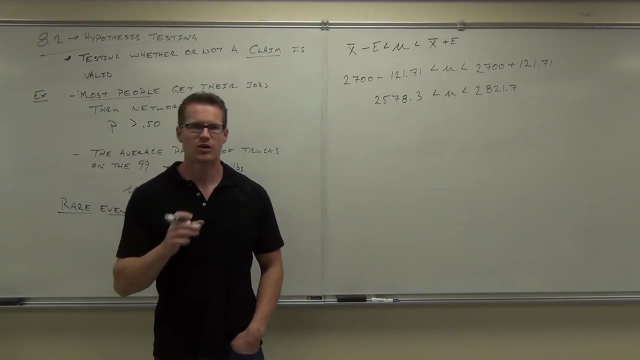 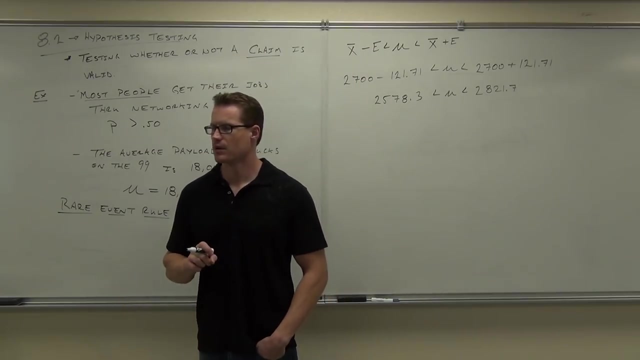 Rare event rule. You see, we're going to be making assumptions out of these claims And we're going to be testing the probability of those assumptions. Hey, if the probability is really, really small, Let me repeat that for you: We're going to be making assumptions out of these claims. 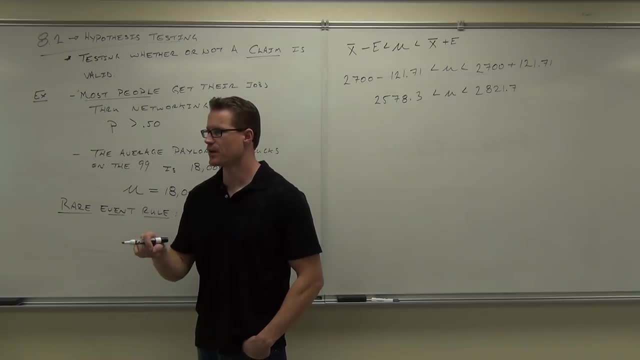 We're going to be testing the probability of those assumptions being true. If the probability of those assumptions is really small, what do you know about that assumption? It's probably wrong. It's probably wrong. Right, Like my 500 million pounds. 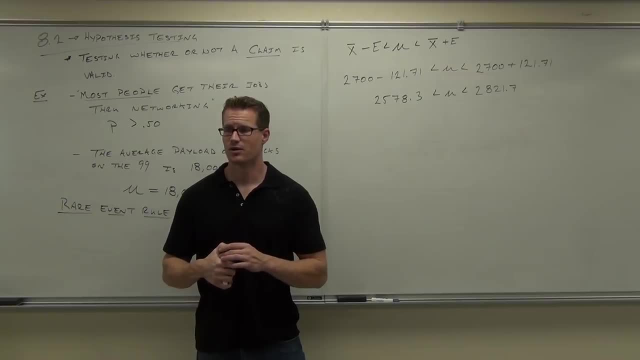 So I'm going to assume that every truck on the road, or the average payload of the truck on the road, is 500 million pounds. Is that a lot of weight? Yes, That's ridiculous. That would just obliterate concrete below it. Okay, It's gone. 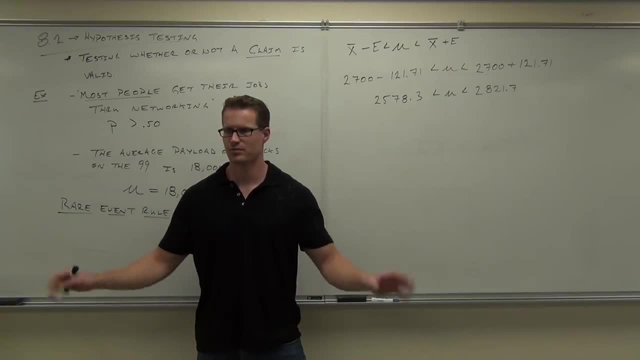 I mean no asphalt, The tires would just pop immediately. This guy would be like Spitting, nothing would happen, Alright. So that's a huge assumption, A huge amount of weight. So is that What's the probability that I'm going to go out there? 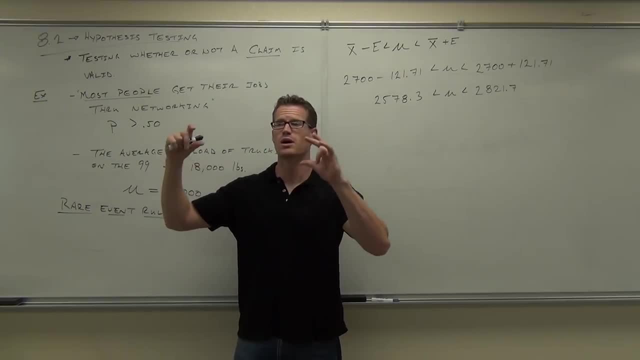 See, here's the thing. If I assume that's correct, Let's say I'm going to assume that the trucks on the road weigh 500 million pounds And I go out there, What's the probability I'm going to even find one of those trucks. 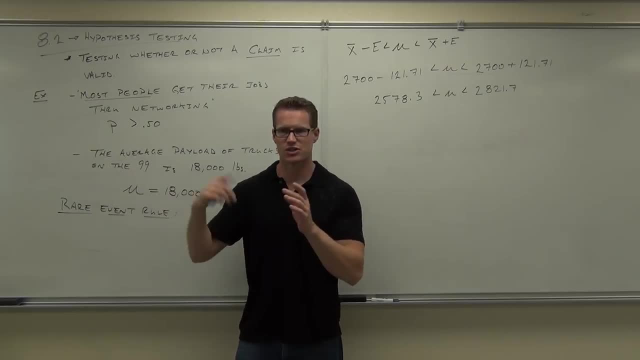 So I'm going to take a sample of all those trucks. right, Is the average of those trucks going to be 500 million pounds? No, So the probability, according to my sample, would be close to zero. Are you with me on that? 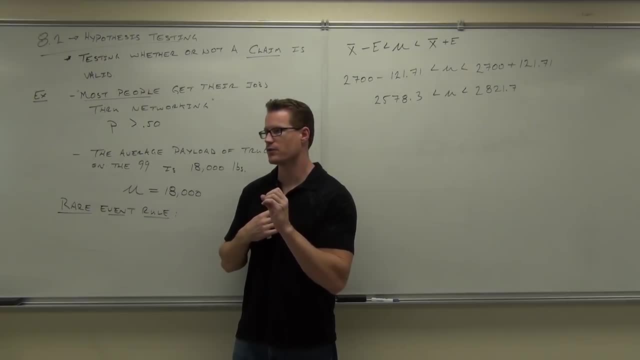 That means that my assumption, My assumption, was probably way off. That's what we're doing. We're going to be testing a claim by looking at a statement, assuming it's true and then proving it wrong. That's what we're going to do. 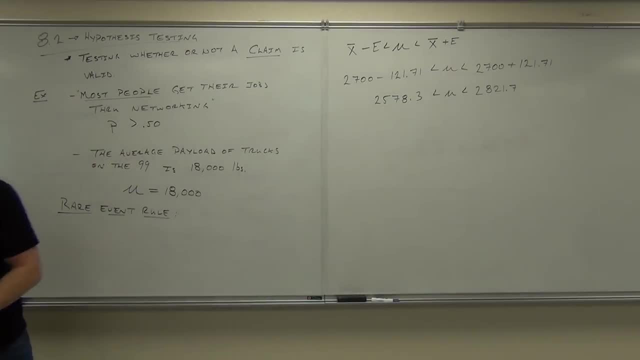 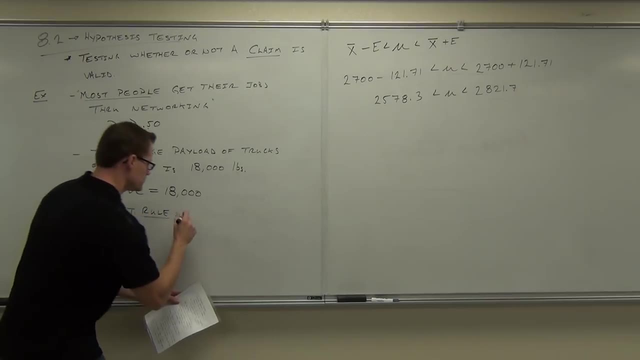 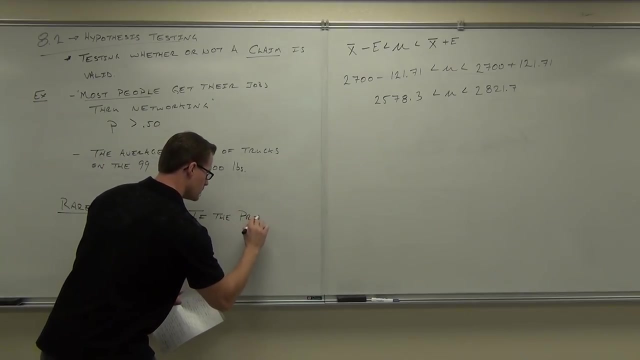 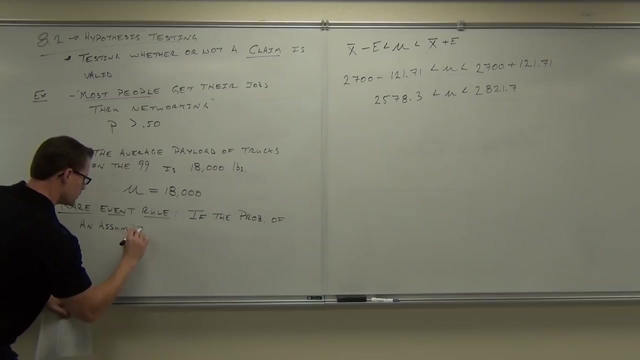 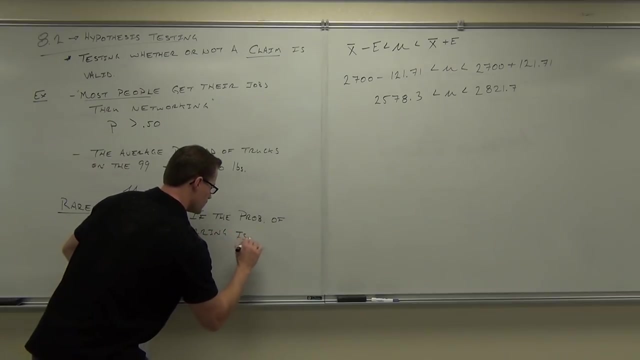 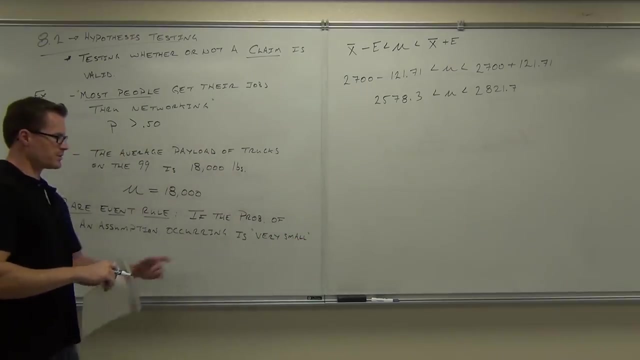 So rare event rule says: if the probability of an assumption occurring is really small, then the assumption is wrong. Alright, Okay, Now I'm going to put this in quotation marks, very small, because we don't know how much that is. 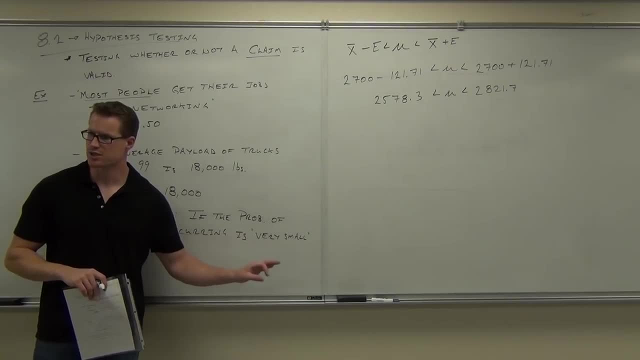 But that's what you're actually going to change on a test by test basis for you. So we're going to study that just a bit. But if the probability of an assumption occurring is really small, then the assumption is probably incorrect. 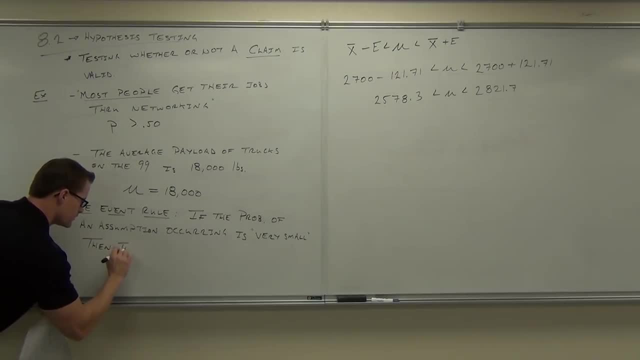 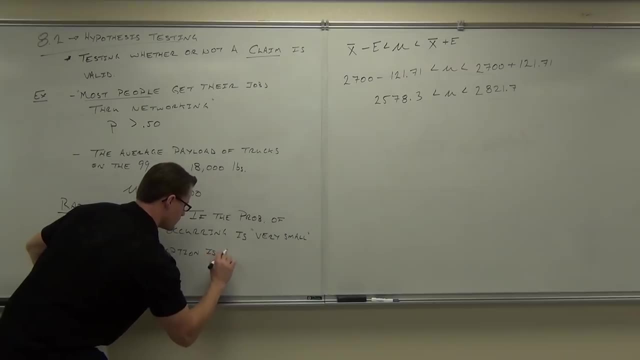 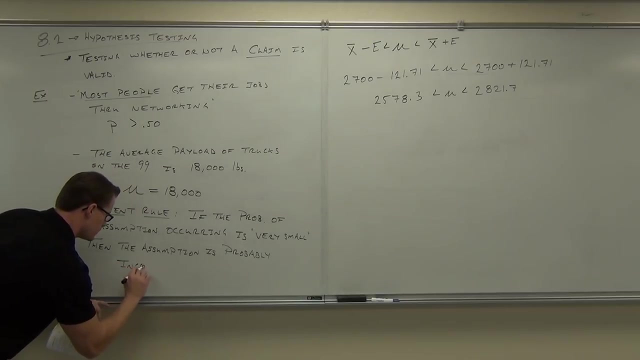 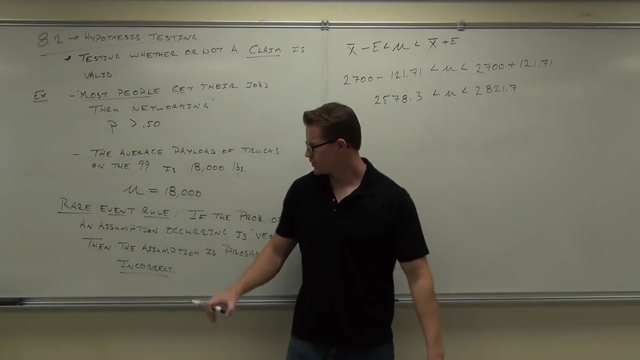 We'll be right back. Sorry, everybody, I'm back. Okay, There is a problem. Now wait a second. I include that word probably. are you going to be sure, 100% sure, whether that assumption is true or false? 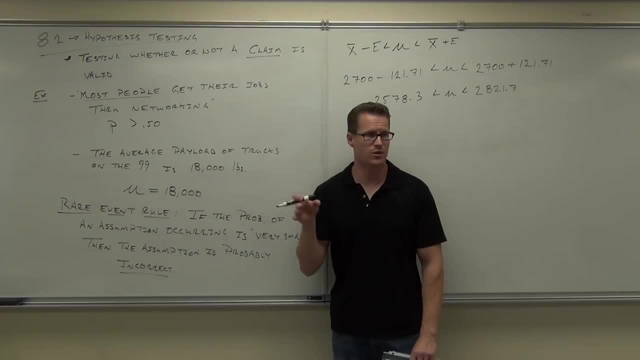 No, Were you 100% sure that the actual value of your mean fell within the range that we just created? Were you 100% sure of this? No, you were 99% sure of this, right. Hey, those confidence levels are going to come back at you. 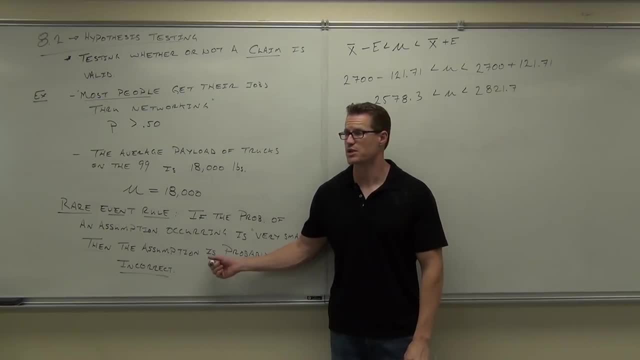 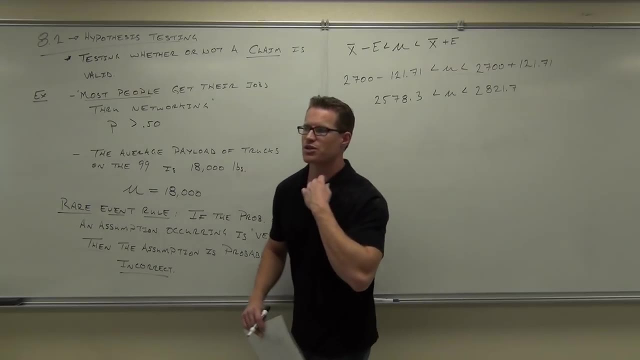 You're going to be 95% sure that your assumption is wrong, or 99% sure that your assumption is wrong, or 90% sure that your assumption is wrong. are you getting me on that? So that level of confidence you're never going to be 100% sure, never, ever going to. 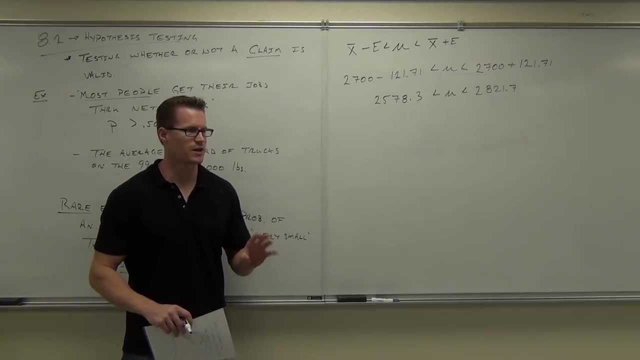 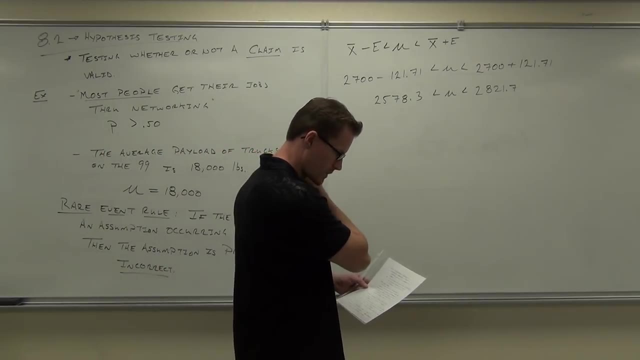 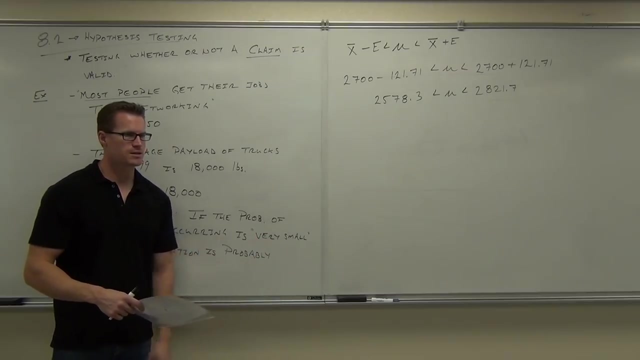 be 100% sure. statistics is not about being 100% sure, but it's finding enough evidence that you're reasonably sure. So now we've got to determine what this very small means. this is the difference between a likely event And an unlikely event. 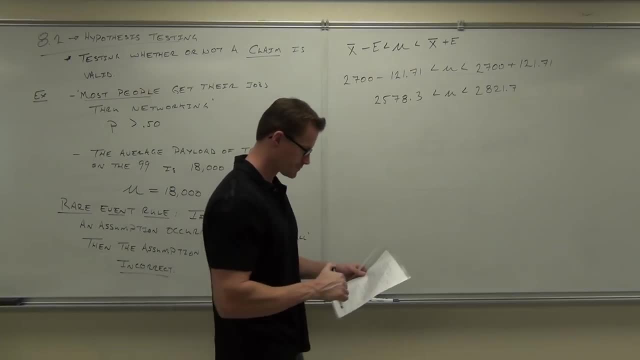 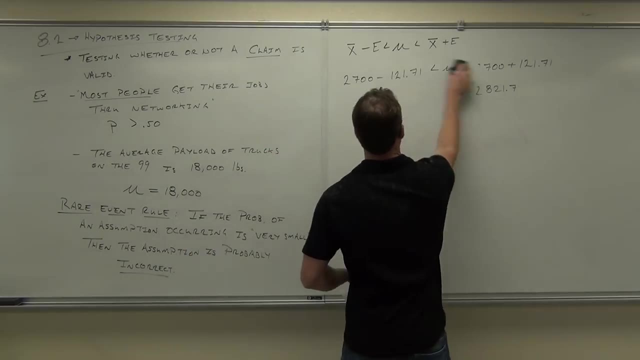 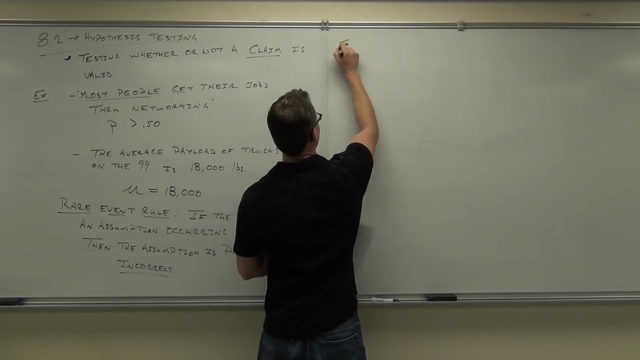 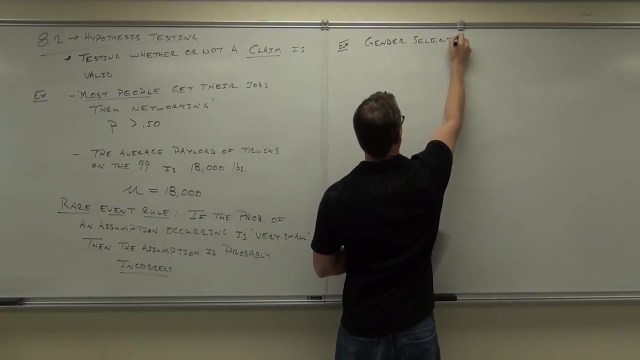 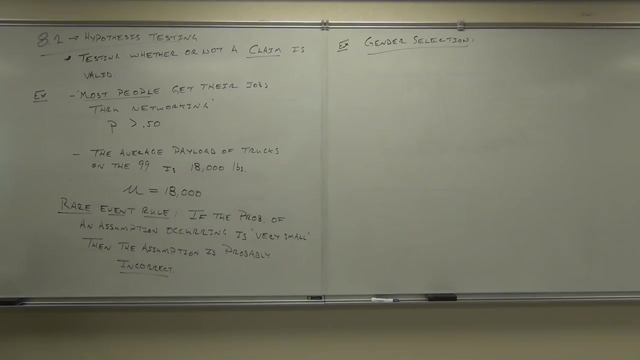 What is usual to happen and what's not usual to happen. Should we do an example on that to kind of illustrate that for you? Okay, Okay, I read this somewhere. I don't know if it's actually true. I could just be making it up. because it happens a lot, But there's a chance that it's true. I don't know One of you sciencey people out there. are there drugs that will determine the sex of a child, like help you get a girl versus a boy? 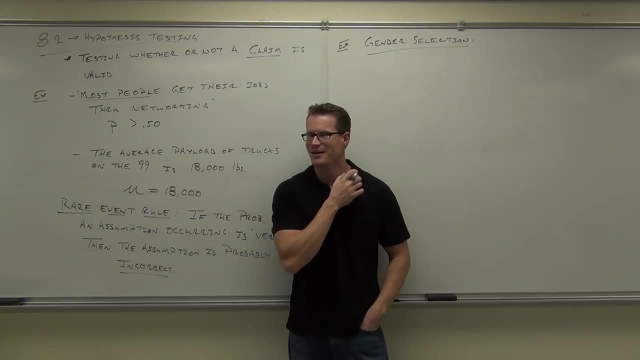 I think there are. I was pretty sure I was right on this. I don't think I just made it up. But if I didn't make it up- and this is right, this is awesome. Is your word there? What now? 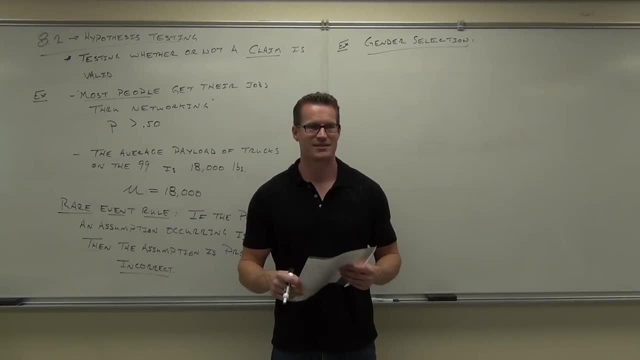 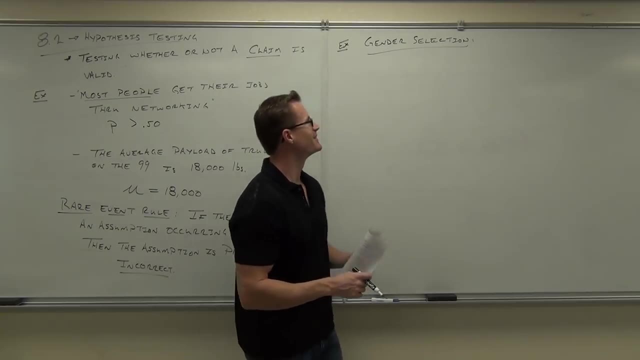 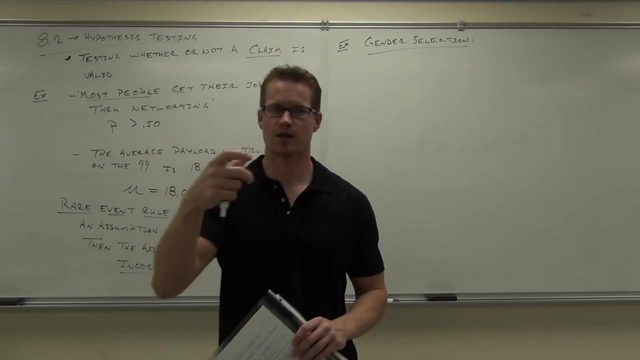 Is your word there? You can't have animals. but I don't know about you. Humans are animals. Well, yeah, but I mean a life song, Never mind. Here's what this drug claimed to do. This drug said that if you inject this drug into a woman, there's an 80% chance that her 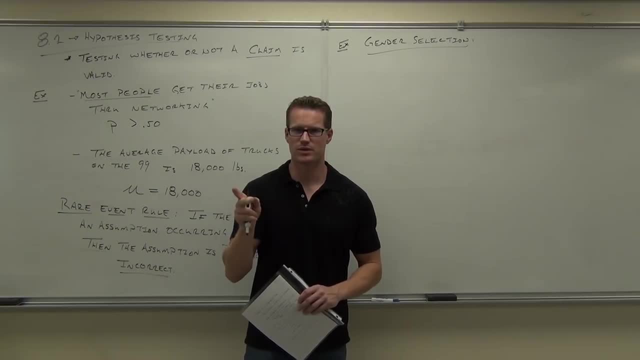 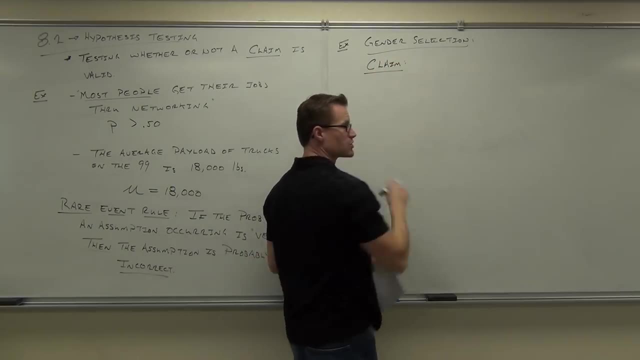 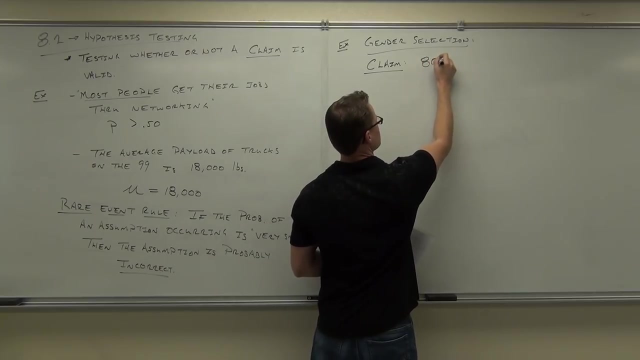 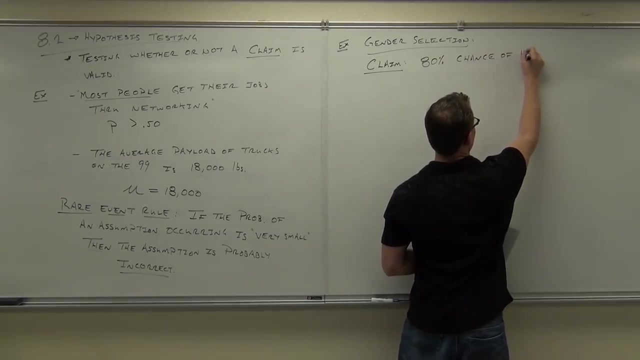 child will be a girl. You got it. You can't do that with boys, but there's an 80% chance you can have a girl. So here's the claim, Here's the drug company's claim: If you use this drug, there will be an 80% chance of having a girl. 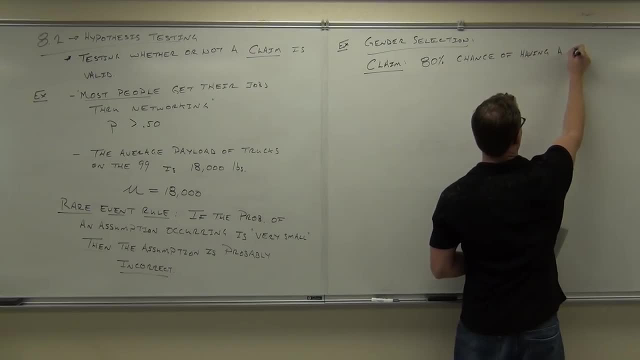 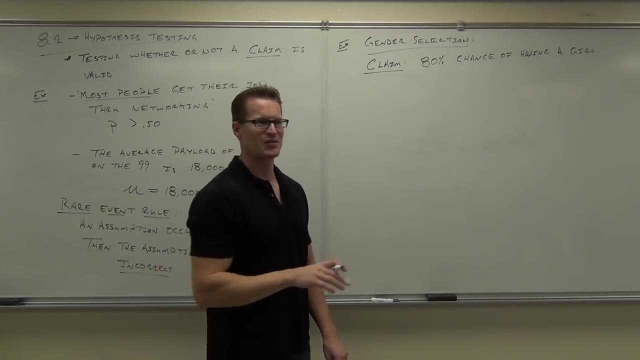 One of you guys should Google that. Not right now, Not right now, But see if that's true. If there's drugs out there like that, I was pretty sure when I first did this that there was. Okay, It could be off though. 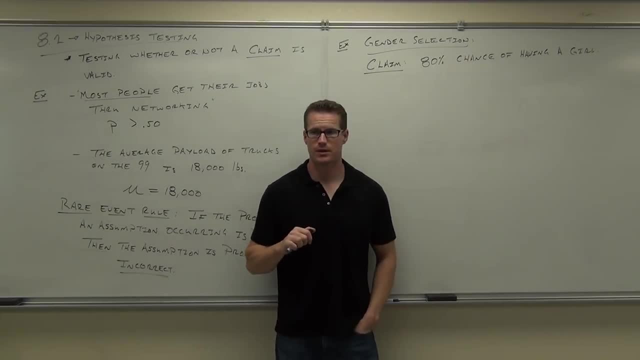 80%. By the way, our claim- you need to be very good at this- is our claim dealing with proportions or averages, Proportions. Why proportions 80%? Yeah, 80%, That's a proportion. right there, right. 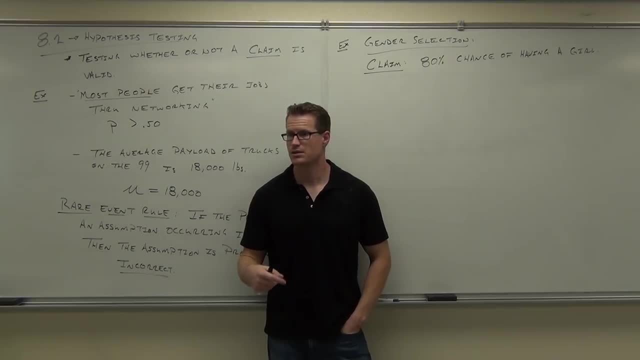 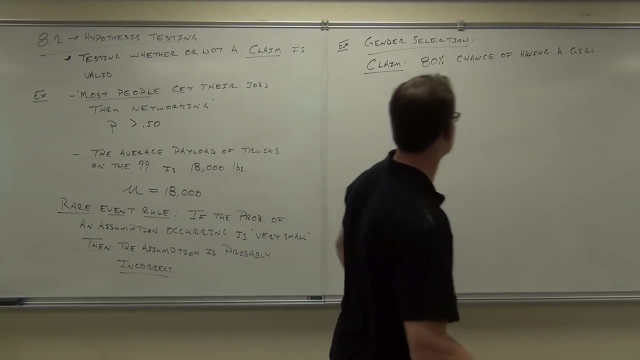 It's not an average. It doesn't say the average of anything, does it? It says 80%, That's a proportion. So this would be a claim about proportions: 80% chance of having a girl, Or at least 80%. 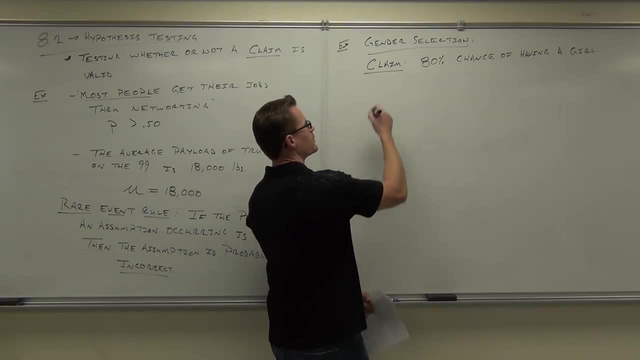 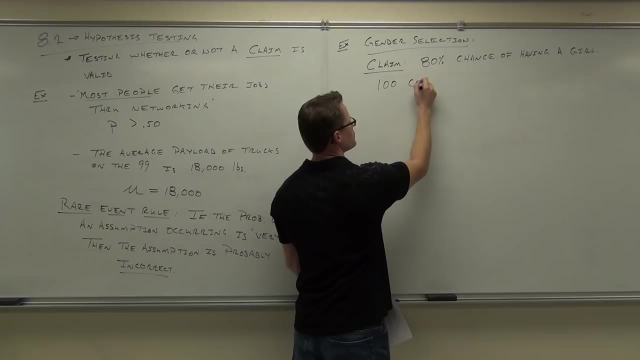 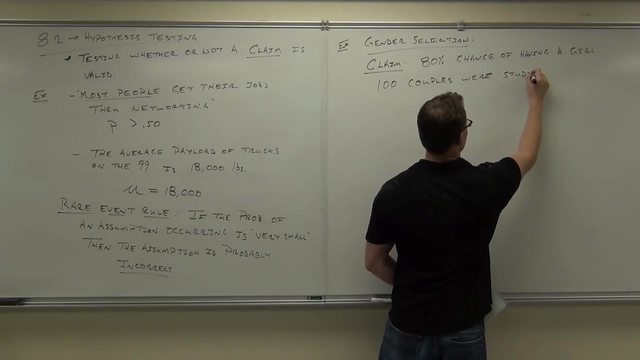 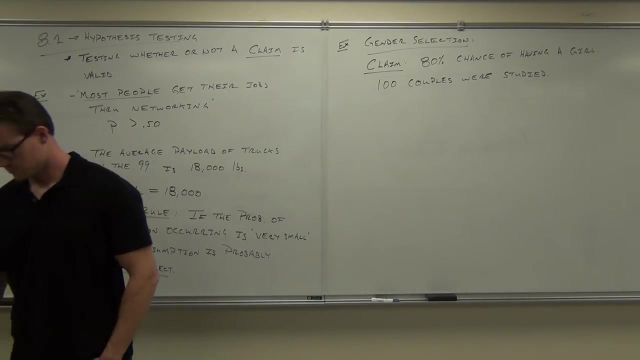 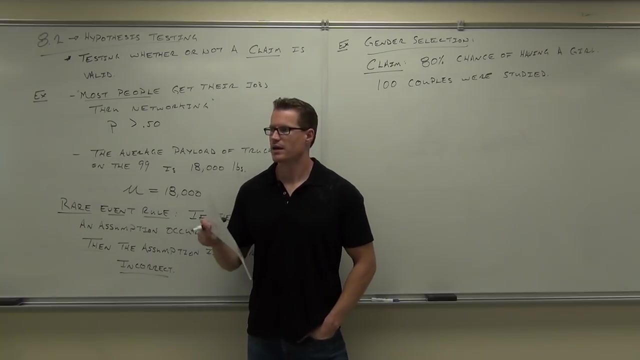 Okay, At least 80% chance of having a girl. Here's what happened. They studied 100 couples. A random sample of 100 couples was studied. Here's what you would do to try to test, let's say at least. 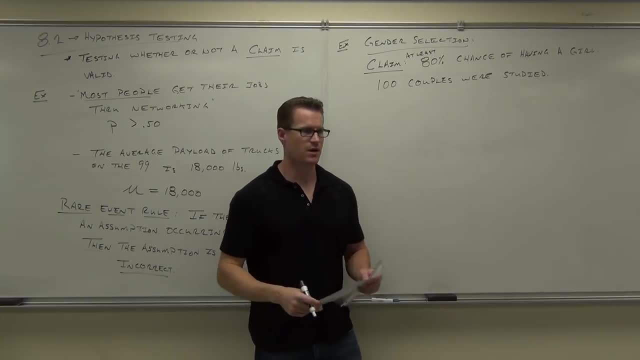 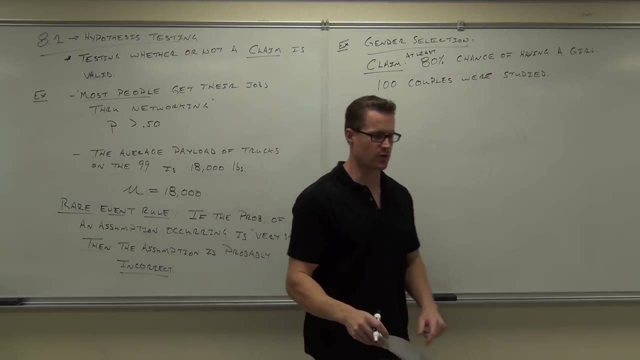 You have at least an 80% chance of having a girl in this case. all right, Not exactly 80%, but we'll say at least That makes things a little bit easier. We'll discover this in a couple sections, but this would be nice for us. 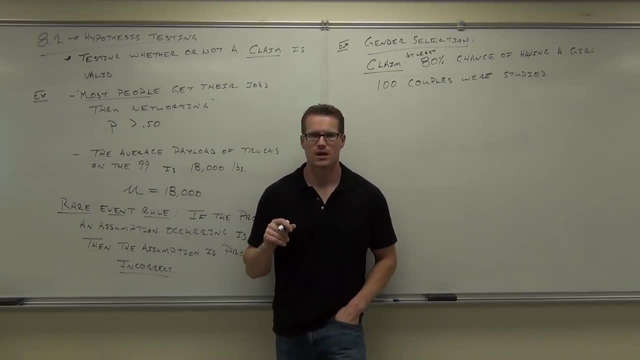 Here's what you would do. Okay, Try to stick with me on this thing- According to your claim- Your claim says that, if that's true, That 80 of these couples should have girls, right, You with me on that- What you would do is you'd start by assuming that the drug doesn't work. 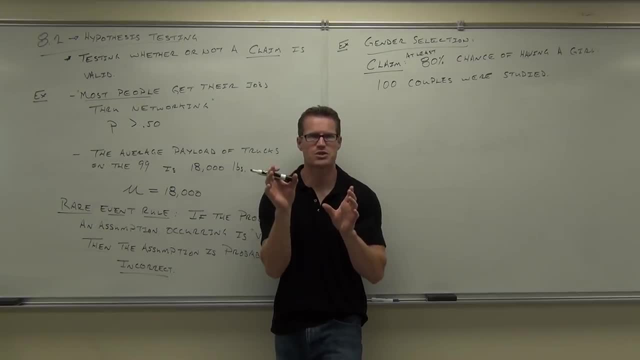 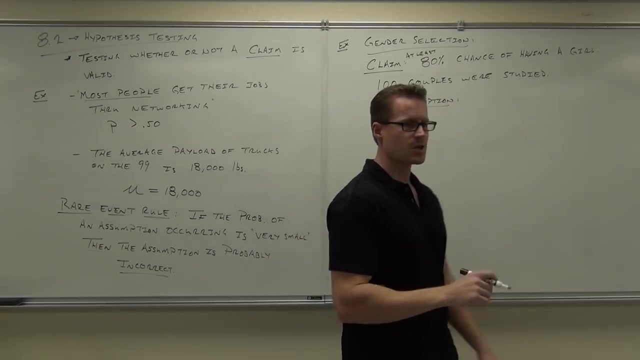 You'd say: I'm going to assume the drug doesn't work. That means that 50% should have girls and 50% should have boys. Are you with me on that? The assumption would be: The assumption would be the drug doesn't work. 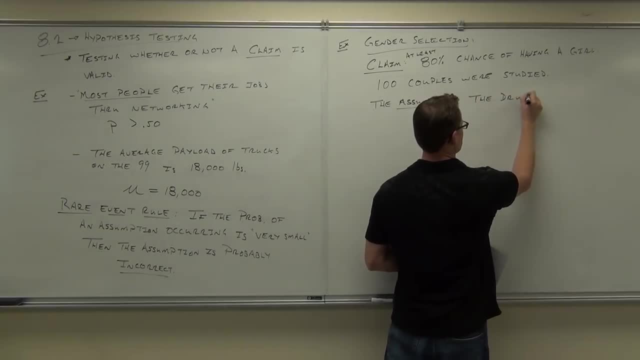 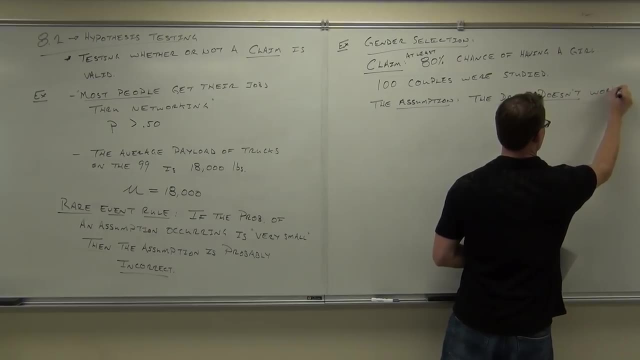 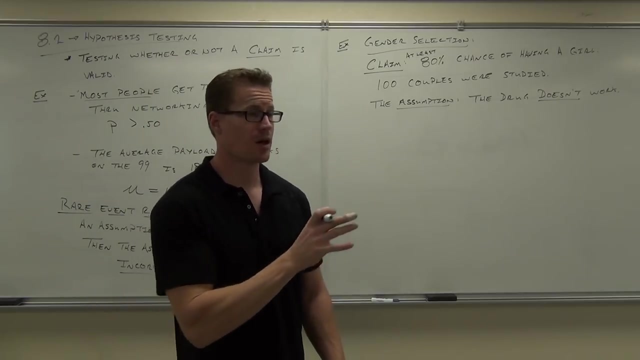 Now you might be wondering why do we even have this assumption? Well, here's the weird part about statistics, kind of the sucky part really, if you want to consider it the sucky part. You can't ever prove anything right in statistics. 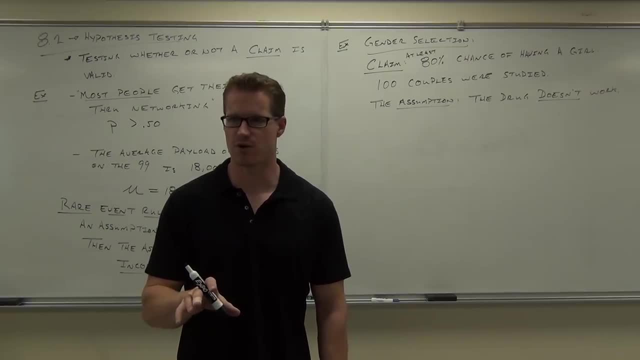 You can't. It's impossible. You can't be sure enough to prove anything right- You're never 100% sure- But you can be sure enough to prove something wrong. So it's kind of like in court: can someone ever be found innocent? 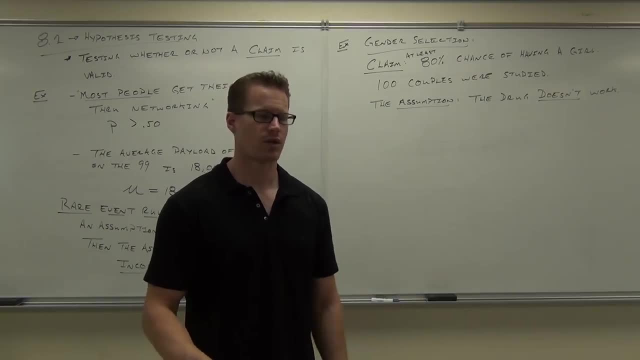 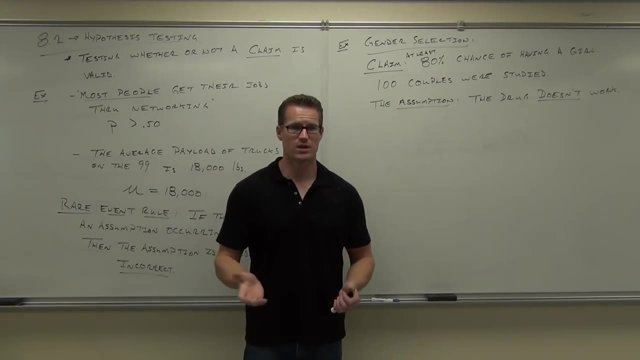 They never say that, do they? They don't say we find you innocent. No, what do they say? Not guilty, Not guilty. It's kind of a pessimistic way to look at it, isn't it? It says: well, either we have enough evidence to convict you or we don't. 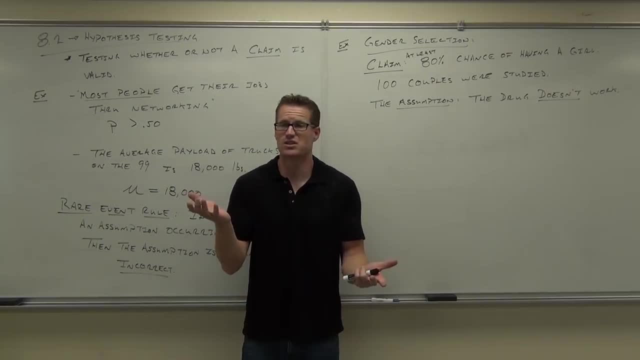 You might have done it in both cases, but here we had it. I'm not saying you're innocent, OJ did it, He did it, But he was found not guilty, wasn't he Right? So it's: either you have enough evidence to prove someone wrong guilty or you don't. 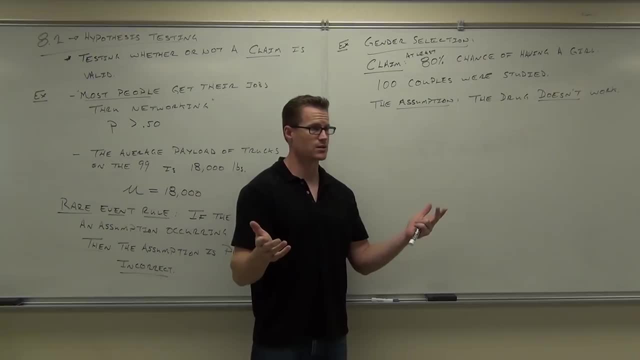 not guilty. You can't ever prove someone right, innocent. You can't do it In statistics. you can't prove anything right. So if you want to prove a statement true, you have to state the opposite of it and then prove that statement wrong. 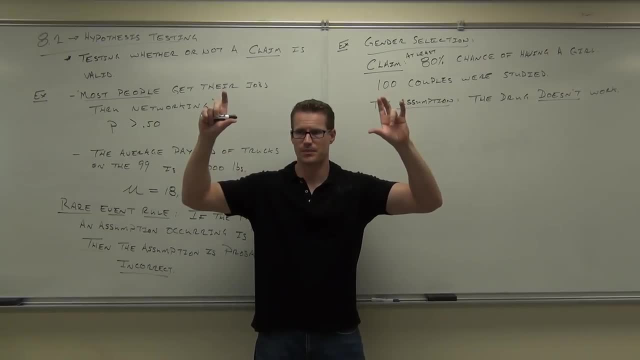 Do you see that idea? You can't ever prove a statement true, so you state the opposite of it and try to prove that statement wrong. That inherently proves your original statement true. It's a weird way of looking at it. I understand that. 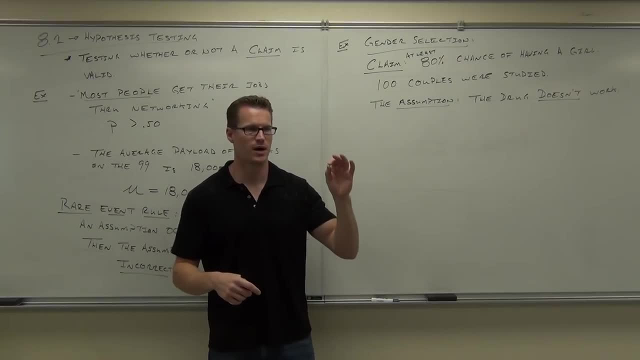 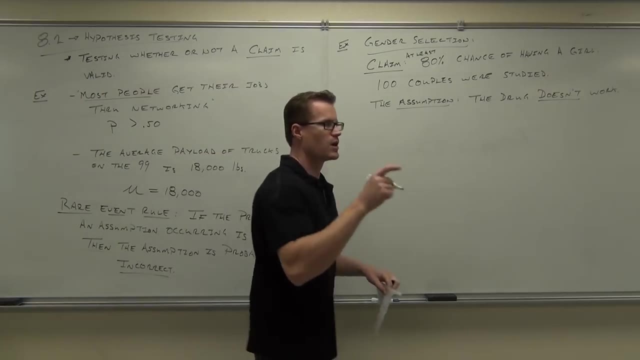 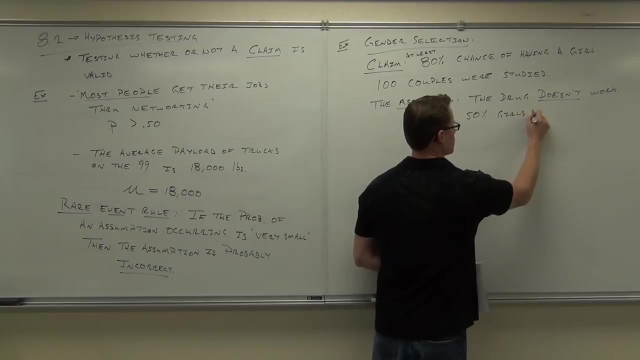 But know that statistics can't prove something right. It can only prove statements incorrect. That's all it can do. So we're going to assume the drug doesn't work. If the drug doesn't work, then that would mean 50% girls and 50% boys. 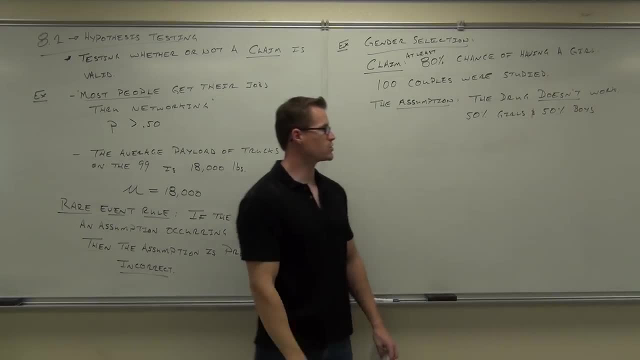 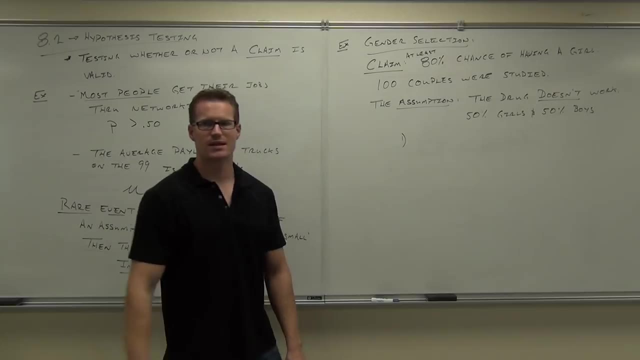 Remember, this is our assumption. We're going to assume the drug doesn't work. Okay, Let me give you two cases. Let's say this happened. Let's say they tested these 100 couples. You ready for this? You ready? 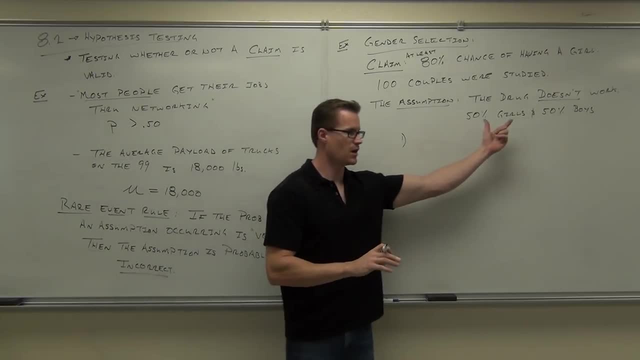 I hope you're with me on this. You understand the idea. that doesn't work. thing right, That we can only prove statements wrong. We can't prove statements right. Just check out how this would work. We're not actually into the math yet. 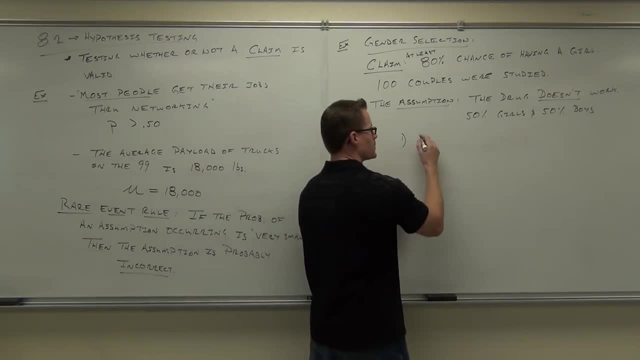 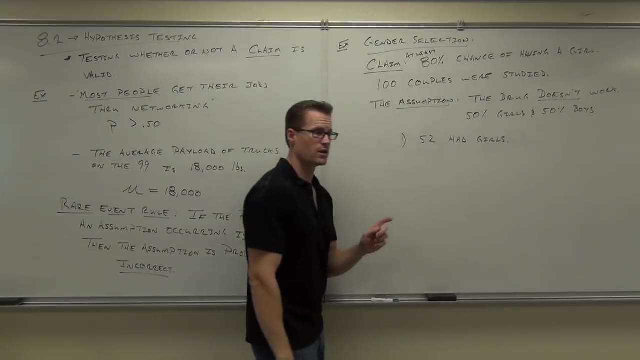 We're all in the theory. still, Let's say that these couples, 52 of them had girls Out of the 100, 52 of them had girls. The question is: is this number- remember this is out of 100, right? 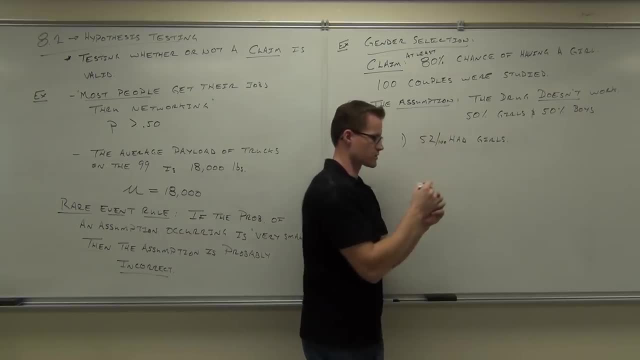 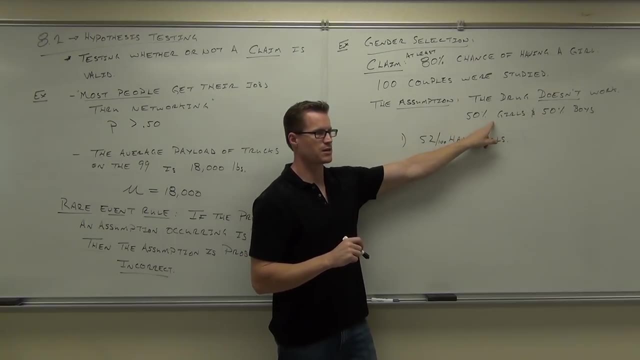 52 out of 100 had girls. Is this 52 different enough from this 50% to make this statement wrong? If I say 50, it's If I say 50-50, but we have 100 couples and I say you know inherently that it's 50% girls, 50% boys, right. 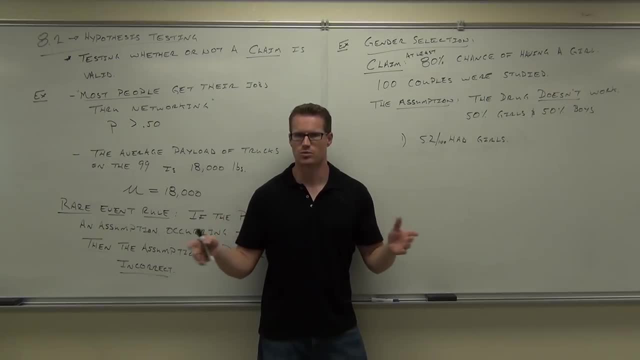 Without taking any drugs. there's a 50-50 chance you're going to get a girl or a boy And I say, okay, 52 of you had girls out of 100.. Is that usual or unusual? It would be pretty normal, wouldn't it? 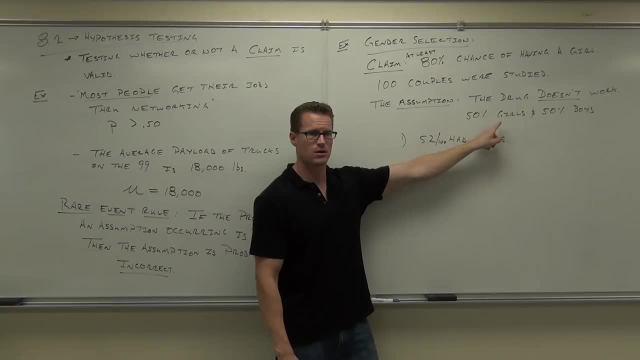 Is it different enough from this to prove that statement wrong? No, This would say. our assumption was the drug doesn't work. This doesn't prove that statement right, But it doesn't. It doesn't falsify that statement either. So we'd say, yeah, the drug probably doesn't work. 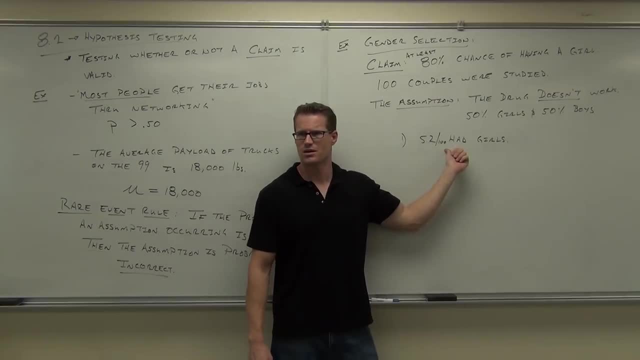 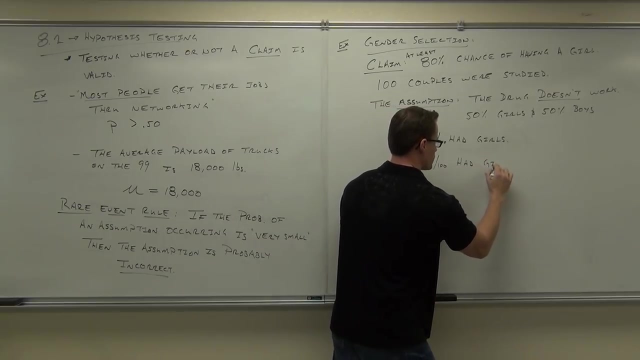 We can't prove it, But only 52 of them had girls. I mean, that's not good enough to prove that statement wrong. Are you with me on that? Now check this example out. Let's say that 97 out of 100 had girls. 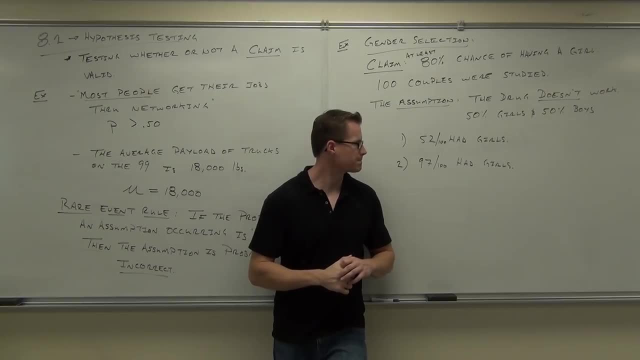 97 out of 100 had girls. Is 97 out of 100 way different than 50 out of 100? It's pretty significantly different, isn't it? If I said to you what's the chances, Think about this. 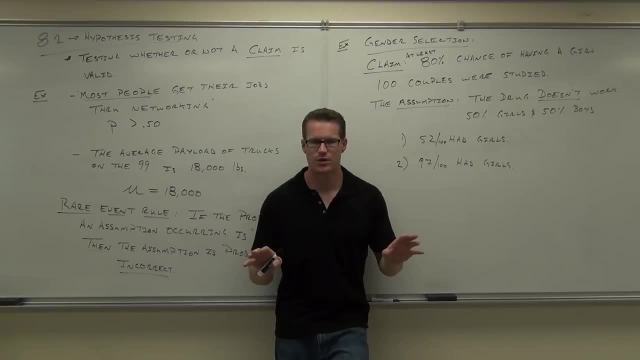 What's the chances that I didn't give anybody drugs or that the drug doesn't work and 97 out of 100 of them had girls? Is that rare? That's really really rare. This is way different than that one. This probability of this happening, assuming the drug doesn't work, is really rare. 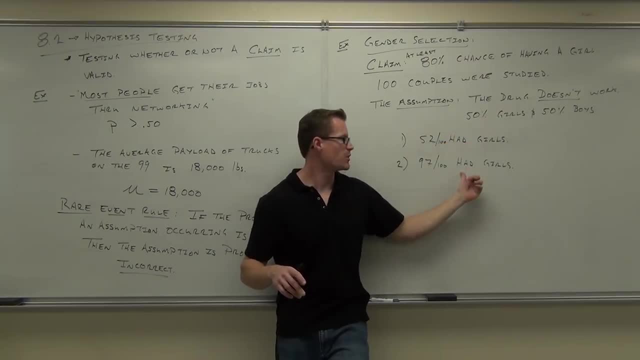 So what's it say about that statement? If the probability of this happening is rare, considering this statement, then this statement is probably false. So the statement the drug doesn't work is probably wrong. What's it say about the drug? 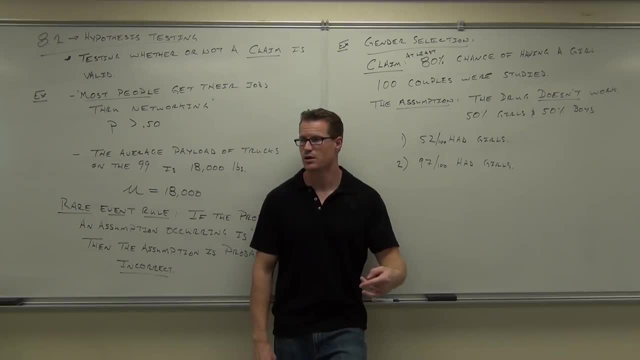 It works, It works. That's how you prove a statement true. You assume the opposite of it. You assume some statement that you can prove true or false, and then you try to do that. Sometimes you're not going to get enough evidence. 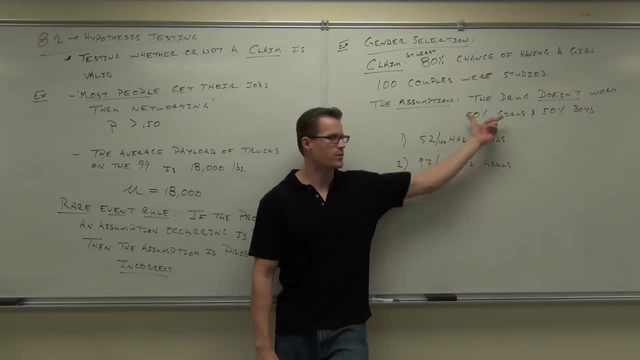 Only 52 out of 100 have girls. Does that prove that one wrong? No, It doesn't say anything. This would do nothing for you, But this one, that's a rare thing. That's a rare thing considering your statement. 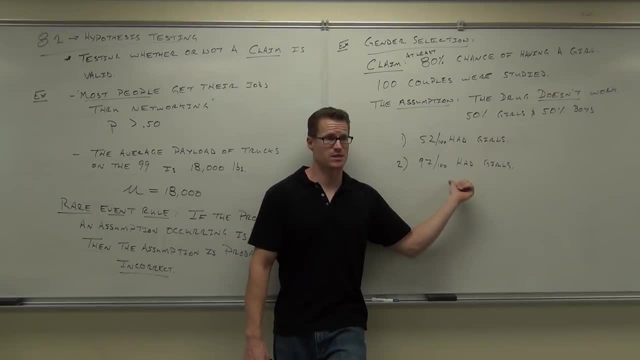 If the drug didn't work, this wouldn't happen. Does that make sense to you? That wouldn't happen in real life If you compared the 100 people with the drugs to the 100 people without the drugs. that's not going to happen to people without the drugs. 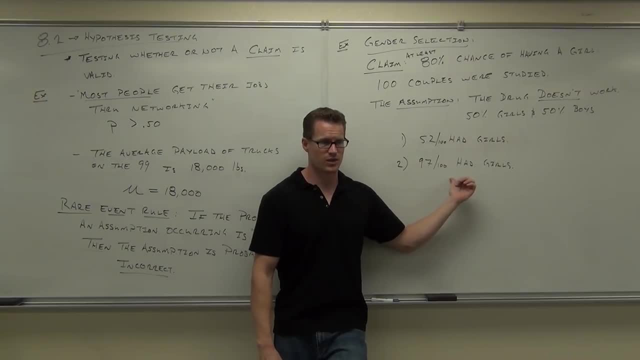 It's going to be really close. It's going to be like that. So this action, this occurrence, is very rare. That says your assumption's probably wrong. If your assumption's wrong, the drug doesn't work. If that's wrong, then the drug does work. 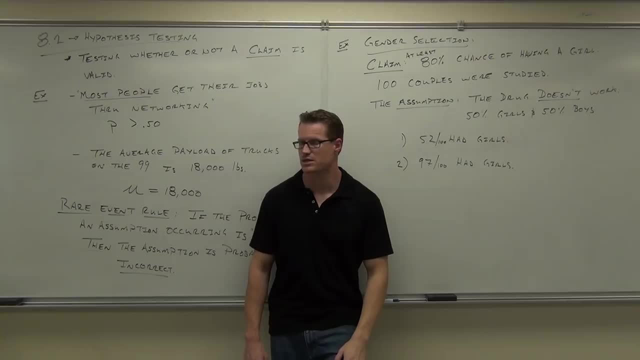 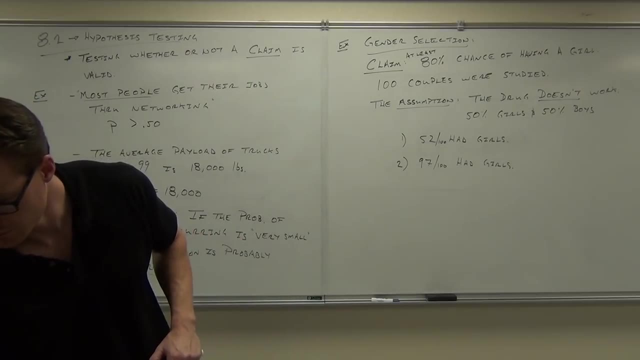 And that proves that claim that at least it'll give you an 80% chance of having a girl. How many people understood the idea of this hypothesis test? Good, Now, that's an overall rundown. What we're really doing is comparing the probability of things occurring. 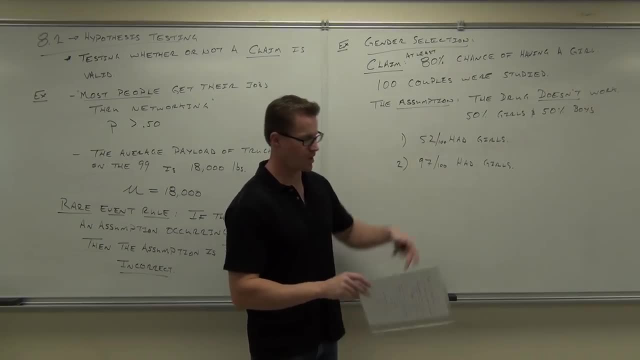 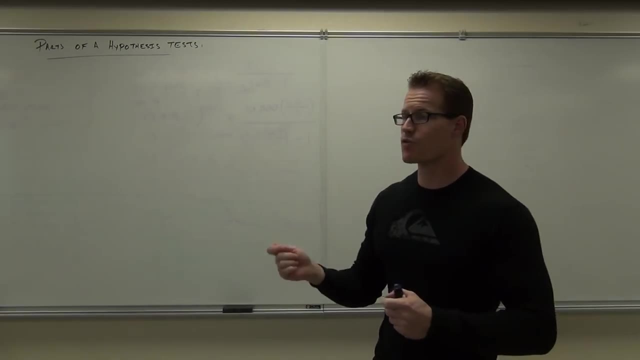 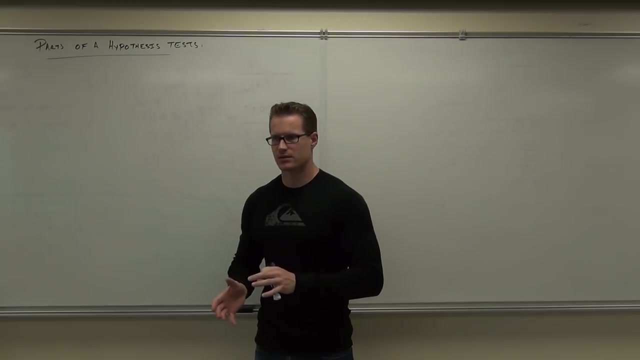 If the probability is rare enough, the assumption's probably wrong. So we are still talking about the introduction to hypothesis testing And, if you remember from the last time we did this, what we're trying to do is to prove a claim incorrect or prove a claim correct by stating that some claim had proven it wrong. 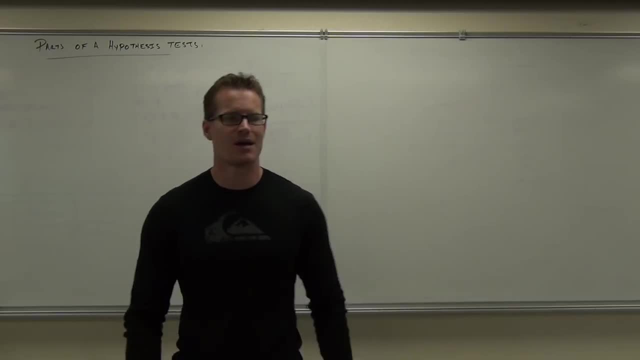 thereby proving our argument incorrect. It's kind of a backwards way of doing things. I made the analogy that this is like when you're in court: You can't ever prove someone innocent right. You can't guarantee they didn't do it. 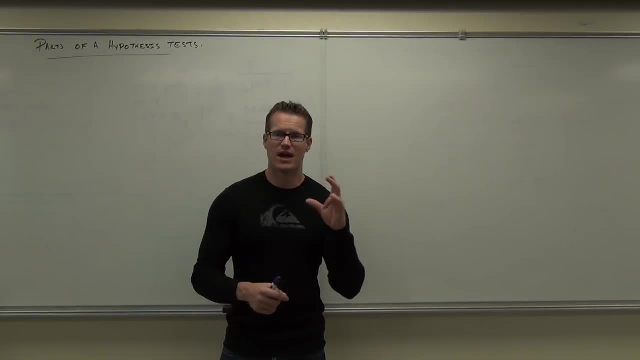 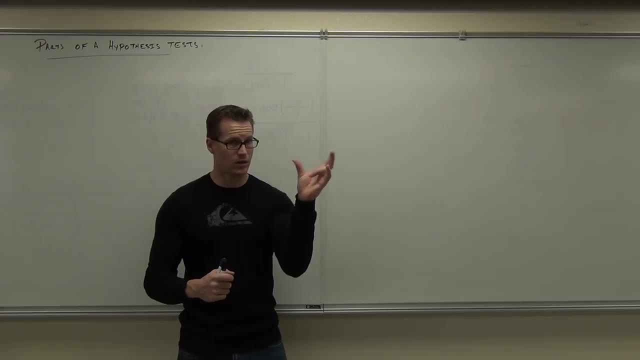 All you can do is prove them guilty or not guilty. Either you have enough evidence to prove it or you don't. You either have enough evidence to condemn them or you don't have enough evidence to condemn them. We are either going to have enough evidence to condemn our claim or not have enough evidence. 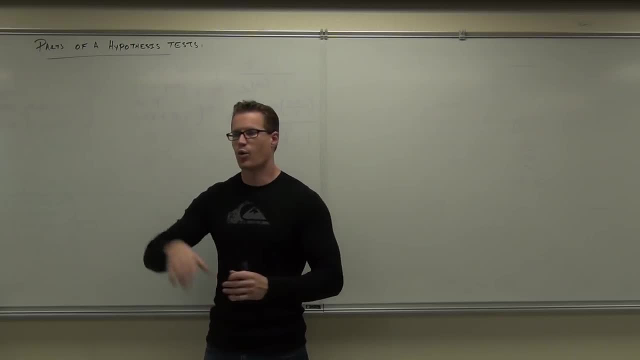 to condemn our claim and therefore can't reject it. We're either going to reject or fail to reject our claim. We're never going to be accepting claim. This next part I'm going to tell you about is called the hypothesis. With hypothesis testing, you actually have two hypotheses. 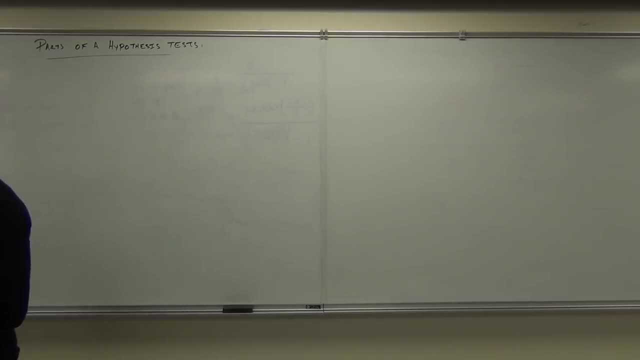 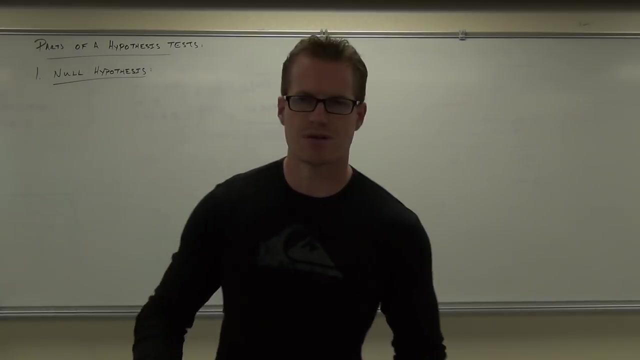 We're going to be having something called a null hypothesis, the null hypothesis and the alternative hypothesis. We'll talk about that in just a second, But let me give you kind of the characteristics of the null hypothesis When we talk about the null hypothesis. 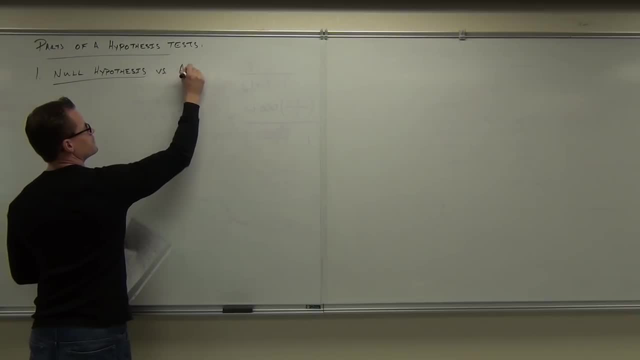 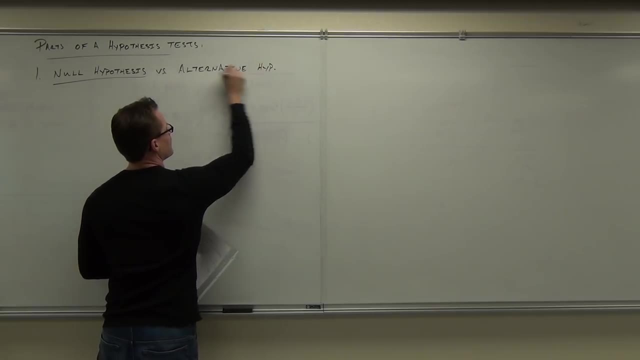 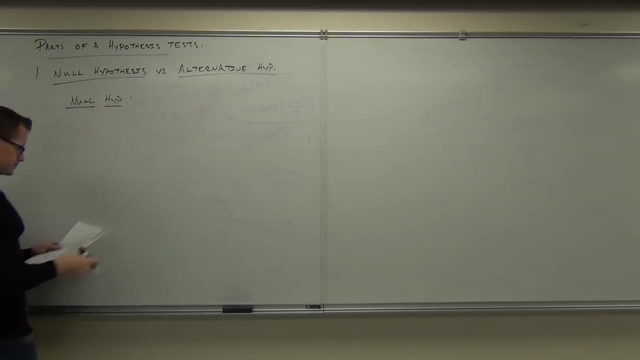 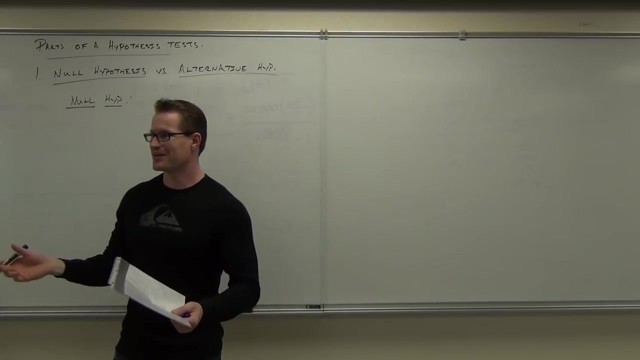 I'll put up here two versus the alternative hypothesis. When we talk about the null, we'll do that first here. null hypothesis. we're going to denote that with a special symbol. This seems kind of appropriate for the season. It is H sub zero. 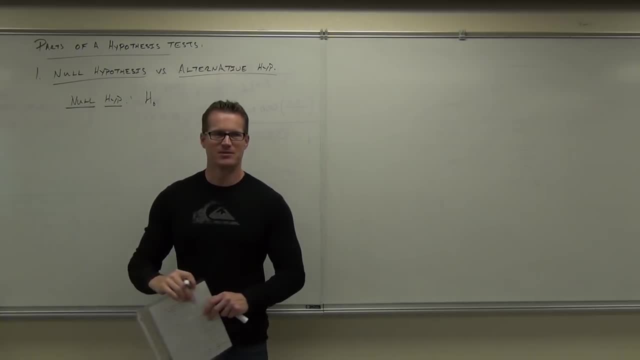 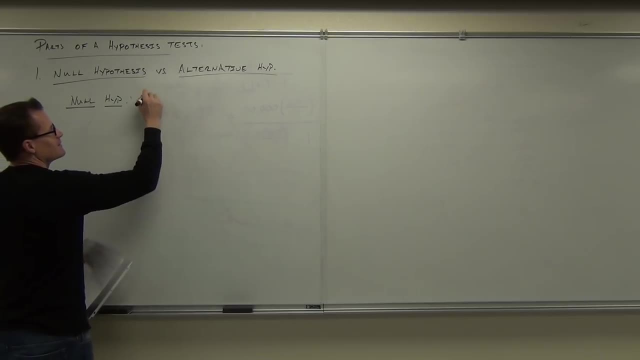 It looks like ho, ho, ho, ho, Not the other type of ho. all right, Sick people. Yeah, it's H sub zero. We don't say ho. Some classes do. They say ho and ha. It's funny. 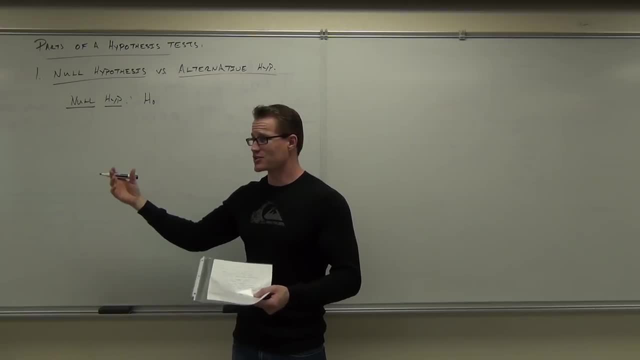 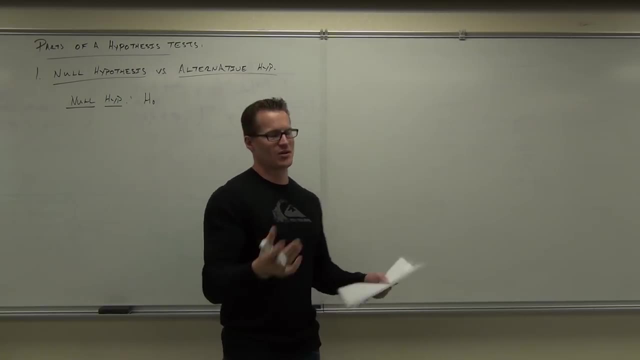 Ho for the null, and then alternative has a little a right. So ho, ho, ha ha, We're going to do H sub zero and H sub one, the null hypothesis and the alternative hypothesis. That just seems a little bit less funny. 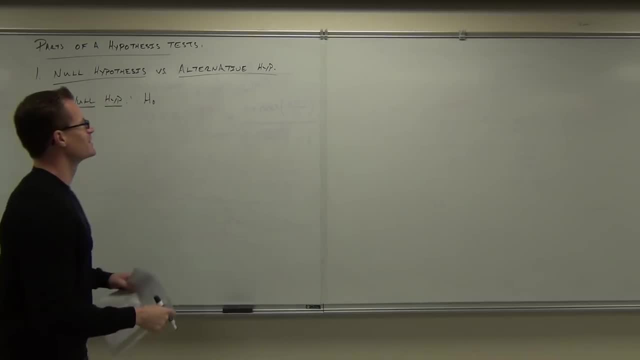 We're going to be more serious, so we can echo serious statistics students. But this is how you write it. It's denoted H sub zero. It stands for the null hypothesis. That's it What this does. this is a unique idea. 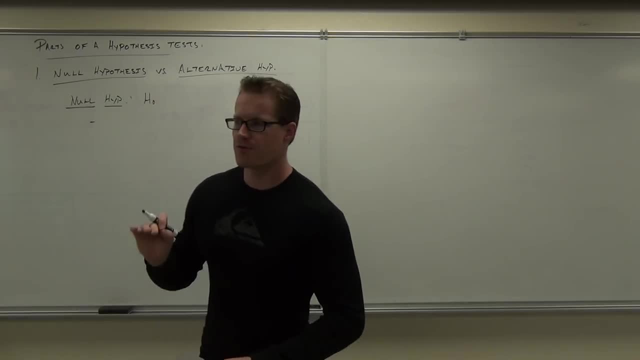 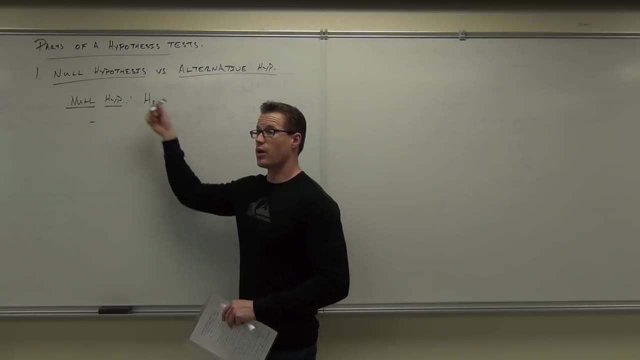 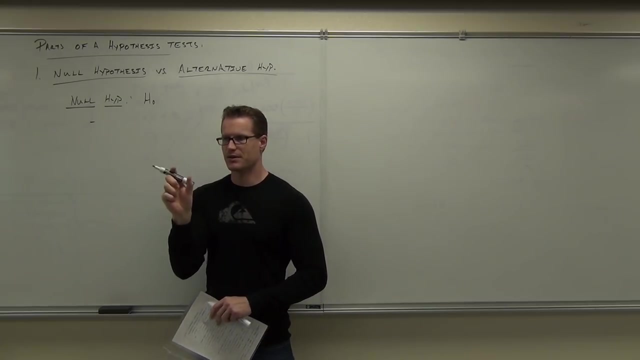 This is always going to be a statement that reflects some population parameter is equal to a value. This is a statement of equality. So when you talk about the null hypothesis, you must absolutely have an equal statement in there. Do you understand? The null hypothesis will have an equal sign. 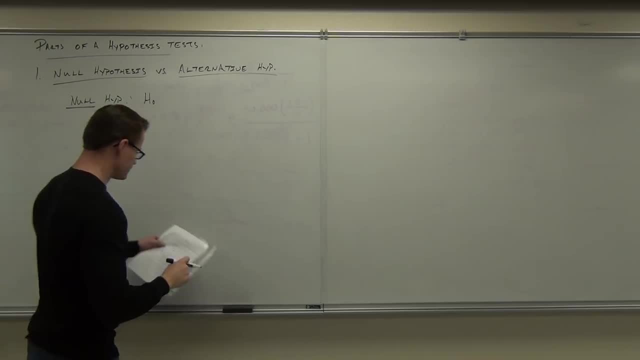 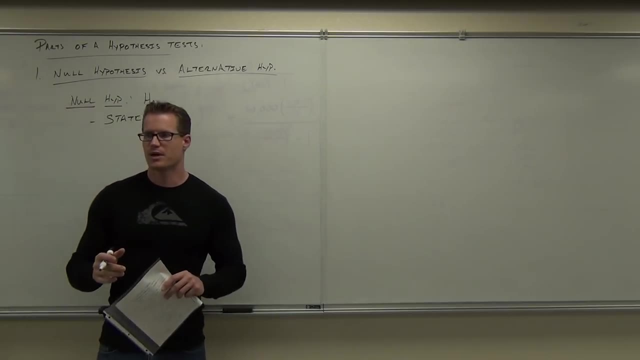 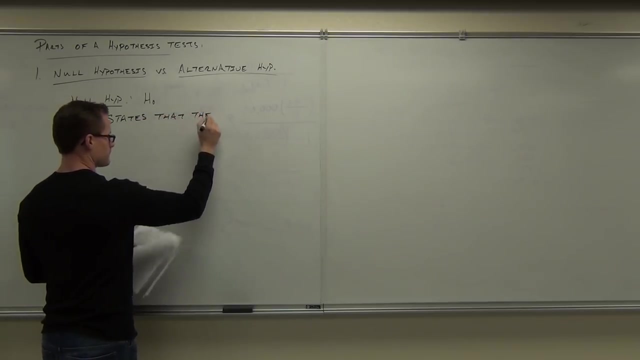 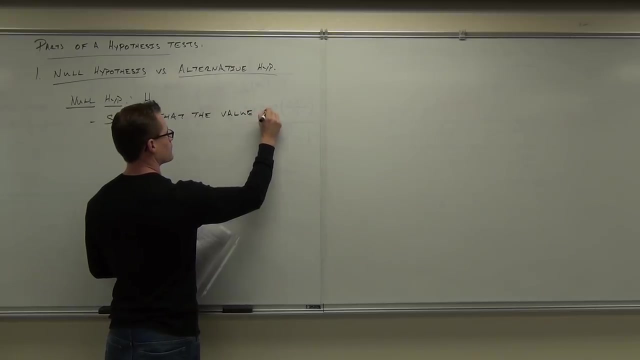 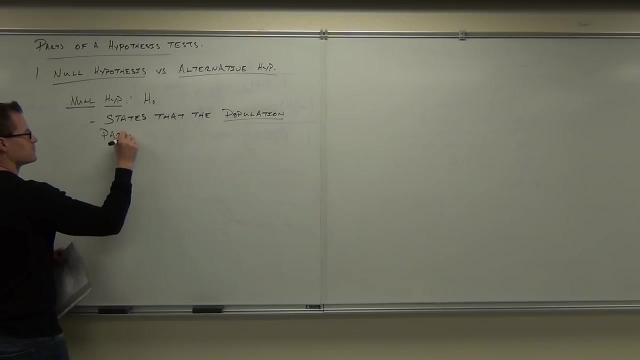 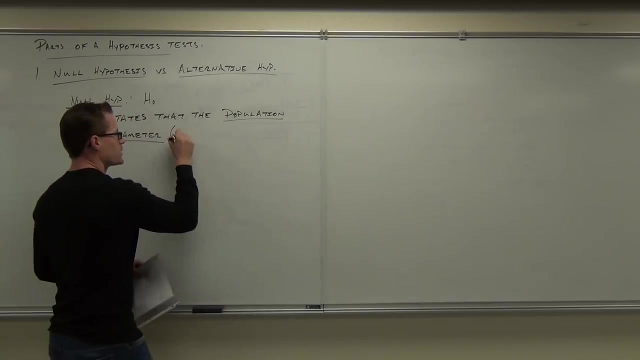 It's a statement of equality. It says the population proportion is equal to some value, Or the population mean, Or the population standard deviation. It's some parameter. It states that the population parameter- remember the population parameter- in our case, we can talk about the mean or the proportion. 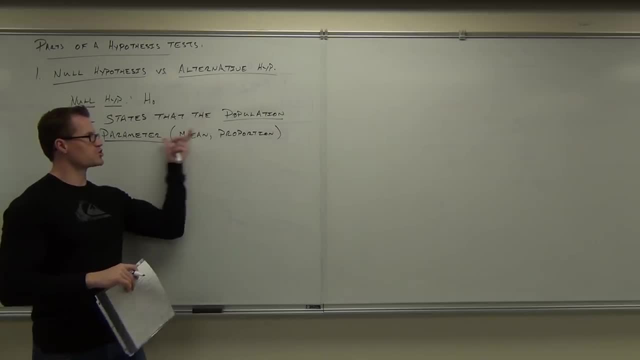 Ladies and gentlemen, what symbol do you use for the population? mean Mu Mu? So we're talking about mu's here. How about for the population proportion? P? P With a hat or not? No hat, No hat, That's population. 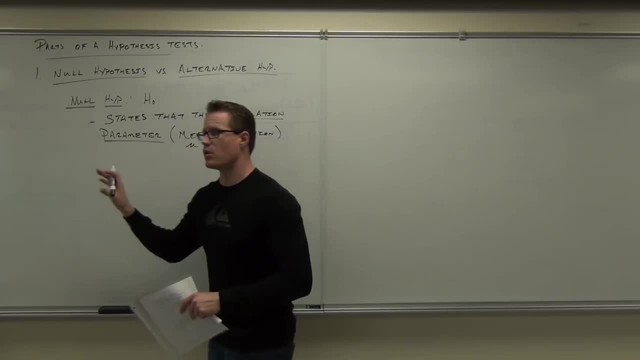 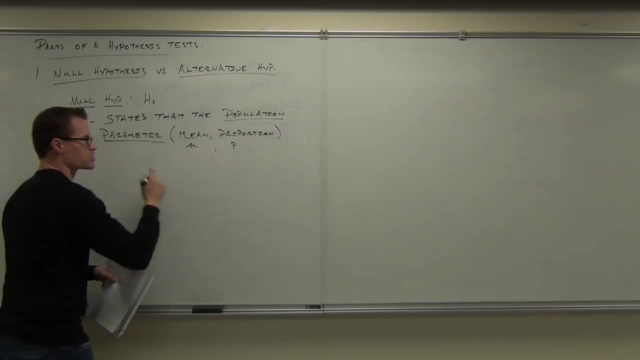 So we're talking about mu's and p's. That's what we're talking about. as far as the null, We're going to have these things equal to some value. So it states that the population parameter, either mean or proportion, is equal to some value. 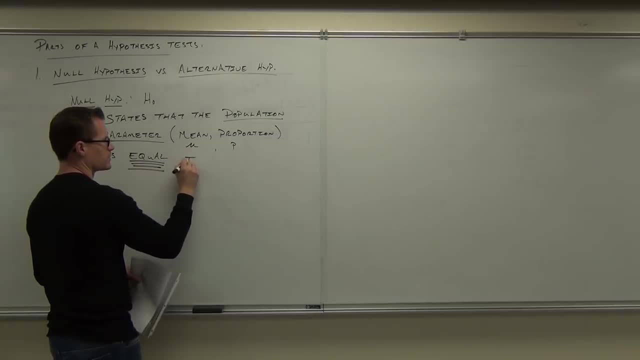 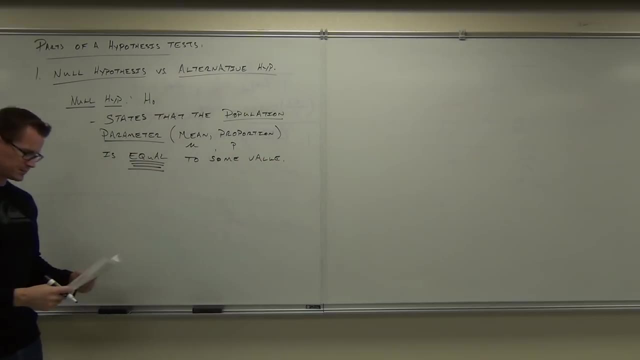 Equal to some value. Let me give you an example, Just a simple example here. Here's how your null hypothesis will look. when you're doing this First example, you'll have H sub zero, with a colon there. You'll have some statement. 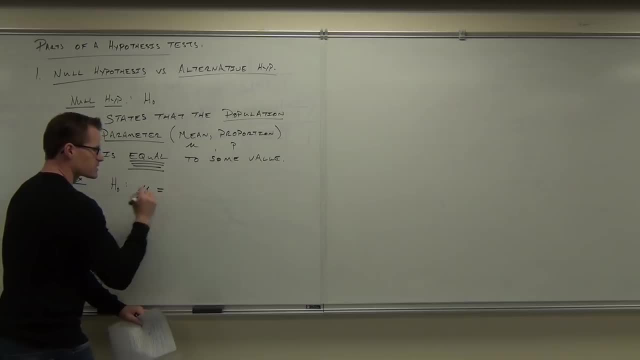 Like, let's say we're talking about the mean, We'd have mu. It's just going to say: let's suppose that the mu is equal to five. That could be a null hypothesis. Notice how we have some population parameter. It's the mean this time. 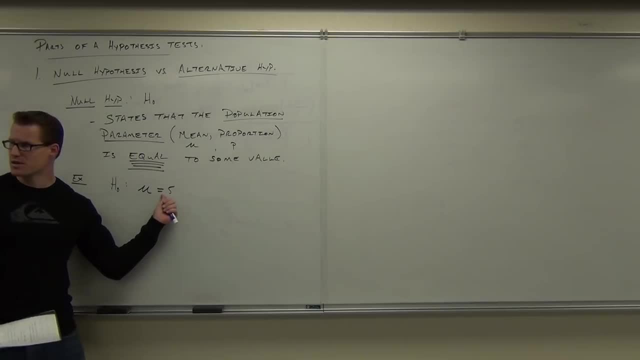 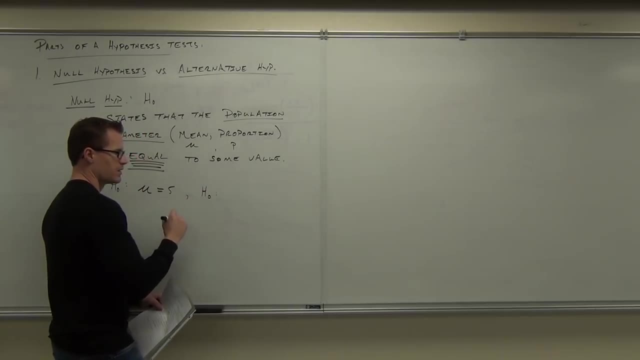 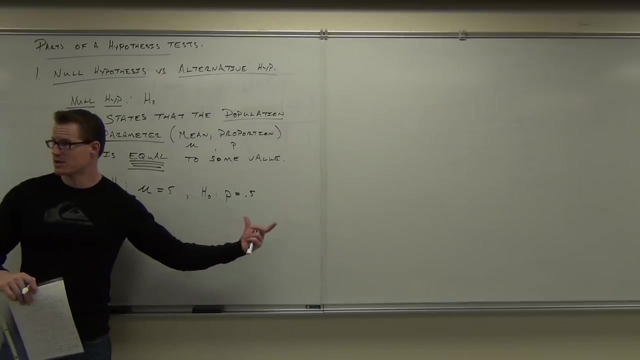 It's equal to some number, So that equality that has to be there. that's always going to happen. for the null hypothesis, If you're talking about the proportion, you would have p equals like I don't know- .5. The proportions have to be decimals. 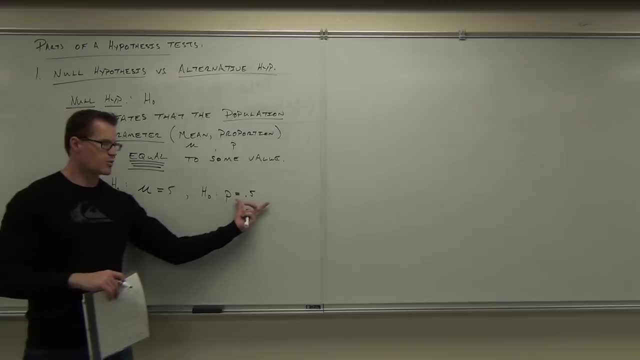 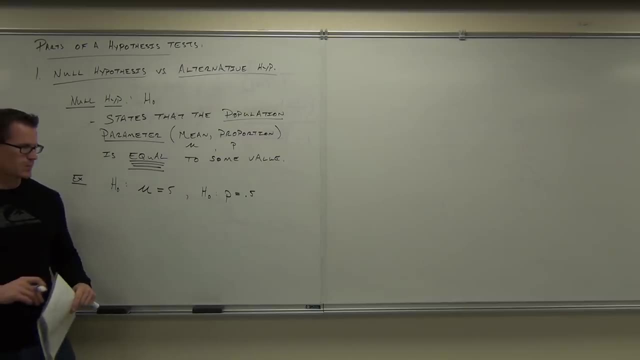 And means don't have to be decimals Less than one. So proportion you're going to have to be between zero and one. Means that necessity isn't there. You OK with this so far. So we just have these things called null hypotheses. 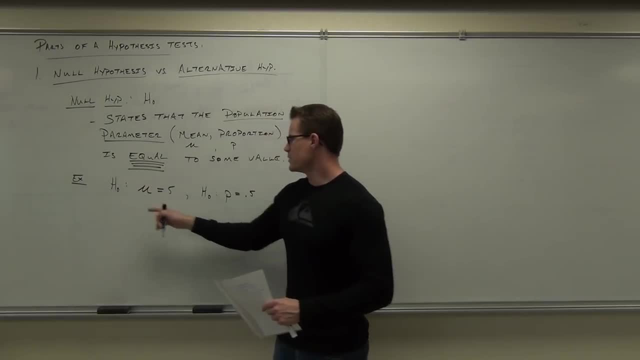 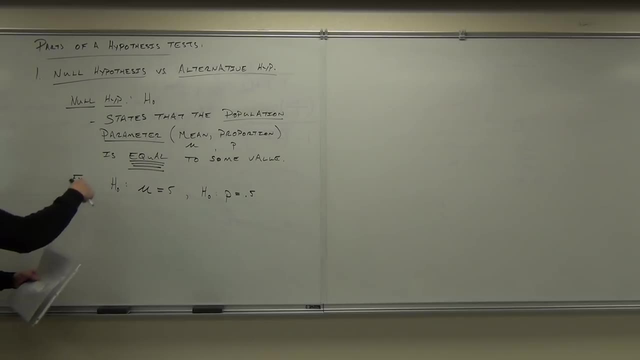 We know that it's going to have some parameter- mu or p- and it's going to be equal to some number. Now, this is always how we do a hypothesis test. This is going to be a little bit of a recall for you. 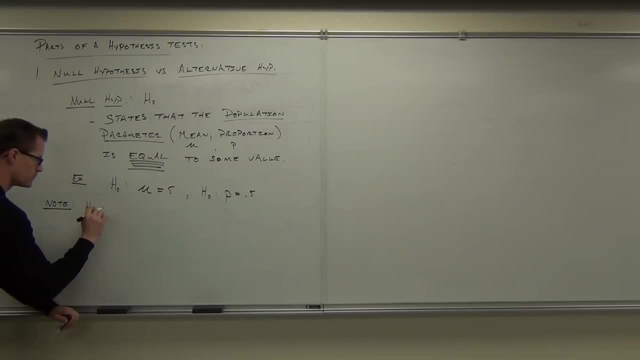 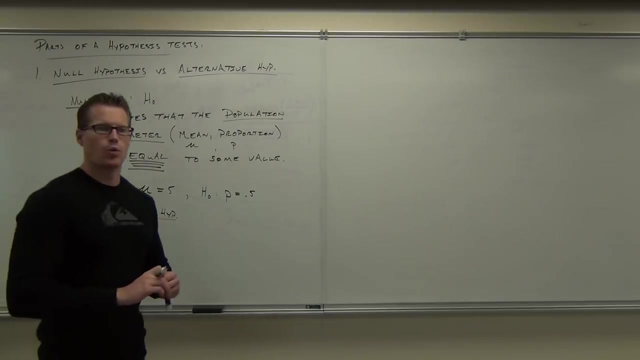 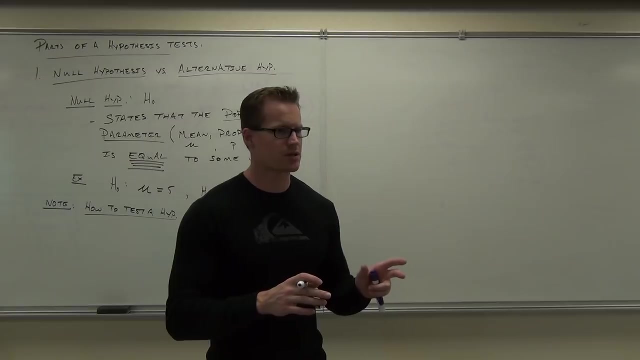 This is how we do it, How to test hypotheses, What you're going to do here. this is the interesting part of hypothesis testing. You are going to assume, we're going to assume this is true If we come up with evidence that's not true. 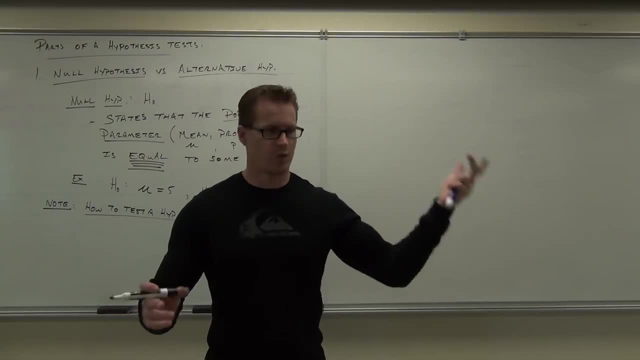 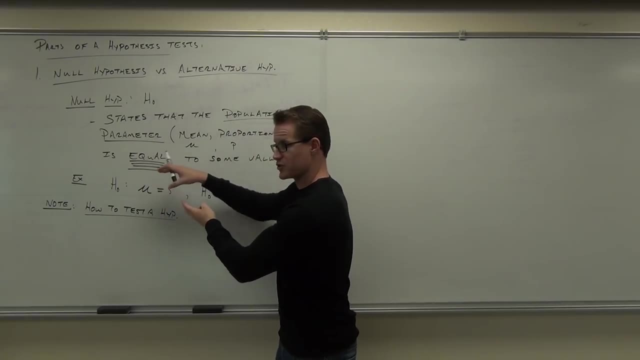 we're going to reject it If we don't come up with evidence. well, we can't assume it's wrong. Here's what you do. You assume that this right here is true. You assume that the null hypothesis is always true. 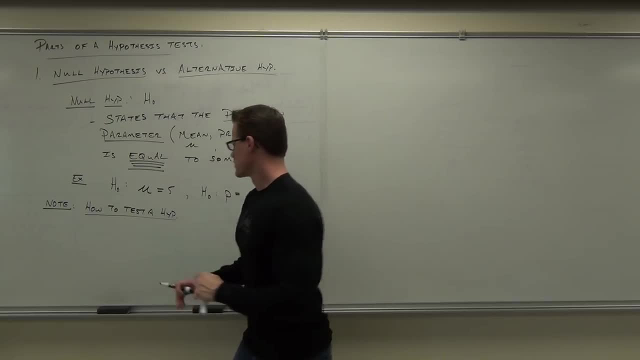 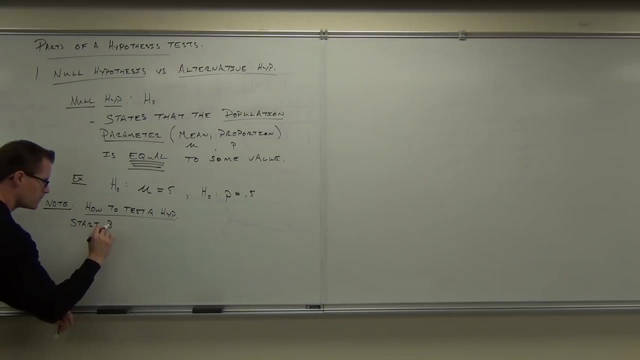 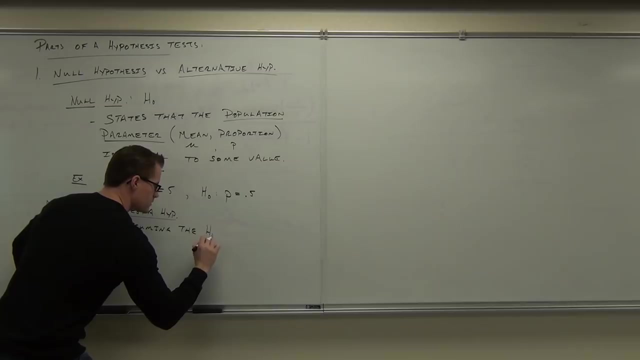 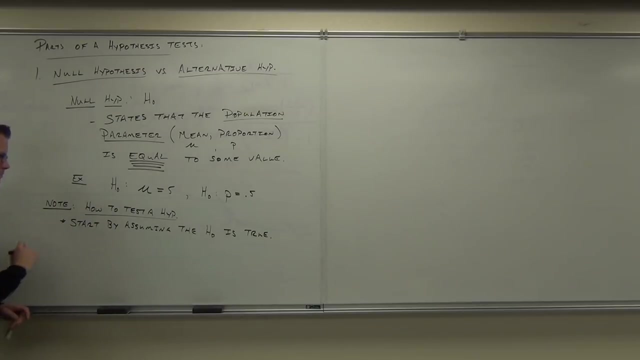 And then you work to reach a conclusion. So how you do a hypothesis test. you begin by assuming the null hypothesis- H sub 0, is true. You start by assuming the null hypothesis is a true statement. Then you use evidence to reach one of these conclusions. 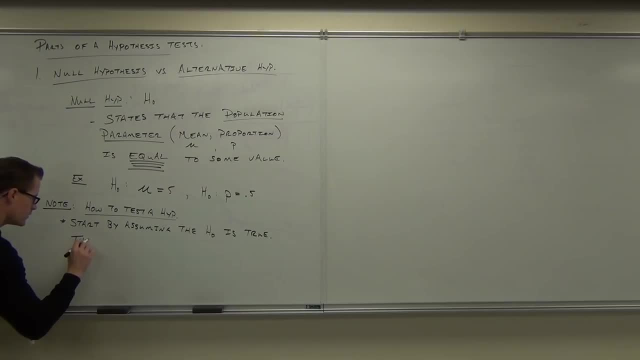 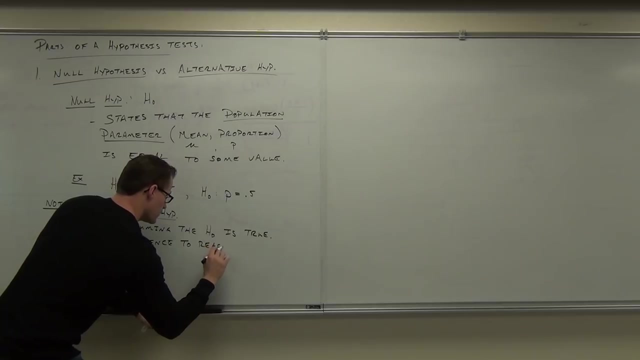 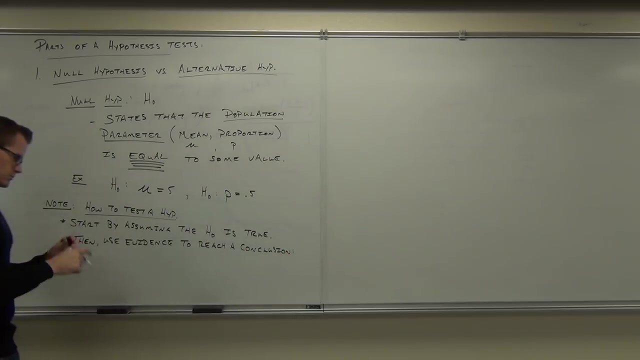 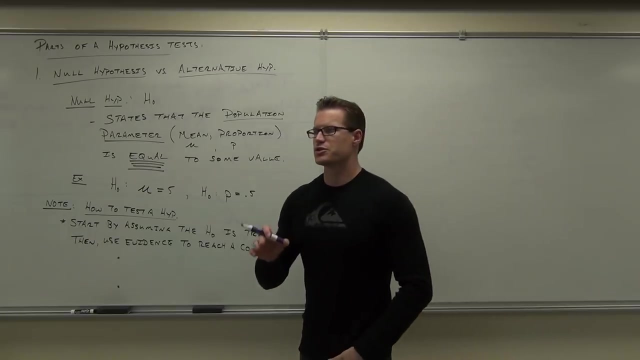 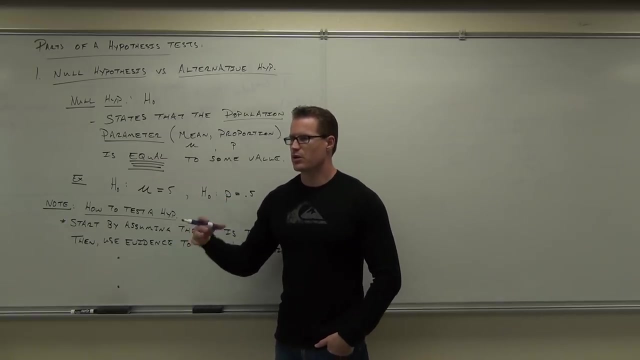 Evidence, by the way, is given to you by your sample. Here's your two options. They're going to be given to you by your evidence. 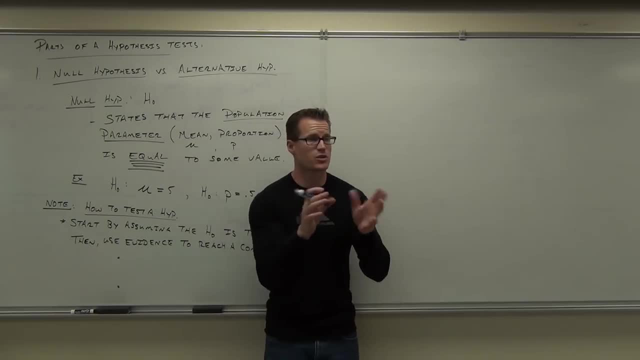 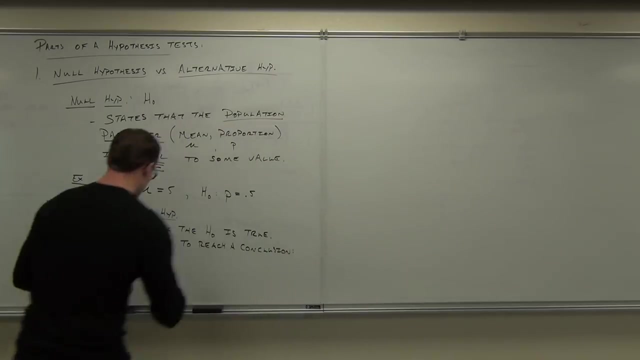 You can't ever prove someone innocent. You can only prove them guilty or not guilty. Either you have enough evidence or you don't. Here's what that comes down to for us. Either you're going to reject the null hypothesis. 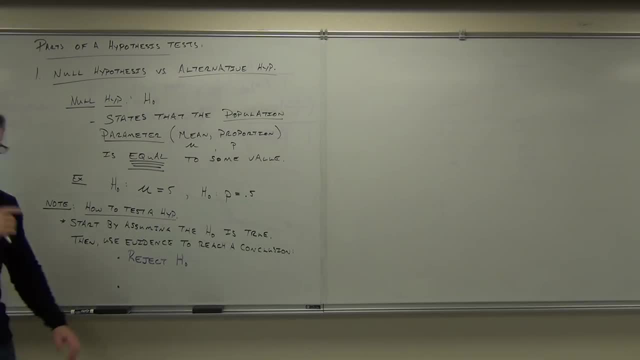 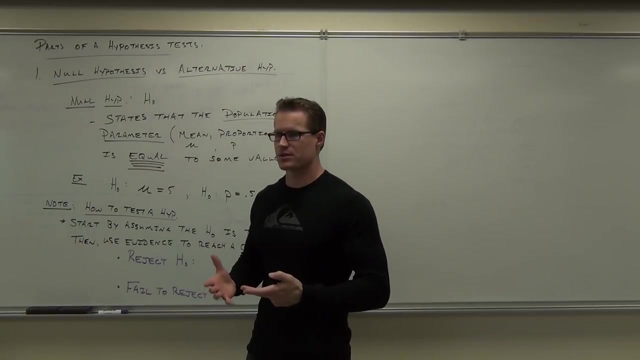 or you're going to fail to reject the null hypothesis. That's it. Are you ever going to be able to accept the null hypothesis? No, never. You're never going to be able to do it Because you're never going to have enough evidence to prove it. completely right. 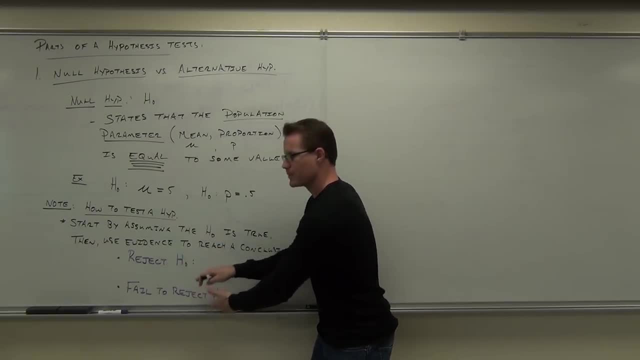 All you're going to have enough evidence to do is to prove it wrong or not be able to prove it wrong. It's kind of a pessimistic way of looking at things. You can't ever prove that claim right, But that's the way the courts work too. 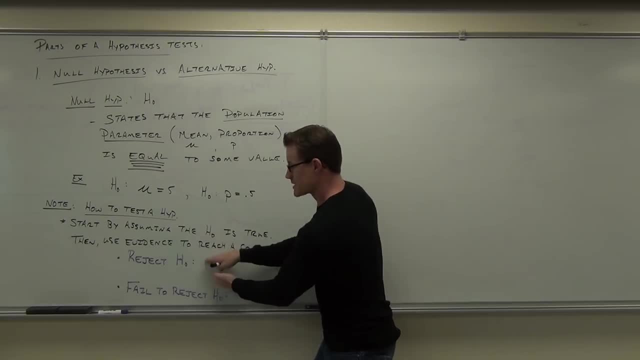 You can't ever prove anybody innocent. You can only prove them guilty. This is guilty. You have enough evidence to say it's wrong Or not guilty. You don't have enough evidence to say it's wrong. Does that make sense to you? 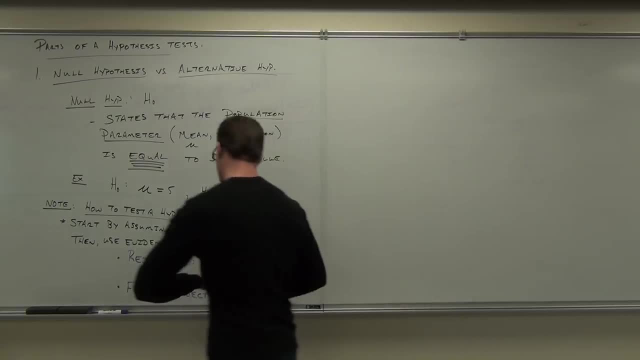 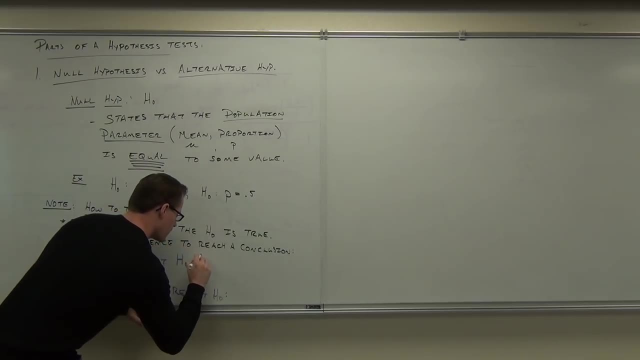 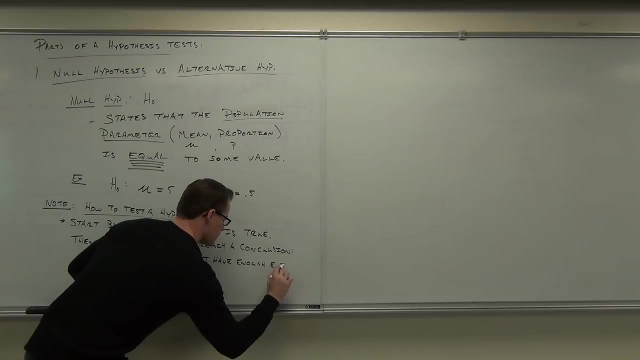 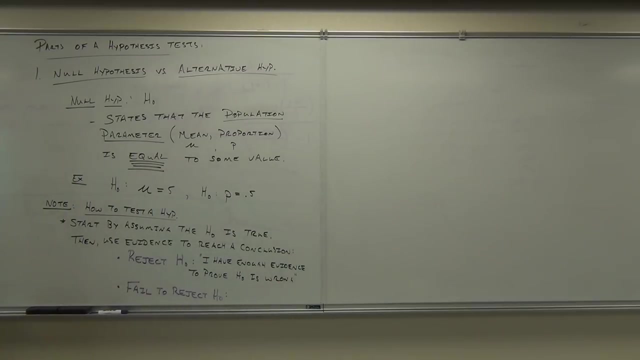 This is our whole theme for hypothesis testing. So rejecting A sub 0,. here's what this says in English. It says: I have enough evidence to prove this statement wrong. I have enough evidence to prove H sub 0 is wrong. Here's what this says. 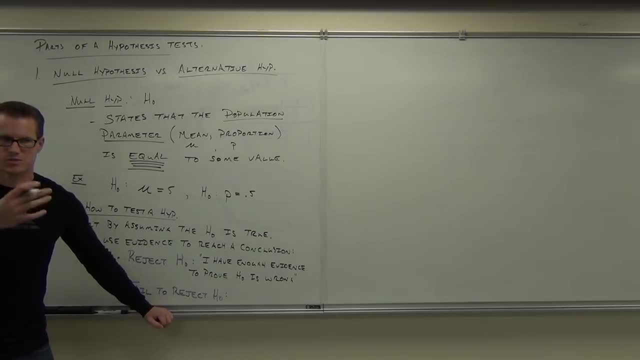 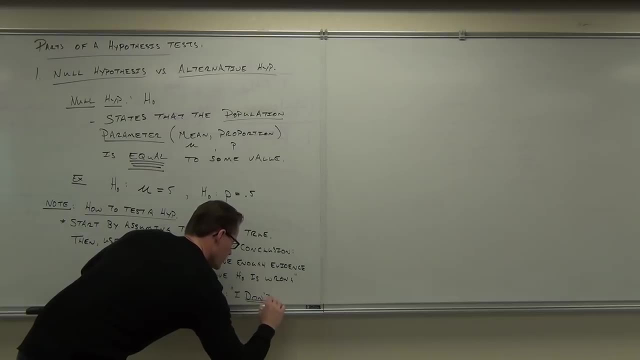 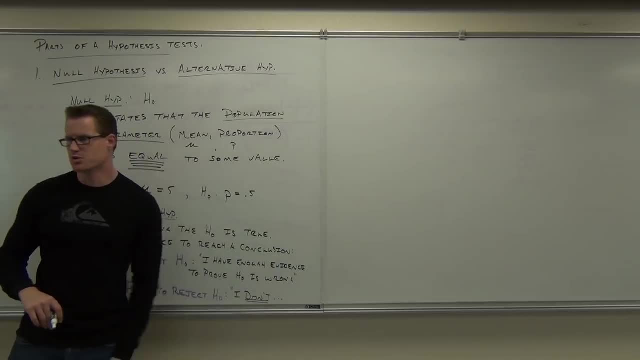 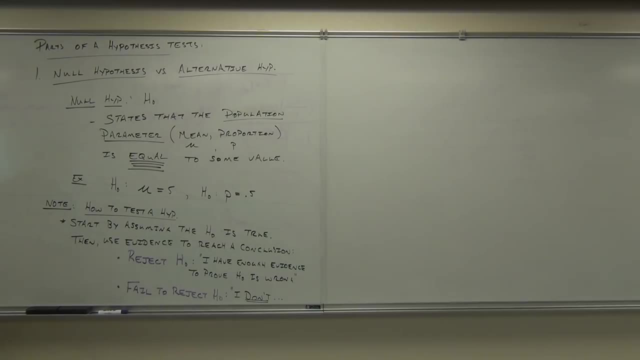 I don't have enough evidence to prove H sub 0 wrong. I don't have enough evidence to prove H sub 0 wrong. I don't- And then finish that off- have enough evidence to prove H sub 0 wrong. So little side note over here. you cannot accept H sub 0,. 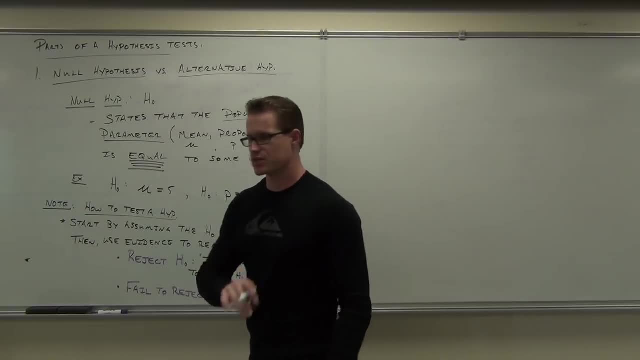 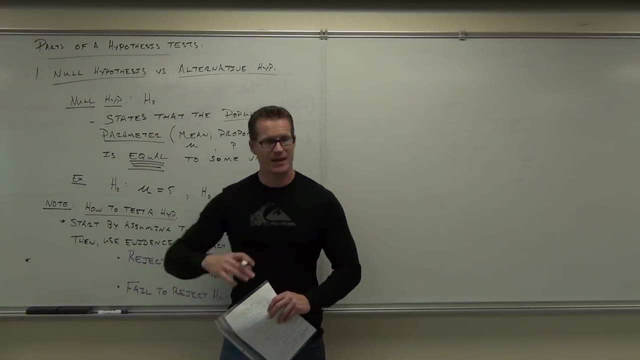 it's impossible. You're never, ever going to accept H sub 0. You can only reject it or fail to reject it. Failing to reject it doesn't mean that you accept it. That's a common misconception for statistics students. They go: oh well, this one's right. 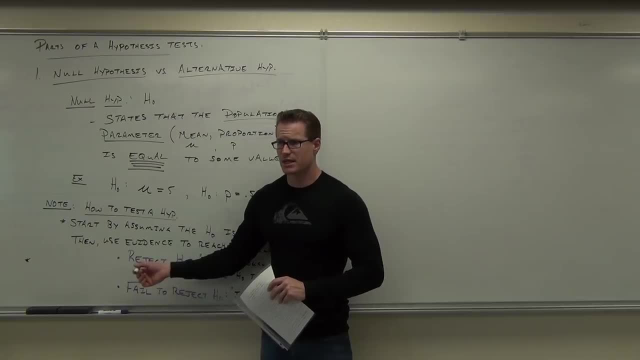 means you reject it and this means you accept it. no, no, you reject it, saying it's dead wrong, or you fail to reject it. that's not saying it's right. right, remember the the court system when you think about this. remember the court system: either it's guilty, they're going to jail, or they're not guilty. they're. 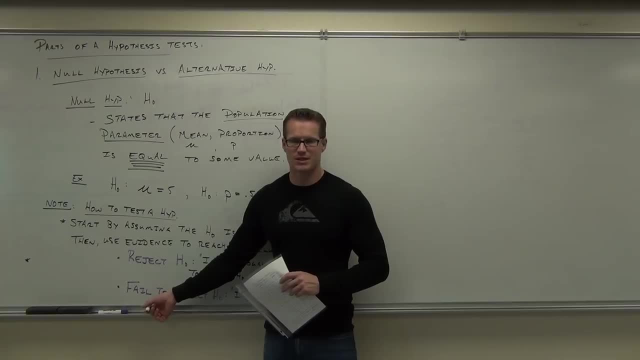 not going to jail. but does that mean the person definitely didn't do it? no, remember OJ, he, he did it, he did it. he wrote a book saying: I here's how, if I didn't do it, but if I did, here's how I did it. okay, he did it, but that's what. 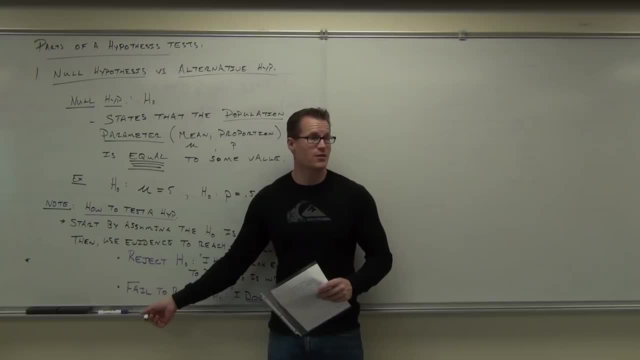 this says: okay, he might not have gone to jail, but he definitely did it. there just wasn't enough evidence to convict him. it didn't say he was innocent. someone who is not guilty might not be innocent. there just wasn't enough evidence to put them into prison. do you understand the difference between being innocent and 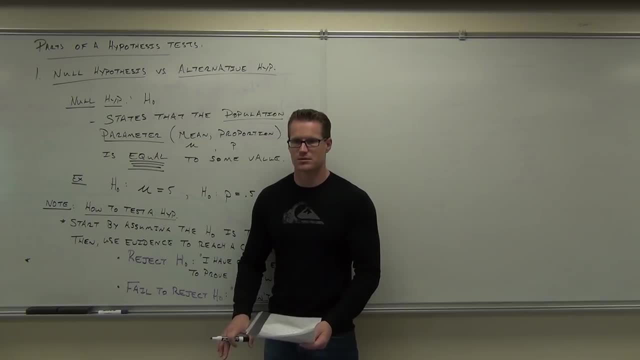 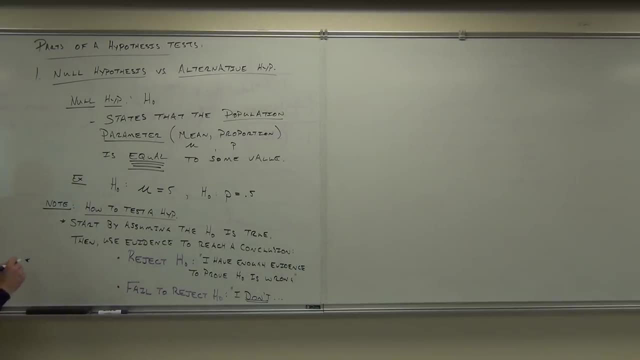 being not guilty. yes, no, okay, that's. that's the idea here. you can't ever accept h20. you can just prove it wrong or fail to prove wrong. you cannot accept h20, okay. well then, why in the world are we doing this, if all we're doing is: 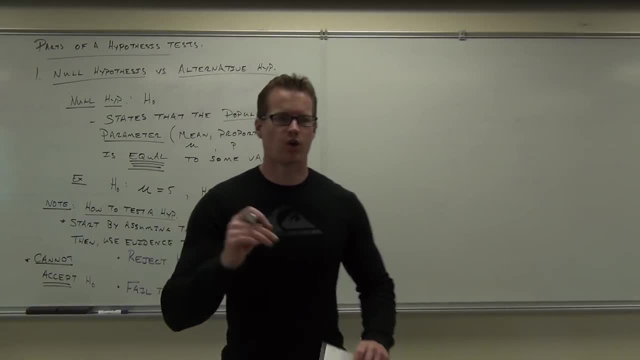 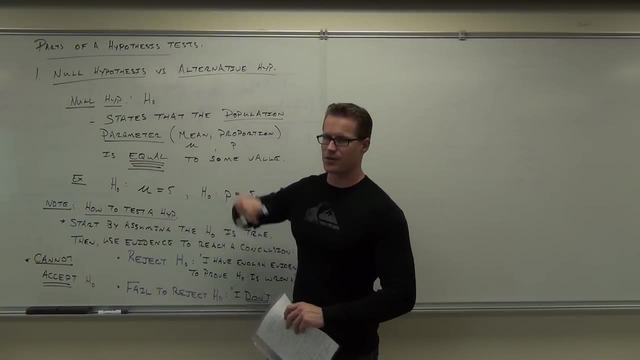 proven statements wrong. well, here's the cool thing about this: we're gonna have another piece of this puzzle. we're gonna also have not only the null hypothesis, but the alternative hypothesis. so let's take a look at that and see how these things interplay between each other. 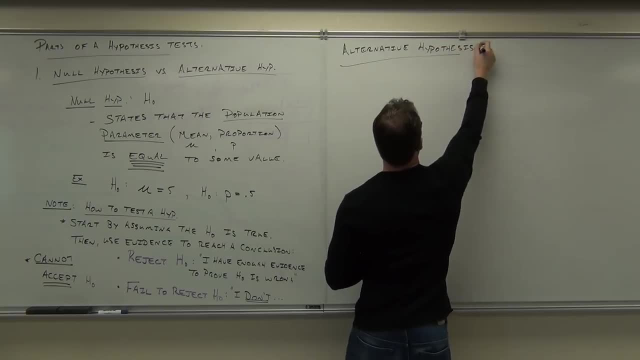 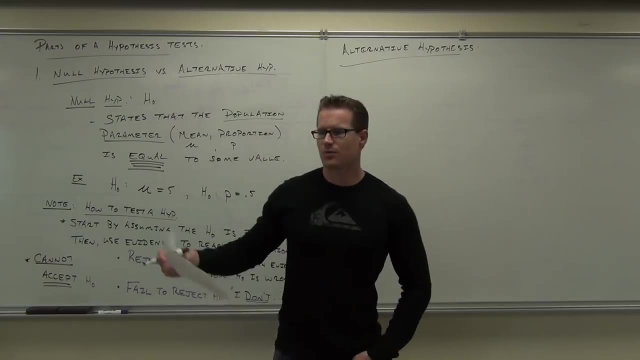 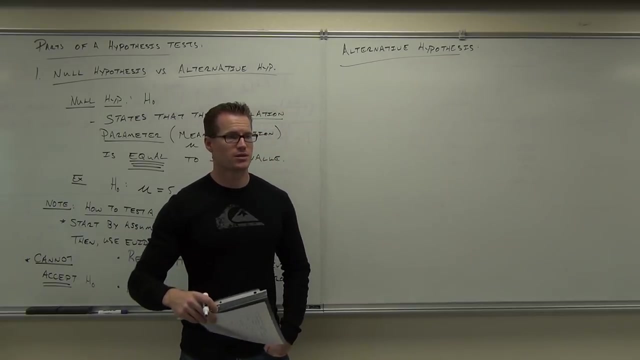 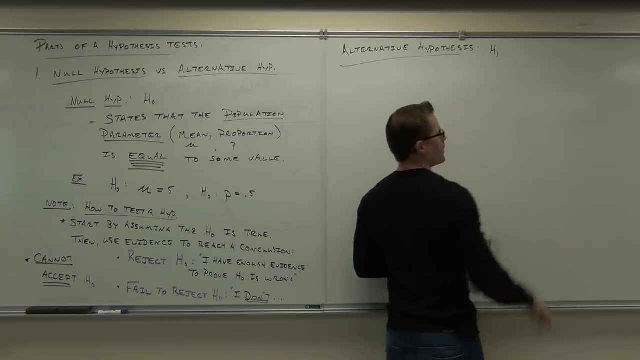 if H sub zero means the null hypothesis, how are we going to write the alternative hypothesis? some books do use a Sabe, they do. they do follow in hop the null hypothesis and the alternative. we're going to use H sub one because we want to be proper, not have fun, right? basically know it's. working with something else. if it's, you know, if it's an alternative, hypothesis clauses. we're going to use price rhymes. we're going to use tropics for all nudes, any 적 slightest options檤 songs. 1 because we want to be proper, not have fun, right, basically no, this is what we have much more to do: work with the many things we find, if not everything, is a necesario. ver Fedl Correccional, a series of rendition. 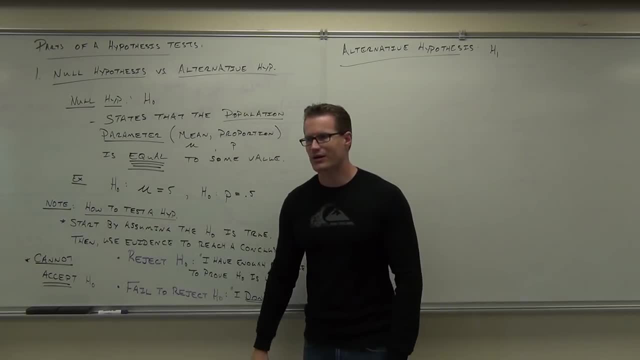 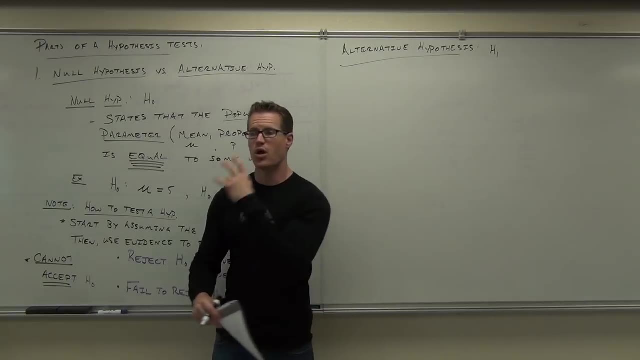 which means the other hypothesis, the alternative, If you think about binary zero one. that's the two different options you have. okay, There's the null hypothesis. that's the statement of equality. The alternative hypothesis is going to be the opposite statement of this thing. 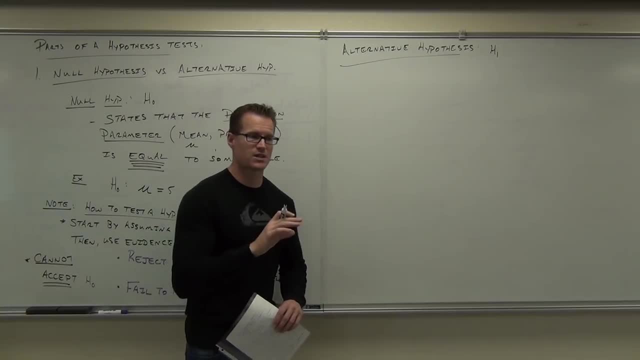 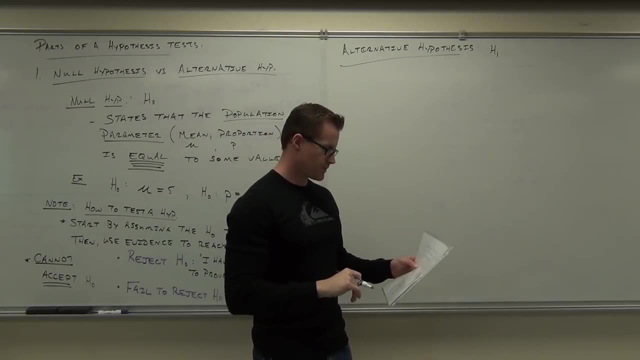 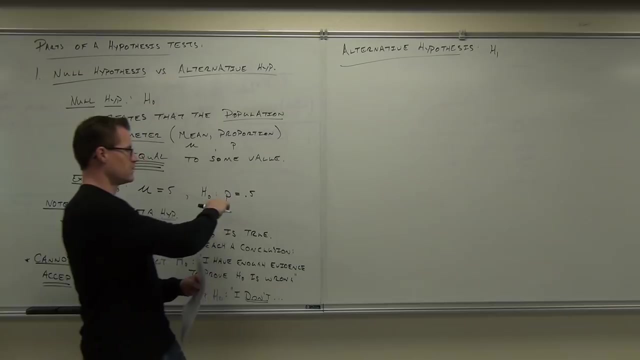 It's not gonna have an equal sign in it. It's gonna have one of these symbols: either less than, greater than or not equal to. The equality goes here: H sub one has the value. the parameter is different than the state that the H sub zero has it. 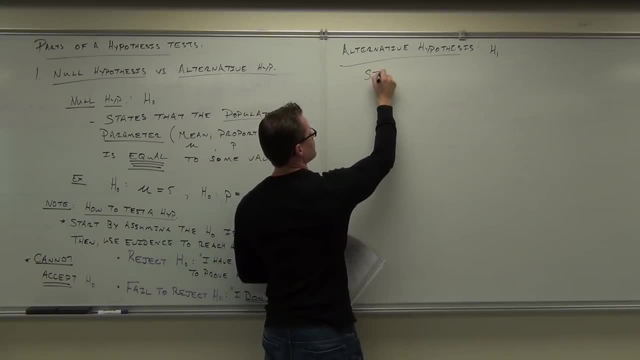 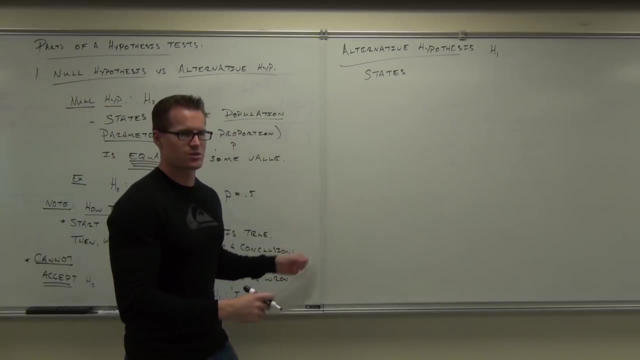 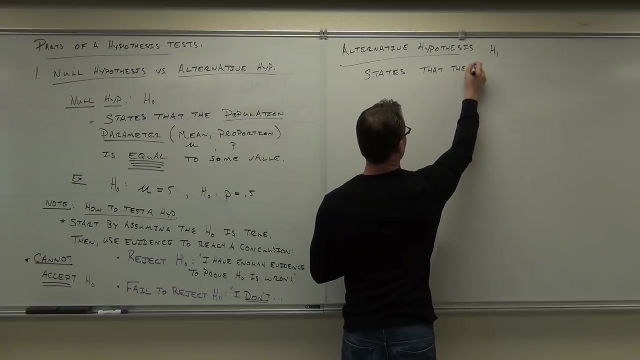 So I'll write that out for you What this does. this states that the parameter- whatever we're talking about- the mean and the proportion- has a value different than H sub zero. Remember: a parameter for us means one of these. 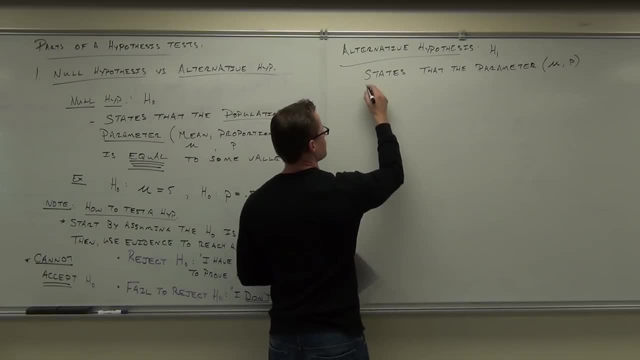 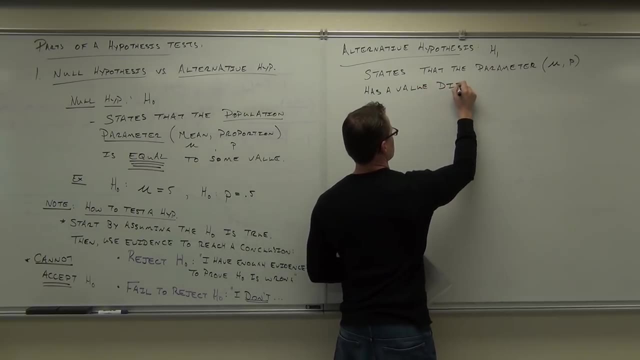 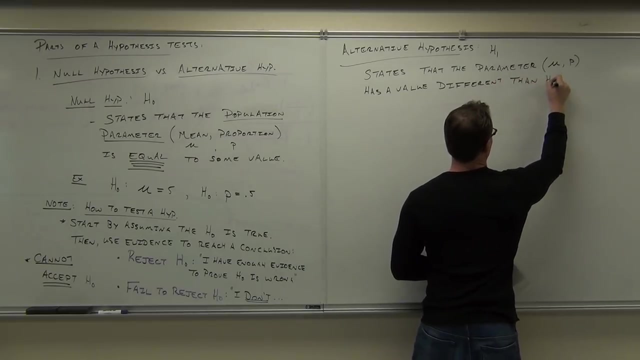 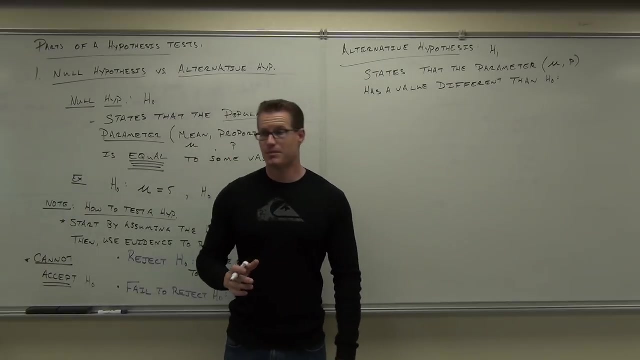 It states: the parameter has a value different than H sub zero has it? Here's how you can be different mathematically. In real life you can be different, lots of different ways, But in math you can be different one of three ways. 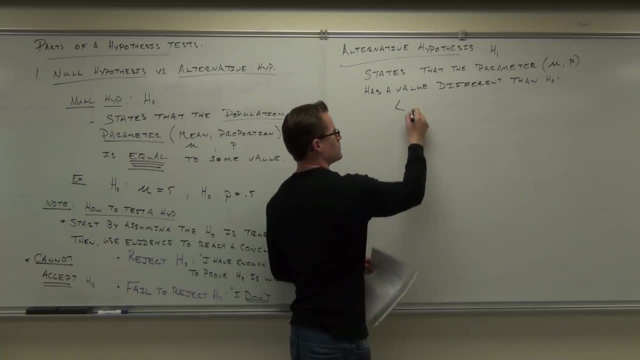 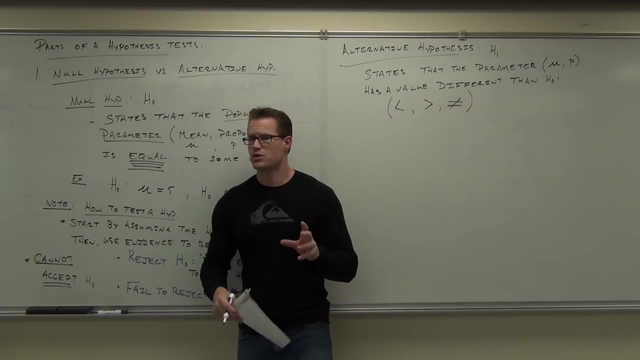 You can be less than a state of value, you can be greater than a state of value or you can be not equal to a state of value. These are gonna be given to you in the problem. You just have to determine which one it's talking about. 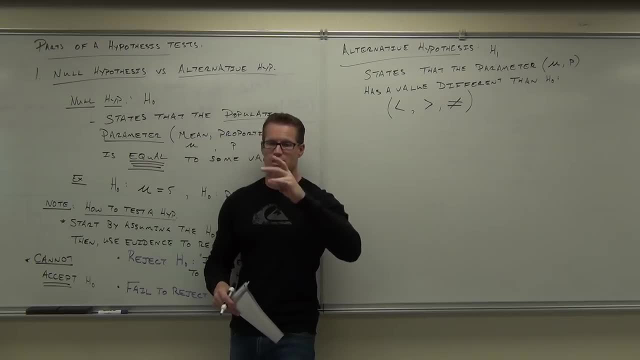 So there's three different ways to not be equal: Less than, greater than or simply not equal. Either you're less than or greater than that. So you can be less than or simply not equal. Either you're less than or greater than that. 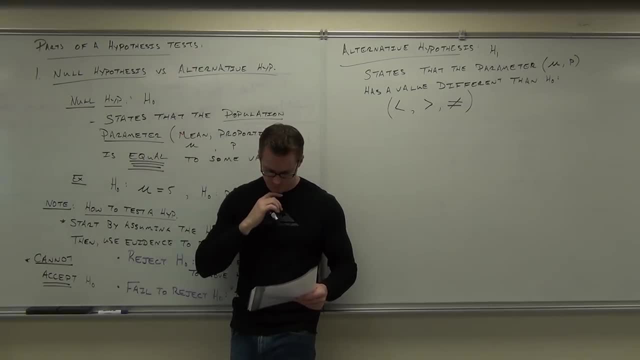 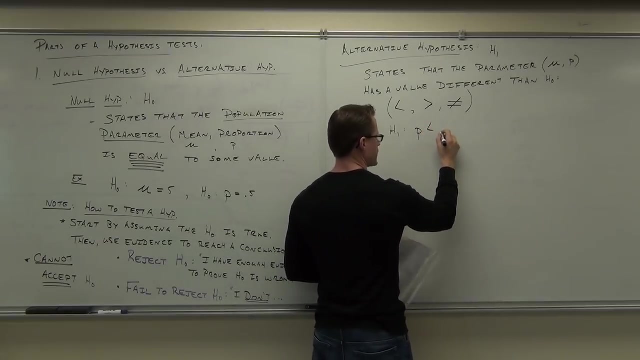 How many of you feel okay with this so far? Good, all right, Let me give you a for instance on how you're gonna see H sub one, just like I did over here H sub one, we might see proportions. You could have a proportion less than a state of value. 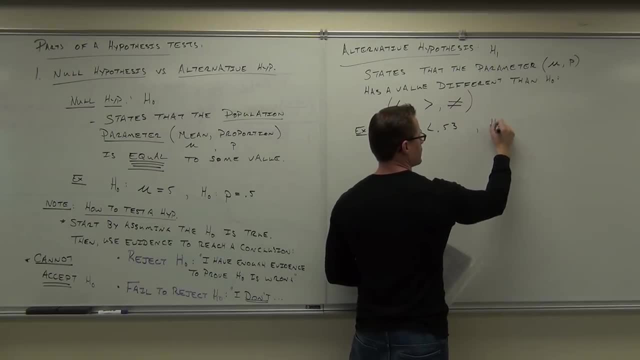 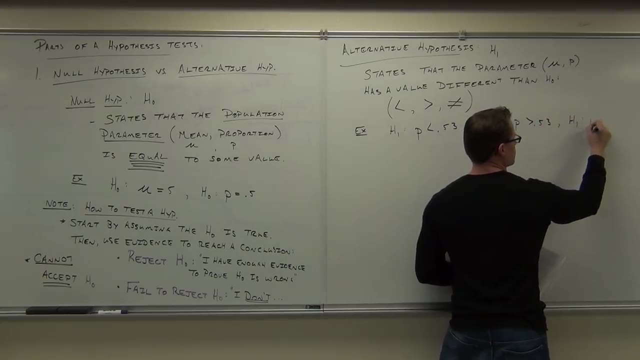 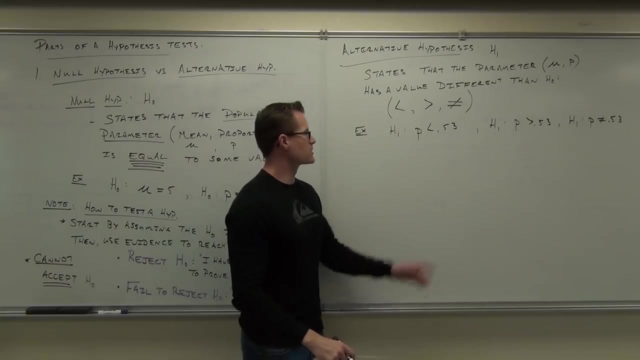 like 0.53.. Or you could have greater than, Or you could have not equal to. Those are really the only three ways that you're gonna see H sub one, the alternative hypothesis. You'll see a less than sometimes, or a greater than or not equal to. 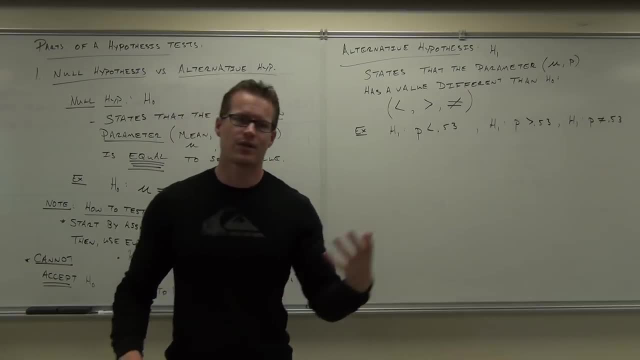 We'll get to the why those are the way they are in just a bit. how you find out whether it's less than or greater than or not equal to. We'll do that in a while. Right now I just want you to get comfortable with notation. 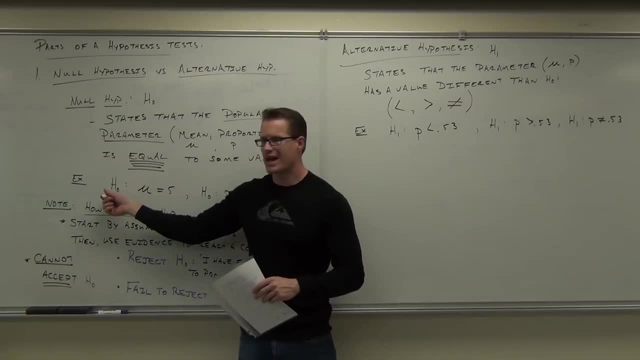 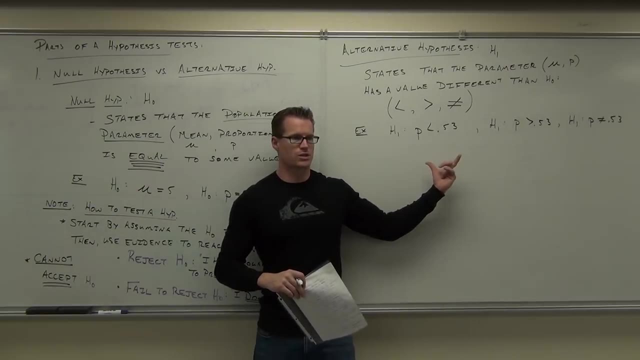 Are you comfortable with notation? So H sub zero is always gonna have a what? It's always gonna be equal, no matter what. That's a statement of equality. Is H sub one ever gonna have an equal sign? Not unless there's a cross through it, a line through it. 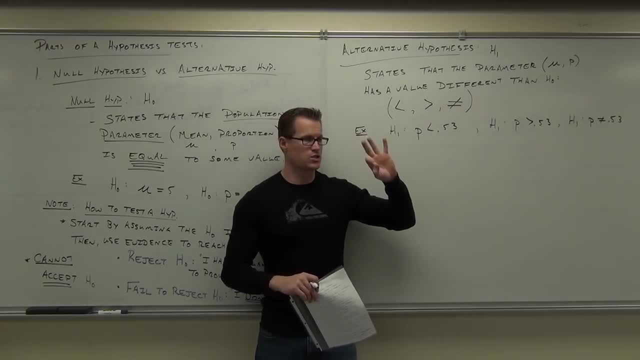 That means it's not equal. There's three options there. I'll teach you how to find out which option you have as you go through our problems, But you're gonna have one of three things If you're talking about not a proportion. 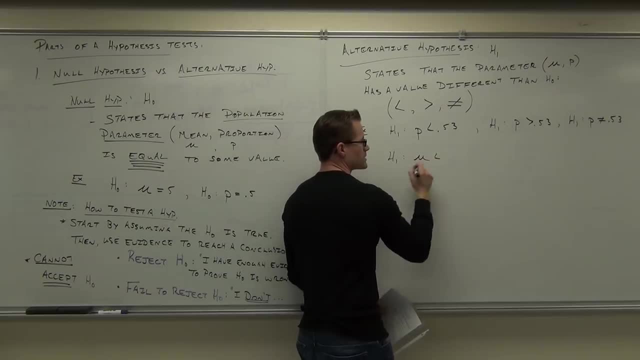 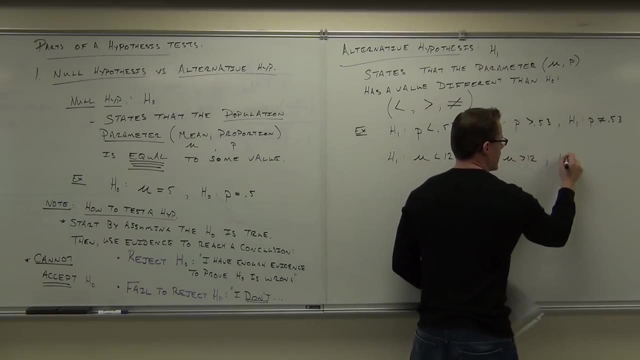 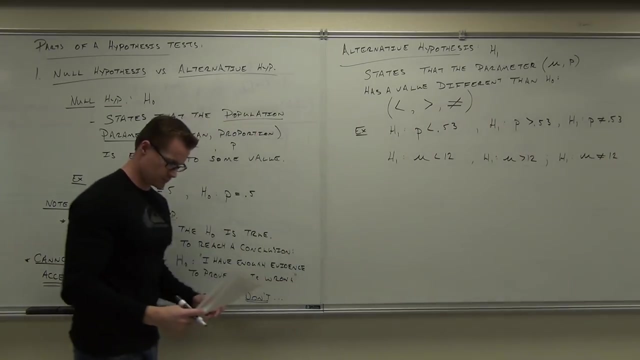 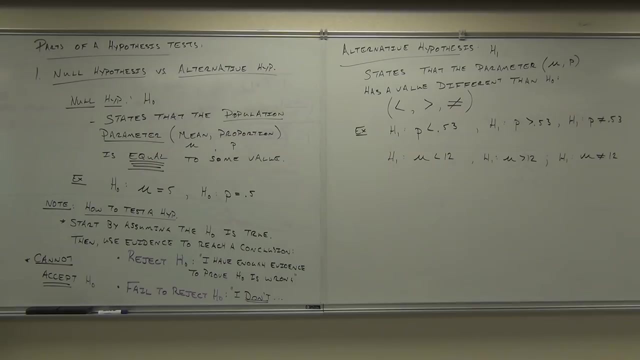 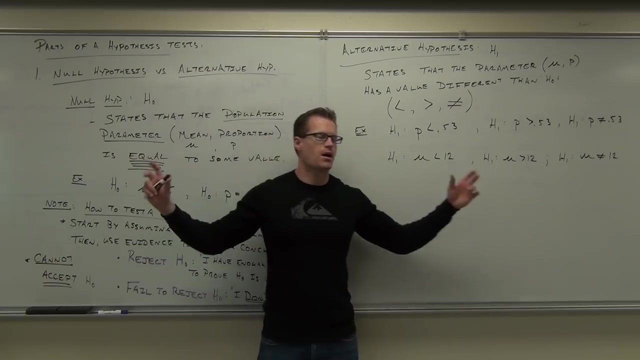 you're talking about a mean. you could have mu less than a given value, 12 let's say. Or you could have it greater than, Or you could have it not equal to. Now, here's the whole idea. The whole idea is that these hypotheses work together. 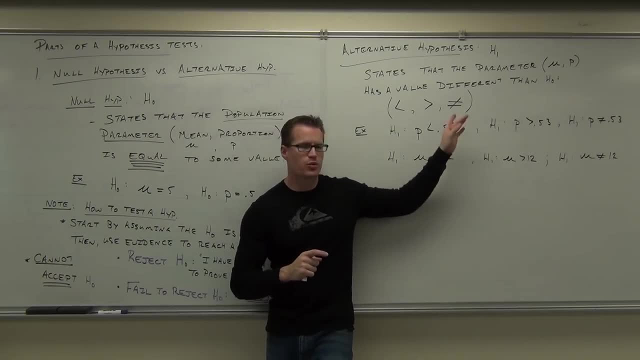 We work together. You see, we're not actually gonna be proving anything directly. What we're gonna be doing is proving things indirectly. It's an interesting way to look at it, But you're going to have, for each problem, a null hypothesis and an alternative hypothesis. 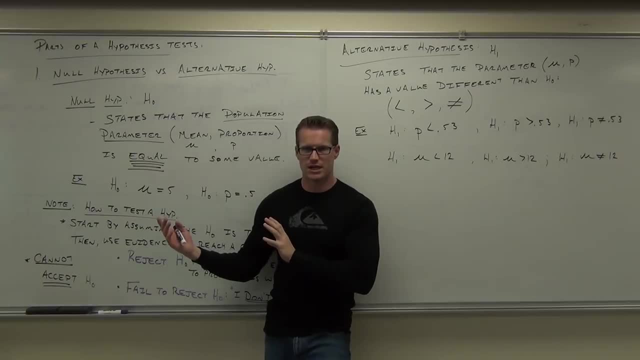 which is the opposite statement of the null. Do you get it? You have two statements: One has equality, One is opposite of that. So here's how this works: If you reject the null, that means that indirectly, you accept the alternative. 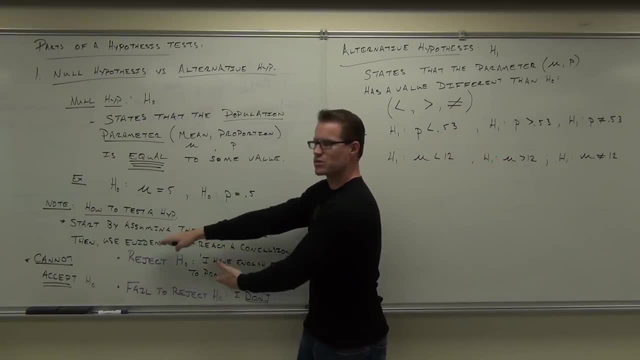 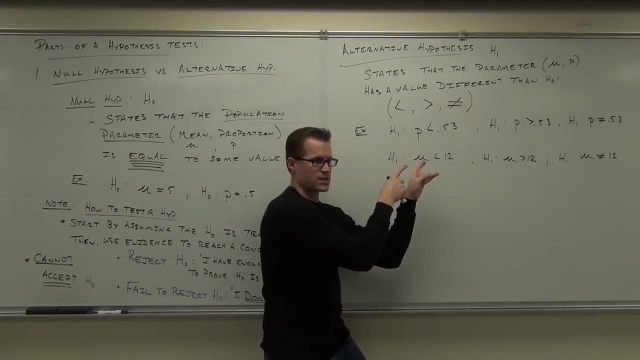 Do you get that? That's kind of cool. So can you accept this one? No, but you can prove it wrong, And if you prove this one wrong, it automatically proves that one right. Do you get that? So, by proving this statement wrong, 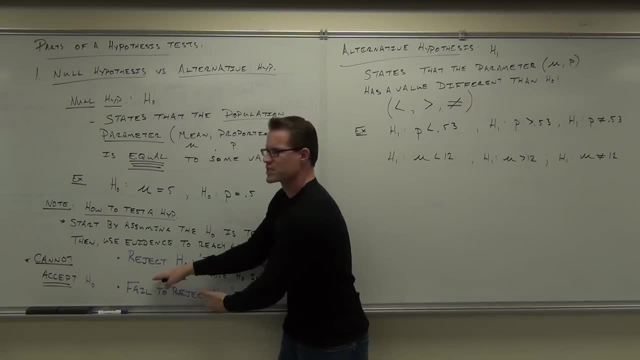 we prove that one right. What if we don't prove this statement wrong? Does it prove that one right? No, then it's inconclusive. You don't know. You didn't say anything about the problem. You didn't prove this right. 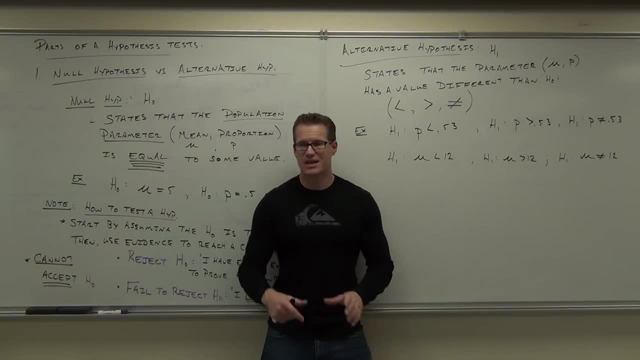 but you didn't prove that one right either. You did that one. So that's basically the way this works. These two things work in conjunction with each other: the null and the alternative. If you prove the null hypothesis wrong, that means that you accept the alternative. 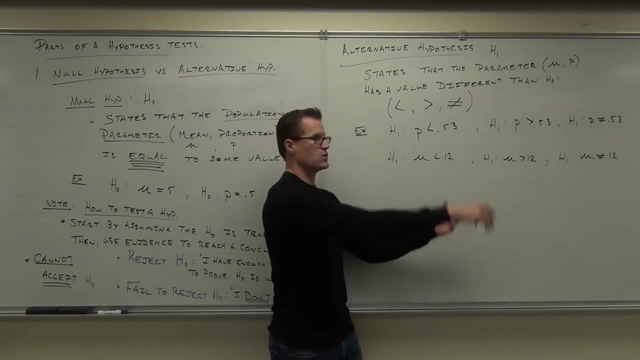 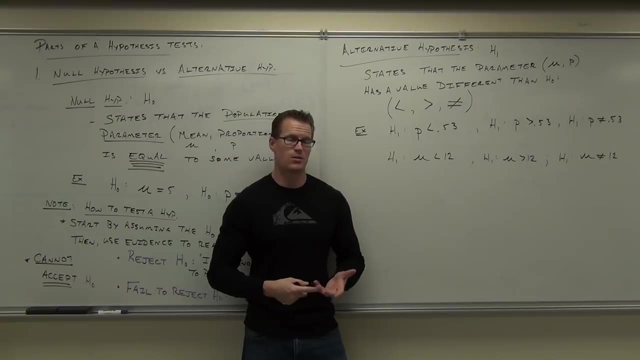 If you fail to prove the null hypothesis wrong, then that means you fail to accept the null hypothesis. They work together. You have to have both. You can't just prove a statement right, not with statistics. The evidence is only there to convict. 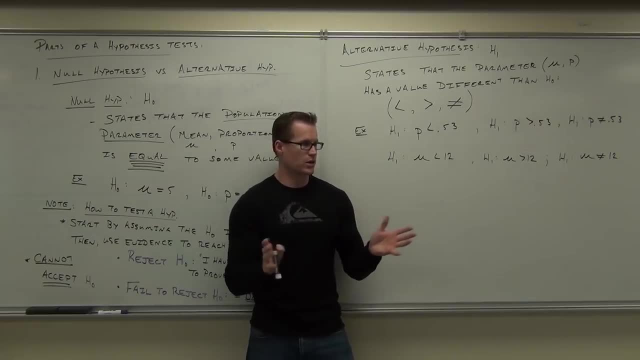 It's a very pessimistic way to look at it, But literally it's a court system, not a cult system. We're not in a cult here. We're not Pythagoreans or something. You know the Pythagorean story right. 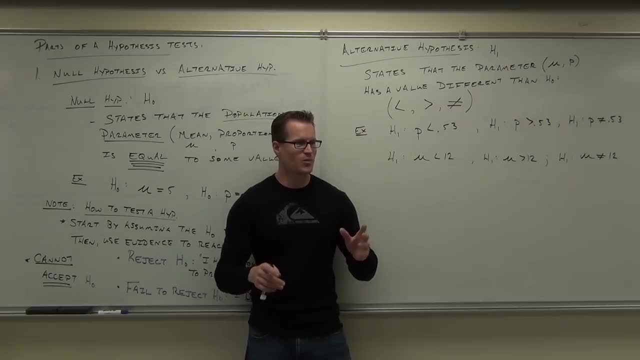 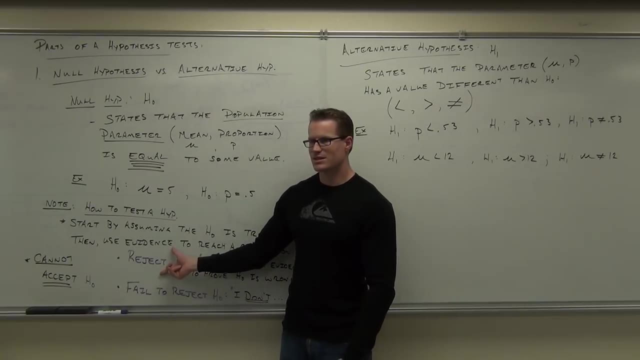 Killed them anyway. I'll tell you that story another time if you want, But we're in a court system, We're in a court system. If you prove this one wrong, it's guilty. then you were right to convict that person, right? 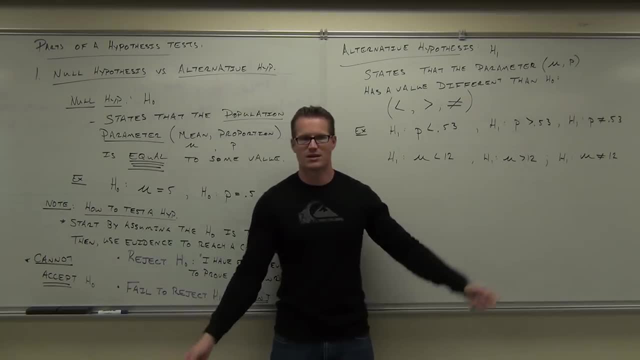 You got it. If you fail to prove that wrong, then you can't convict that person. He's free to go. Does that make sense to you? You prove this one wrong. he goes to jail Bingo. You don't prove that one wrong. 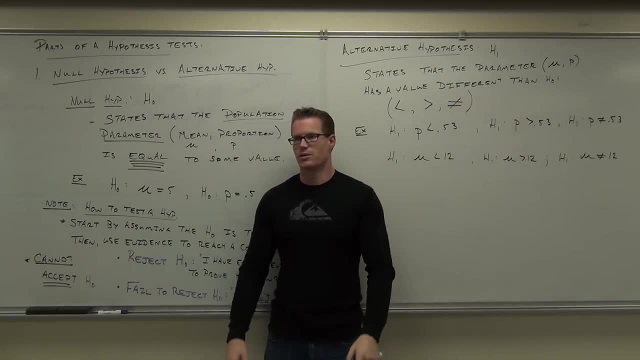 he doesn't go to jail, Nothing happens. He walks free. You don't know whether he's right or wrong. You don't know whether either one was right or wrong. So, ultimately, this is what it boils down to. If you want to prove a claim, 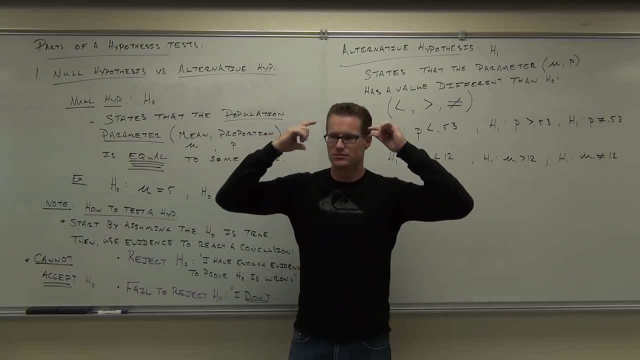 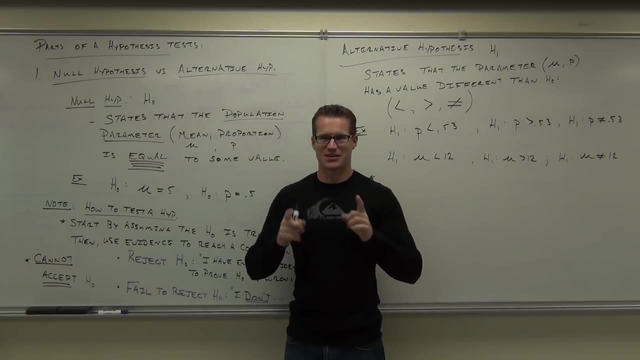 I hope you have your critical thinking hats on. No one has said, oh, one person has a hat on, The rest of you imagine hats. Two people have hats on. Technically, that's a hat. That's good, I like it. 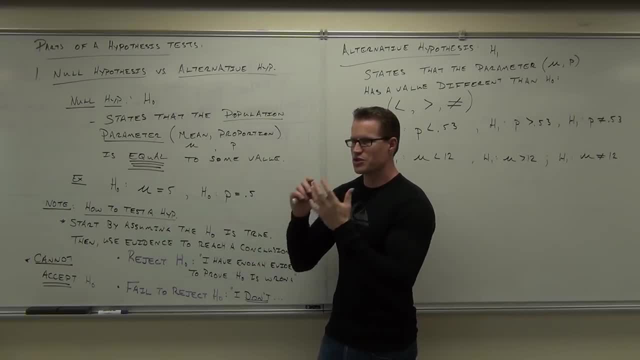 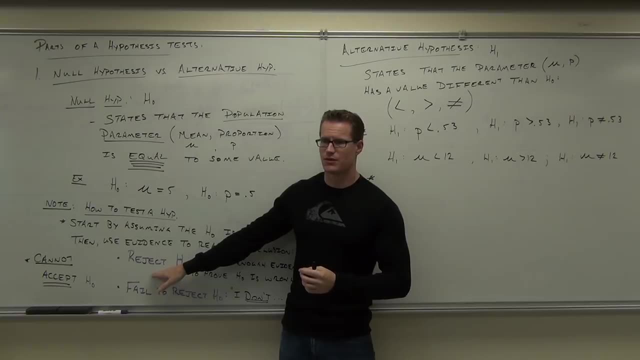 So if you want to prove a statement true, if you want to prove it right, can you state it as the null. If you want to prove it right, all you can do over here in this null is prove it wrong or fail to prove it wrong. 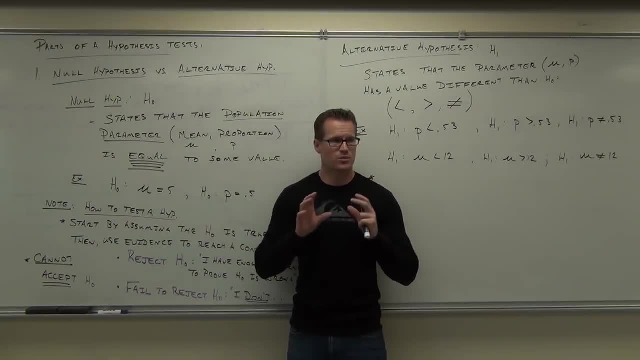 Can you accept it? That means you can't prove it right. So if you want to prove a statement right, should I use? should I state it as the null hypothesis? If I want to prove a statement right, true, I must state it as the alternative hypothesis. 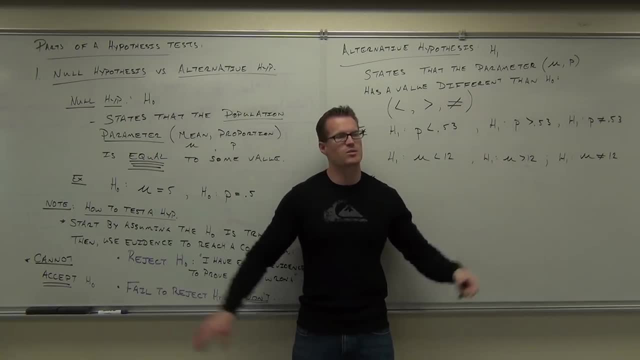 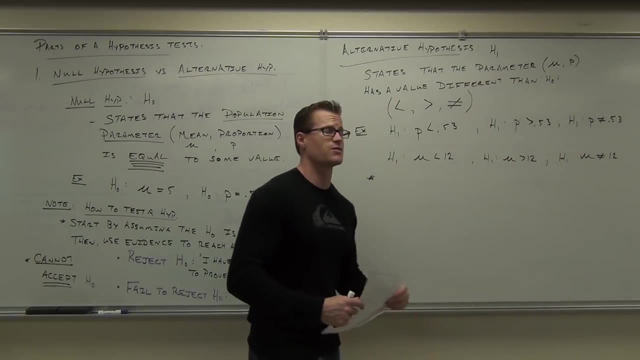 because that's the only one you can accept. And the only way you can accept it is by proving that one wrong. So that's what it boils down to. I know this is very vague because we're in the introduction. Trust me, we'll go through lots of specific examples later. 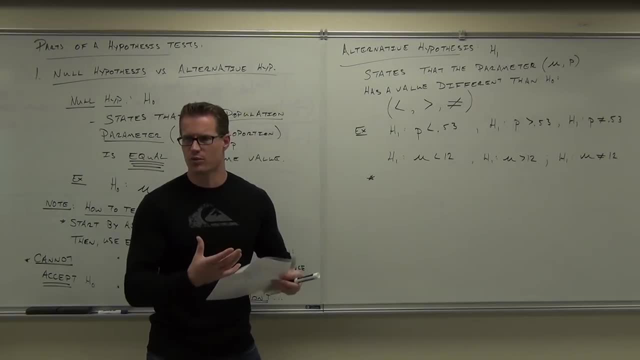 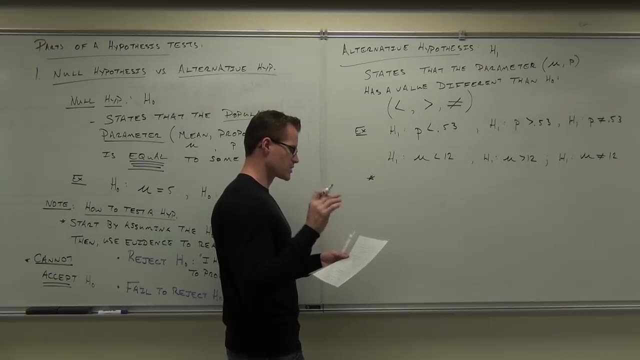 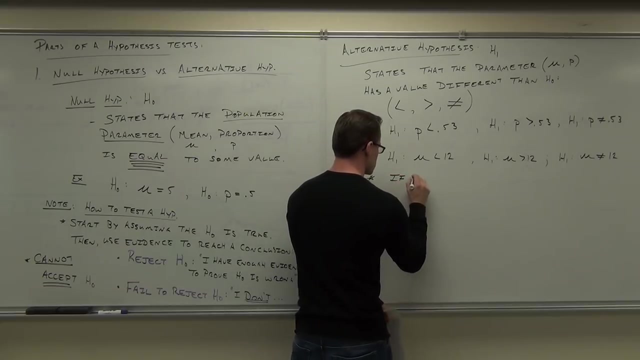 I just need to get you kind of comfortable with the scenario before we get to it, Are you okay with that? So here's what it boils down to for you. If you want to support a statement, you must state it as H1, not H0. 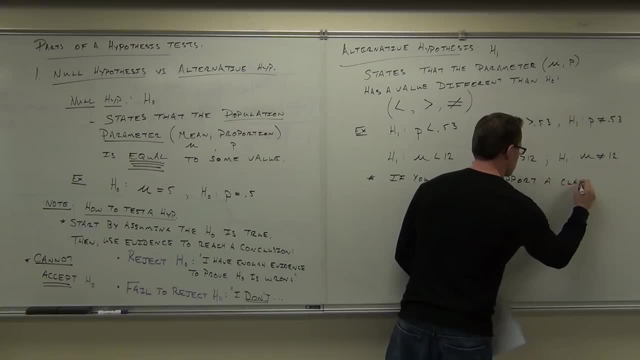 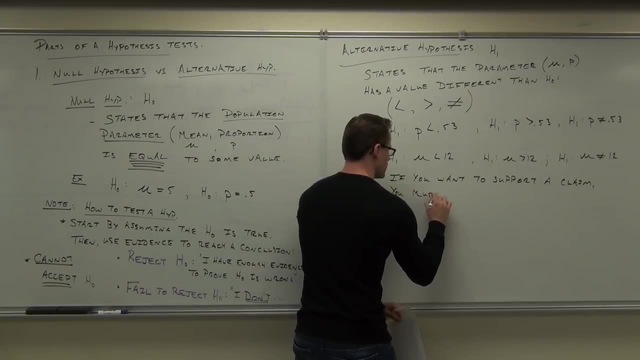 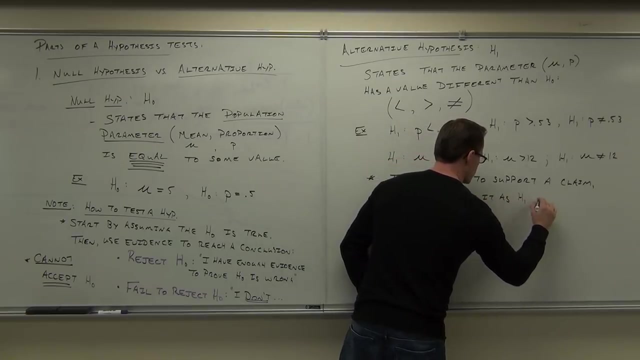 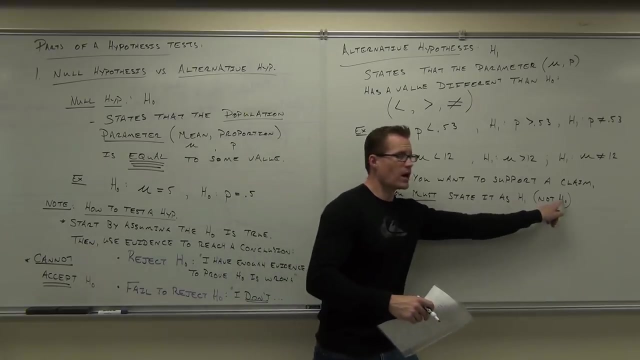 If you want to support a claim, that means prove it right. basically, If you want to support a claim, you must state it as H sub 1.. Why not H sub 0? Why not? Well, you can't prove that right. 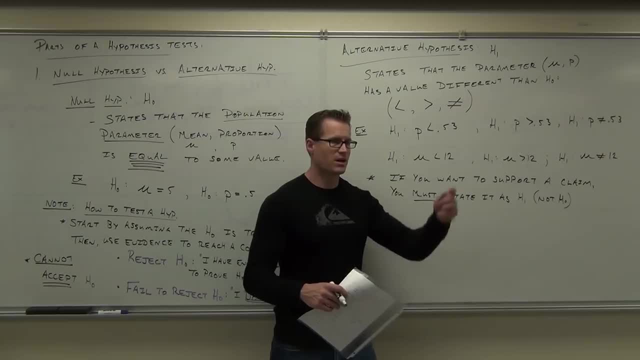 You can't prove H sub 0 right. All you can do is prove it wrong. You don't want to make a claim. you're trying to prove right and then prove it wrong, do you? Let's look at your options, okay. 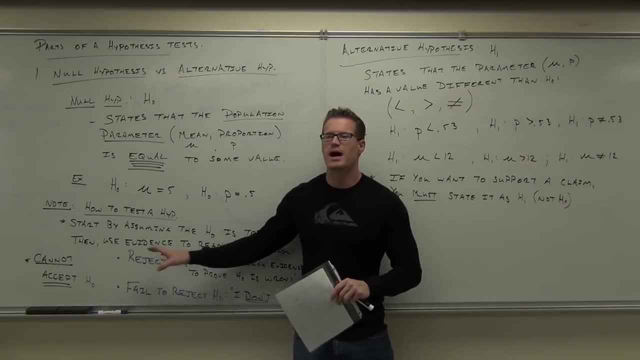 Let's say that you stated your claim as H sub 0. I'll teach you how to state a claim in just a bit. Let's say you stated it as H sub 0. All you could do with that is prove your claim wrong. 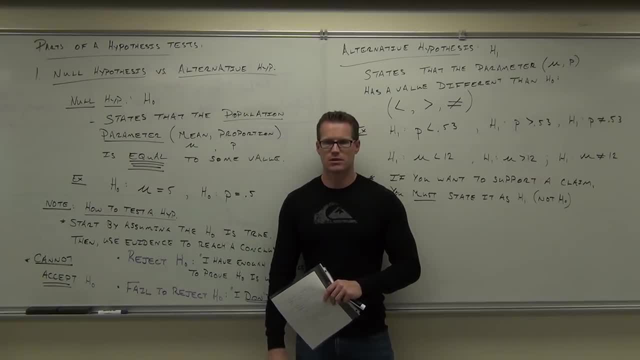 or not prove your claim at all. Are either of those a good thing? You're trying to prove it right. So, if you're trying to prove it correct, if you're trying to prove a statement true, you stated it as this Claim the opposite and then prove that wrong, 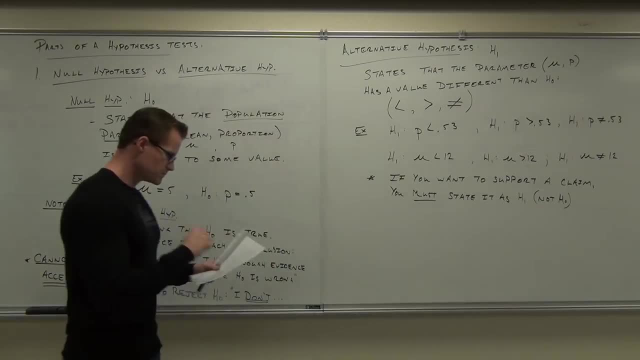 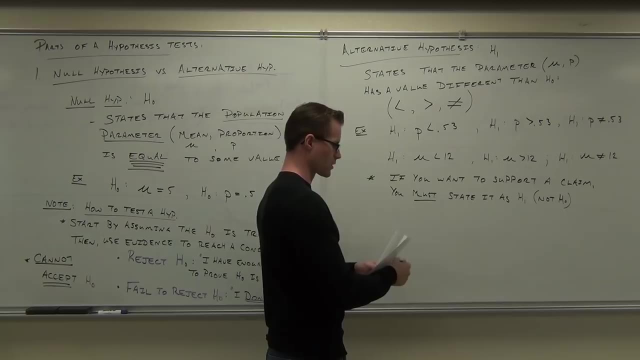 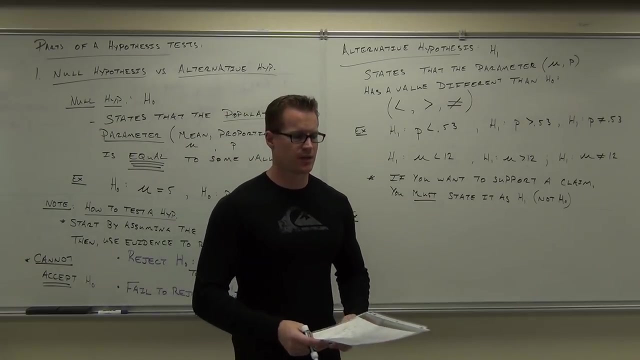 That proves your claim. That's what you're doing. Let me give you an example of how this is going to work. Remember that fertility drug I talked about that said it gives you a. the drug said it gives you an 80% chance of having a girl. 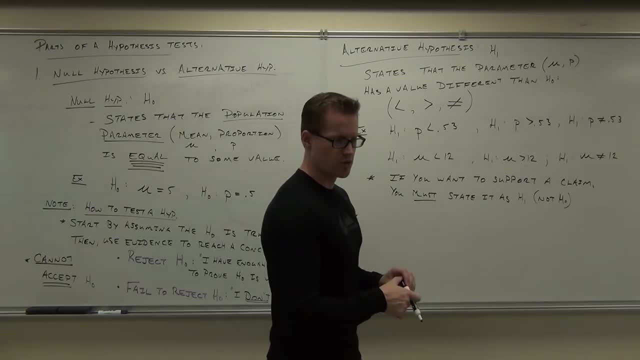 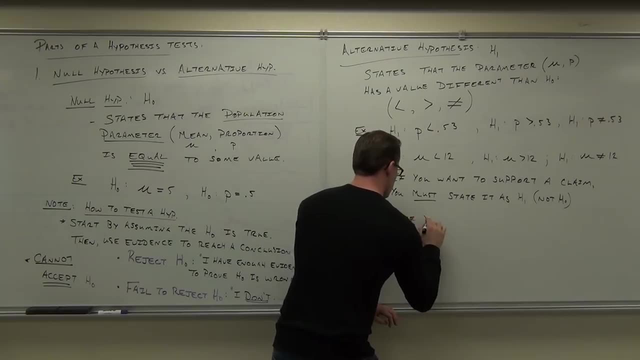 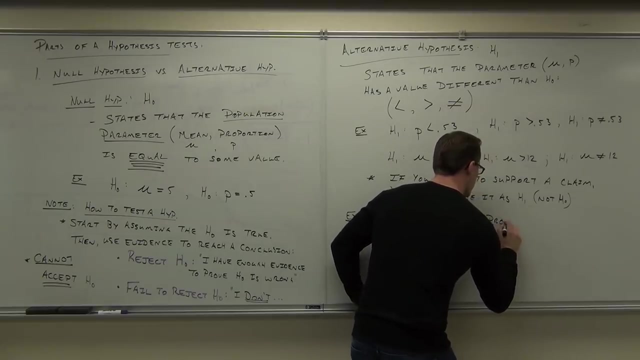 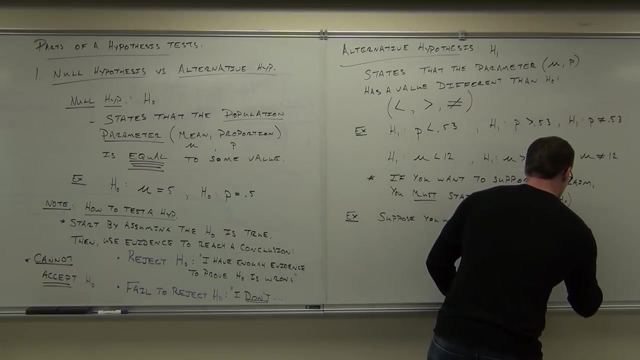 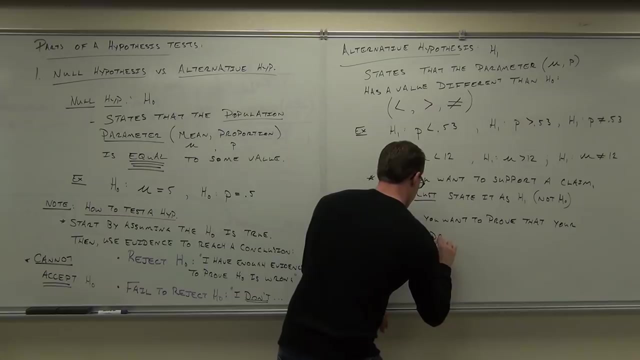 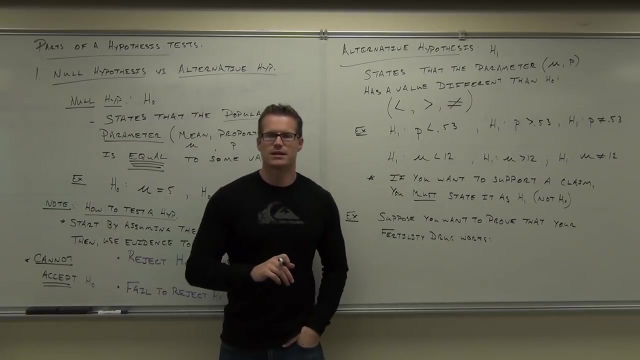 Remember that one. Let's say you're trying to prove that right. Suppose you're trying to prove that your drug works, that your fertility drug works. Suppose you want to prove that your fertility drug works. Basically, here's what you would do. 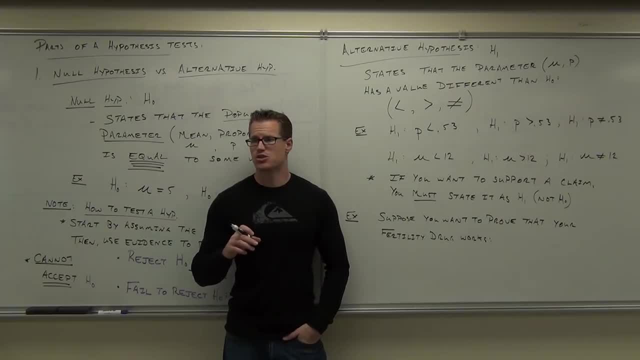 You're not going to make some claim like it gives you more than an 80% chance of having a girl. All you want to show is that it's significantly different than 50%. You want to show that more than 50% of people. 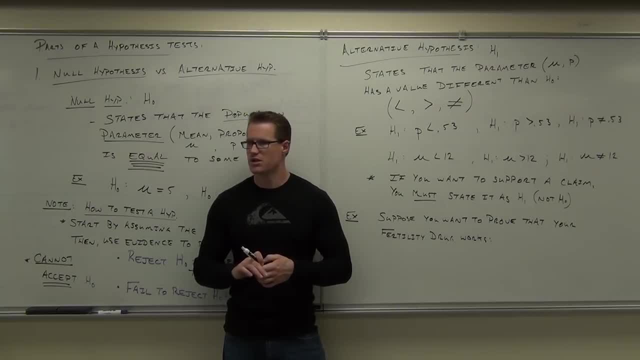 are going to have a girl with this drug. Isn't that what you want to show? Because 50-50 would be normal. You all have a chance. Well, actually you guys. you're out of luck. You can't have children. in case you didn't know that, 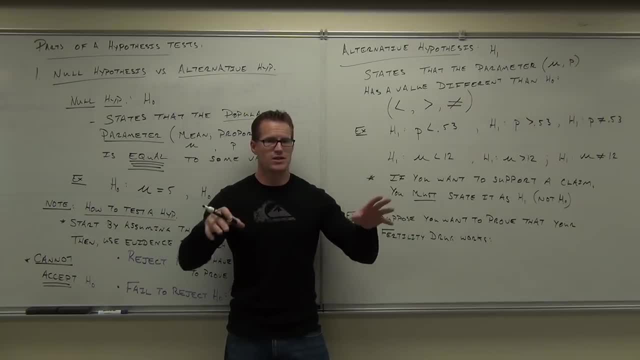 But only women can actually have it. So you guys- you know this part, But you girls would have a 50% shot at having a girl. Does that make sense? Or a 50% shot at having a boy if you didn't take this drug at all. 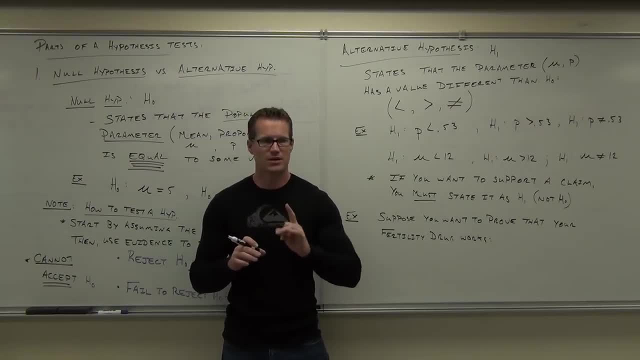 So what you're trying to show is that people who take this drug- more than 50% of them- are going to have girls. Do you get the idea? That's what you're trying to show? Should I state that as my H sub 0?? 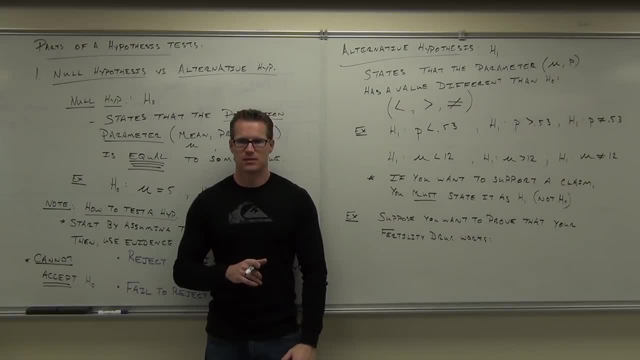 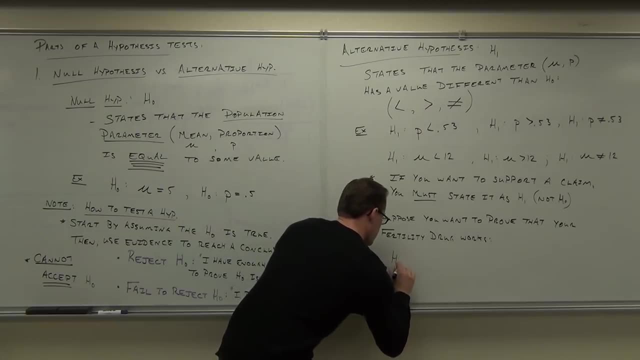 Or my H sub 1, if I want to prove it right: H sub 1.. H sub 1.. So here's what you do. You say, if I assume the drug doesn't work, the proportion of people who have girls would be 50%. 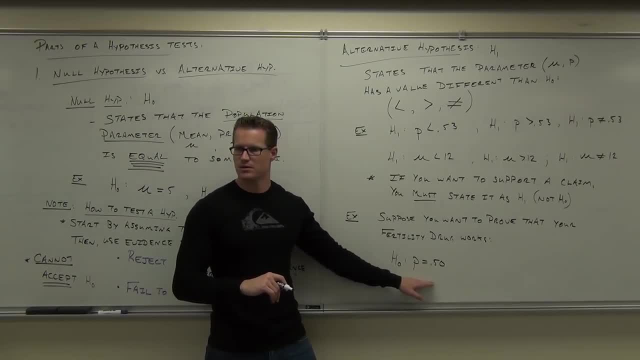 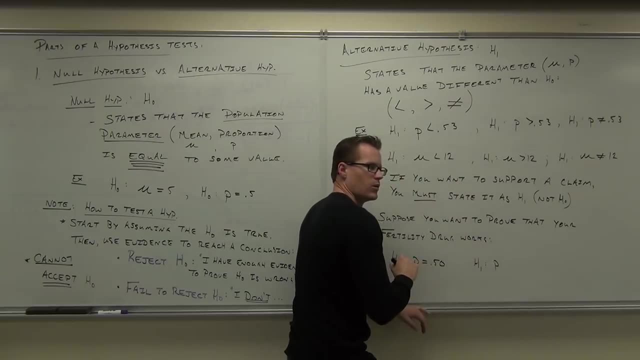 Notice this would be assuming the drug doesn't work. You with me on that, Because 50-50, it doesn't work. And then the alternative: you would state: oh well, I want to show the proportion of people who do have girls. 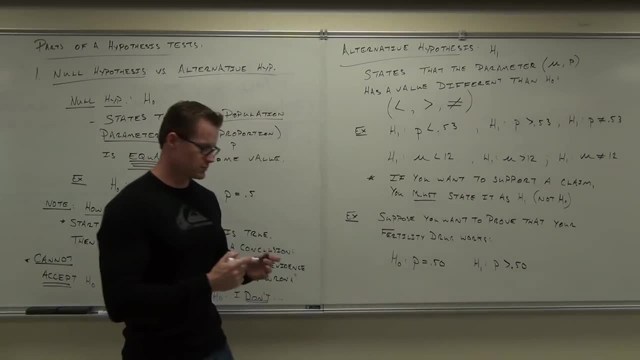 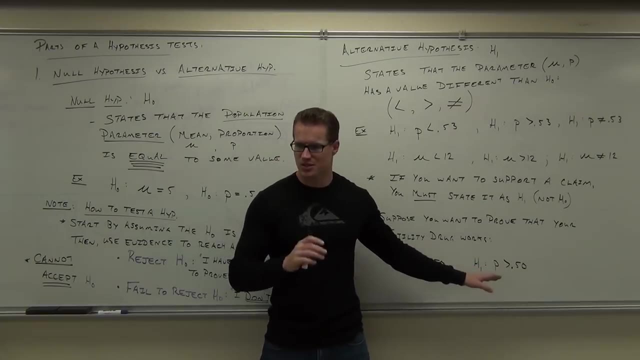 is more than 50%. That would be the alternative. I'll show you how to do this from a statement specifically later on. Right now, let's just assume that we did this correctly and this is what you got out of it. I'll show you how to do this later on. 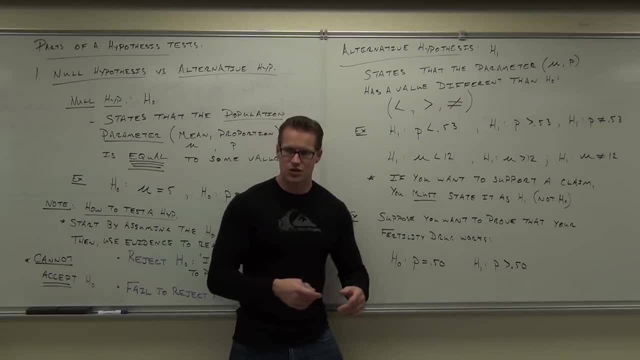 But here's how this would work. What you're going to be doing is you're going to be testing this claim. You with me on this. This is the claim. That's the alternative. This is the null hypothesis. This is the alternative hypothesis. 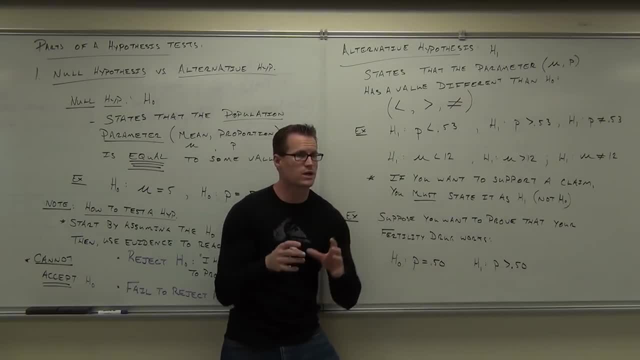 You test the null hypothesis, You work it down. There's two options here. You can either reject it or fail to reject it. So here's how this works. This is pretty cool If you work it out and you reject the null hypothesis. 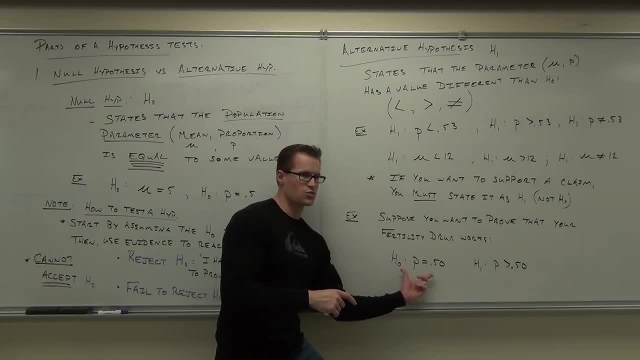 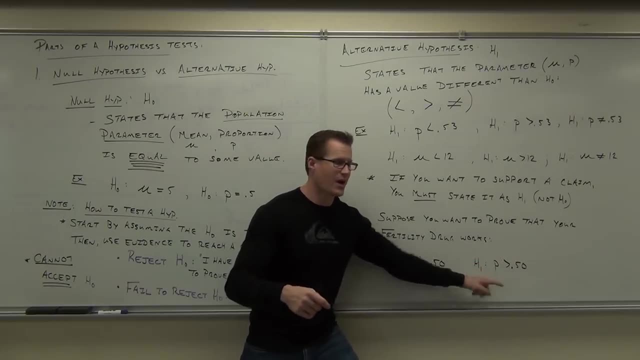 if you say, oh, I got evidence, this is wrong. you know what it does: It automatically proves that one right. And then you prove your original claim, which you wanted to show You go: oh hey, if this is wrong, this is true and my drug works. 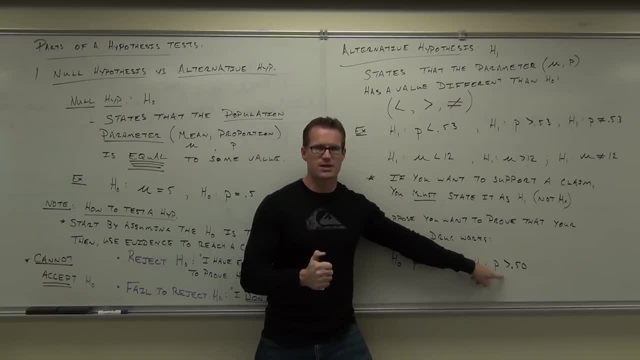 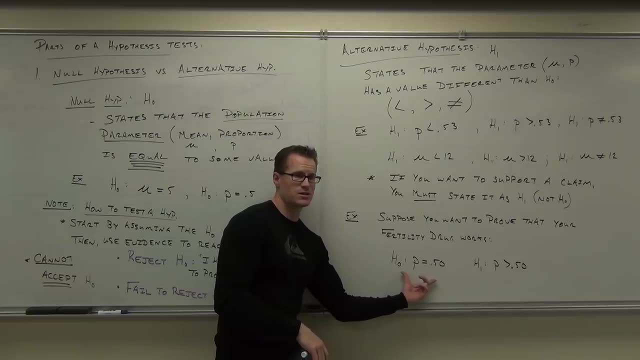 More than 50% of the people will have females If they take a stroke. Do you follow the idea? Now, let's say you fail to reject it, You go well, I don't have enough evidence to show that this is wrong. 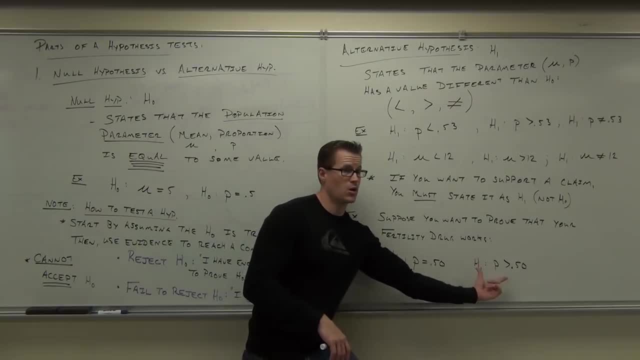 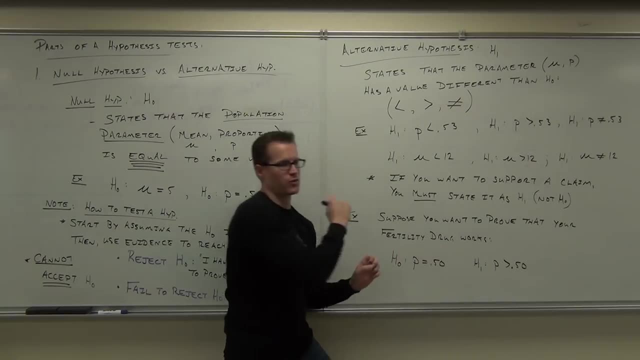 Is this one right? No, Is this one right? No, It's inconclusive. You don't have enough evidence to say anything. You can't ever prove this one right. You can only prove it wrong or fail to prove it wrong. 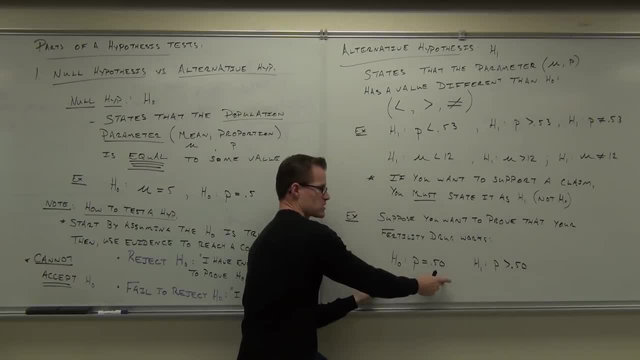 So your options are: reject this, accept that, Fail to reject it, Fail to reject this- Nothing. And then you're done. You're stuck, You can't say anything at all. You're stuck in either situation. How many of you understand the idea of hypothesis testing? 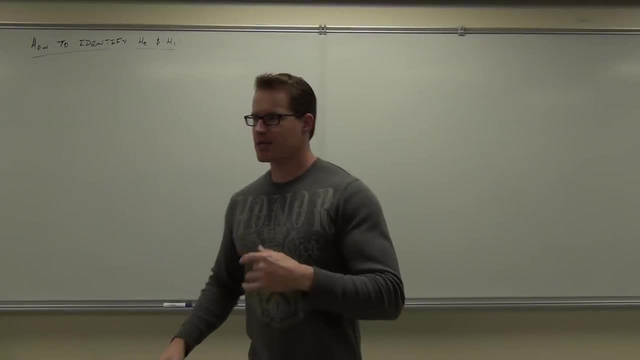 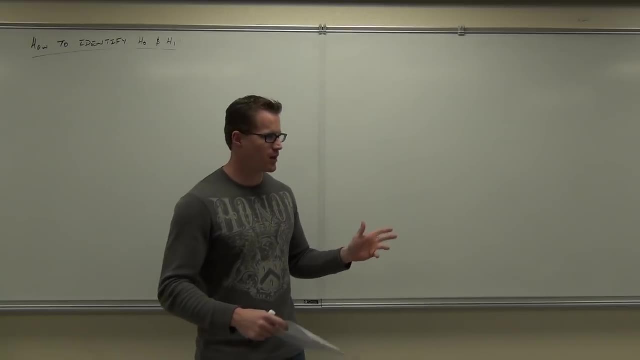 Good, All right. So, continuing on this hypothesis testing, I haven't taught you how to identify your H sub 0 and your H sub 1, which is your null and your alternative hypotheses. We've talked about what those things are. We've talked about how we can state claims. 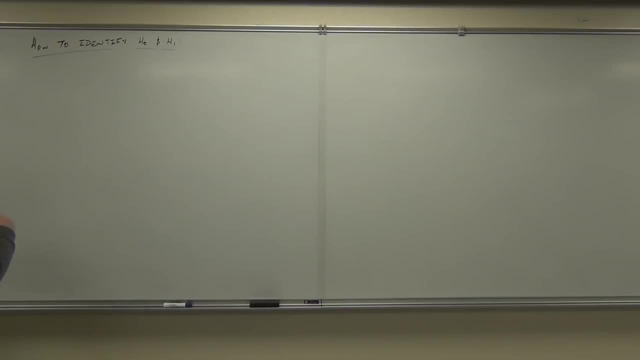 But we haven't really dealt with the claim yet. We're going to do that right now. So here's how to identify your claim as either H sub 0 or H sub 1, your null or your alternative. The first thing you're going to do, you're going to state your original claim, symbolically. 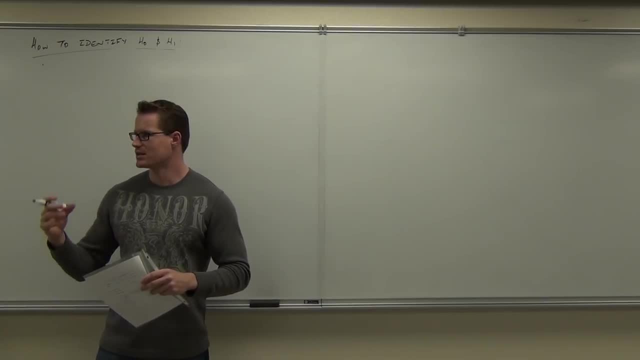 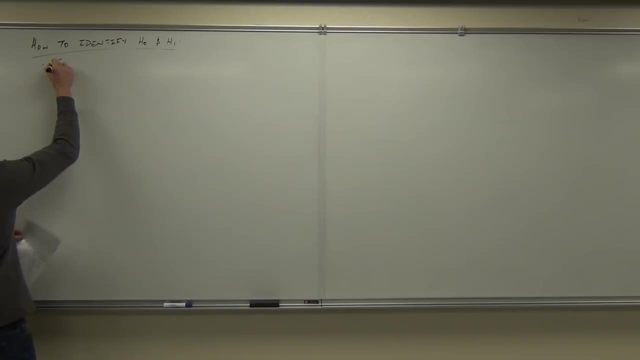 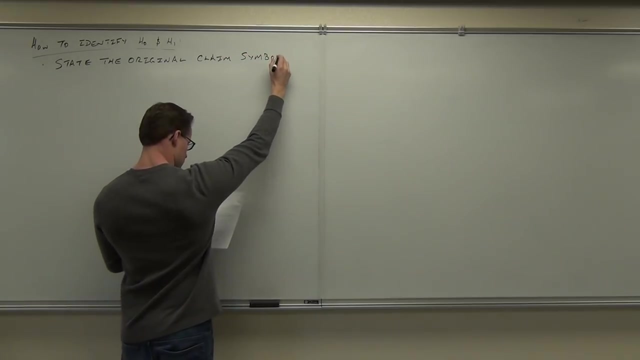 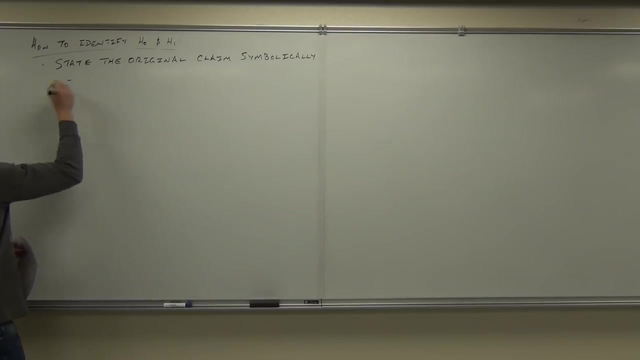 That means that you're going to take that word sentence and make it into something like equal signs or inequalities, something like that. We're going to state our original claim symbolically. Also very important thing, you're going to state the opposite of your claim as well. 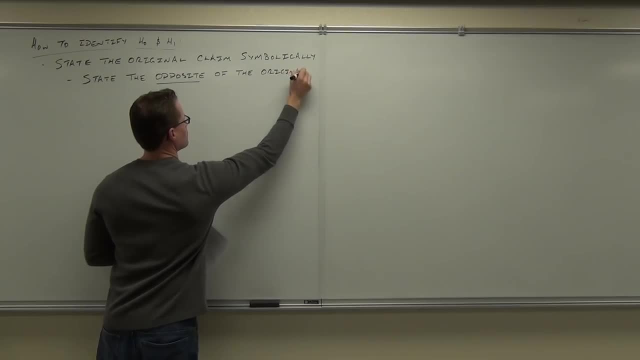 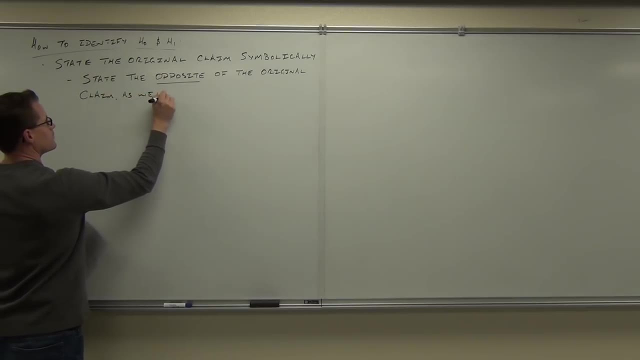 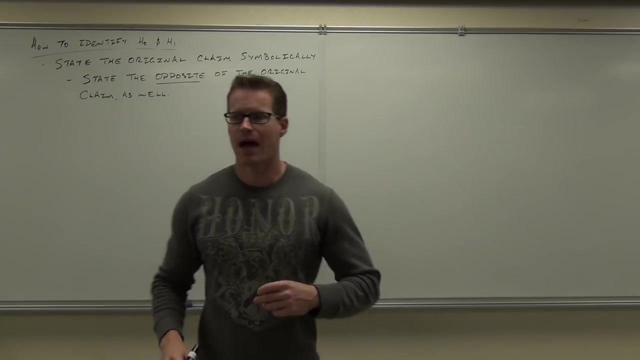 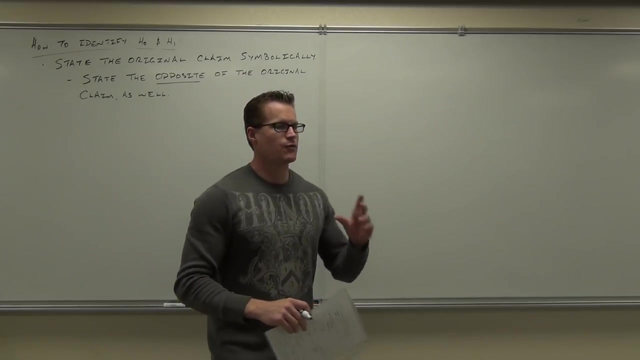 You're going to state your original claim symbolically. You see, here's the deal. Depending on how the original claim is worded, it could be either H sub 0 or H sub 1.. If you are trying to prove your own claim. if you're trying to prove your own claim, 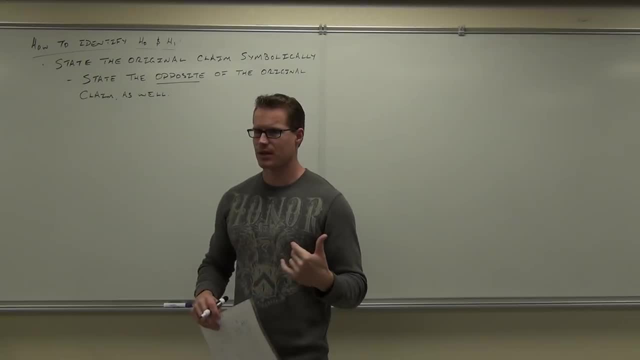 you have to state your claim symbolically. You have to state it as H sub 1.. We talked about that last time. You remember talking about that last time for the people who were here. If you want to prove your claim, you have to state it as H sub 1.. 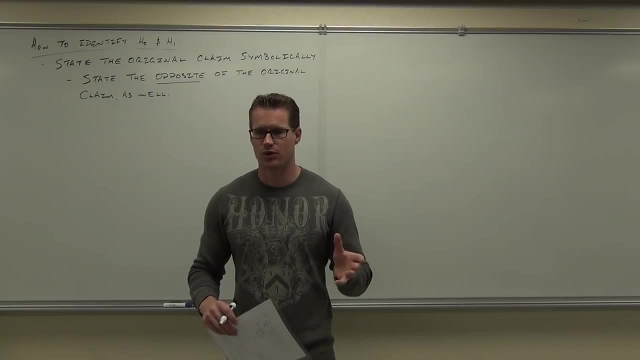 If the claim is given to you, you can't change that. It's set in stone. All your claims are going to be set in stone. You're not testing your own claims in this class. That's further on, when you actually do your projects and statistics or you use statistics. 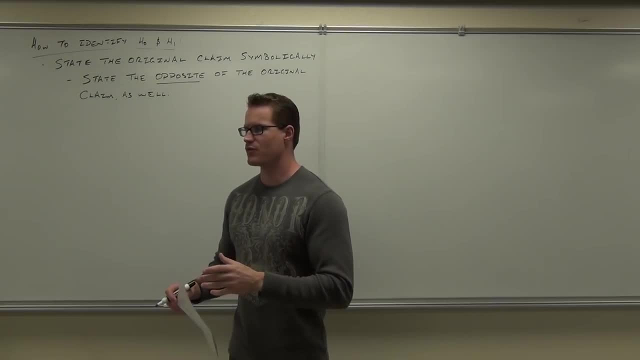 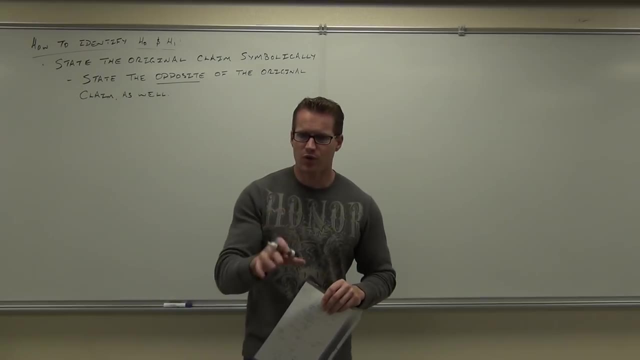 in your actual classes to do something like your master's degree or if they have a bachelor's project or something for you. you'd have to use statistics about that if you do any sort of survey. But anyway, if you want to prove your own claim, it's got to be H sub 1.. 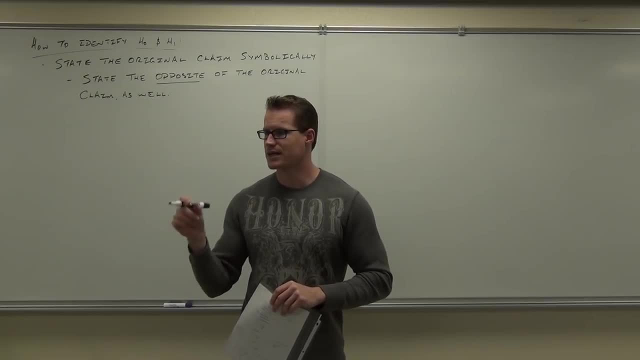 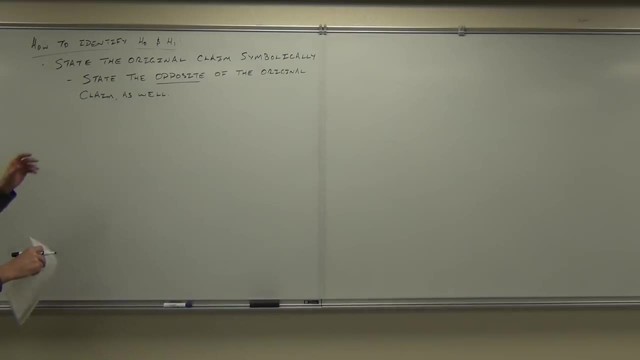 These claims are going to be given to you. They can either be worded as H sub 0 claims or H sub 1 claims. We're going to have to identify how to figure that stuff out. In order to do that, you state your original claim symbolically and you state the opposite. 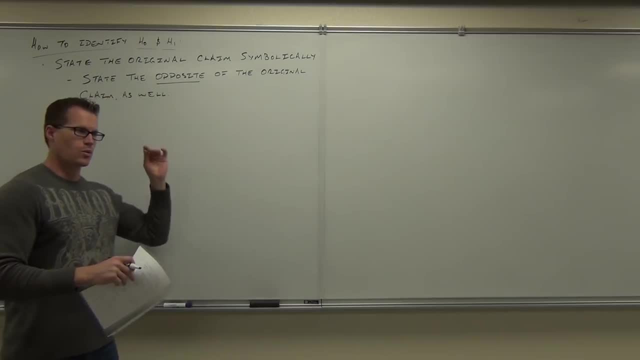 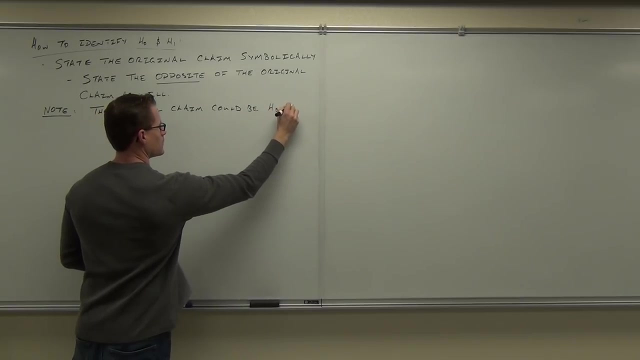 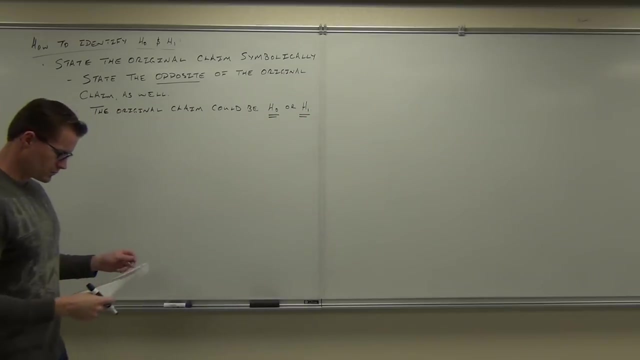 of the claim. symbolically. Your original claim could be either H sub 0 or H sub 1.. Make a note on that. The original claim could be H sub 0 or H sub 1.. How do you tell? It depends on where the equality is. 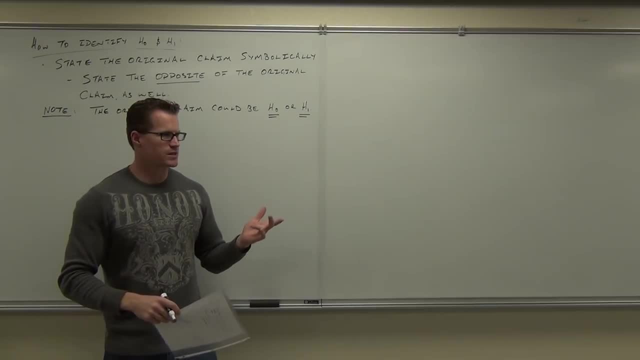 We learned last time that H sub 0, which one has the equality, The equal sign, H sub 0 or H sub 1.. H sub 0.. H sub 0 always has the equality, So it depends on where the equality is which one is going to be: H sub 0. 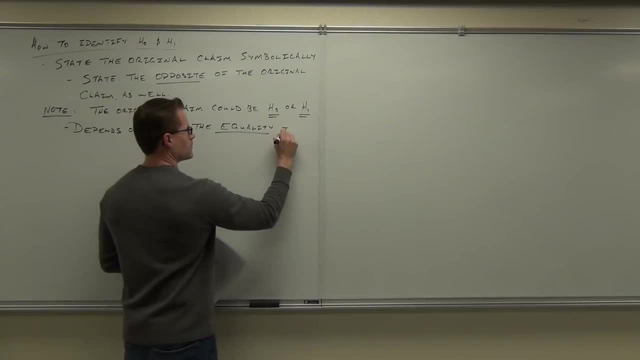 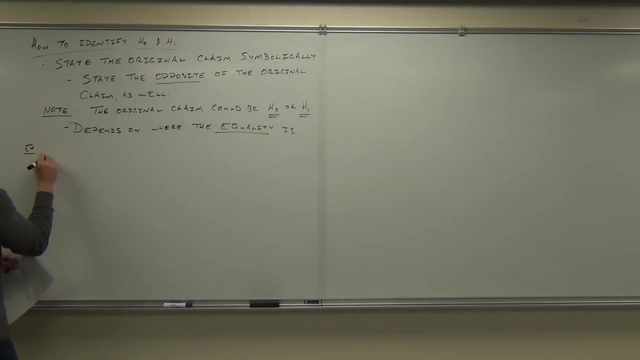 As far as referring to it, H sub 0 is equal to 2.. So H sub 0, therefore should not be completely. Come back In a letter. try each of the names. As far as referring to it, H sub 0 and H sub 1 have to be equal keys. 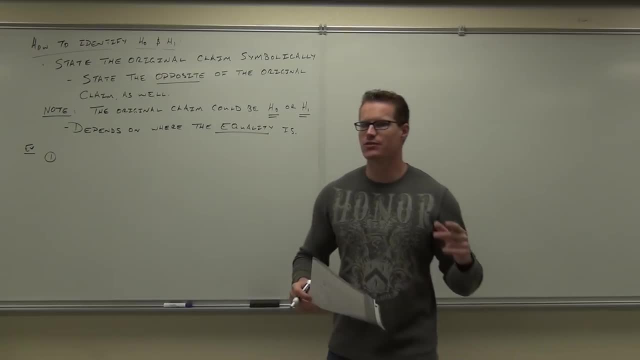 You want everything to be equal in the dalamos, But be sure that you have every word you know with H, No matter what number you put in. All you have is what you wrote in the Europail Dialog wheels. Take an example. I'm sorry. 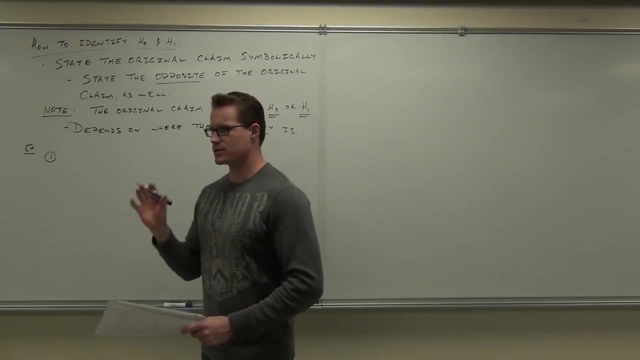 model useful. talking about proportions or means- That's the two scenarios you deal with at this point in the class- is proportions and means. Later on, when we get to the last day of school, last two days of school, we'll talk about variance. 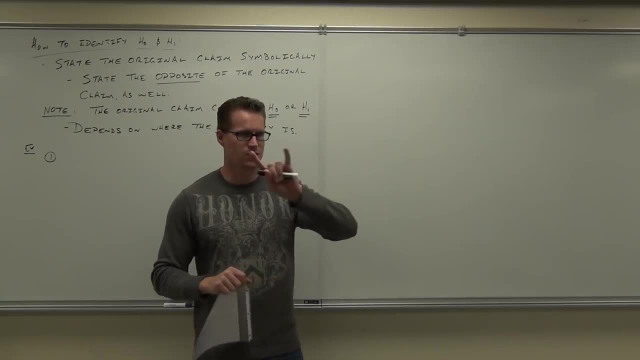 or standard deviation. we'll talk about that, For right now you have only two options: It's either a proportion or it's a mean. you got it, So you identify that first. Secondly, we'll translate this claim into symbolic notation. 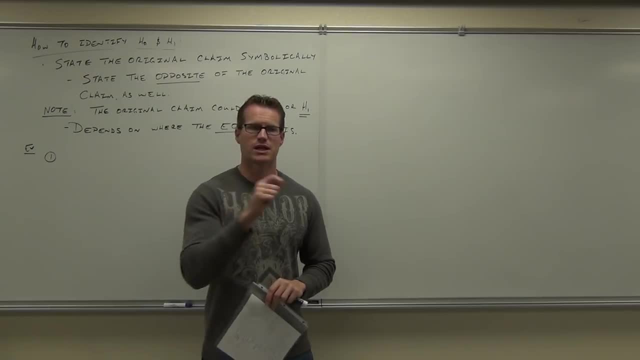 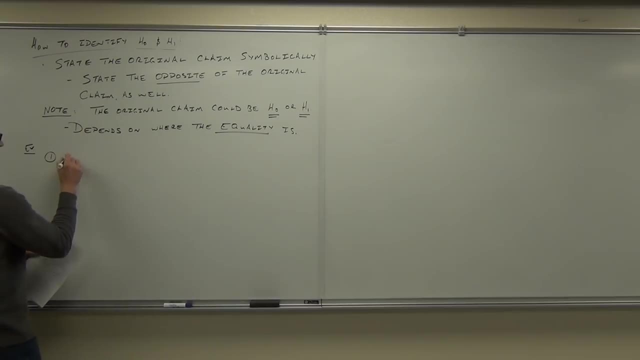 so, like with equal signs, or greater than or less than, and then we'll determine which one's H sub zero and which one's H sub one, after we write both the claim and the opposite. So here's our first statement. Remember? I'm giving this to you step by step. 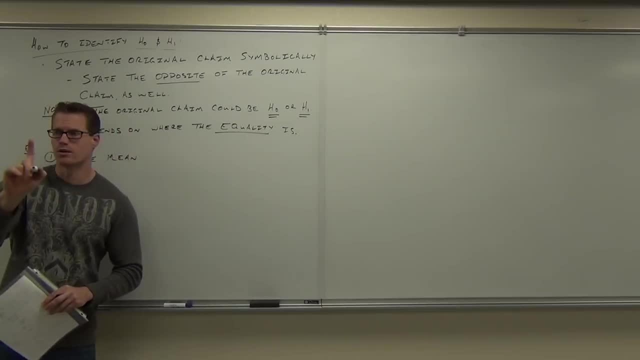 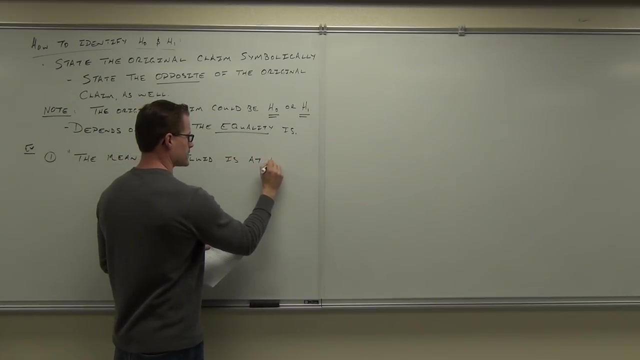 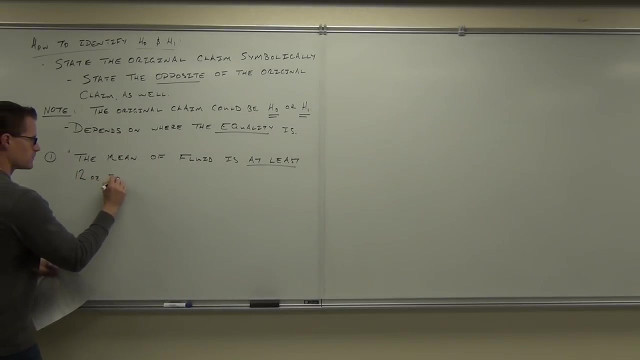 This is the first step in doing hypothesis testing. This is number one, what you do right off the bat. So here's the statement: The mean of fluid is at least 12 ounces in a can If you're a soda manufacturer. 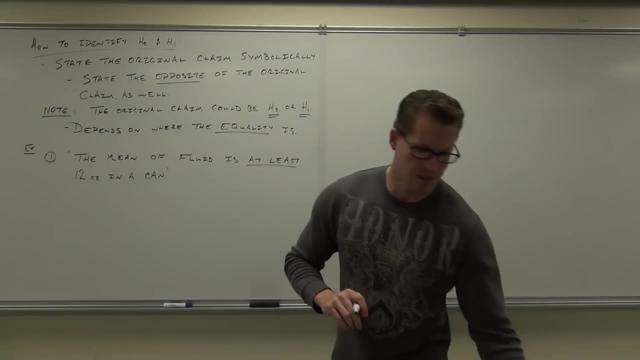 you might want to actually test that claim right, Because you don't want to be giving people less than 12 ounces in their soda can because they're going to be mad. You ever open a can and go. well, it's half gone already. 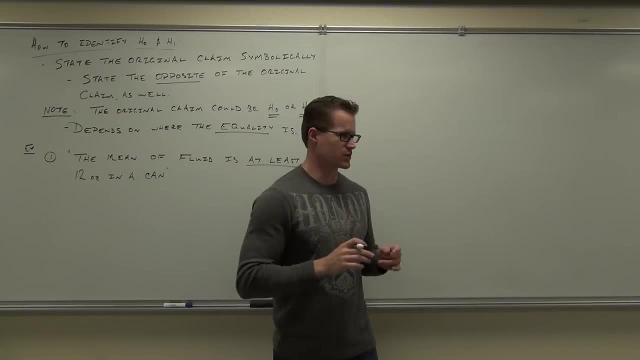 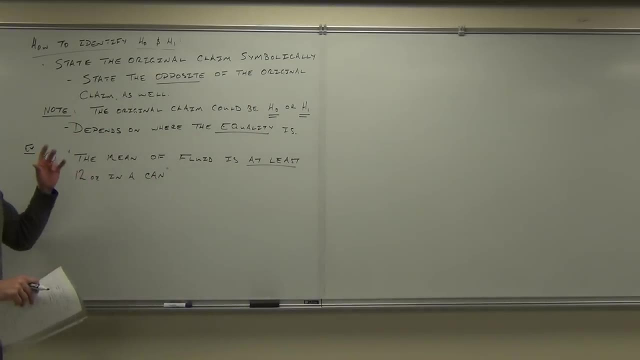 Oh, it sucked right. So they want to make sure that they're giving people at least 12 ounces to fill that. can You with me on that? That's their claim. Firstly, you've got to understand whether we're dealing with a proportion or a mean. 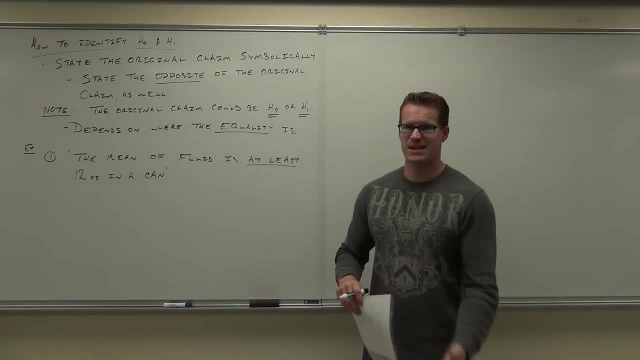 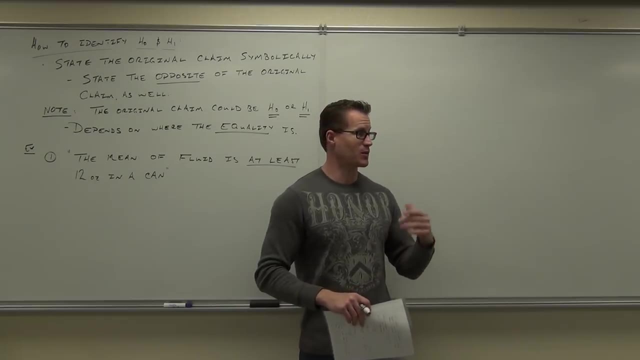 What are we dealing with here? Does it say anything about most, or give a proportion or percentage or anything? Does it say mean? Hey, there's a clue, right, We're dealing with a mean. So it says the mean of fluid, or the average level of fluid is at least. 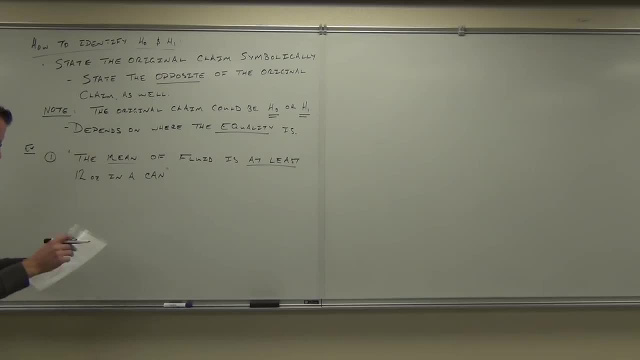 average volume of fluid is at least 12 ounces in a can. What we're going to do is we're going to state the claim. So, on every single hypothesis test you do, you're going to, you're going to have a claim. 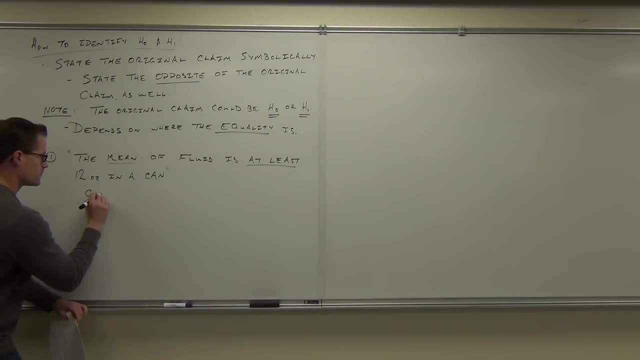 So, on every single hypothesis test you do, you're going to, you're going to write this, You're going to write claim and you're going to write opposite. You write claim and you write opposite. This is non-negotiable. Remember how I tell you sometimes, if you don't do it, 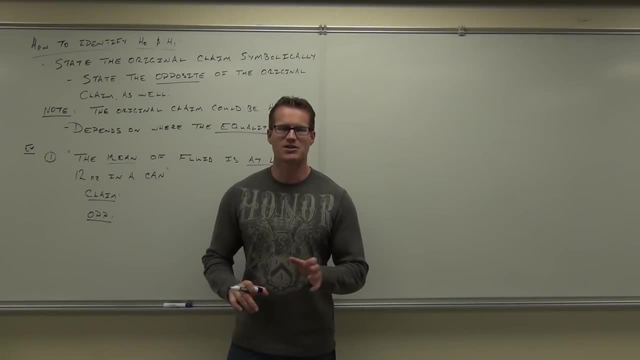 this way, you're probably going to get it wrong. And some of you listen to me and some of you don't. Once you listen to me, you get it right. Once you don't listen to me, you always get it wrong. all right. 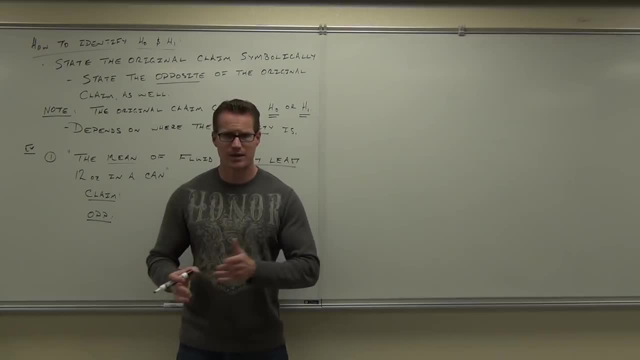 This is one of those things where you have to do it the way I tell you, Only way this stuff works right. So follow these steps verbatim. Do it exactly the same way I'm doing it and you're going to be okay. 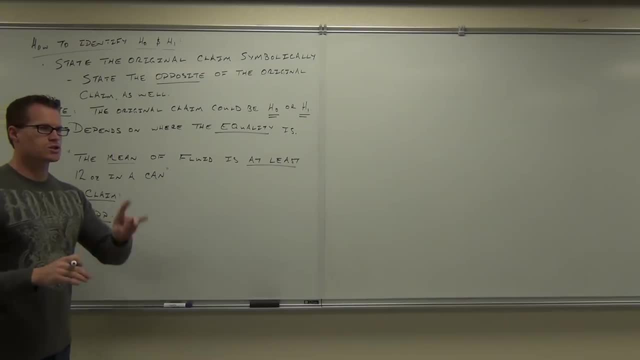 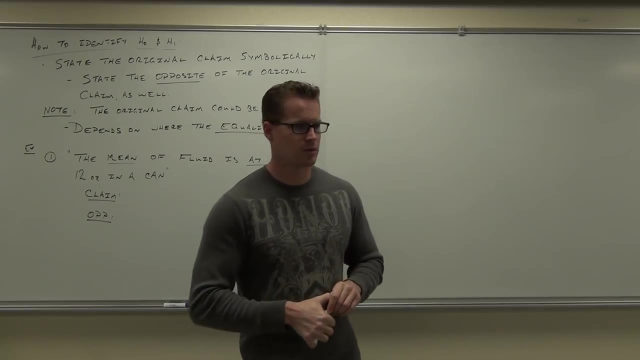 So, first thing we do, we have to state the claim symbolically. So you just determined that you're talking about a. what was it? a mean or a proportion? Are you going to use the letter P or the letter mu, What these statements are about, by the way? I hope you understand this. 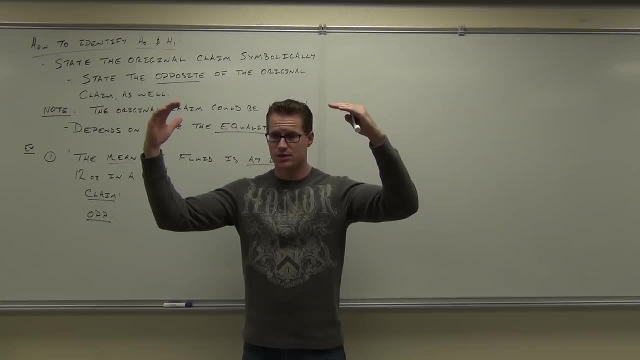 These statements are about populations. What we're doing, this in this chapter, is taking samples, using that as evidence to test a claim about a population. Why would we want to test a claim? Why would we want to test a claim about a sample? 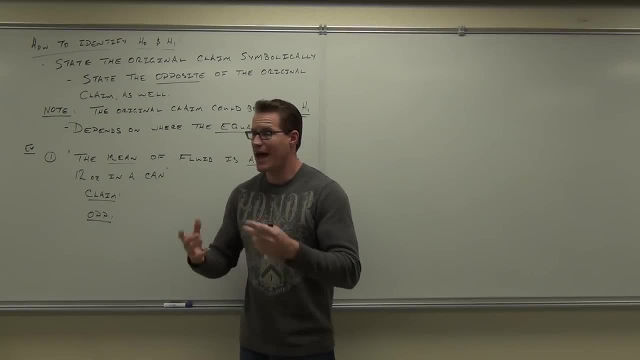 You have all the information about the sample. You don't even need to make a claim. You have everything there. Does that make sense to you? What you don't have is information about a population. So what this says is: use your evidence to confirm or reject some statement about a population. 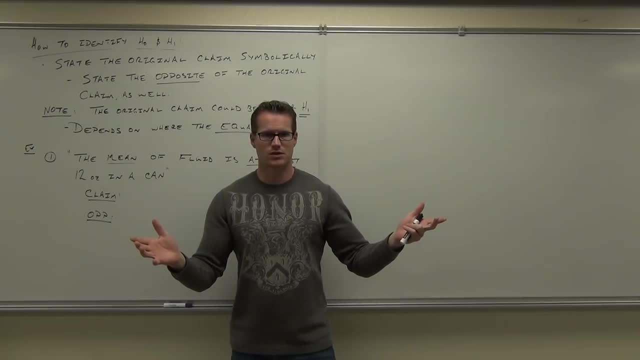 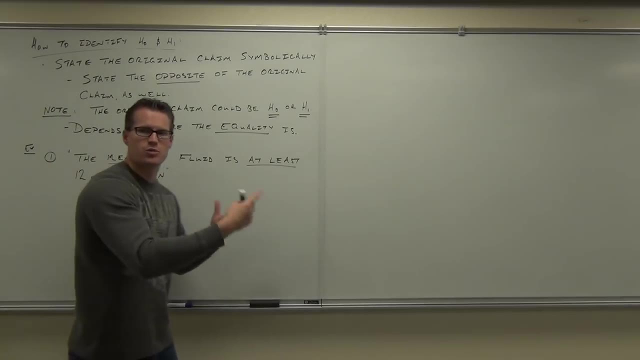 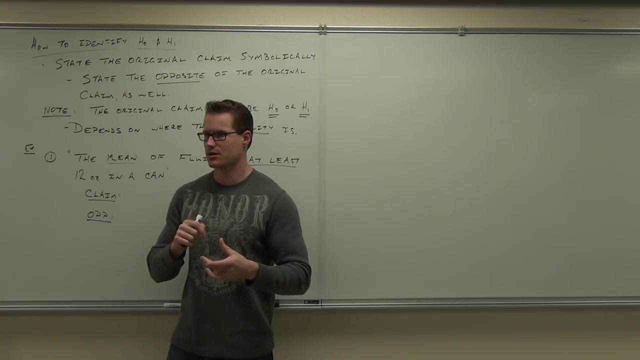 Do you get the picture here? I hope you get the picture here. Do you get the picture here? So we're testing claims about populations. So these claims are all going to be based on population parameters. That's P, that's mu, that's sigma, that's not x-bar, that's not p-hat, that's not s. 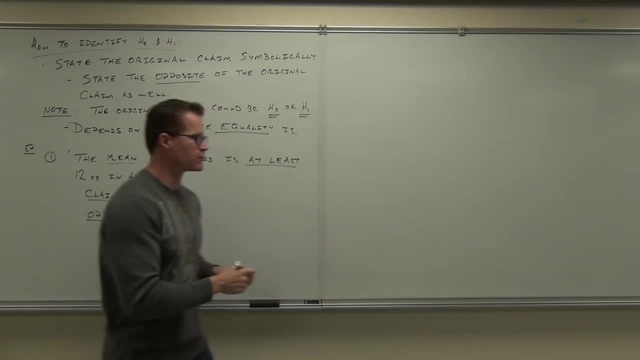 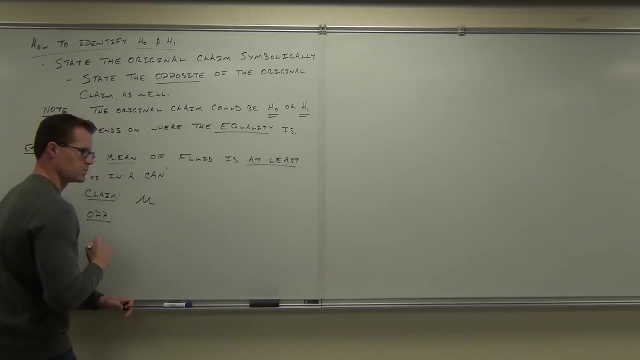 Are you seeing the difference? Those would be sample stuff that we already have all the information for. So we're testing a claim about a mean. What letter do we use then? Mu Mu Mu. Okay, Now you've got to translate. the mean of fluid is at least 12 ounces in the can. 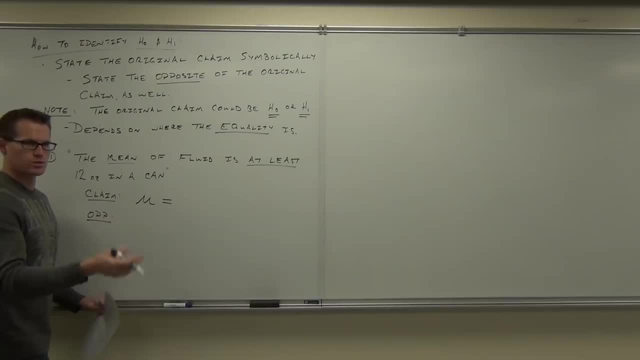 Does this mean at least No? No, That means is That's equals to? How would you say: at least, At least, At least Yes? Is there a difference between those? Yes, You know what That's going to be. the key point in finding out these claims is: can you determine this? 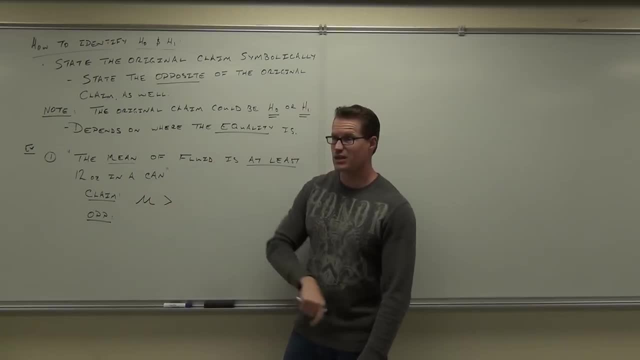 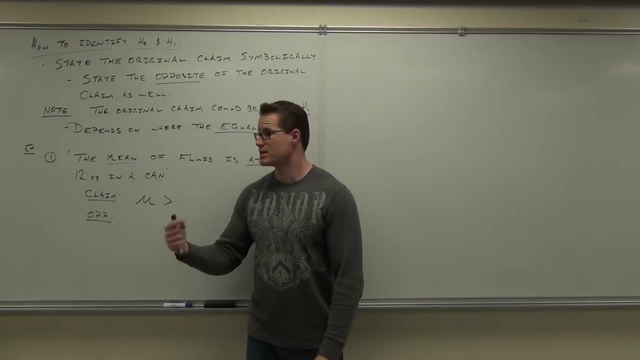 thing appropriately for your claim. If you put this, you're going to get the wrong answer. It's that big of a deal. So you need know what, at least at most. more than greater than greater than greater than less than all those things could be mean as far as inequalities go. 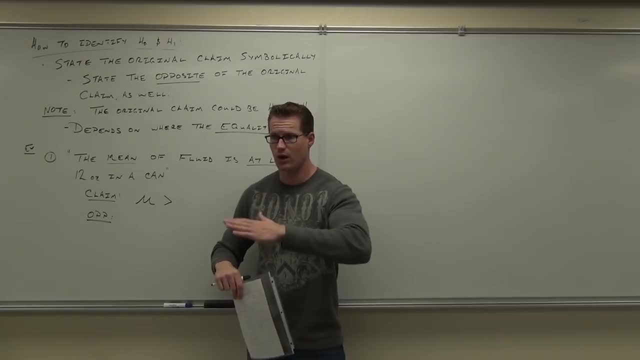 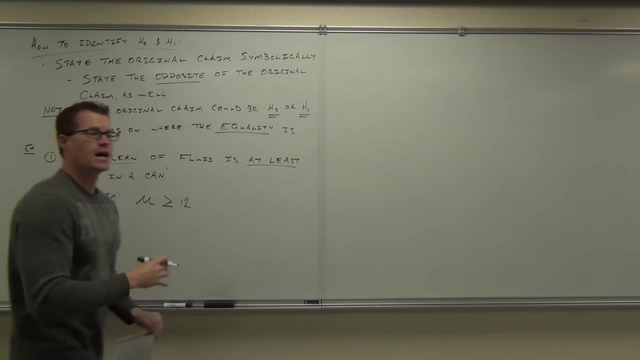 If I say I have at least 12 ounces, that means I could have 12 or more. Does that make sense? That gives you that equality right there. Now, that's all you have to do to translate your statement into your claim. 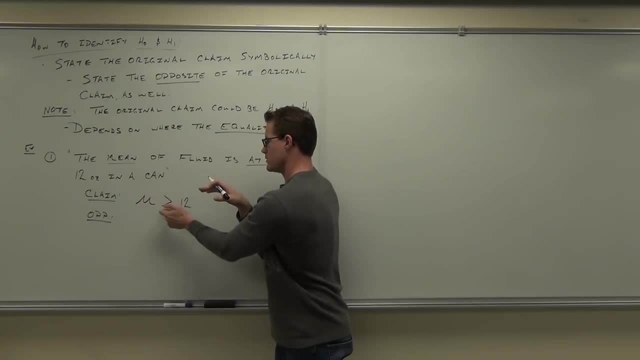 This is your claim. The mean of fluid is at least 12 ounces. mean at least 12 ounces. How many of you feel okay with that? so far, Good, All right. Do you agree with the claim? Now state the opposite of the claim. 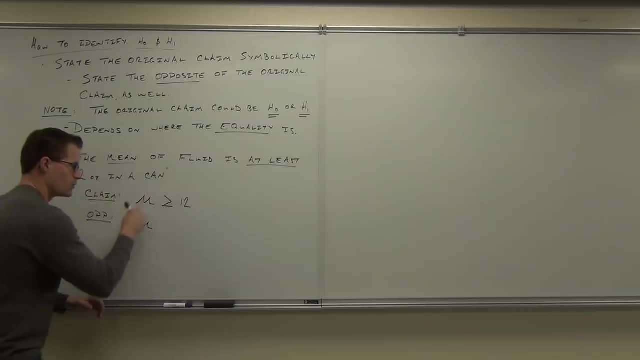 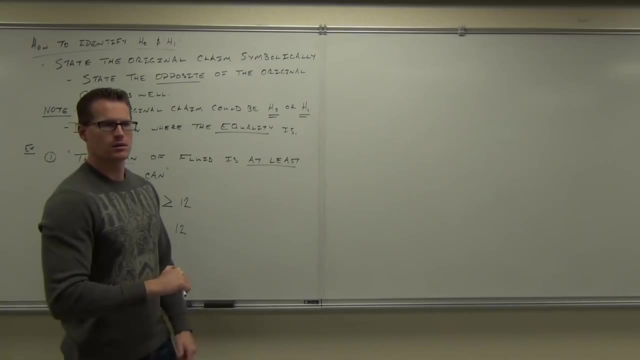 You're going to have exactly the same numbers and letters. So mu is mu, 12 is 12.. You just have to state the opposite part of it. What's the opposite of that? Less than Say it again, Less than. 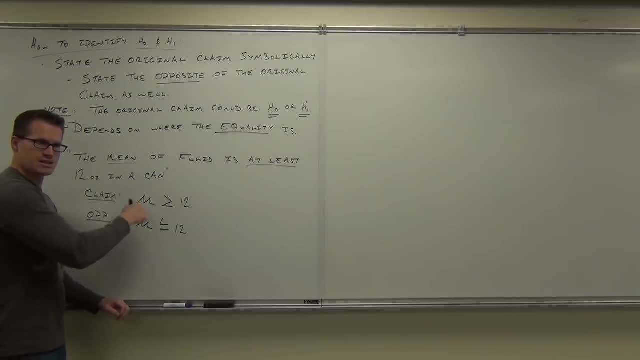 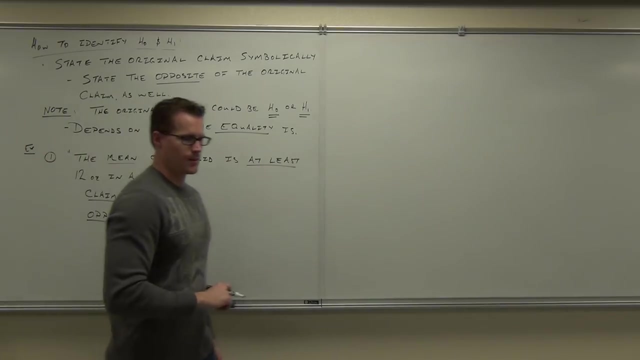 Less than like that. Is this the opposite? No, Notice how you have equals two places. That can't happen, It cannot happen. So if you have greater than or equal to, the opposite of that is strictly less than So we state the claim and then we state the opposite. 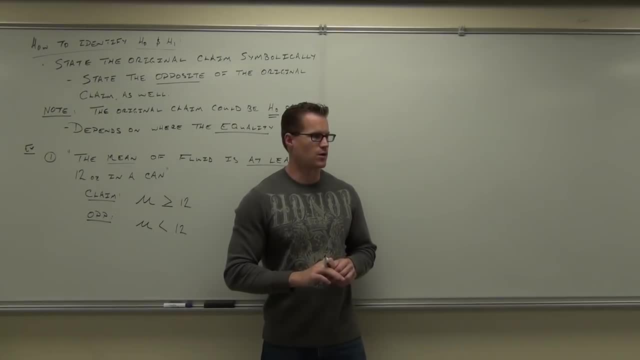 I need a nod of heads. if you're okay with that so far, You sure That's a big step. That's step number one is just doing this. Do you got it Now? Now is the part where you identify which one of these statements is h sub zero and which. 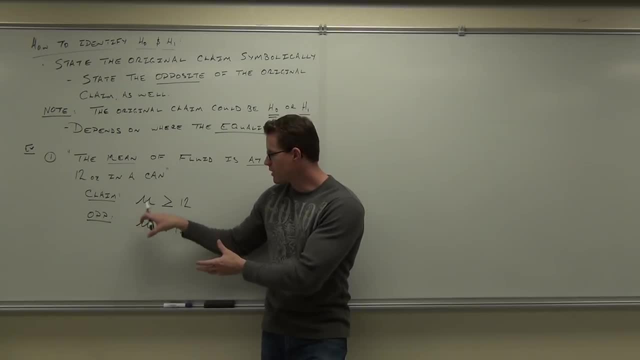 one is h sub one. It could be either one here. It depends on what these symbols are. All right, There's no rule that says: oh, your claim is always h sub zero. It's not. There's no rule that says: your claim is always h sub one. 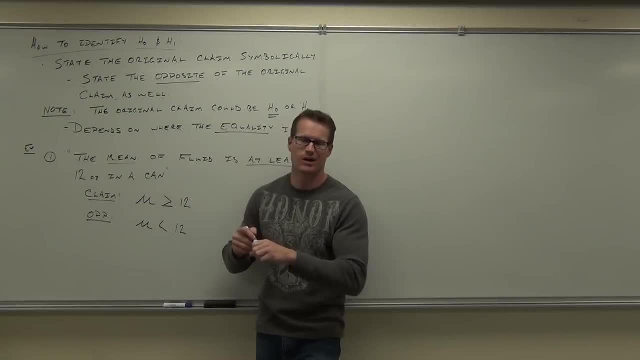 It depends on how it's worded. Notice that. oh, I'll show this in a second. Okay, I need you to notice where the equals is. Where's the equals? Is it in the claim or the opposite of our claim? 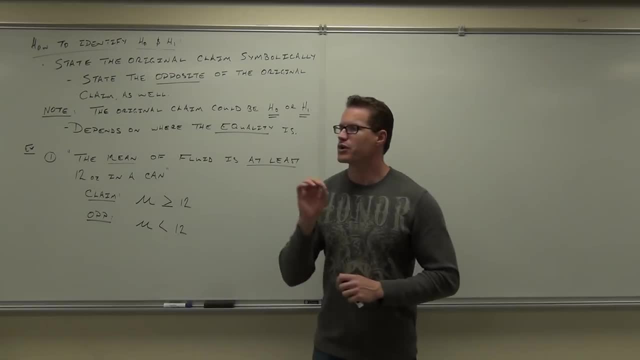 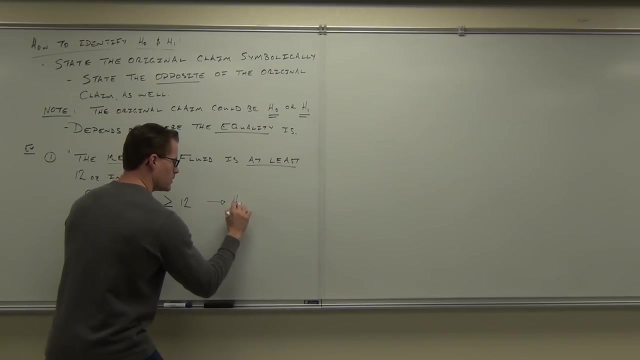 It's in the claim. It's in the claim. Wherever your equals is, that is your h sub zero. So have you identified which one is your h sub zero? Is it the claim or the opposite Claim, Claim? So wherever your equals is, that's your h sub zero. 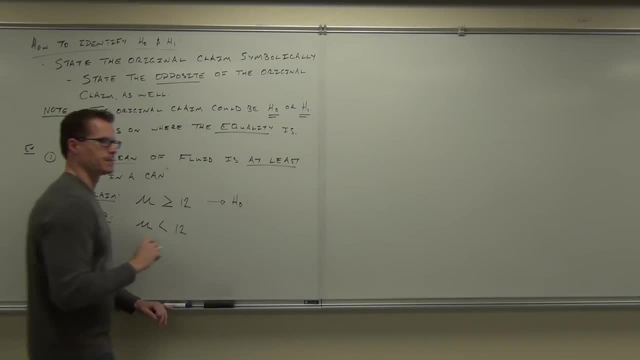 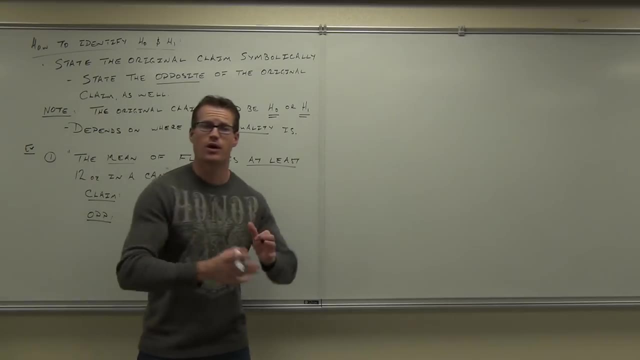 And you're going to slightly restate it. So your idea is: you write the claim, you write the opposite in symbols, you identify where your equals is. You're going to have an equal somewhere. It has to be there. It's either going to be here or in the opposite. 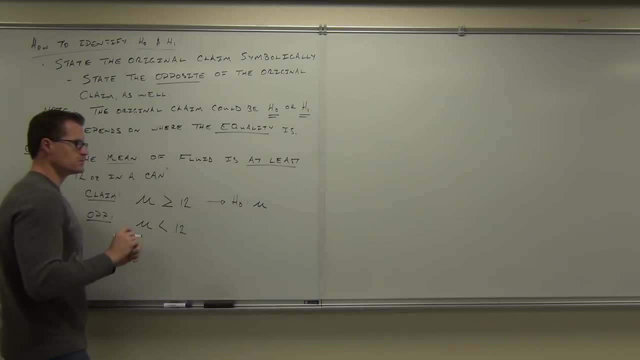 You're going to rewrite this mu. This is something that's kind of new in statistics. They didn't always do this. Sometimes they left this symbol the way it is. However, in this kind of modern era of statistics, what we do is: wherever you have the equals. 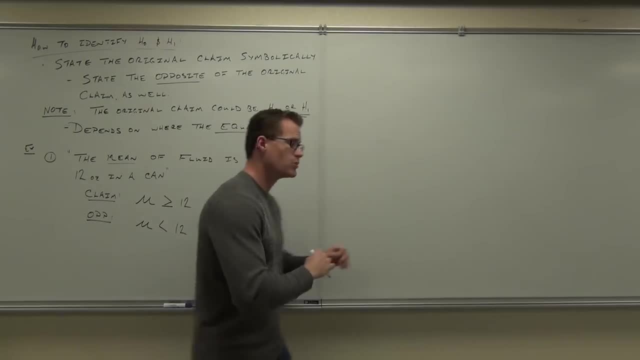 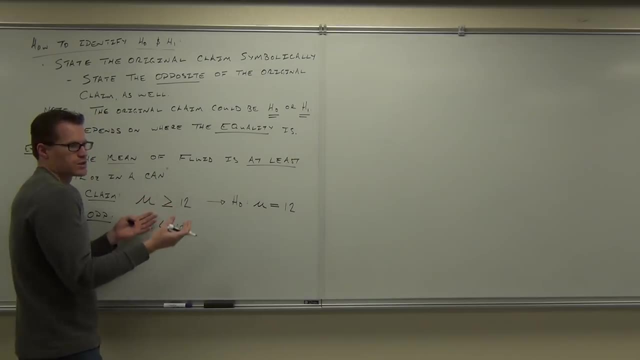 you're going to completely omit the greater than. You don't care about that. What you really want to show is equals 12.. Yes, you're looking for the mean that's greater than or equal to 12, but according to statistics, 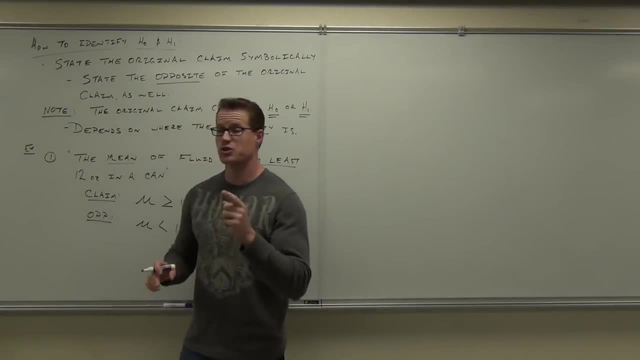 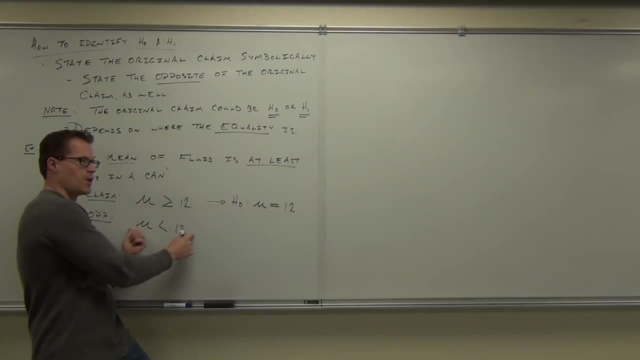 we're going to make that equals 12.. That way we don't get confused on a later step. I'll show you why when we get to that later step Right now. you've just got to buy into this right now. Identify your claim and your opposite. 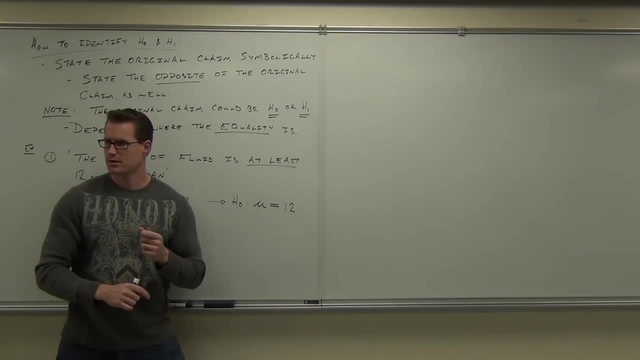 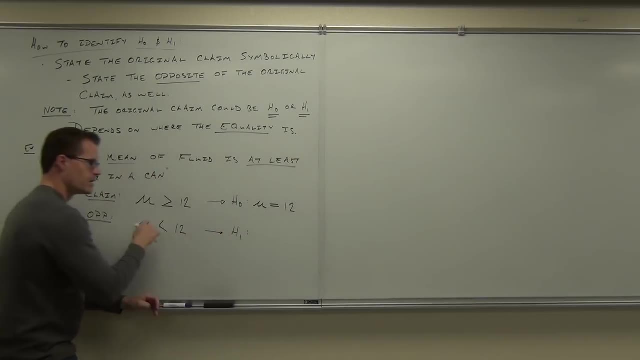 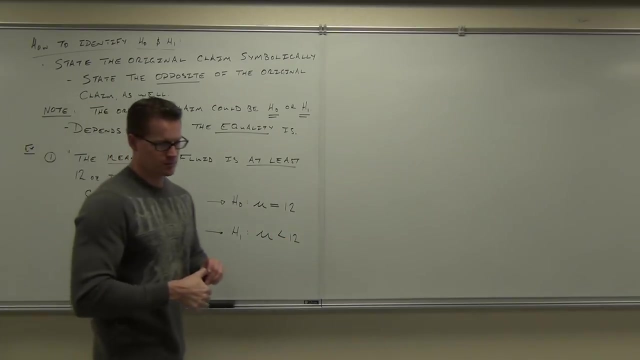 Whatever your equals is, just write equals. Can you do that for me? Yes, No, The other one, you leave it exactly like it is. In this case, h sub 1 has no equals. We write mu less than 12.. 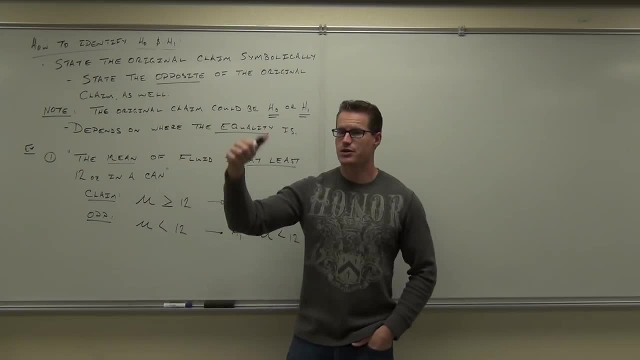 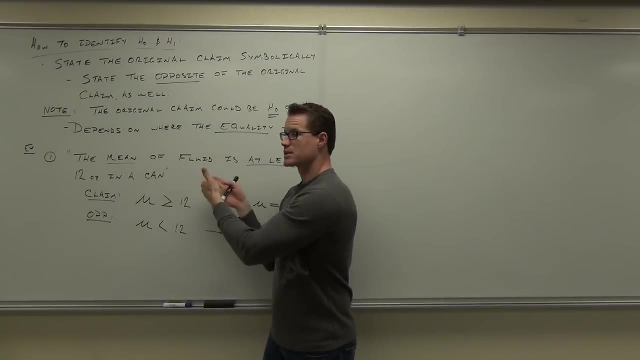 So just a very small recap. You read a claim, You identify whether you're dealing with proportions on one hand, or means on the other hand. That's p, That's mu. Here we're dealing with a mu. You write the claim in symbolic notation. 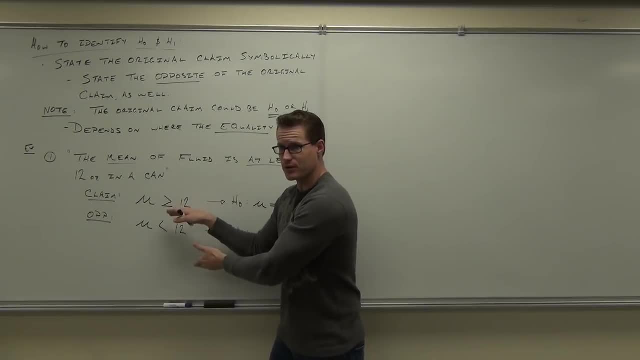 We've got that right here. You write the opposite of the claim. You have to be very good at that, don't you? Then we translate this: Which one is h sub 0?? Which one is h sub 1?? You look for the equals. 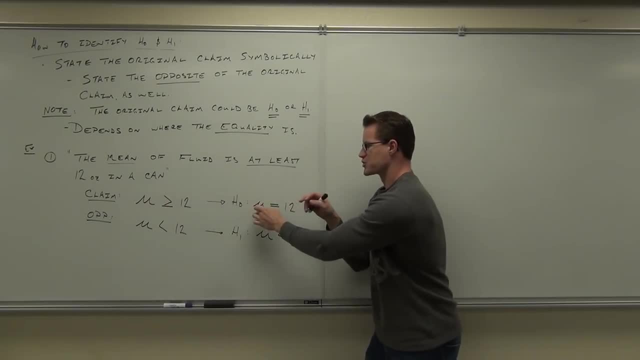 This has the equals. That means my claim is h sub 1. I just rewrite it without this greater than or equal to. just with the equal to. That's just the formality of writing statistics in this age. That's what we do. 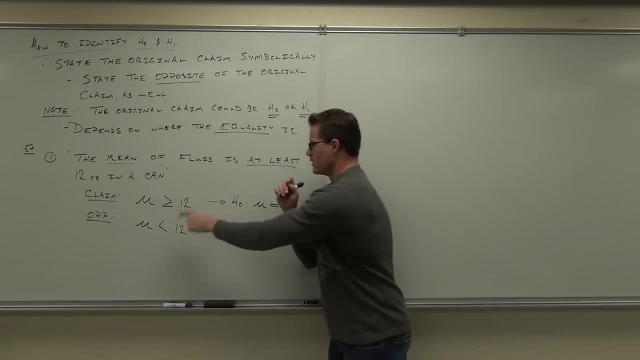 Some other books. Some other books don't have that. The opposite in this case was our h sub 1, because we have no equality statement. There's only been an equality statement on one of these pieces here, So we just simply rewrite it as h sub 1.. 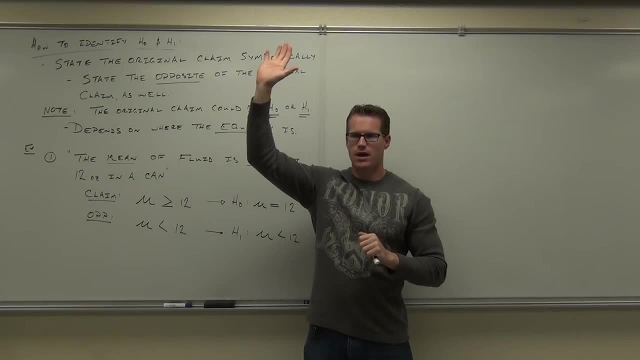 We have mu is less than 12, originally okay with this so far. Now, notice something. That's good, That's everybody. Notice something: If I didn't have, at least if I had more than if I had more than that wouldn't be there. 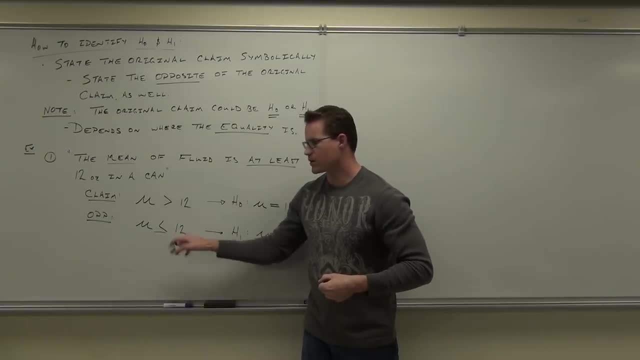 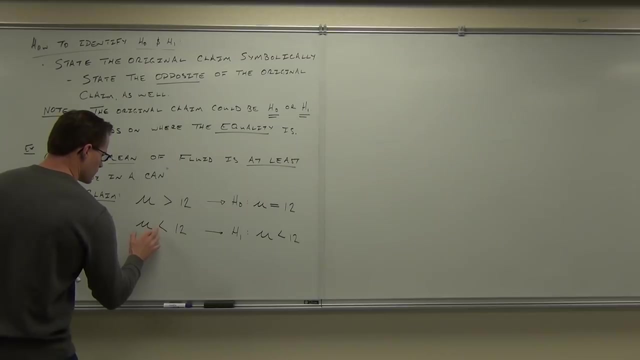 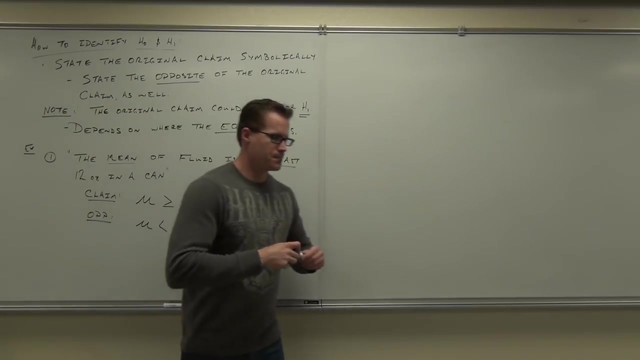 Do you see that? That would actually be here? Does that make sense? That would no longer be h sub 0. That would be h sub 1 and that would be h sub 0.. You with me? Do you remember me saying that in order to prove a claim, right, it's got to be stated? 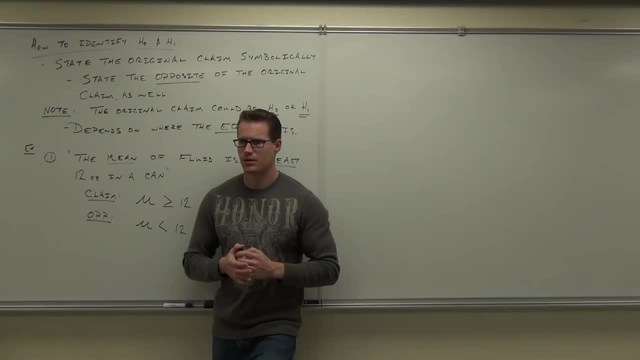 as h sub 1?? Which one? h sub 1.. h sub 1.. That's got to be stated as h sub 1.. That's got to be stated as h sub 1, because you're trying to prove h sub 0 wrong and that. 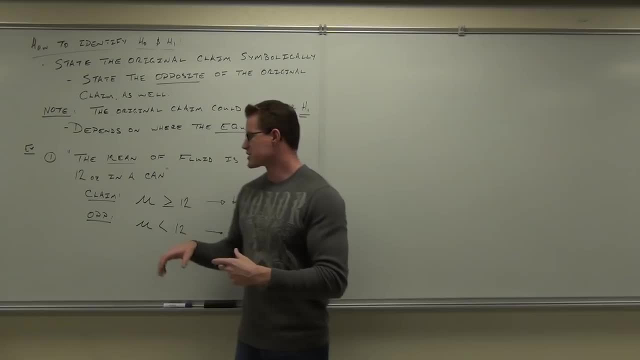 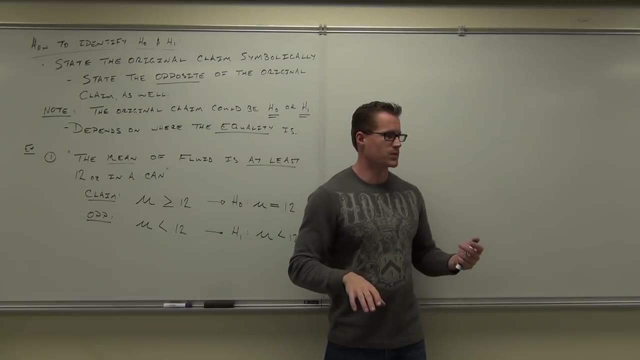 statement proves h sub 1. correct This statement. our claim is h sub 0.. We're never going to be able to prove that right. We'd never be able to prove it equal to 12.. It's impossible, You can't do it. 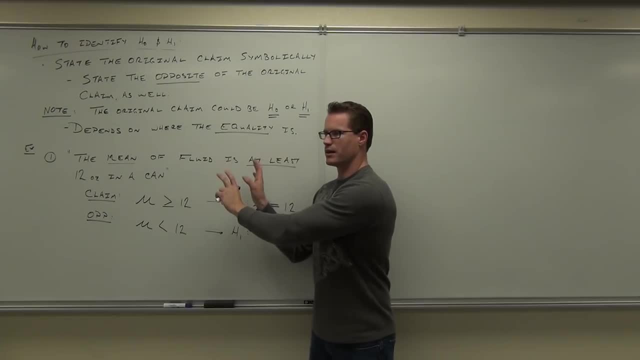 Not with statistics. okay, So we wouldn't actually ever be able to prove that claim. It's stated incorrectly for us to prove it. If we wanted to say that the fluid is greater than 12 ounces, we could prove or disprove that statement, but we can't prove it equal to 12 ounces. 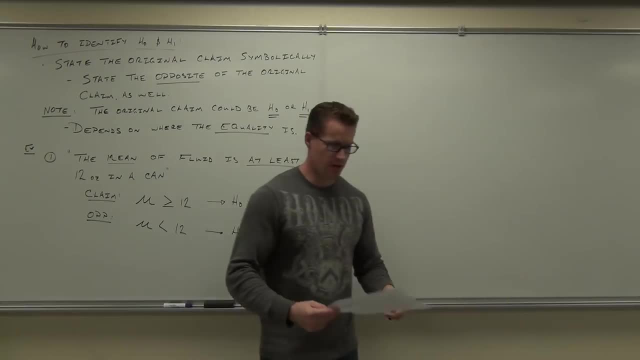 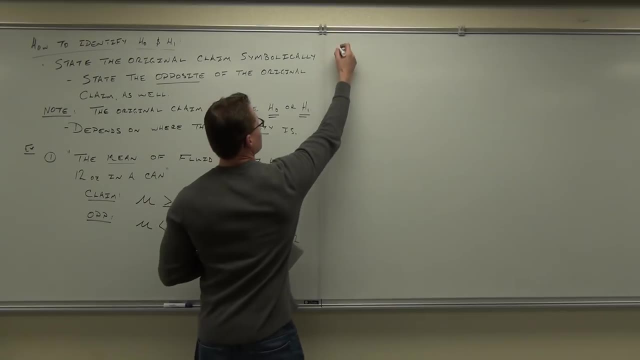 That would be stated incorrectly. if you wanted to prove that statement right, Did you guys kind of get the picture? All right, Let's try a couple more. We'll try three more. Of course, I really need you to get this before we move on right, because if you don't get, 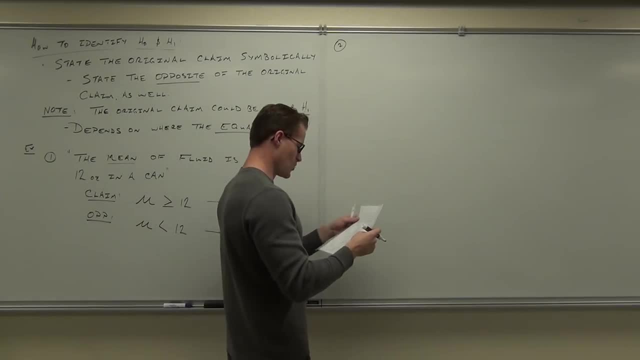 this. you're stuck. There's no way you can get any further. So let's try a few more of these things. Let's say, the proportion of male CEOs is greater than 0.5.. Let's try a few more of these things. 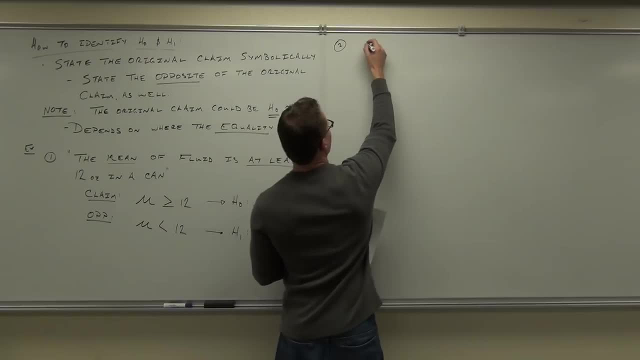 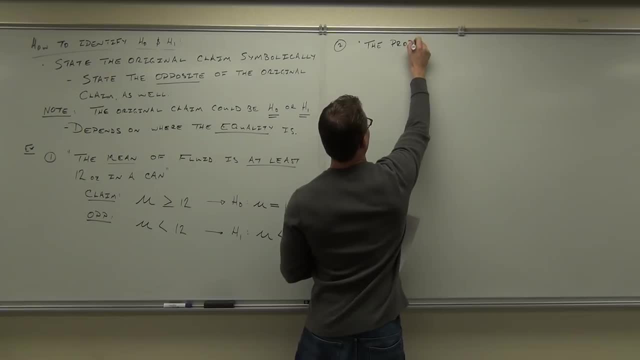 By the way, the proportion is 3.2 procent of male CEOs. That's T, That's T. Let's try this one. Let's try this one. T is greater 3.2 percent of male CEOs. T is greater 3.2 percent of male CEOs. 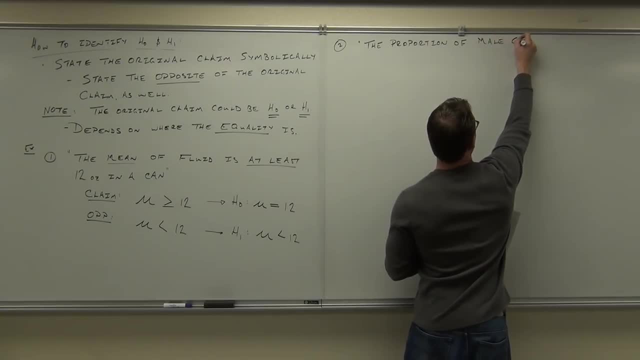 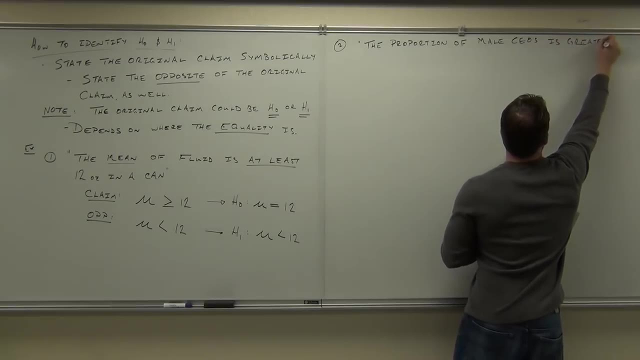 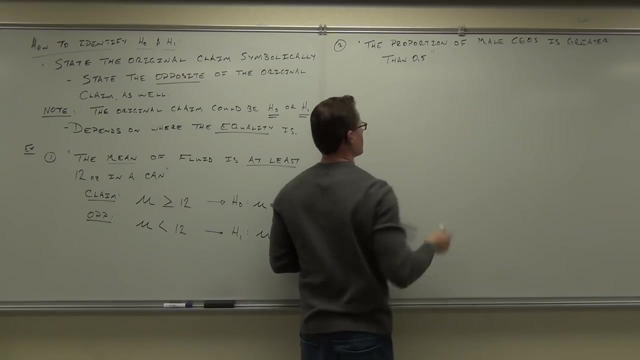 T is greater, 4.0 approach- And only around that, And only around that. T is greater through a million times T is greater in percentage: 0.8 percent 🎵, 0.5 pascals. I also want to show you this in this example. that's why I gave this one. 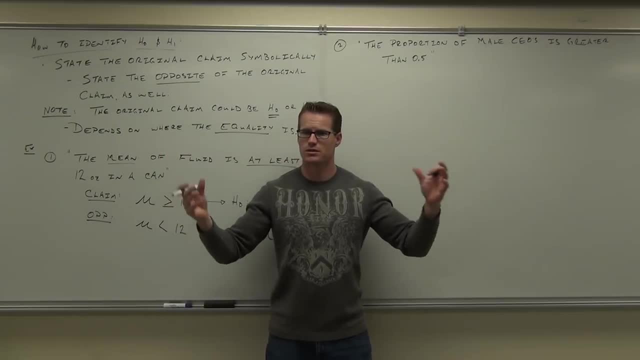 The proportion of male CEOs is greater than 4.5.. Are we dealing with proportions or means Proportion? Clearly, because it says proportion up there. But check this out. what if I worded it a little bit different? you should still be. 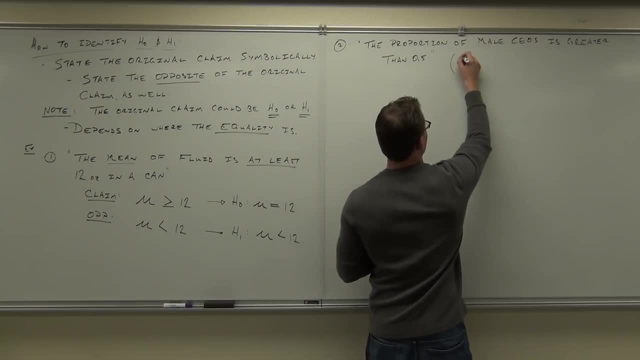 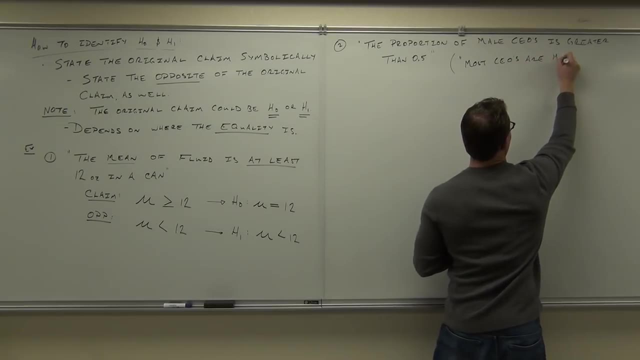 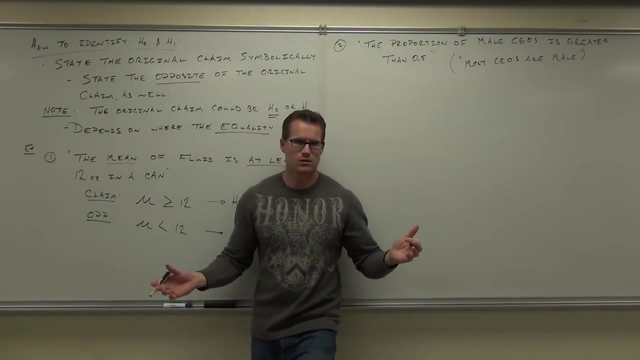 able to see that we're dealing with proportions. I could word it like this: Most CEOs are male. Right there, You see that a lot. What's most mean More than what Half. Half is 50% or 0.5.. 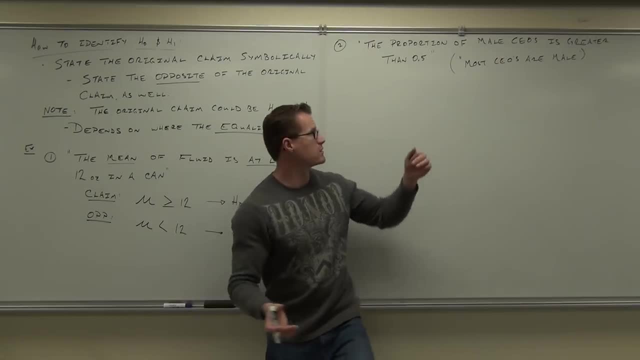 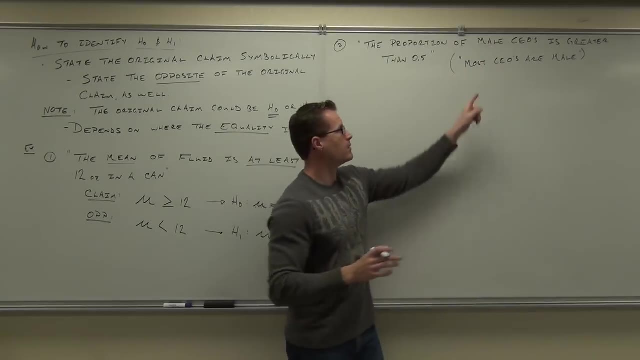 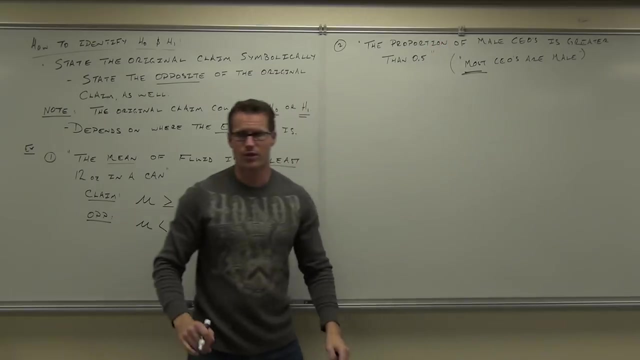 Are you with me on that? So most CEOs are males. means this: right here, The proportion of male CEOs is greater than 0.5.. So if you ever see most, most means more than 50%. Are you clear on that? Most means the proportion is more than, or greater than, 0.50, 50%- 0.50. 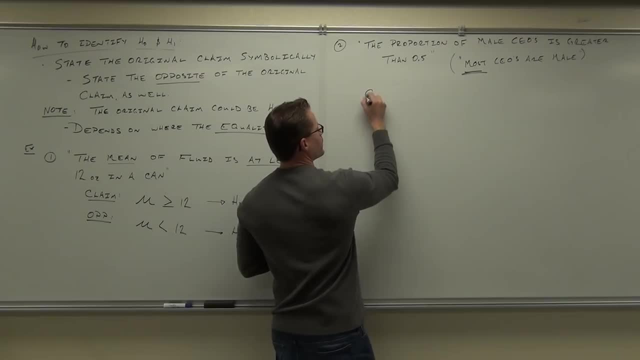 Okay. Well, you've already determined that we're dealing with a proportion, So are we dealing with mu still or with p? So we need to identify our claim and our opposite. Let's start with the claim first. We always start with the claim. 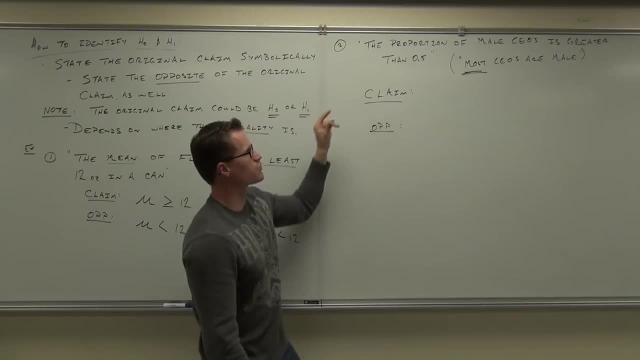 What's actually given to us. So the proportion of male CEOs is greater than 0.5.. What letter are we using again? P, Because we're dealing with a Proportion Good And we're trying to make a statement about the population proportion. 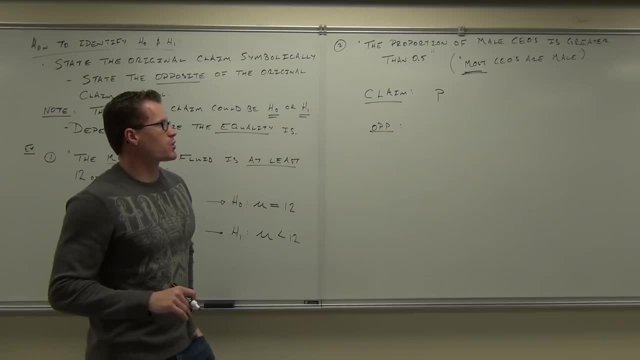 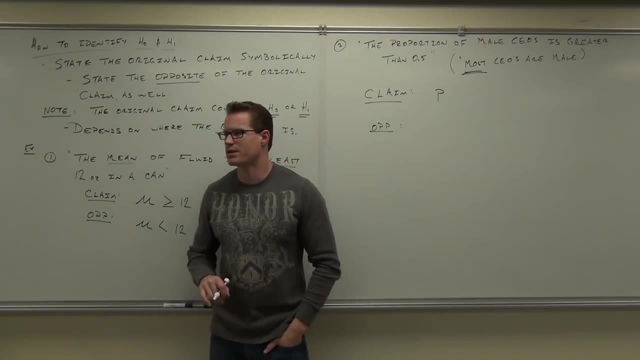 P. Can you write: proportion of male CEOs is greater than 0.5?? How would you write it? Would it be equal to A greater than or equal to A less than, or equal to A greater than or a less than? 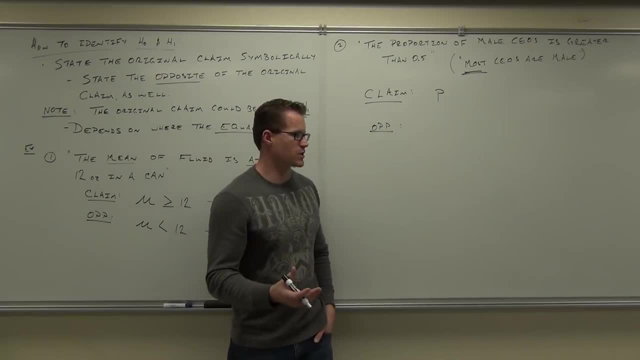 Which would you pick? Greater than There's only several. there's a few options here. right, You could do equal to, not equal to, Greater than less than Greater than equal to or less than equal to. There's six options that you have. 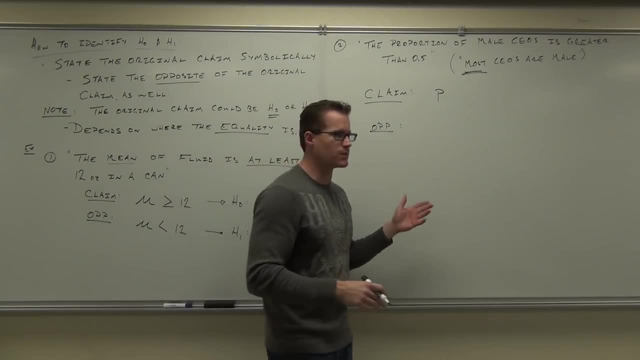 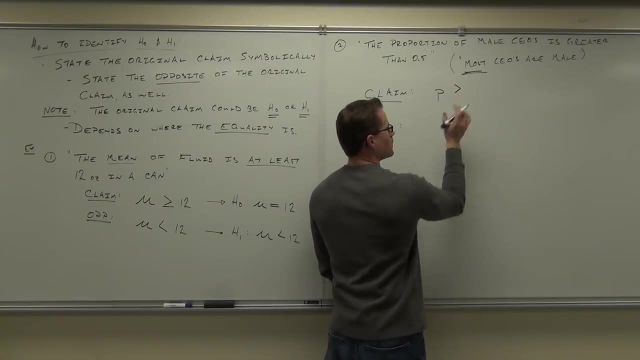 Now, only one's the correct option, but those are the six symbols you'll be using. Which one was it? The greater than Okay? Greater than what? 0.50, because this means most. You need to be really good at reading this, or reading this and getting this. 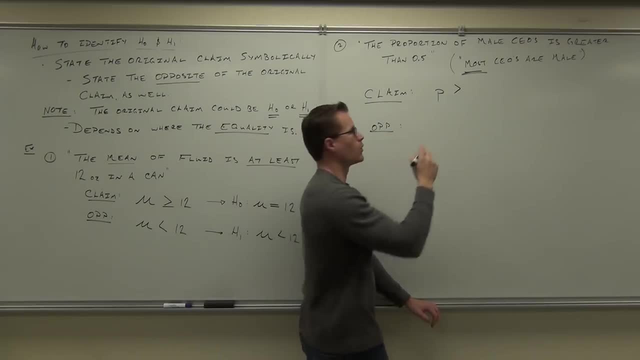 Most CEOs are male. Hey, most, More than 50%, are male. I'm not sure if you're okay with that one. so far, Yeah, All right. Now can you write the opposite of that? claim Both of them. 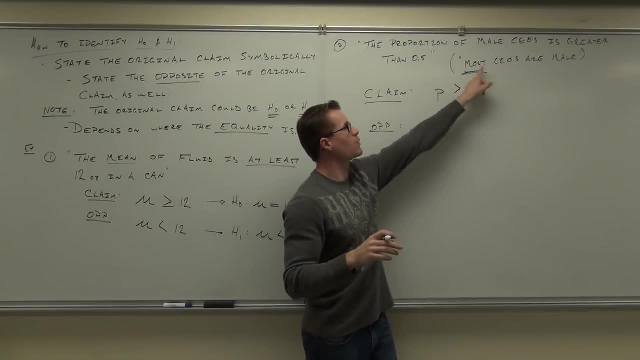 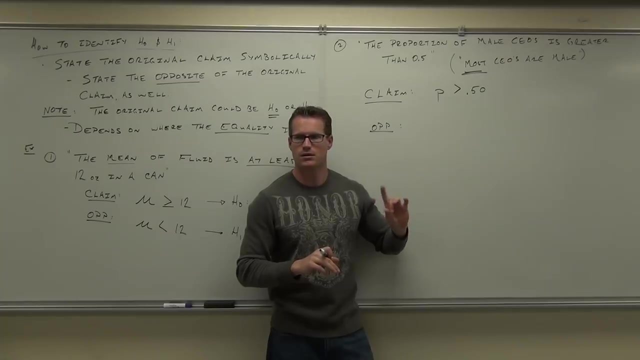 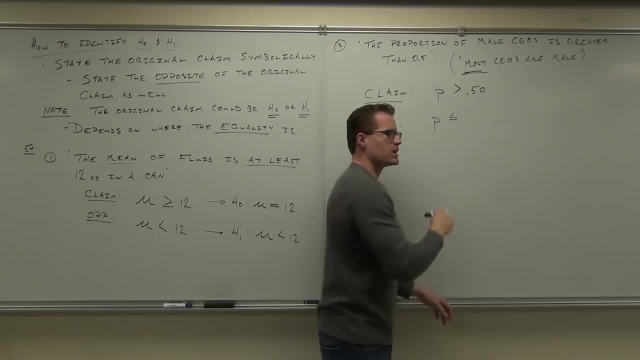 Less than, Less than, or what? Less than 0. Oh, There's got to be an equality somewhere, right, There has to be an equality somewhere, because H sub 0 has the equality. It's got to be somewhere, In our case, which is the H sub 0, the claim, or the opposite. 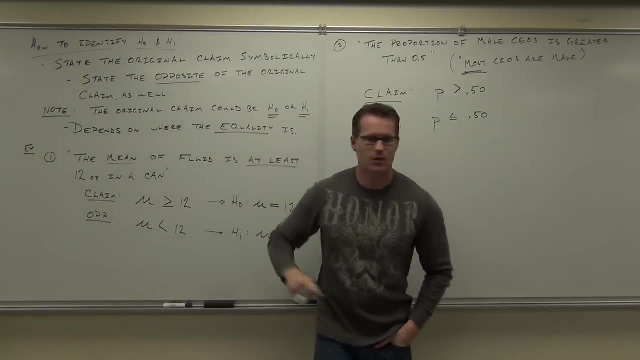 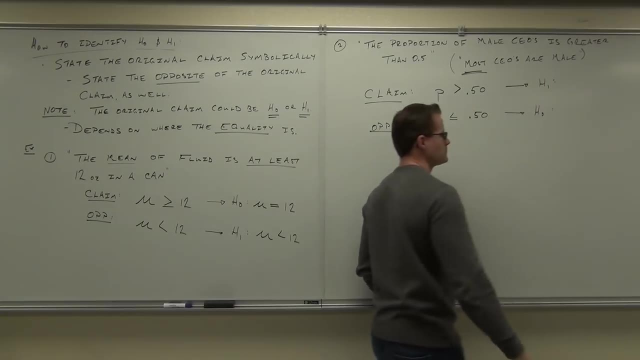 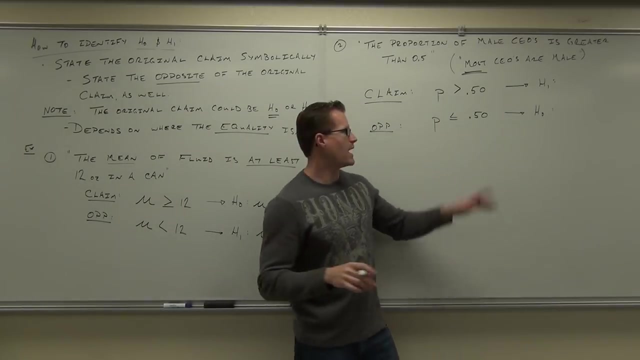 坂. So notice how it changed. It's not the same all the time, right? This one? in this case, this is H sub 0.. This one is H sub 1.. Let's rewrite H sub 0 first. H sub 0 has the equality. 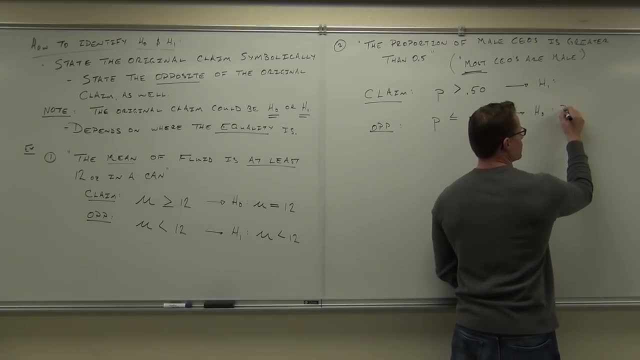 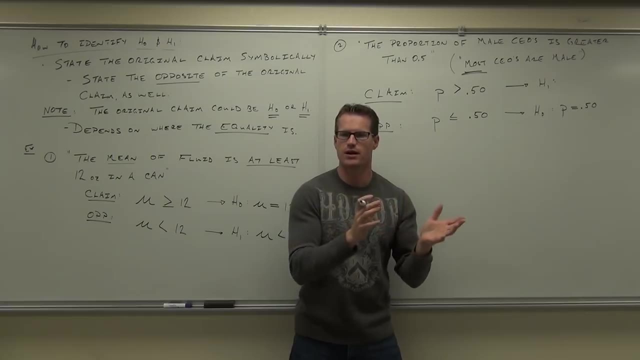 Equality is right here. so we write what now: P equals Good, We kind of ignore this part. once we find the equality, We just write equals to make it a simplified version of this scenario. Now, as far as H sub 1, we don't change that ever. 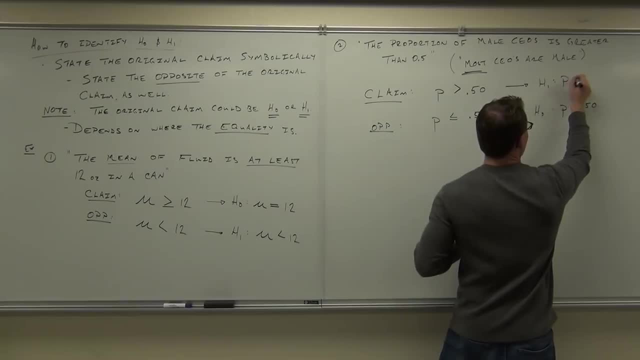 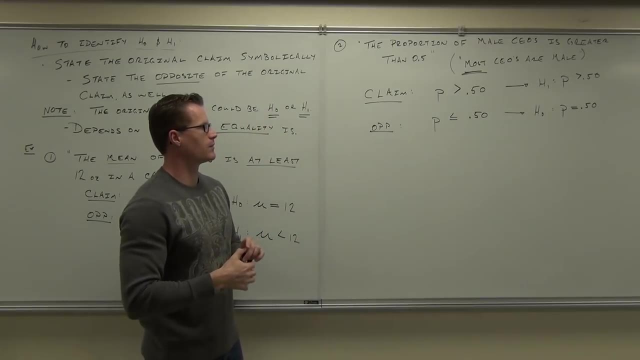 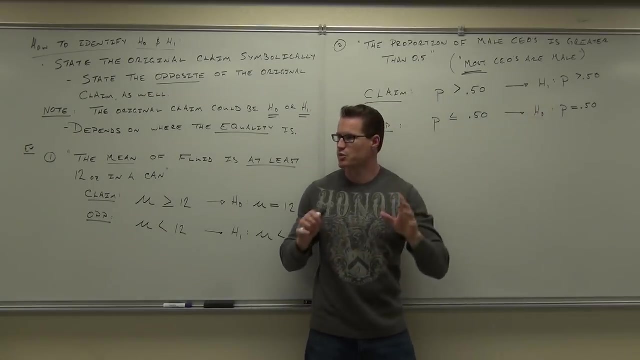 H sub 1 stays exactly the same. It doesn't have an equals to it P greater than 0.50.. Notice how your claim. listen how your claim is your H sub 1.. Here's how this would work. We're going to be stating H sub 0s and trying to prove them wrong. 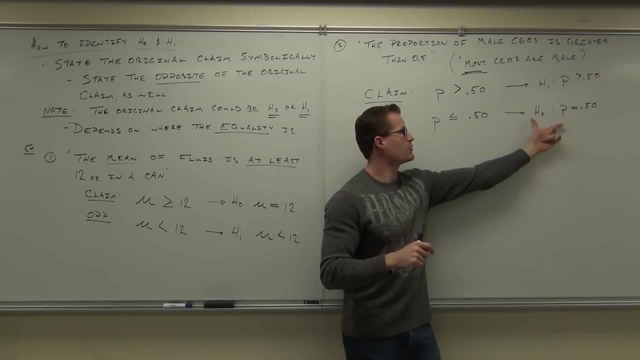 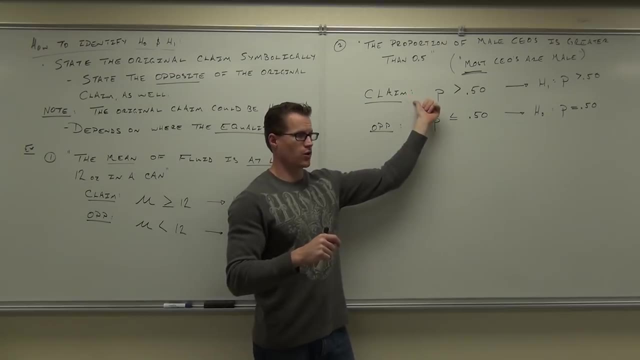 If we prove our H sub 0 wrong, we prove our H sub 1 right. Does that make sense? If we prove our H sub 1 right? look what we just proved. We just proved, We just proved our claim. Do you see how that would prove our statement? 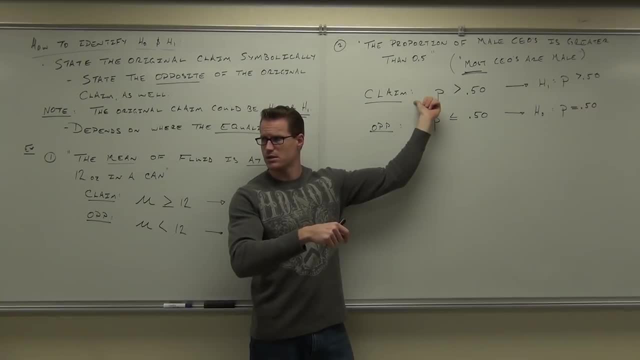 if we state our claim as H sub 1?? No, Yes, Iffy, Some people are iffy. The only thing you can do is disprove H sub 0.. That's all this whole process does is disprove H sub 0.. 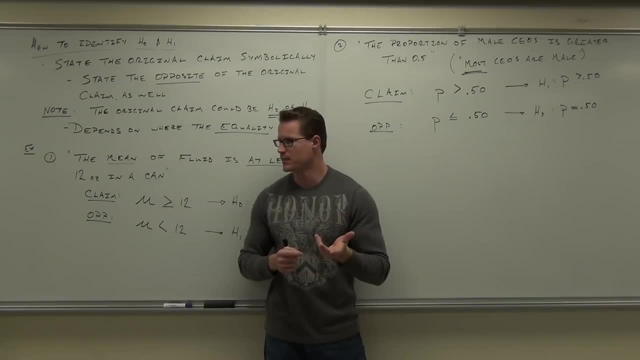 You can either disprove it or fail to disprove it. Failing to disprove something doesn't prove it right. It's like guilty versus not guilty: You can find it guilty, Disprove it, Or you can find it not guilty. 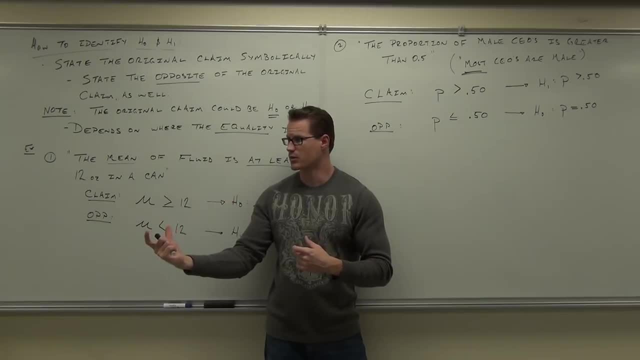 Fail to disprove it. Guilty means they got caught and they're punished Right. Not guilty doesn't mean they didn't do it. There's just not enough evidence. Do you see the difference there? That's what you can do with H sub 0.. 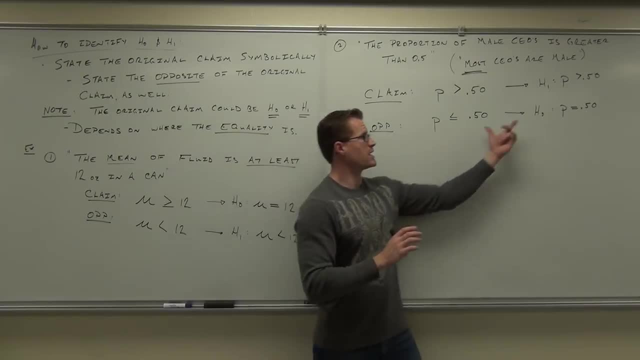 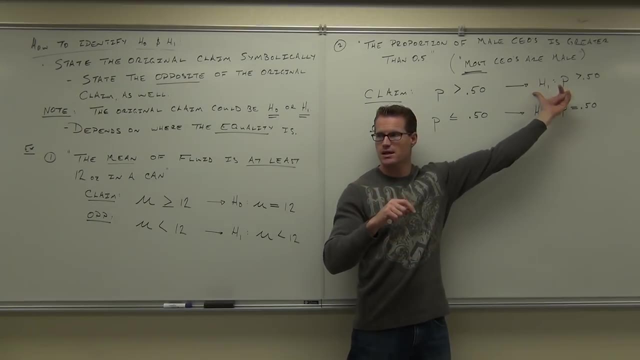 You're going to be testing H sub 0. So if you test H sub 0 and find it wrong, that means H sub 1 is right. If you can find H sub 1 right, that means you proved this statement. If your statement's set up as your claim, you just proved your claim. 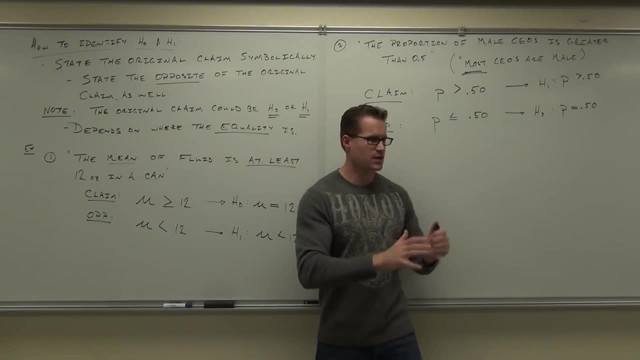 Compare that to this. Remember, you can only test H sub 0, not H sub 1.. So let's say you tested H sub 0. If you found it wrong, your whole claim is completely wrong. Right, You didn't prove that statement at all. 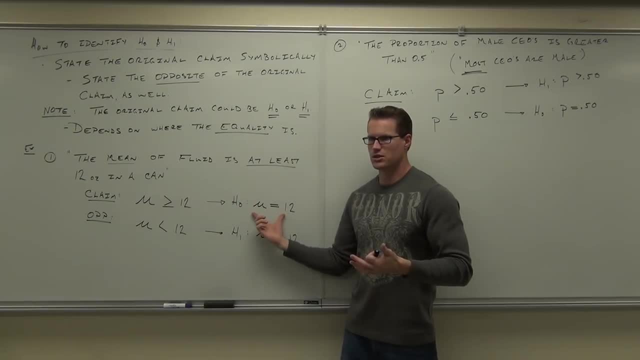 This is your claim. If you found it not wrong, did you find it right? You said nothing. You didn't say anything about that. Found it wrong? you proved this, that your statement was wrong. It's what you were trying to prove is completely incorrect. 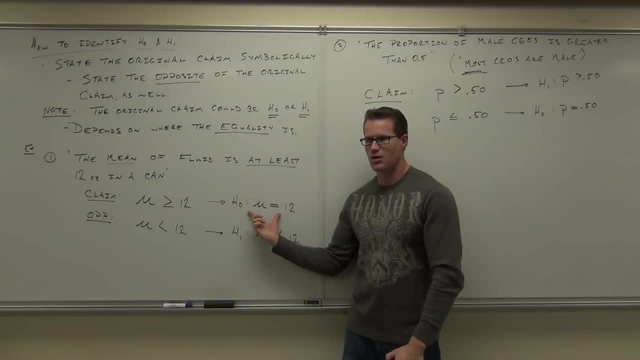 That's not good, Right. But if you're trying to prove this statement correct, well, you can't do it here. There's never going to be enough evidence to prove something right, Just like there's never enough evidence to prove someone innocent. 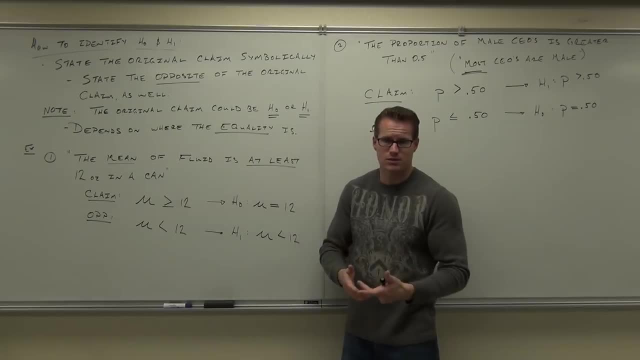 Can you ever prove someone innocent? No, It's either they're guilty or not guilty Here. you have not guilty, sure, but it doesn't prove it right. It doesn't mean that they actually didn't do it, which means there wasn't enough evidence to say that they did. 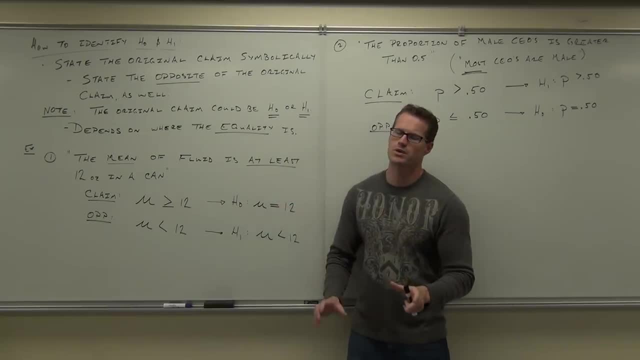 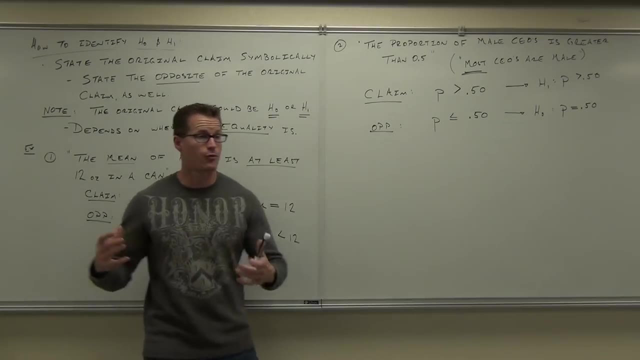 Do you see the difference between these two things? I sure hope that you do, because that's really an important piece of information. That's how hypothesis testing works. Are there any questions on it before we get going? If you're not clear on it, now is a perfect time for questions. 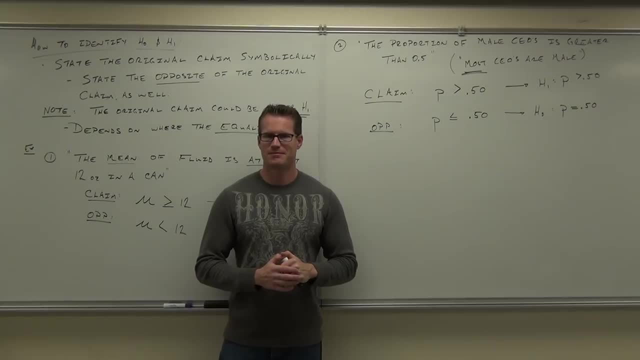 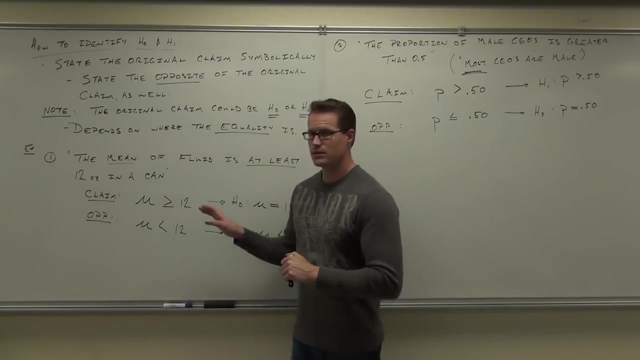 We've got time. So if you do all the math right for the first one and you figure out that the mean is actually like 11 ounces but we're looking for exactly 12, basically right, Yes. But if we find out it's actually 11 ounces and we're looking for 12. 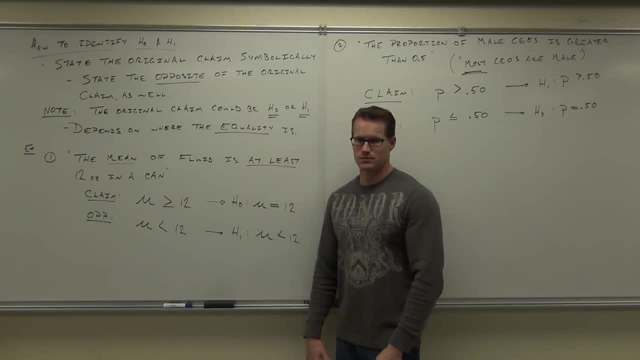 or 20.. That's what we're looking for. Then it wouldn't prove this wrong. So what would we? Nothing. That's the point, Right. It doesn't tell you anything, But we know that it's. Now let me say this. 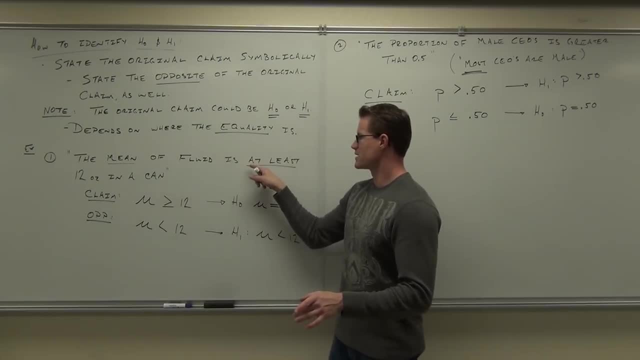 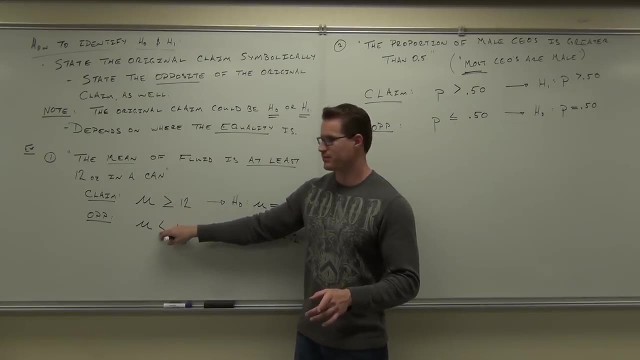 You're looking for this right. If you said the mean fluid is exactly 12 ounces of canned, that would be equals. This would be not equals but still wouldn't say anything about that. You'd have to test the claim. the mean fluid is different than 12 ounces. 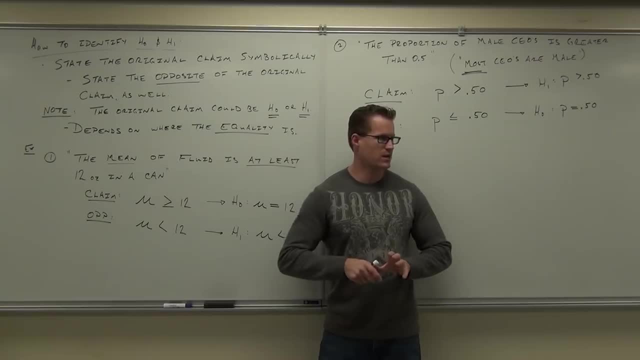 You'd have to test that claim. That way you could prove the opposite correct or, I'm sorry, you could prove the opposite incorrect. That would prove your claim for you. You can never prove anything about H sub zero. You can only prove things about H sub 1 by disproving H sub zero. 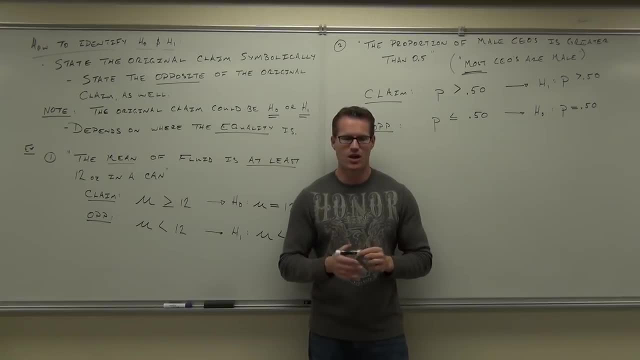 That's the whole idea. I know it's reverse logic, right, Because we're used to going: oh, we want to prove this, We're going to go directly at it and hammer at it. Nope, Not with statistics, You go like a backdoor approach. 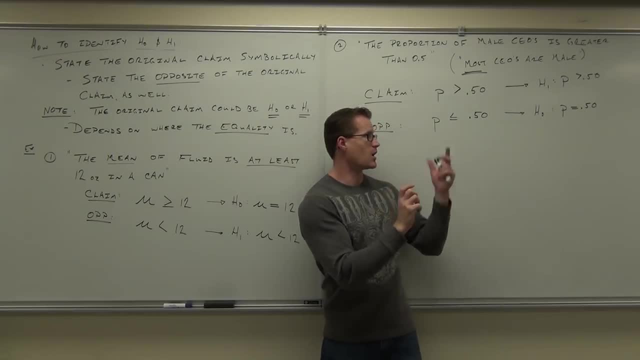 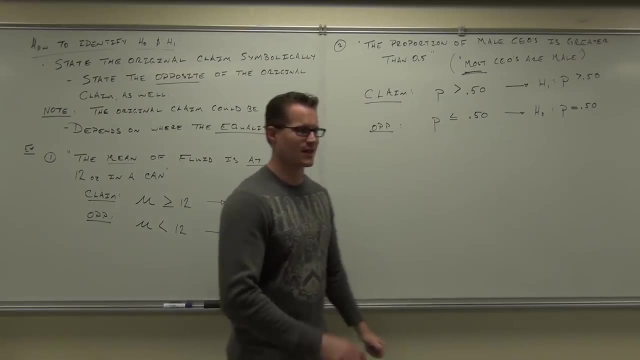 You state it kind of what you don't want, You state the opposite And you go about disproving your H sub zero to prove that claim. It's a weird way of doing it right. It's like an indirect proof in mathematics. 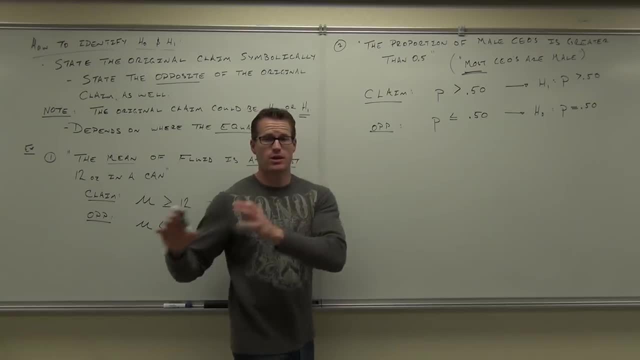 Did that answer your question? The 11 won't do anything here? Sure, it is, but it's not what you asked. This is only going to work with what you specifically asked it. That's it. That's why we have to ask the right questions to get the right answers. 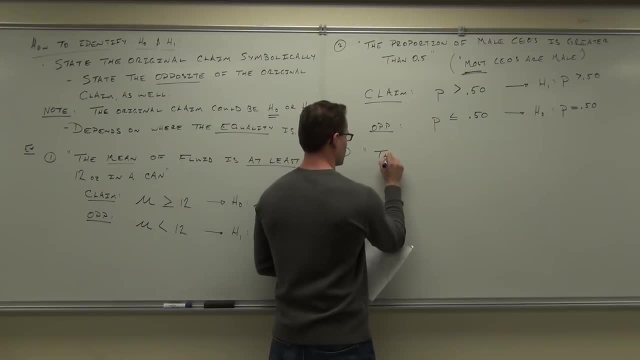 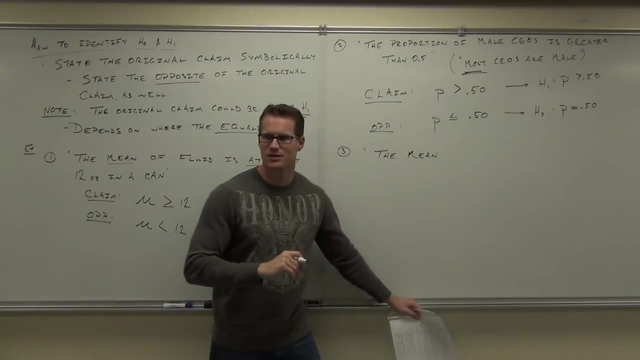 You guys ever seen iRobot? Yes, And at one point he goes: ah, now that's the right answer. And then he shuts off And you're like: oh, come on, jerk, Ask the right answer, Give me the answer. 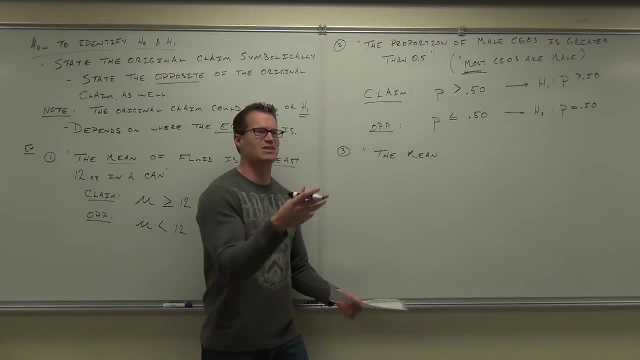 Well, that's kind of how this works, right? You don't ask the right question, He says that's the right question. He doesn't give an answer. If you don't ask the right question, you're not going to get the right answer. 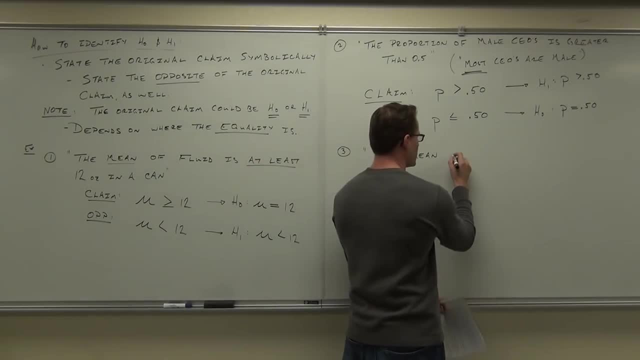 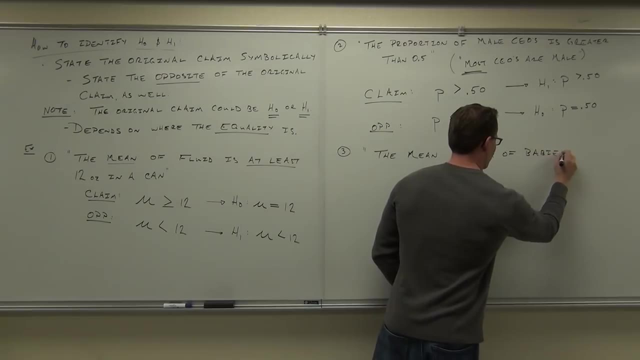 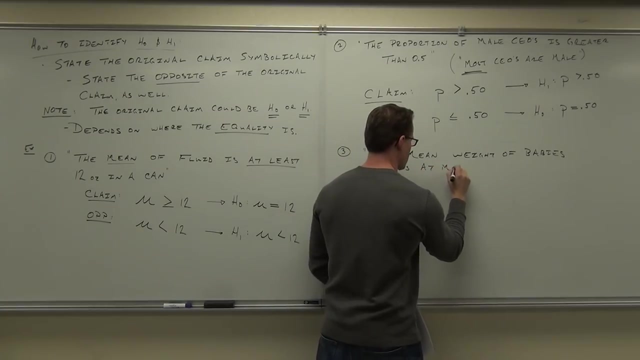 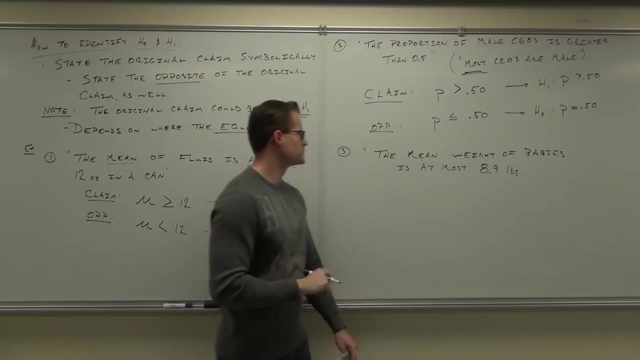 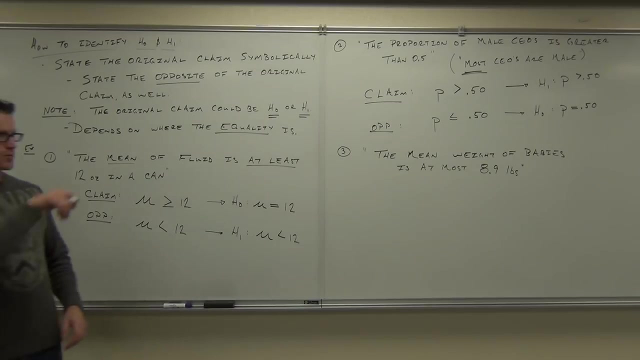 That's what this whole thing is about. Okay, The mean, The mean weight of babies. The mean weight of babies is, at most, 8.9 lbs. The mean weight of babies is 8.9 lbs. I have no idea if that's true. 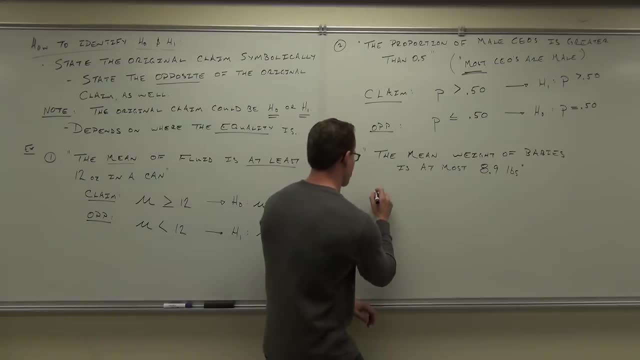 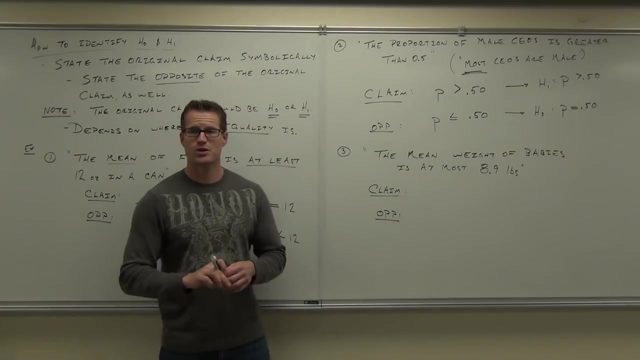 I think I just made it up. That's a pretty big baby, Smaller than my turkey. My turkey was worth like three babies. Okay, Of course we're going to try to stake the claim and state the opposite of the claim. 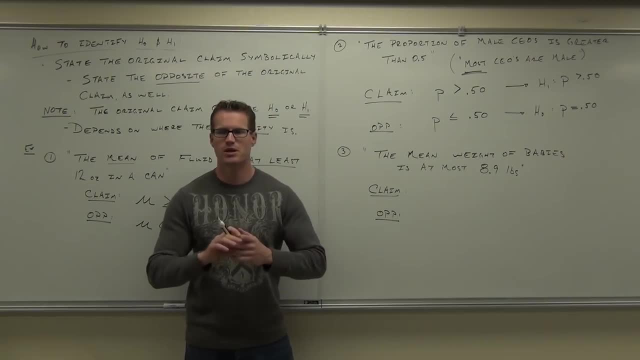 So first thing you've got to be good at is identifying whether you're dealing with proportionate or mean. which are we dealing with here? Mean, Mean, Definitely mean. So you're talking about, remember, population stuff, parameter, mean or p. 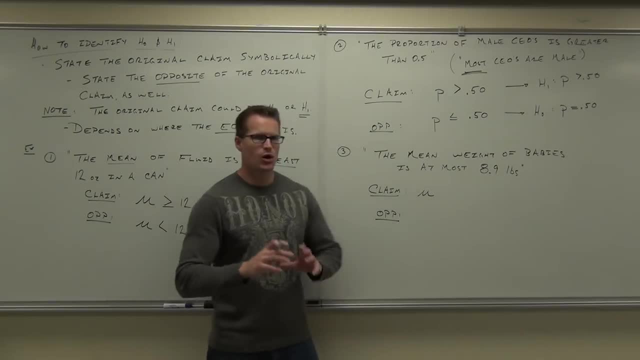 Not p hat, not x bar. The reason is you already know everything about x bar. You're going to know that stuff. It's a sample right. You were able to take samples. What you don't know about is population stuff. 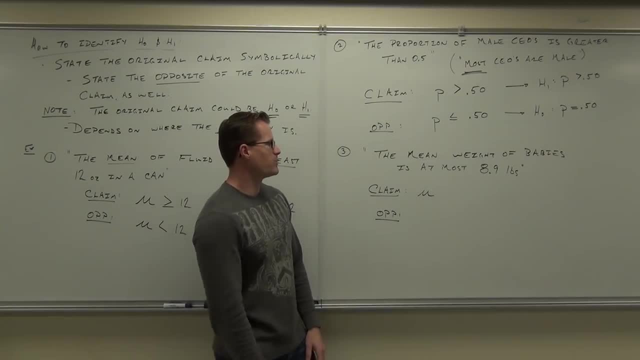 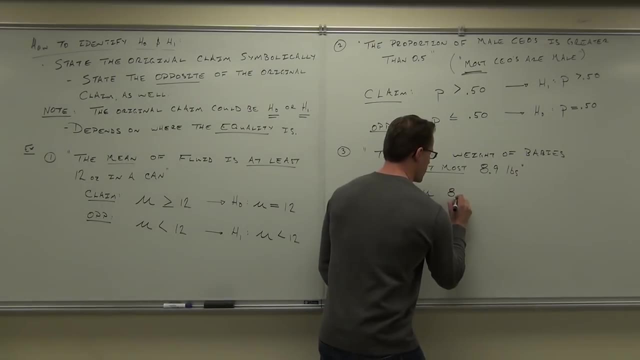 These claims are about populations. Now, the mean weight of babies is, at most, 8.9 lbs. So I know I'm going to have a mean. I know I'm going to have 8.9.. You just need to know whether it's equal to, greater than or equal to. 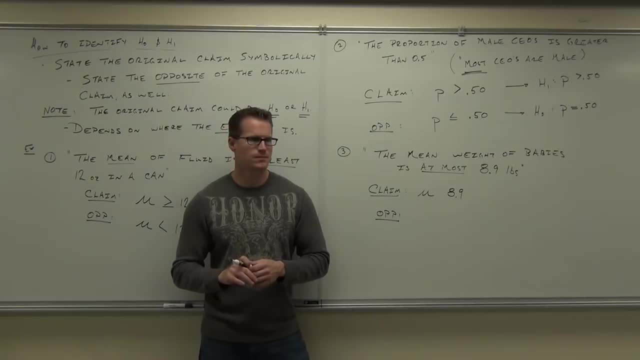 less than or equal to, greater than or less than. What is it? At most 8.9.. At most, 8.9 lbs. At most We deal. we certainly understand that the mean has to be less. it could be less than 8.9, right. 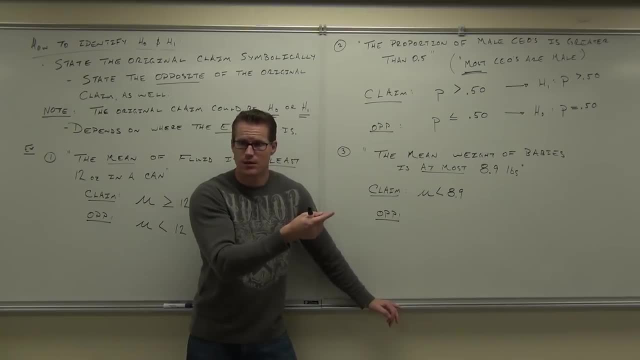 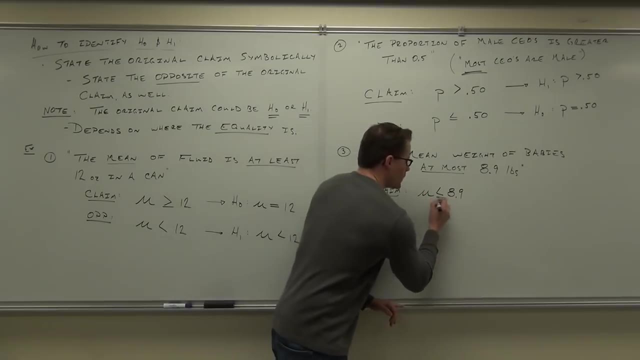 Now is there. it equals or not. That's the key. Yeah, If you have at most 9 dollars, you could add 9 dollars and be okay. right, If you have at most 8.9 lbs, it could be equal to. 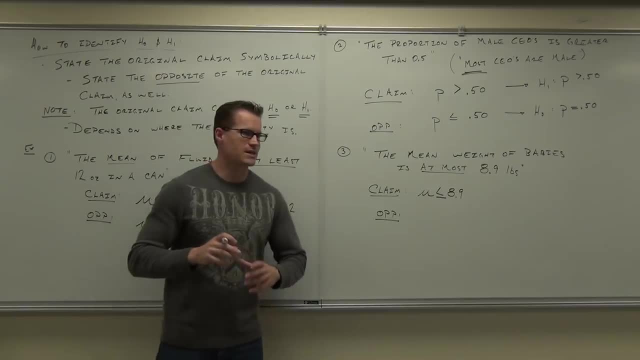 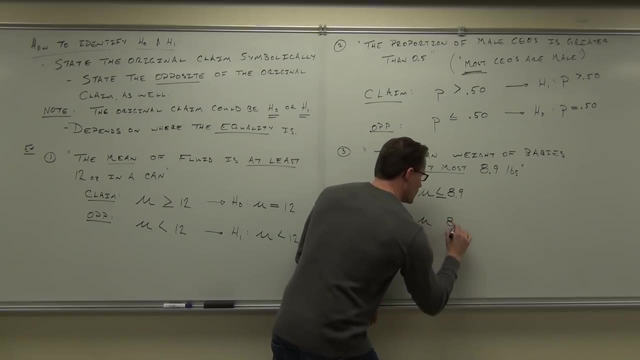 At most includes that inequality. That's important because that dictates what your h sub zero is and what your h sub one is. This is one of the most important steps you can do After that. state the opposite. What's the opposite of mu is less than or equal to 8.9?. 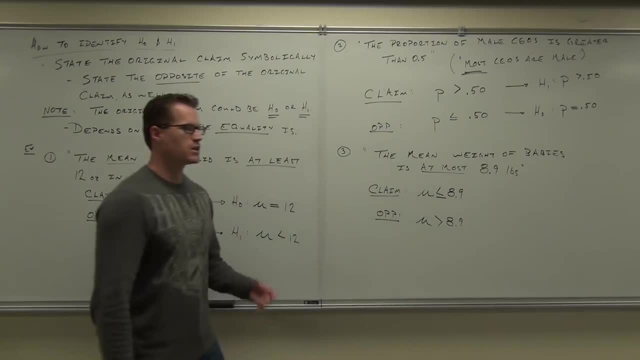 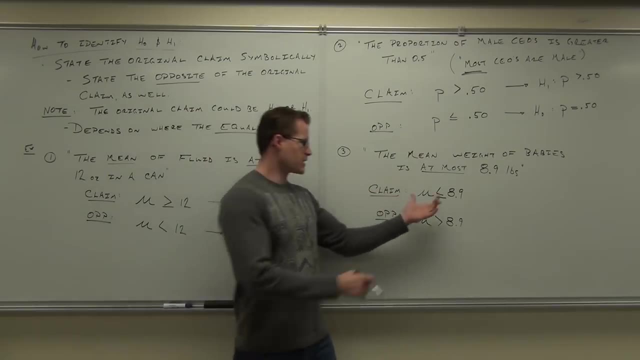 Greater than Strictly greater than You can't ever have an equals in two spots. Okay, which one is our? h sub zero, The claim or the opposite? Which one Claim? Yeah, because the equal sign is right there. We're going to say h sub zero. 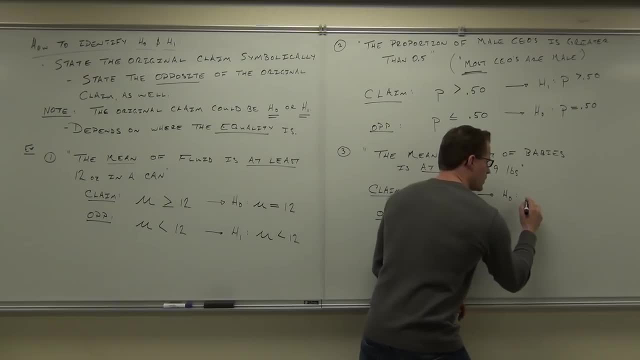 We'll just simply rewrite it. You're going to write What? Whatever the equality is, you omit that sign. You just put an equal sign, h sub one. we don't change anything about that. ever Mu is greater than 8.9.. 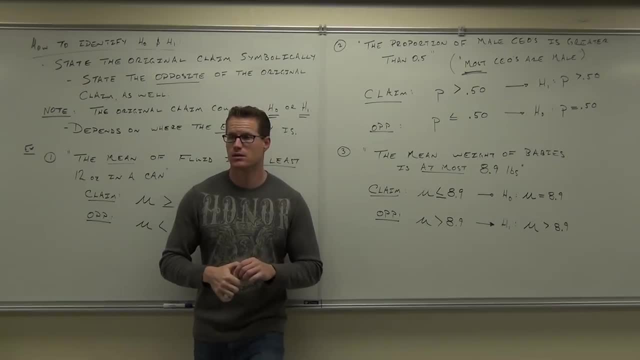 Tell me something. Would we be able to prove our claim correct in this case? Would we be able to, after we did all the work, prove our claim correct? I'm going to write h sub zero here. What do you think? Why Can you ever prove h sub zero, right? 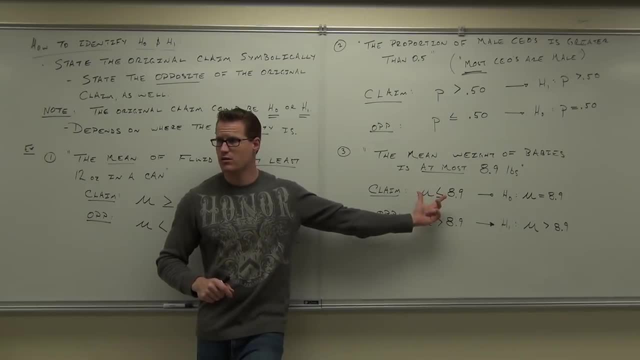 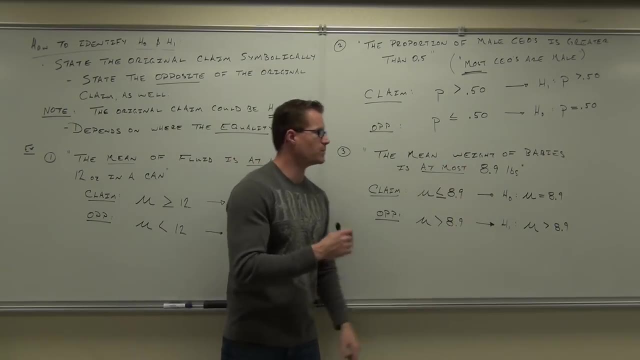 No, Our claim is stated as h sub zero. All you can do is prove that wrong. So you wouldn't be able to prove this claim ever. You can't prove right. You could prove it wrong, but that is not what you're trying to do. 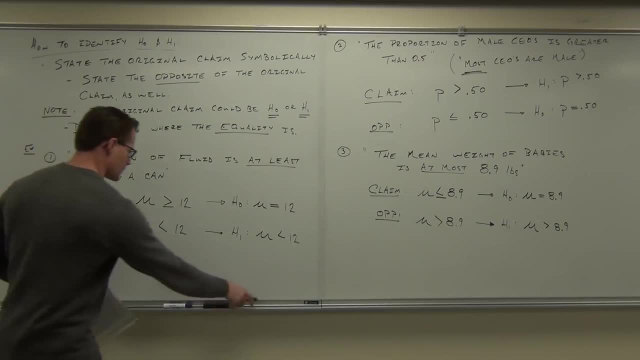 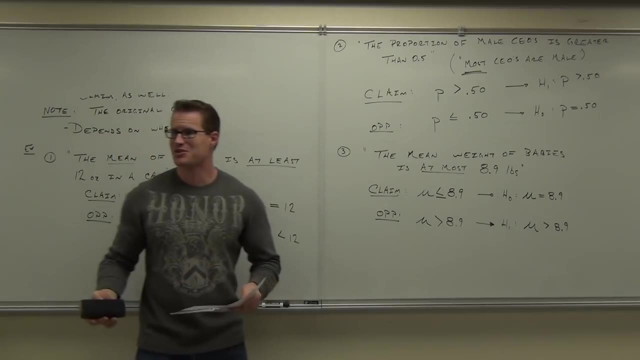 That's not what the statement asks. So when you get to doing this on your own, you better make sure you state it. So you get to doing this on your own, you better make sure you state it. You better state your claim is correct. right. 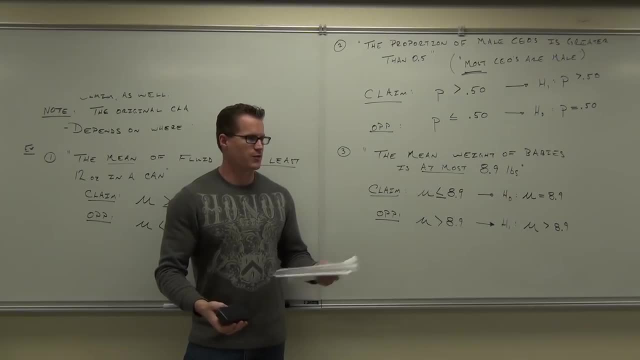 Now these claims are going to be given to you. You're not going to have to do that in your homework or your test, But when you get out to real life and you want to actually do this- which happens in a lot of jobs and a lot of fields- if you ever ask to do research on something, 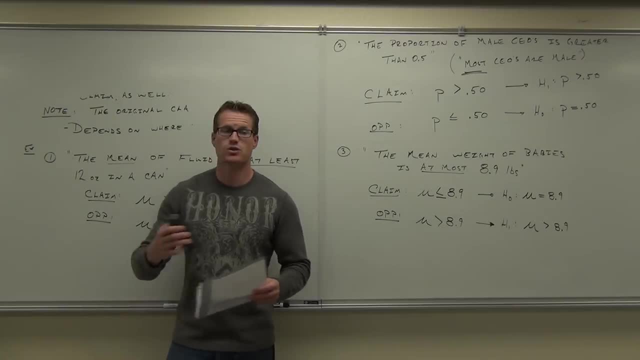 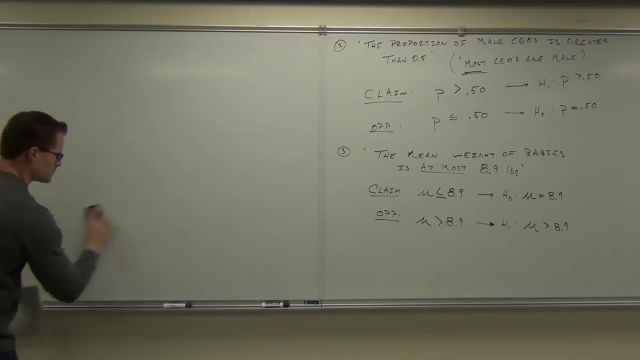 you are going to be doing statistics, because it deals with samples- You better state your claims correctly, Otherwise you're never going to be conclusive on it. That's not good, Okay, Last example, before we get on to something just a little bit different. 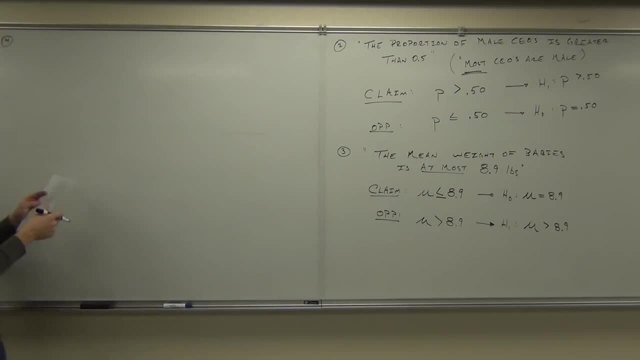 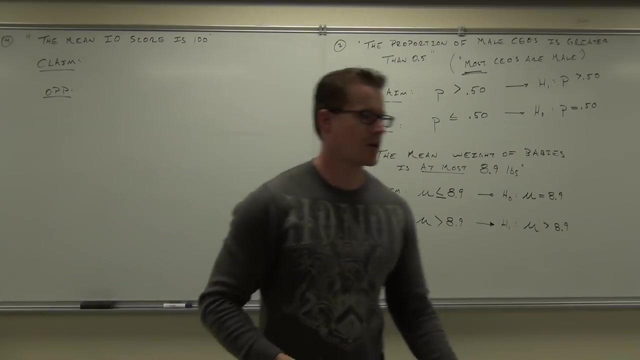 Our second step in hypothesis testing. So last one, I'm going to have you do this on your own, Piece by piece. First thing you're going to do is look for your claim, So I want you to identify on your own whether you're dealing with a proportion or a mean. 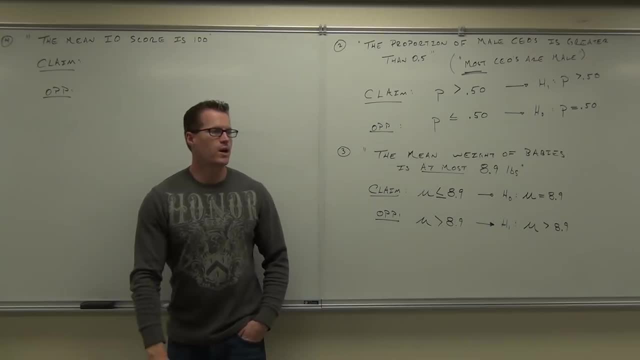 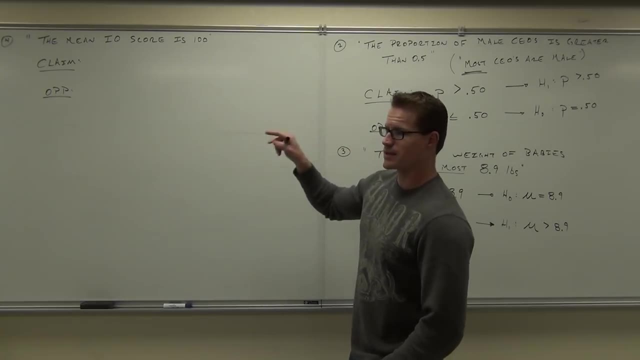 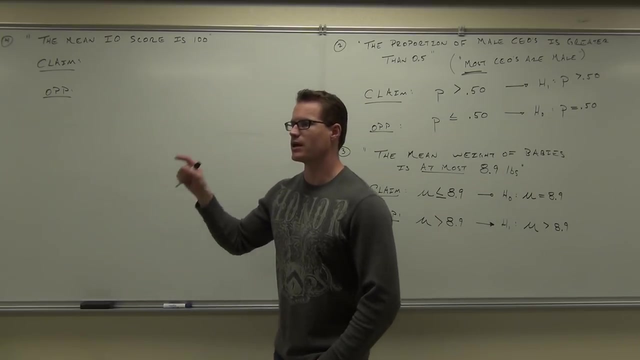 Usually it's pretty obvious what you're dealing with And write down the appropriate symbol. Now, with that statement, write down mean is equal to or greater than, or equal to or not, equal to or less than, or equal to or greater than or less than 100, because that's the value you're given. 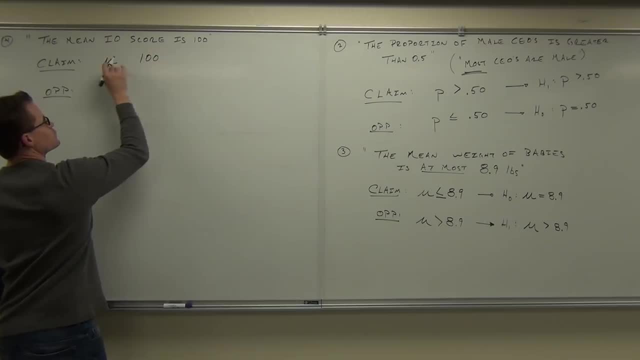 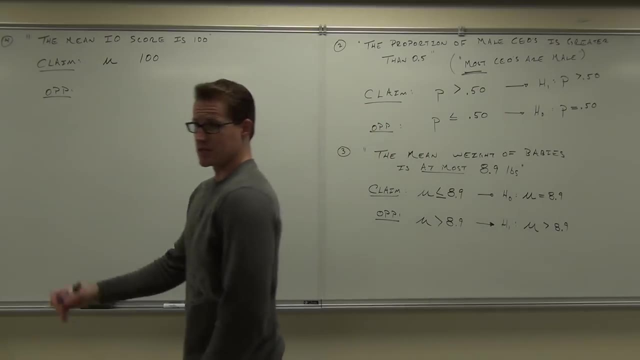 So you should have mean, and you should have 100, and you should have mean, And you should have some symbol between there. What symbol is it? Equals Is means equals. Sure, Now you've got to write the opposite of that statement. 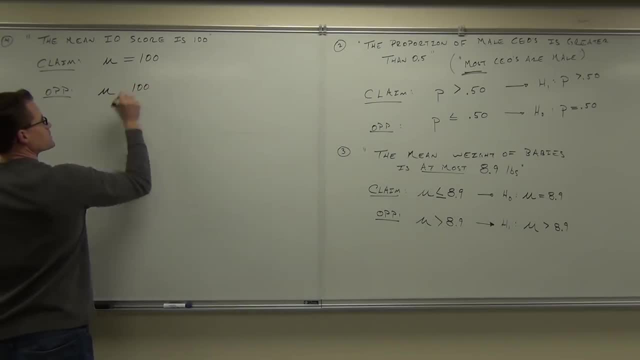 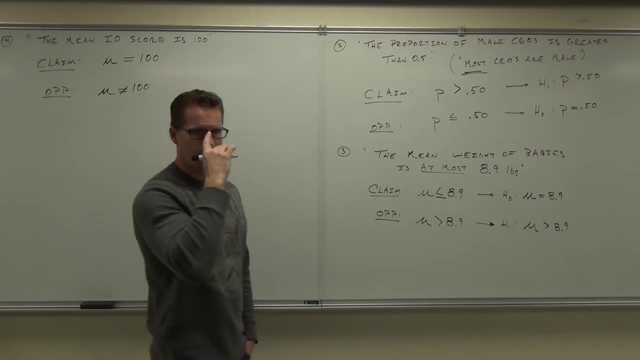 So you should still have the mu and the 100.. What's the opposite of equals One? One equals. Good, That's okay, We can have that. We can have that. What this means is actually probably the question that they should have asked. 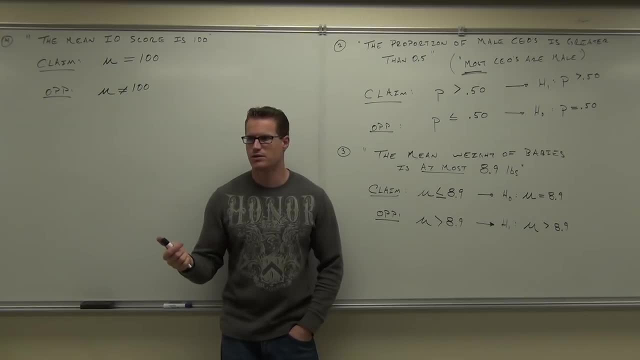 on the. The soda can one. They don't want it more than 12 ounces, or they don't want it less than 12 ounces, but they also don't want it more. right, They want it exactly equal to 12 ounces. 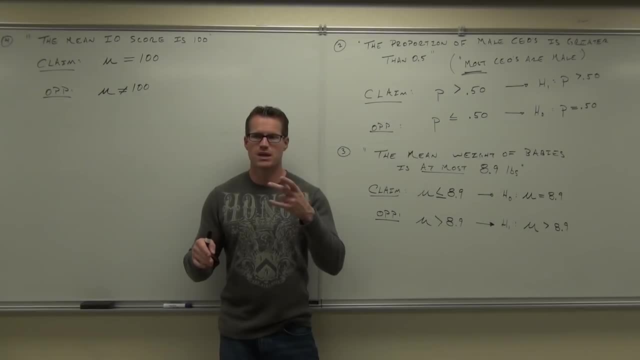 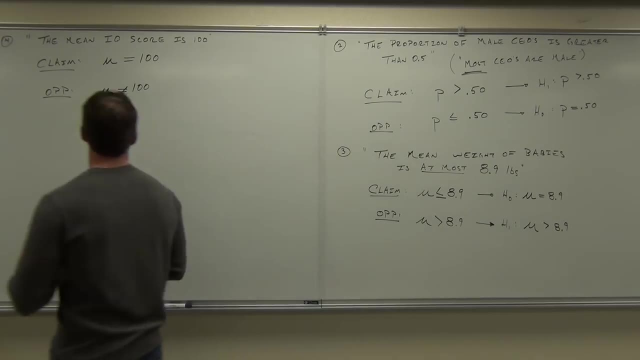 You'd probably test the claim. The claim would be: the mean volume of soda is not equal to 12 ounces. Then you could actually prove it right or wrong. Hey, which one of these is the H sub zero Claim? Do we have to rewrite anything? 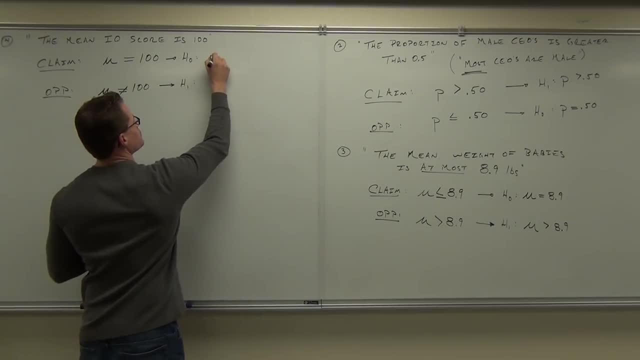 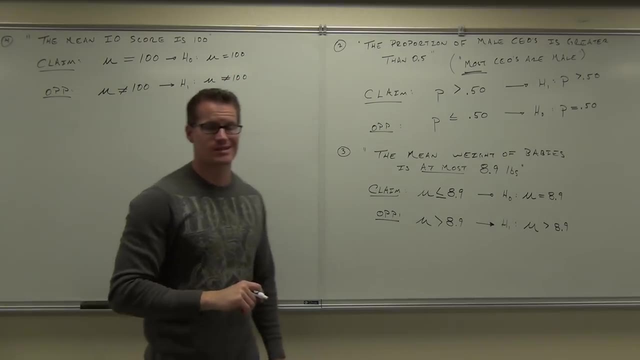 That's kind of nice right. We don't really have to change anything about this. We're just going to say the mu is equal to 100, mu is not equal to 100.. You'll notice that if H sub zero is stated as our claim. 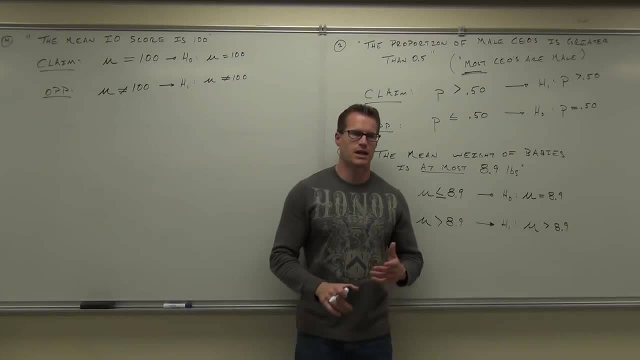 we also wouldn't be able to prove that one correct. You'd have to prove things Like the mean IQ score is not equal to 100, or the mean IQ score is greater than something or less than something. Those at most, those at least, those things aren't provable. 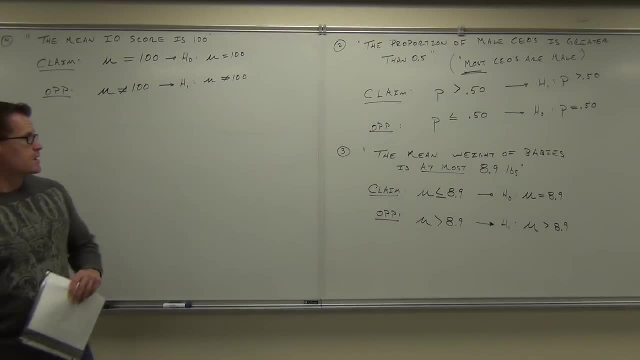 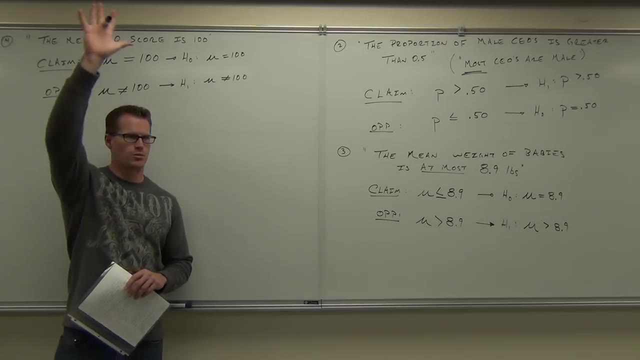 They include the equality. Not great for us. Okay, now we're going to move on to something. Do you feel okay with stating these claims the opposite and determining which one is H sub zero and H sub one? How many of you feel pretty good about that? 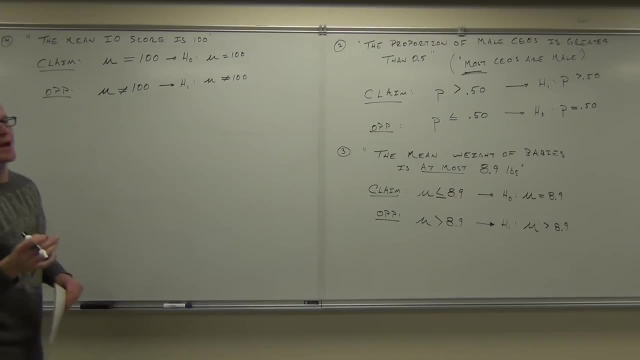 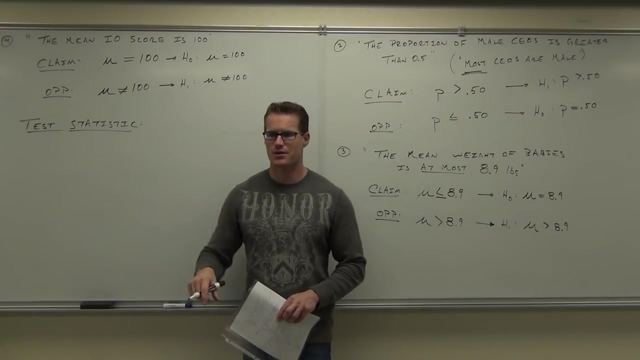 Good, okay, Good, The next thing you do after you do your claim. so this is step number one. no matter what, You do it exactly this way, You've got to find what's called the test statistic. The test statistic- hopefully the name implies- is what you use to test the hypothesis. 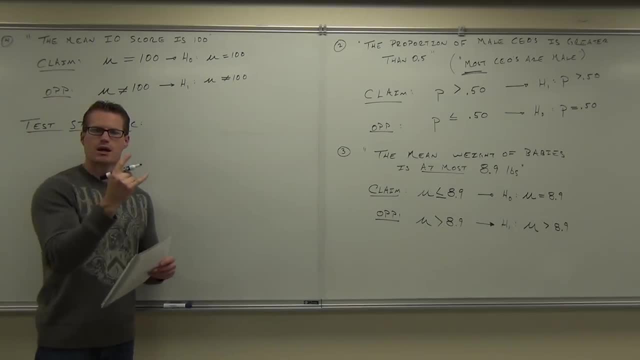 Now there's a couple. there's actually three we'll be dealing with. I'll give you two of them today, one of them later on when we get back to standard deviation. You have two different test statistics. One is for a proportion. 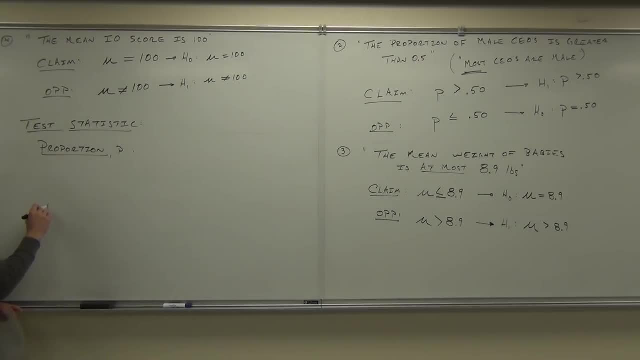 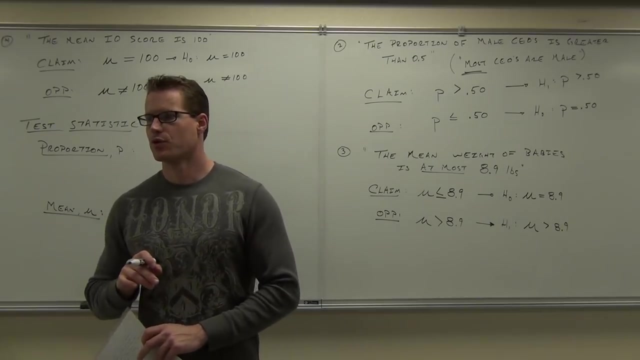 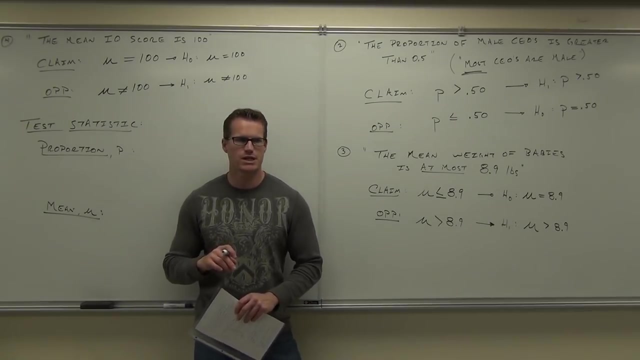 P, And one is for the mean mu, For the proportion, For the proportion. Oh, this is going to be great for you. Let's go back to your test, chapter seven, For proportions. did you have an option between Z or T, or was it all one of them? 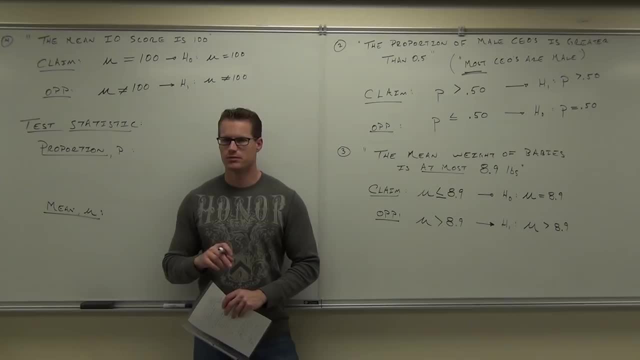 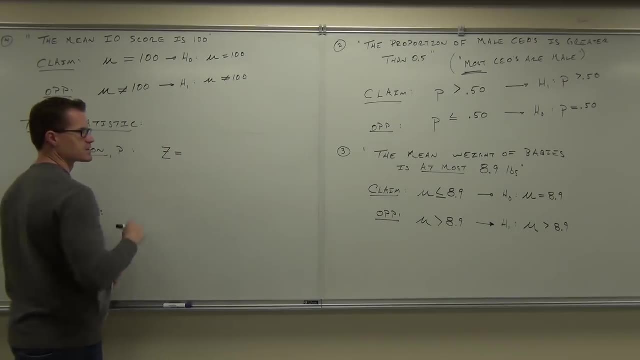 For proportions. Z. It was always Z for proportions. Do you remember that? Always Z For proportions? you're still going to have a Z test statistic Notice. please watch this on the board. Do you notice? there's no alpha over two. 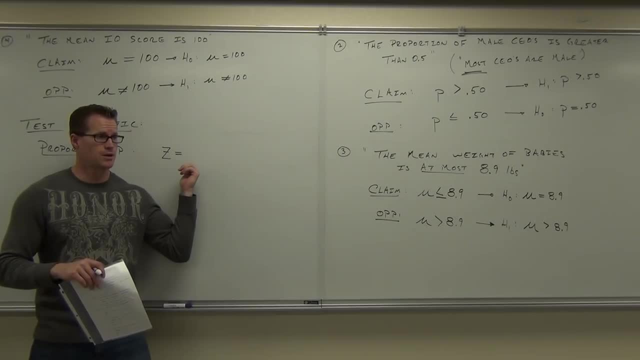 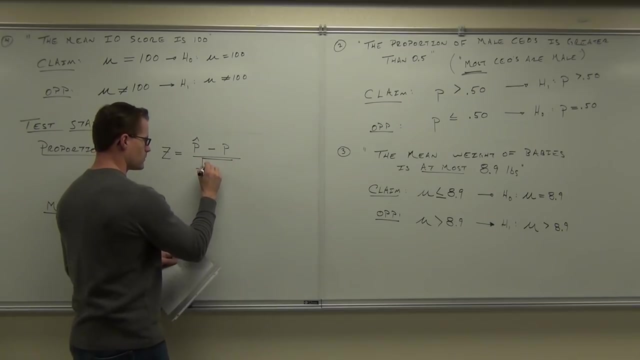 This is not a critical value. This is different. This is a test statistic. It is a typical Z score, like what you've done before. A typical Z score, like what you've done before, is a sample measure minus a population parameter over the standard deviation, over the square root of M, That's it. 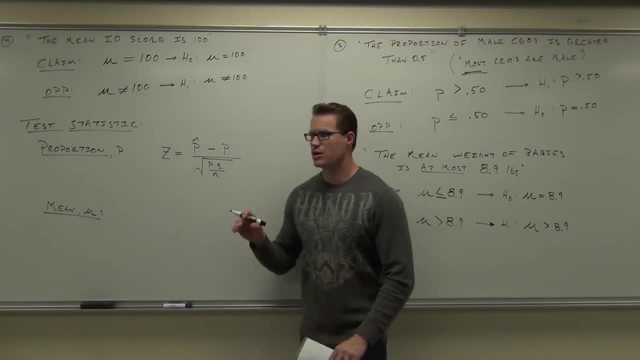 Okay, one big thing, One big big big thing here. Please note very carefully that this right here, that P and that Q. I want to make sure I double check this for you. Yeah, it's right on your table too. 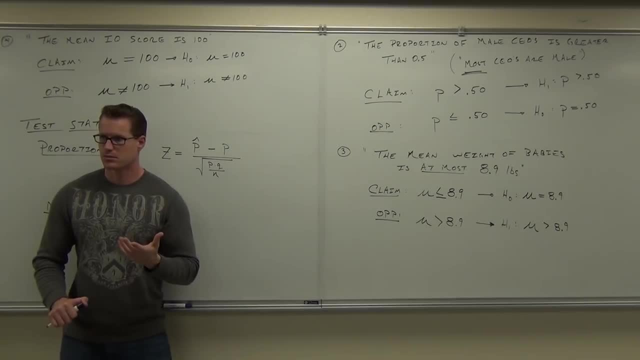 That P and that Q do those have a hat on them. So is this P the same as this P? Is this P the same as this P? Yes, these P's are the same. So this is going to come from your claim. 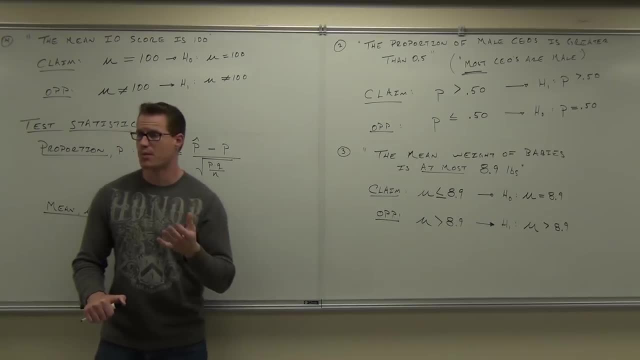 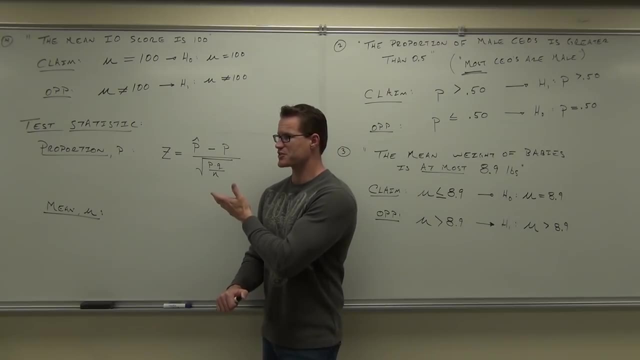 This right here is the only thing and this right here is the only thing that comes from your sample. is that information? You okay with this one? It's a Z score. It's just called test statistic. now, Now mean. we had two options for mean. 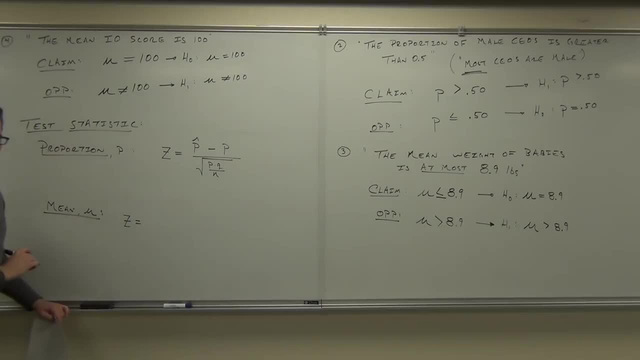 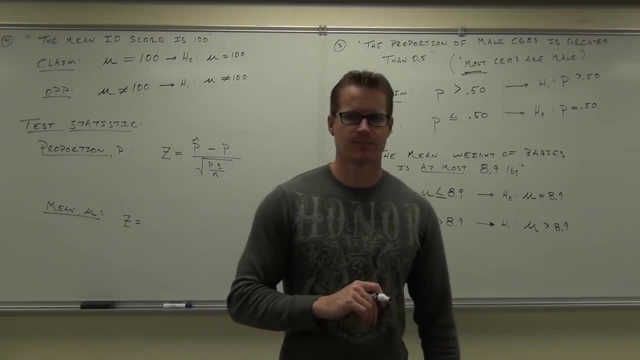 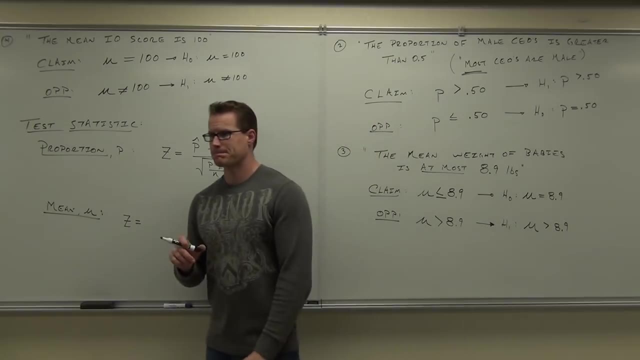 Z, Z, Z, Z, Z Z Z. When did you use a Z, folks? When did you use a Z? Well, clearly, four proportions. but when you talk about means, when did you use a Z? Oh, okay. 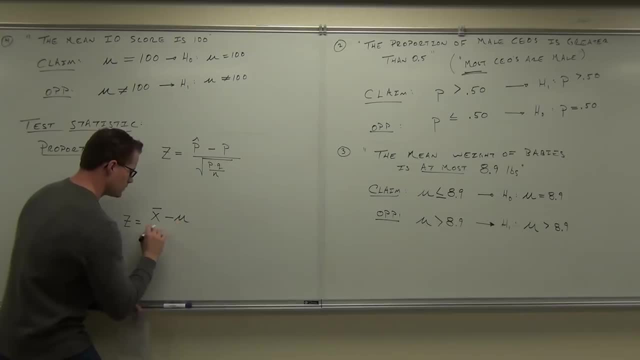 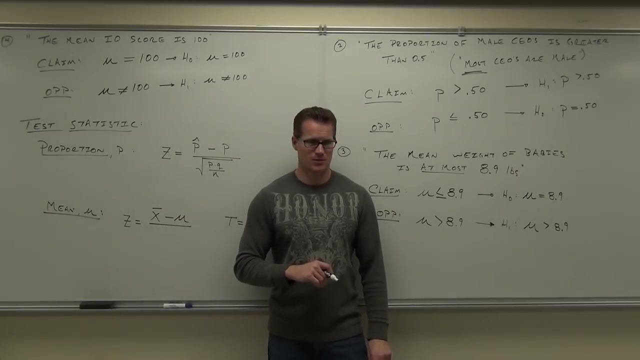 Go back and read chapter seven. When did you use a T? Was there a difference between Z and T? If you didn't know there was a difference between Z and T, why didn't you use it? Z and T? you've got fours on a lot of your problems. 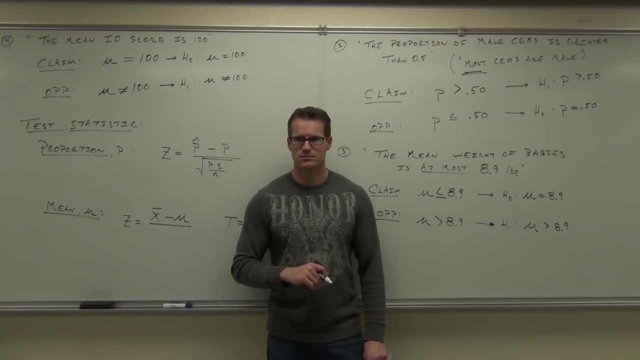 or zeros on your test. Sample, Sample. what Standard deviation, Standard deviation. It was all about the standard deviation. If you knew population standard deviation, you used Z. Yeah, that's great. If you didn't know population, you knew the sample. 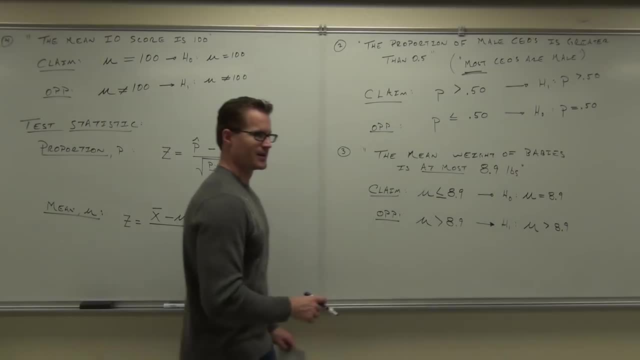 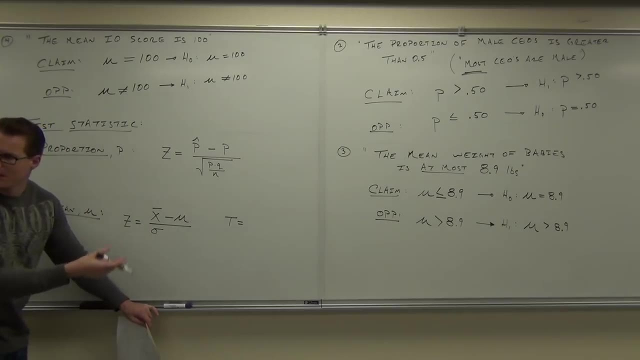 standard deviation and you used T If you didn't know that well, you used T Why? Because a Z-score's based on sigma. If you don't know sigma, how are you supposed to find Z? Does that look familiar to you? 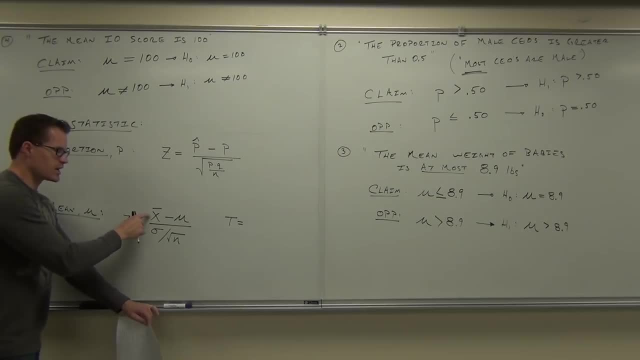 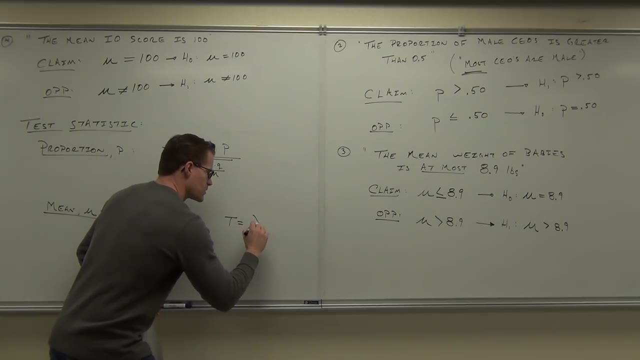 Geez, I hope so. Yeah, but you should've used that on your test, right. A Z-score is X-bar minus mean over. the square of sigma divided by the square root of N. T is very similar: X-bar minus mean over, but you don't know sigma. 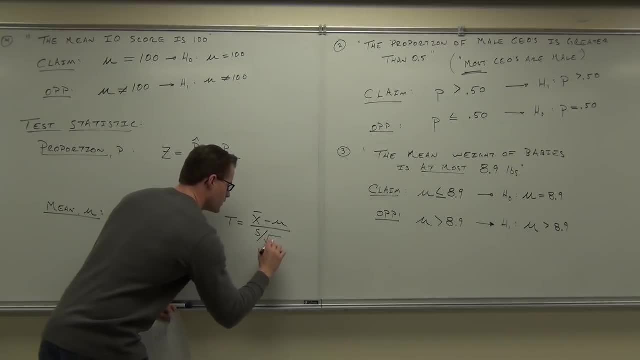 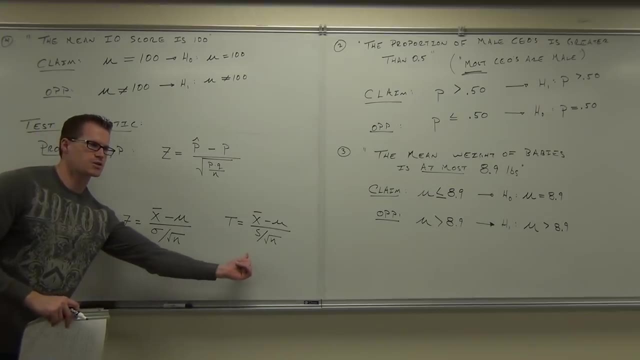 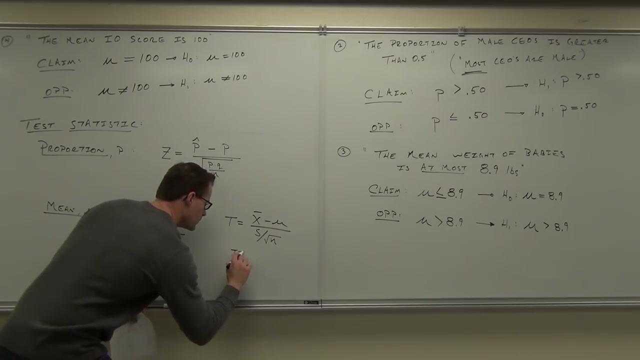 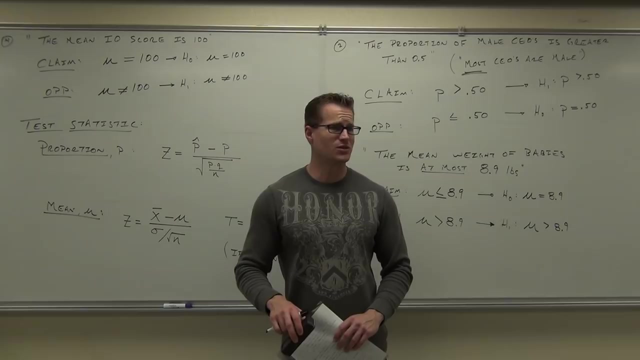 you only know S Over the square root of N. Remember that this happens when sigma is known. this happens when sigma is not known. that's a population standard deviation. Are you going to try to put a couple of these steps together? Yes, no. 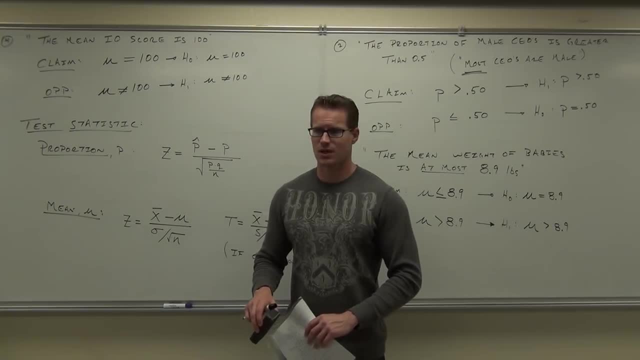 You okay with stating the claim right And the opposite. We haven't done it, We haven't done this yet, but well, we haven't done that yet. We've done this stuff before. We've done all that already. 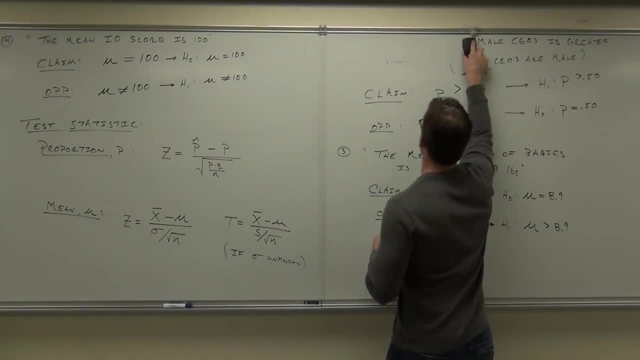 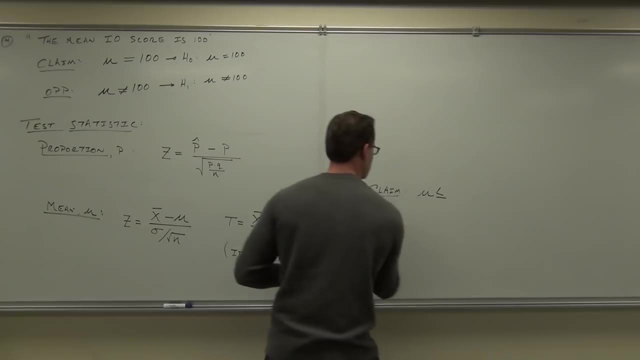 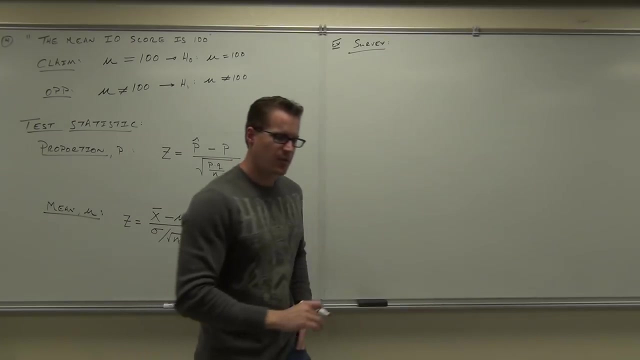 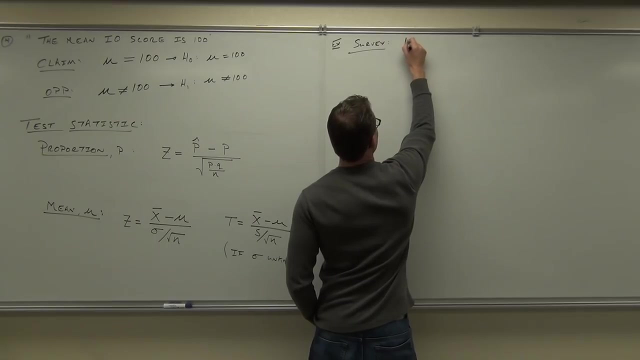 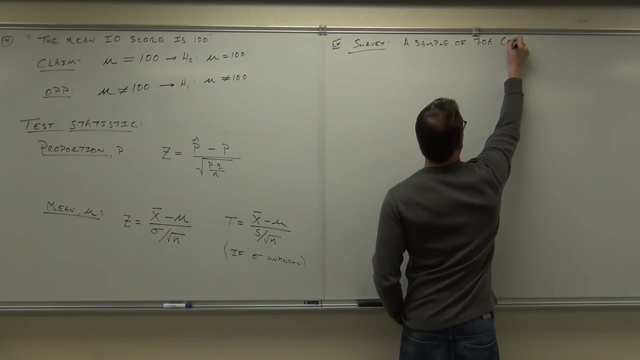 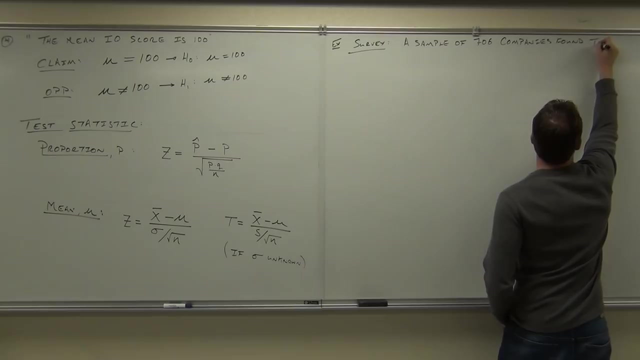 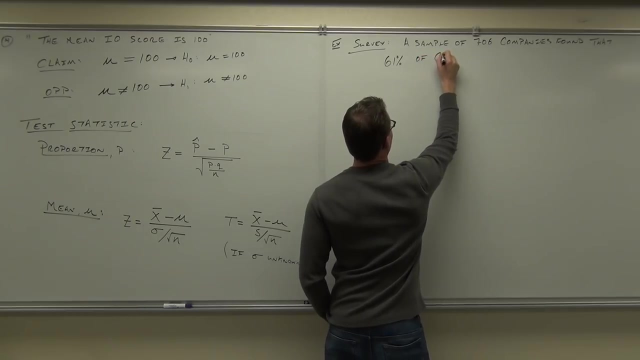 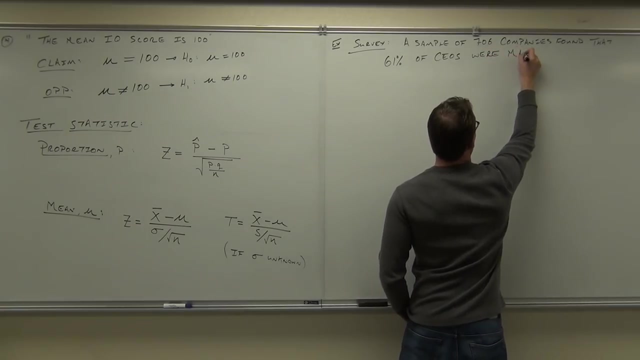 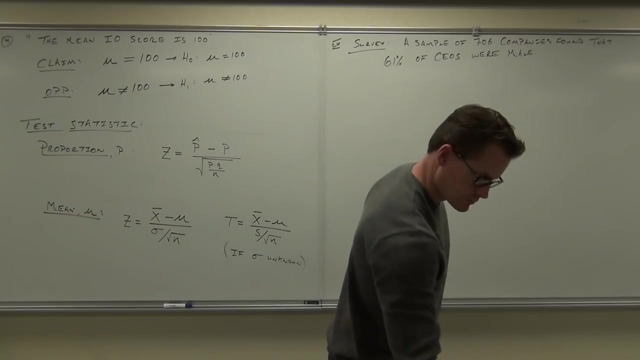 Now we're just tying together some loose ends, putting everything together. Here's a survey. Let's take a look at the. By the way, your homework problems and your test problems will all say something about a claim. You'll say, like test the claim that blah, blah, blah. 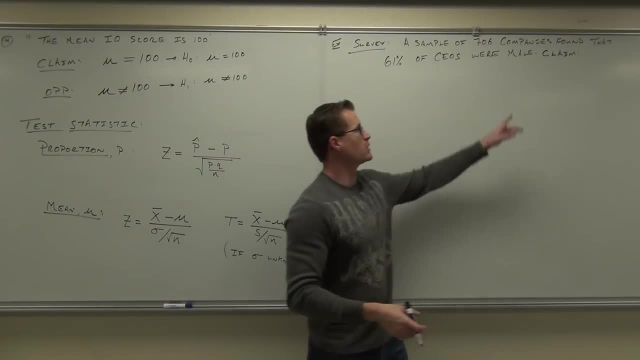 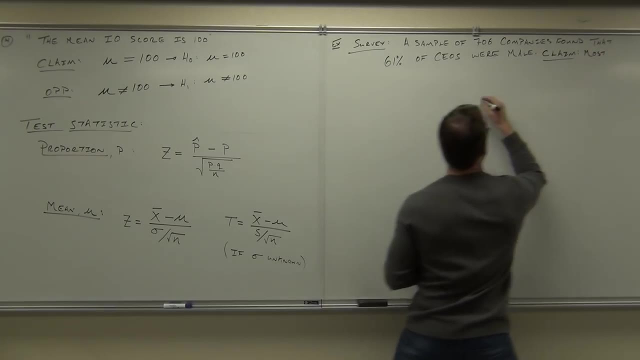 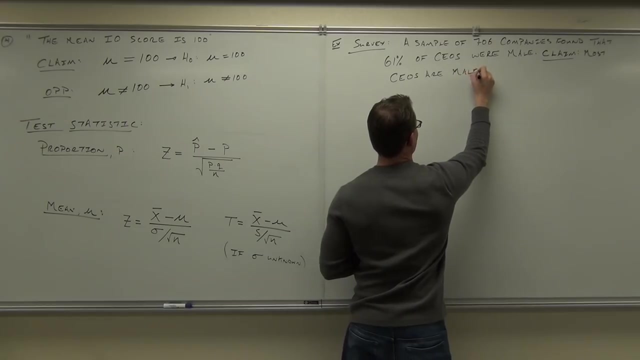 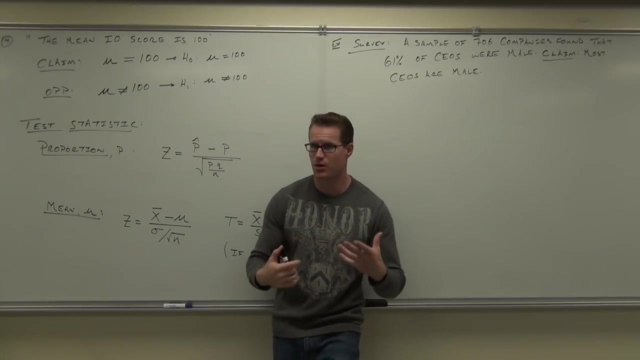 Or the claim is blah, blah, blah. It'll ask you to test some claim. I'm telling you. here's the claim: Most CEOs are male. Okay, now here's the idea for you. all right, We're getting more into the process of hypothesis testing. 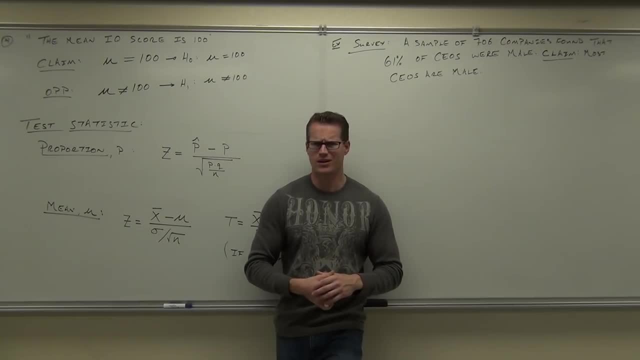 Here's the idea. You can't just look at that and go well clearly, I mean, the sample said 61 percent were male, So clearly most are male. Well, it was a sample. It was a fairly large sample. 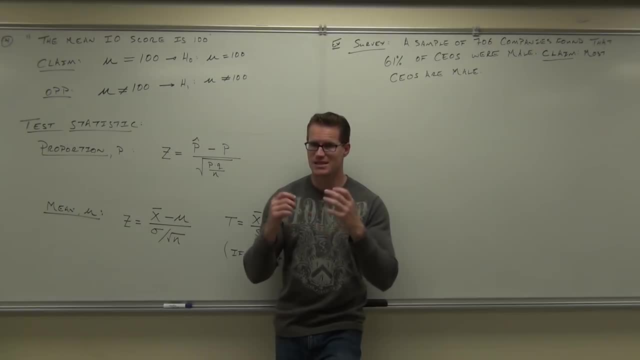 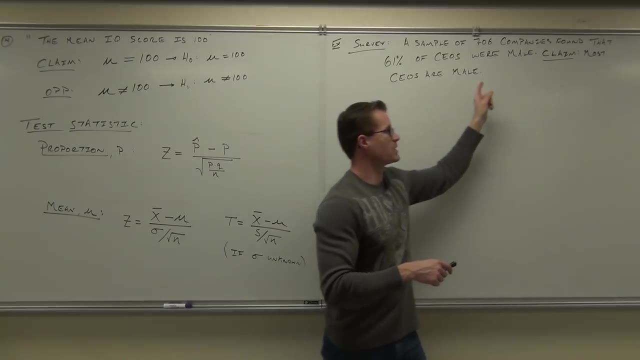 But is it different? The question is this for the hypothesis testing: Is it different enough from this, from this claim, or is it different enough from some statement to prove it right? That's the idea. Is it different enough? Is 61 percent big enough to say that most are male? 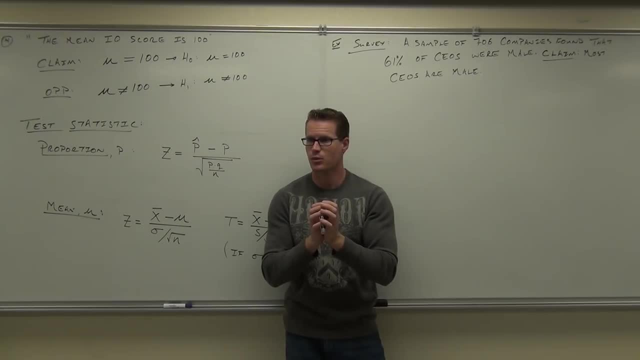 Would 52 percent be big enough? Would 51 percent be big enough? Would 55 percent be big enough? You don't know, do you? Because there's no way to just determine that, Because is a sample going to reflect perfectly a population? 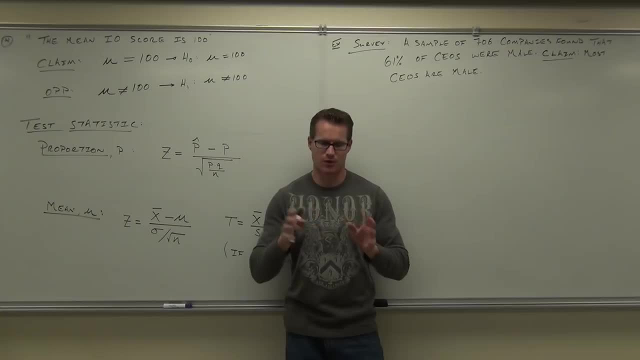 What do you think? You're a sample of the college, right? Do you reflect perfectly the college? Clearly not. No, not even close, right? We're not even a random sample. You're based on taking certain math courses to get here. 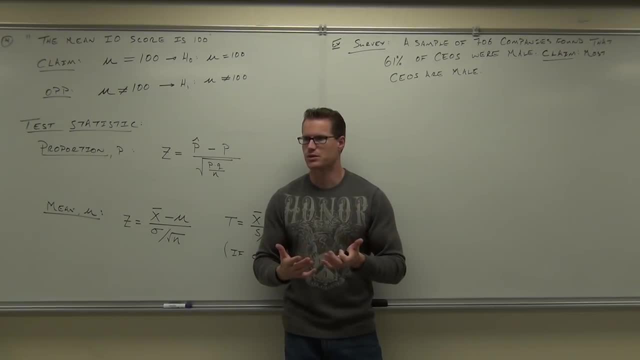 It's not random. You don't represent the college very well actually, But this sample might represent the population really well, But we're not sure how well are we? We don't know that. if they have 51 percent male, that's enough to say that most CEOs 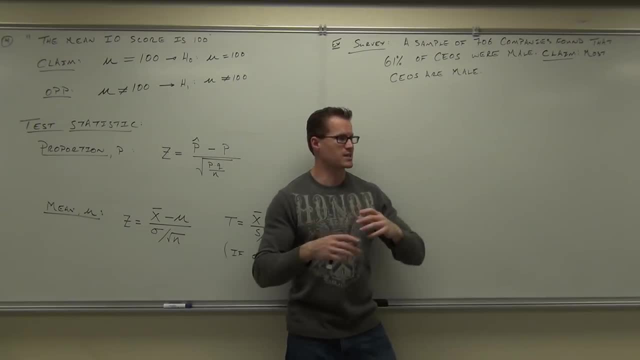 are male. Or if they had 52 percent male, that was a 52,, whether that says most are male Or 61,, is that big enough? We don't know. That's a process of hypothesis testing. You're going to see. 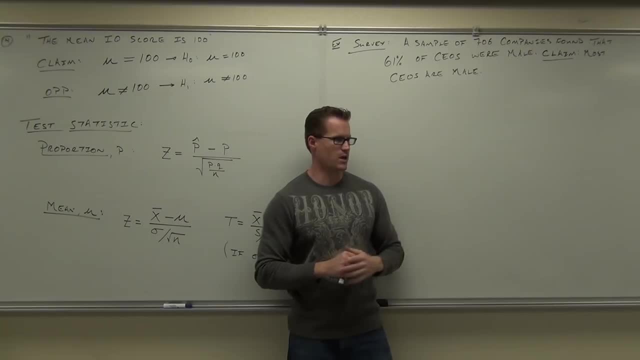 Is 61 percent, big enough to say that most CEOs are male. You're going to see. You're going to see How many people say that most CEOs are male. Do you get the idea? Are you starting to get the idea? I hope so. 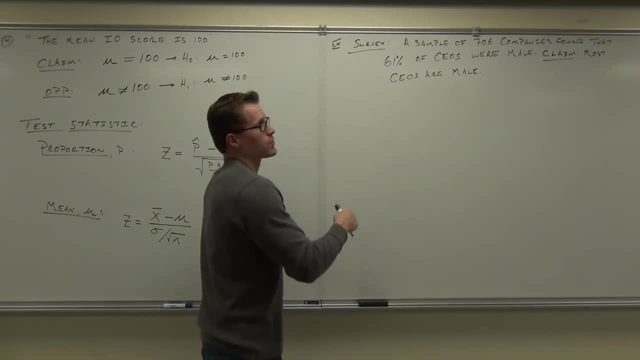 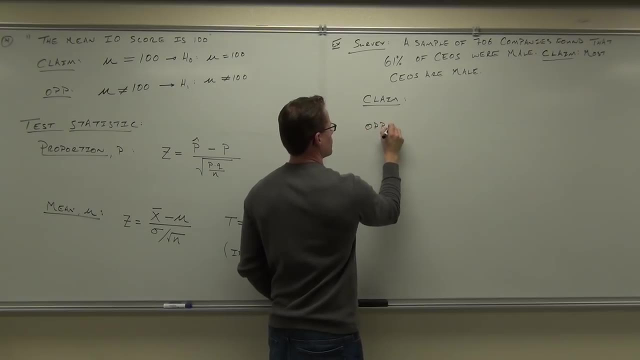 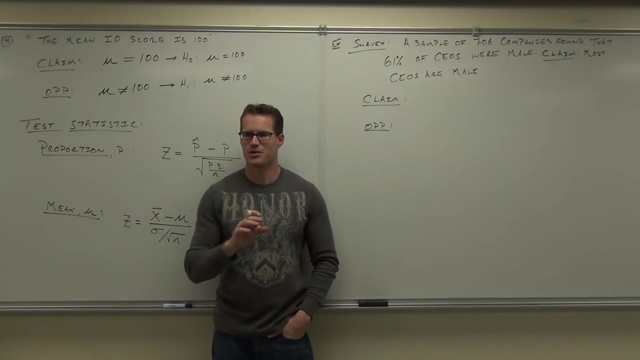 Well, we're going to go through at least the first two steps here. So claim Okay- don't get tricked up with all the fancy wording and stuff like that. Your claim is based on where it says claim, That's it. 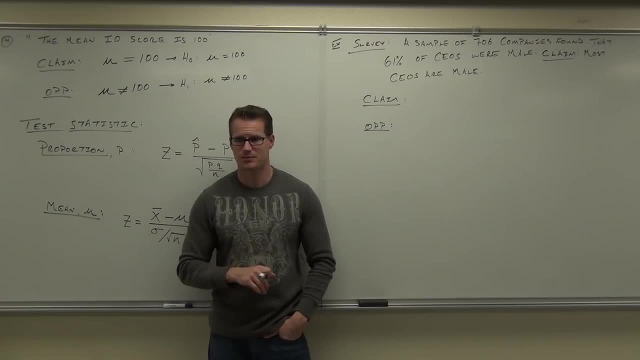 It's going to say claim somewhere or it's going to make a statement somewhere. test the claim that most CEOs are male. ladies and gentlemen, are you working with a proportion or a mean here? definitely proportion, absolutely right. so you're gonna put B. remember we're working with the claim: most of yours are male. so claim is P is what is. 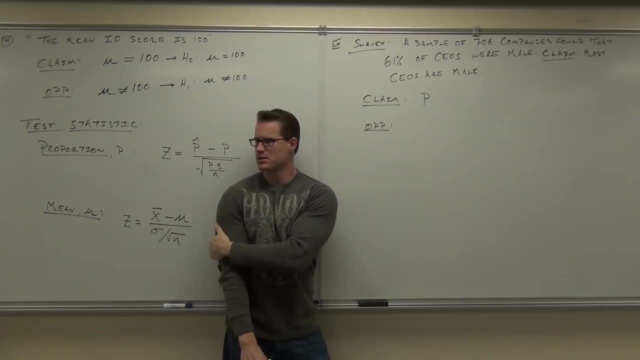 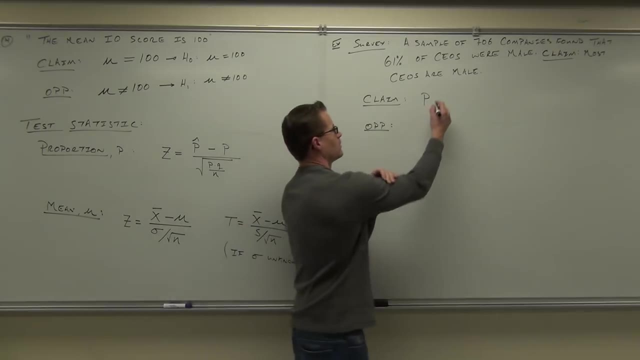 that greater than greater than equal to, equal to, not equal to less than lesser, equal to. what do you think? how would you state your claim most, most, most. what do you think if you have most the pie? do you have exactly half the pot? you have more than half the pie. what do you think? you all had pie, right. 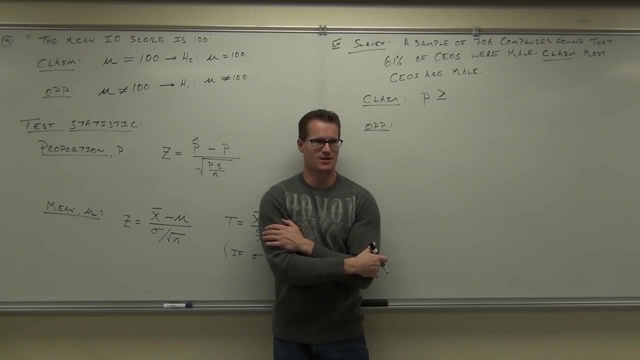 pumpkin pie is amazing on Thanksgiving. if you didn't, it's un-american. whatever you, if you have half, exactly half the pie, did you have most of the pie? no, you didn't have most, because someone else had half the pie. you had equal shares, didn't you? if you have most of the pie, you have like a little bit more than 50%. 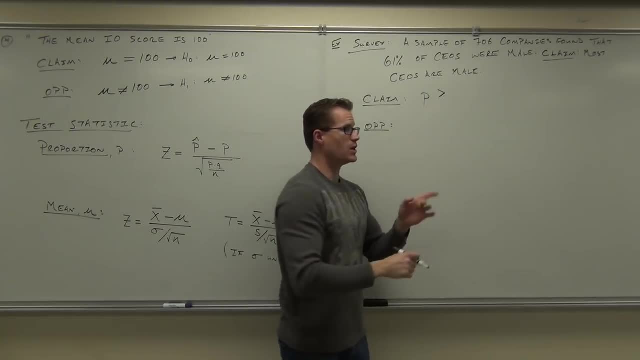 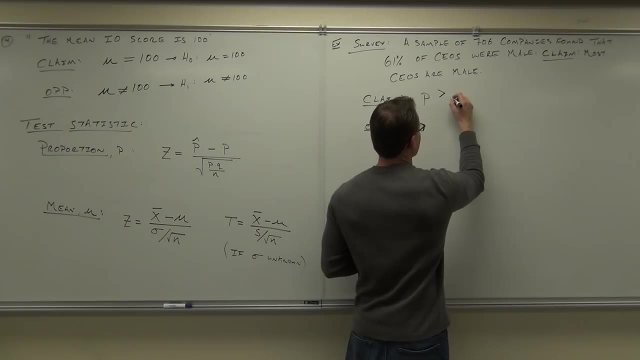 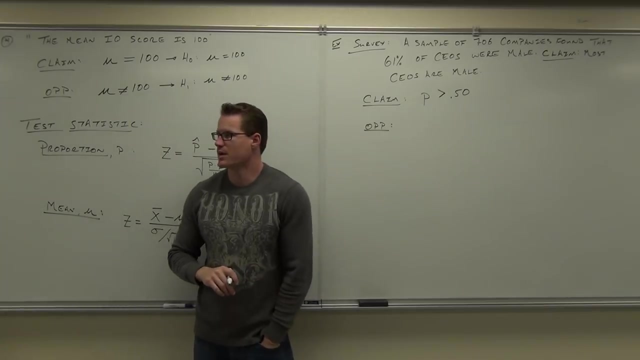 don't you? that's a little bit more than 50%. you need to know that most means more than you have to know that you got that most is more than 50%. that says most CEOs are male. more than 50% of the CEOs are male. you are you clear on that? now why don't I? 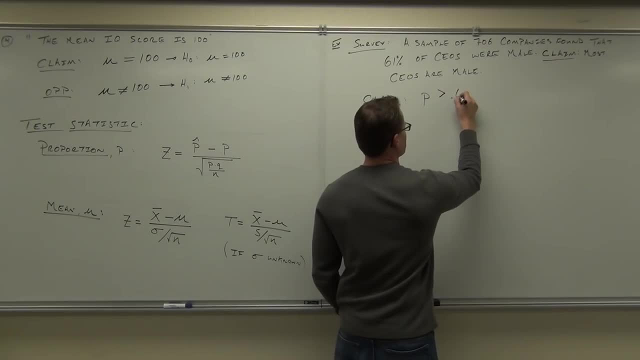 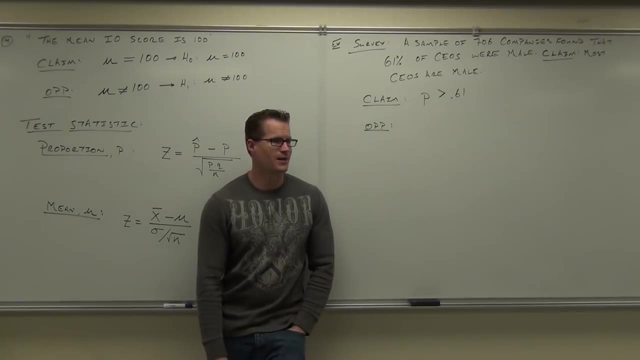 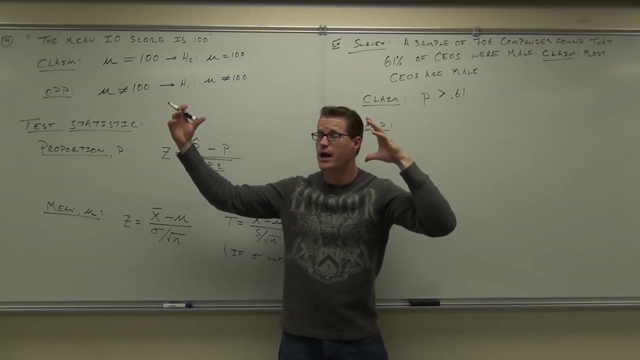 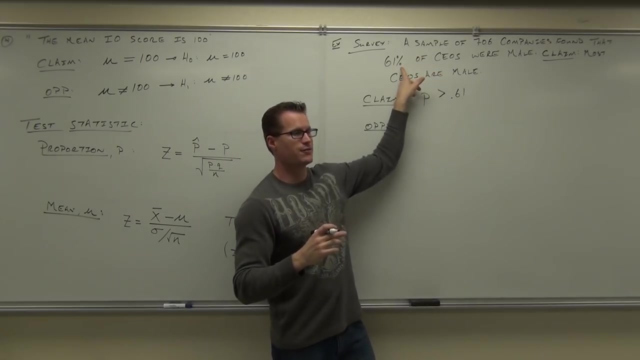 have this. I don't have that. does that have to do with my claim? no, look at the difference. the claim is based on a population right. we're trying to say a general statement about an entire group of american companies that says most are male. this right here. that's our evidence. 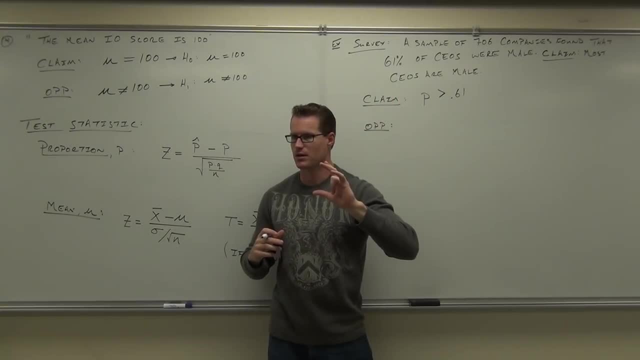 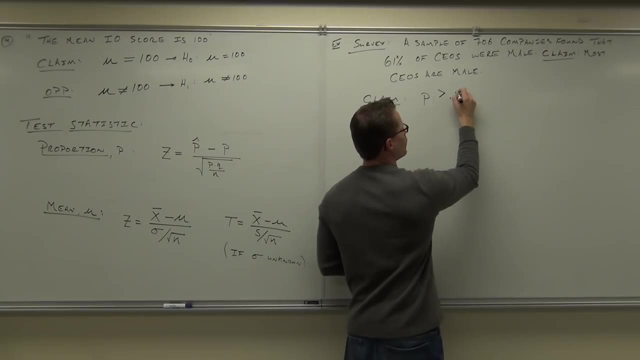 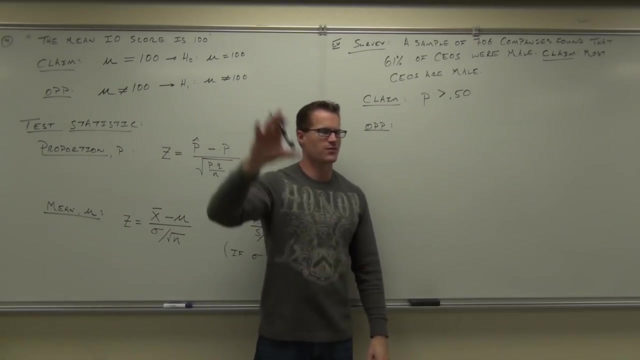 that to confirm or deny our claim. You with me? That's the idea. So the 61% that will come in later, but not now. Right now, I have only my claim. That's all I'm worried about. The proportion is greater than 50% or 0.50.. Raise your hand if you feel. 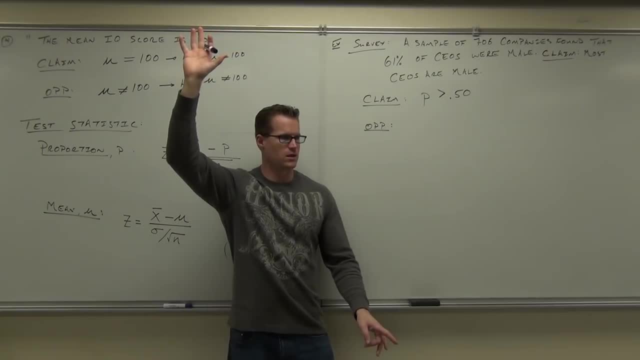 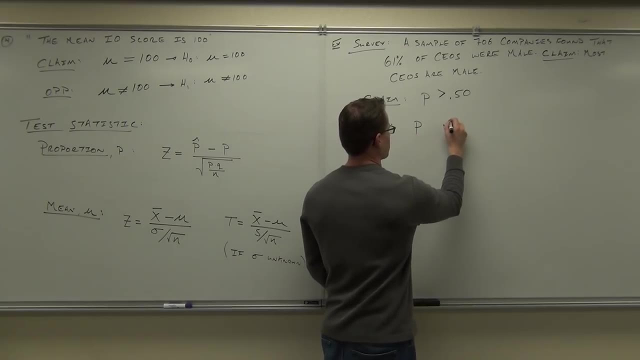 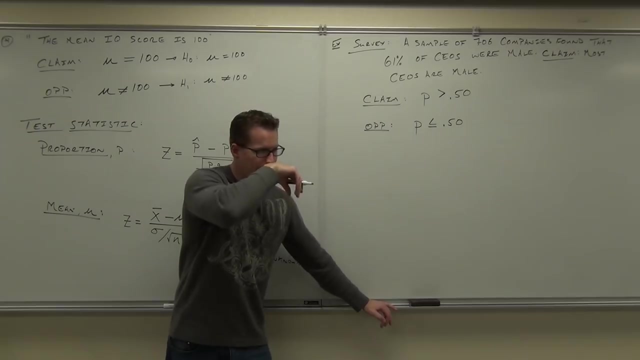 okay with that so far. Yes, no, yes, okay. State the opposite, Go ahead. The opposite is going to be less than or equal to. Got to have an equality somewhere. Did you catch the equals to Which one is my H sub 0, the claim with opposite right. 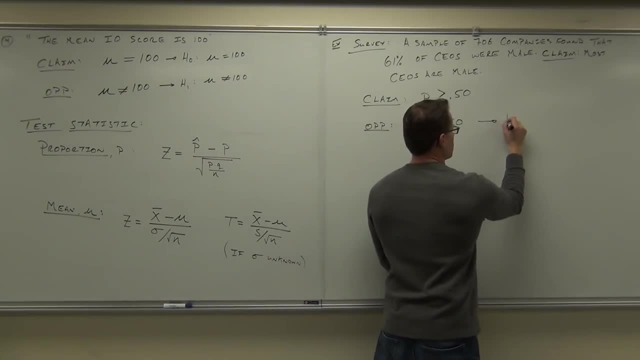 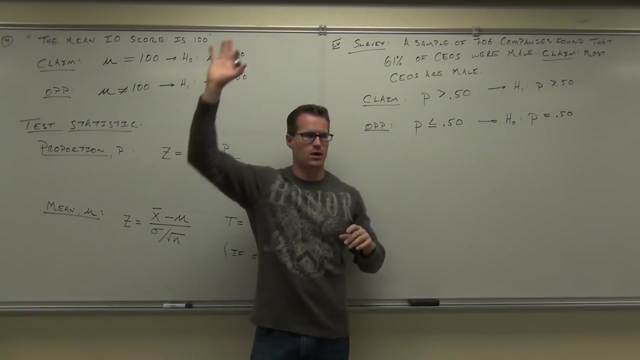 now, Good, And do you use the symbol again? No, What do you use? Okay, this is old news. now We've done this five times. Some people feel okay with doing that. You need to know most, right. You need to know what most means. The proportion means. 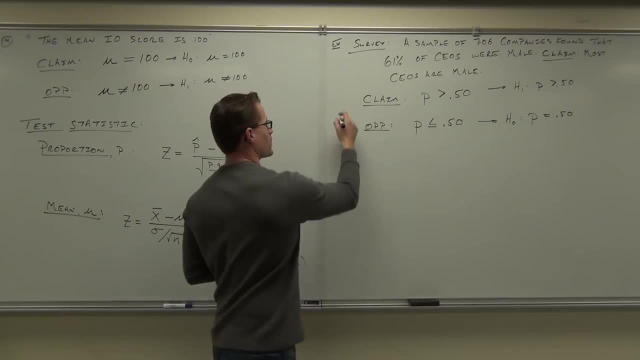 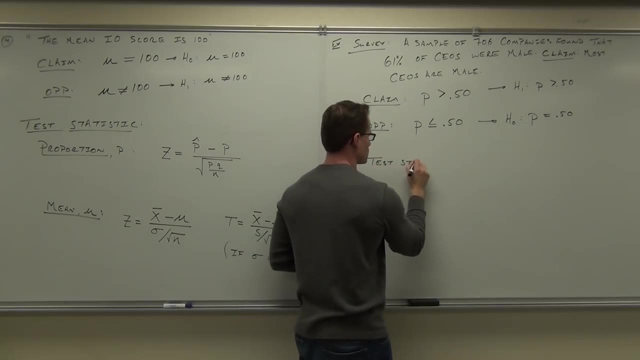 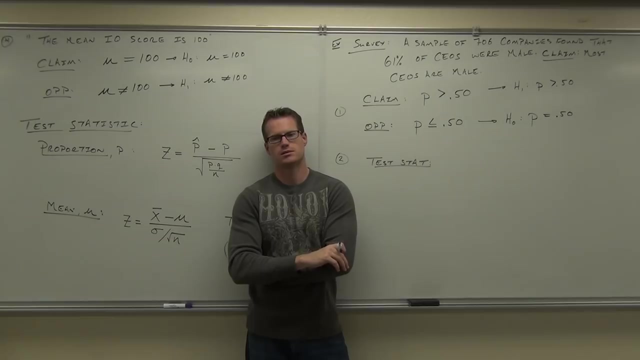 more than 50%. Now the next thing we're going to do is the. this is step number one. Next thing we do is the test statistic. Will we be using a Z score or a T score, and why Z score? yeah, absolutely. Why a Z score? Why a Z test statistic? 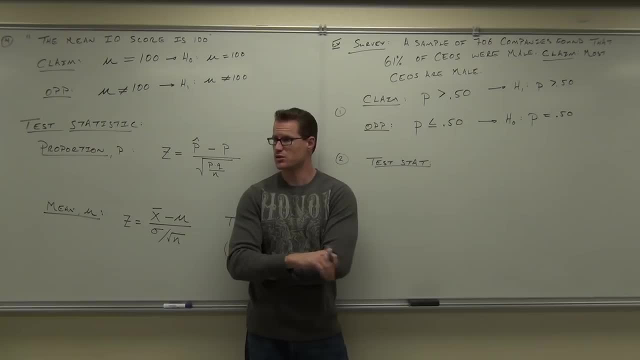 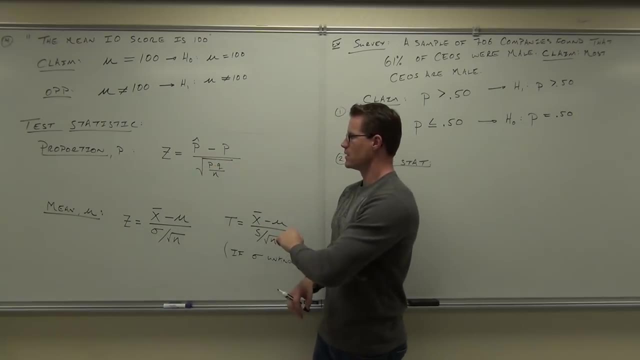 Yeah, proportions. That's the only one we've got for proportions. right, There was no T over here, So let's look at the letters that we need to know. for Z, We've got an O, P hat. Hey, look at the problem. Can you identify a P hat? P hat was a sample proportion Did. 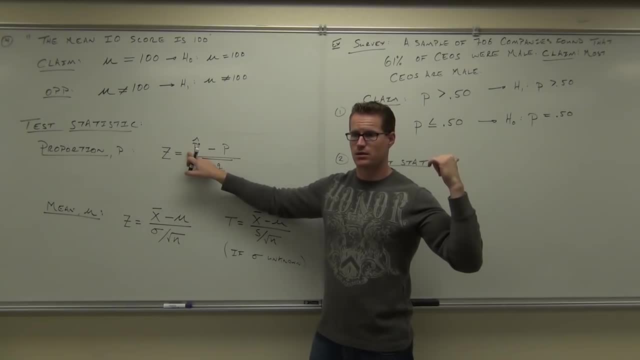 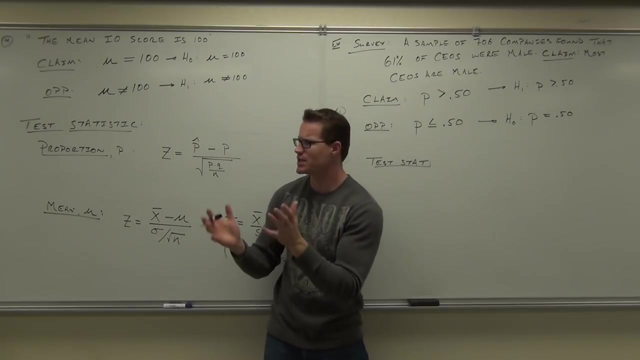 that. give you a sample proportion. What was it? 61% or 61.. Do we have a P now? Does it say: this is why we do this? You probably were thinking: why do we put the equals to? Why do we put the equals to? Where's the equals to coming? 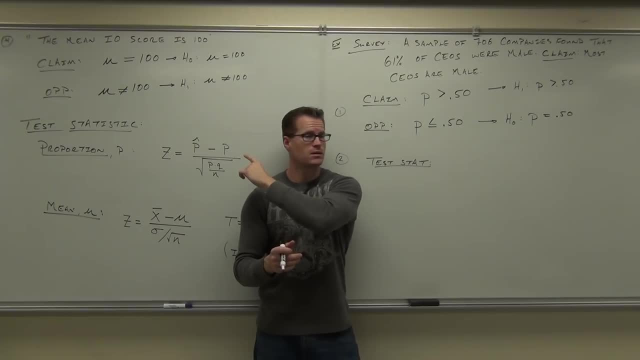 Does it say P equals something? up there right now. No, Yes, it does. Oh, okay, Up there right now. Yeah, It says P. I know, I saw it, I wrote it, I wrote that on the book. Does it say P equals? 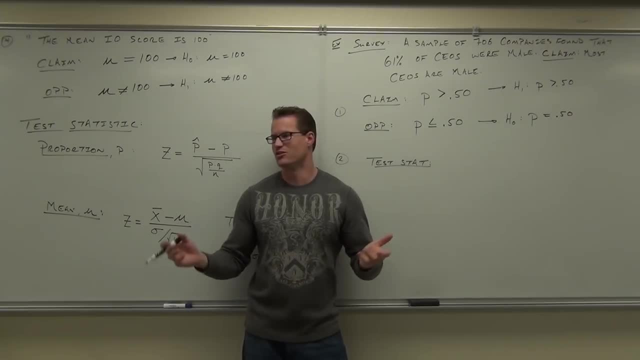 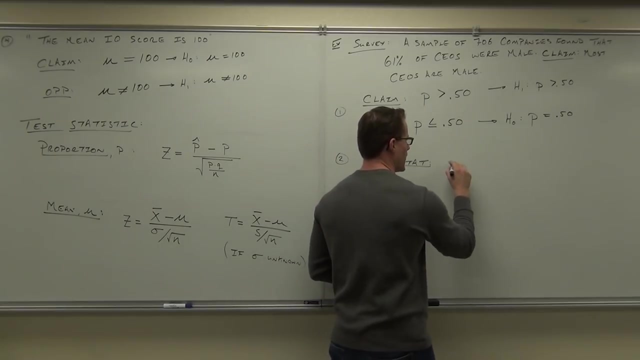 to Yeah, What's P equal to 2.. That's why you put the equals to: Do you get it? now, That gives you P. Could you find Q? Yeah, and do you know N? Very good, So list those things up. P hat, in our case, is .61.. We know that because 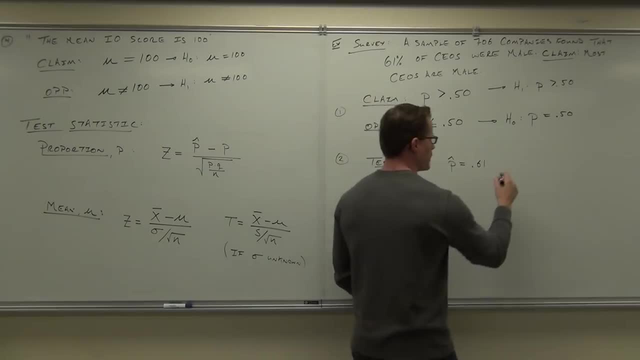 it said from a sample. P hat means from a sample. It's a sample proportion. P comes from your H sub zero. P comes from your H sub zero. That's right in front of us. It's right there. If your P is 50% or 0.50,, what's your Q? 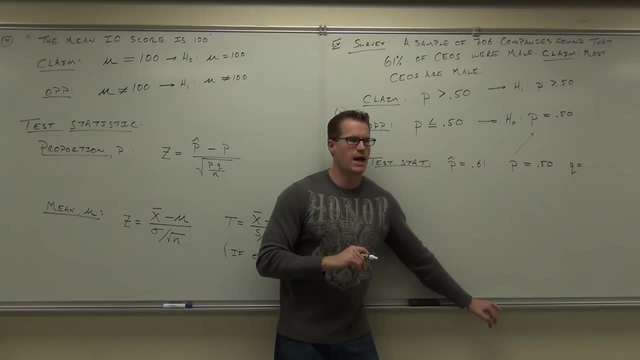 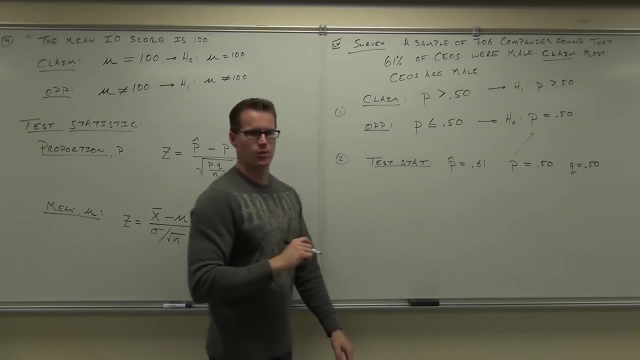 Is it 0.39?? Is it coming from your P? hat? No, these two things work together. Do you remember how to find your Q from your P? Take that 1 minus And last thing we need to know is just our N. 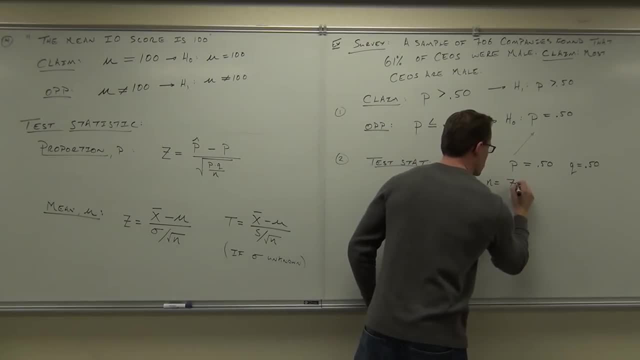 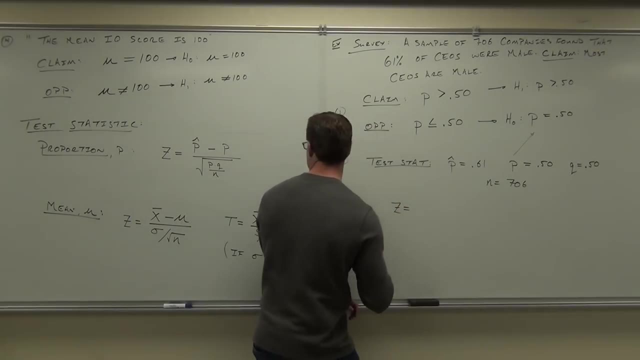 Our N is our sample size. In this case, it's what? Now you're going to go ahead and find your test statistic. It's a Z score. It's a Z test statistic. So you get your 0.61 minus 0.50 all divided by it. 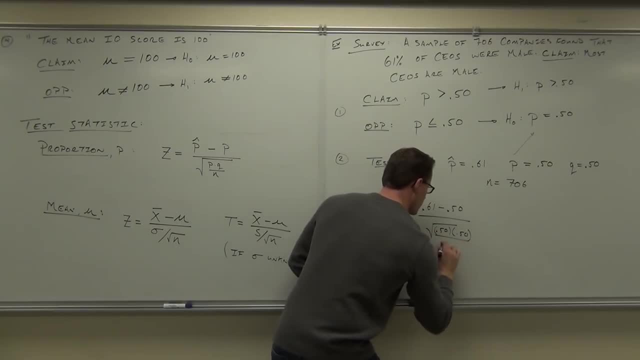 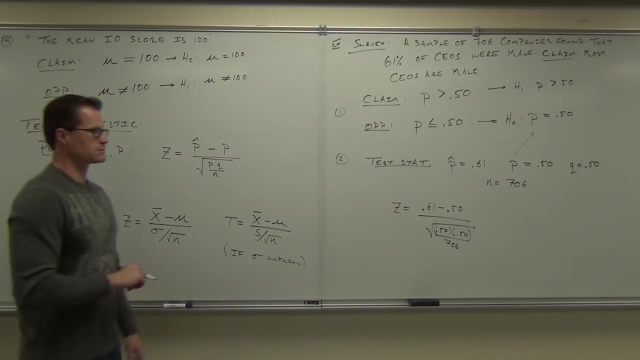 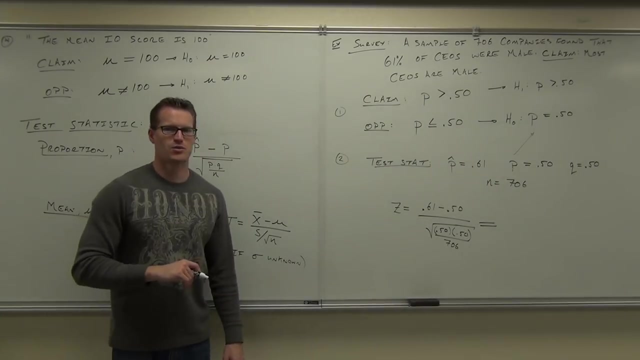 0.50 goes there, 0.50 goes here, Divided by 706.. You take the square root. after that I hear the rustle of calculators. It makes me happy. The top number you should do first. 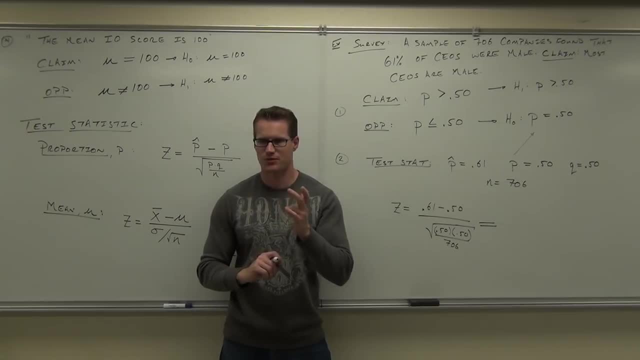 Do that operation. Do 0.61 minus 0.50 because you won't have to round it very much. It's not a big operation. You're going to get 0.11.. Did you get 0.11?? I hope so. 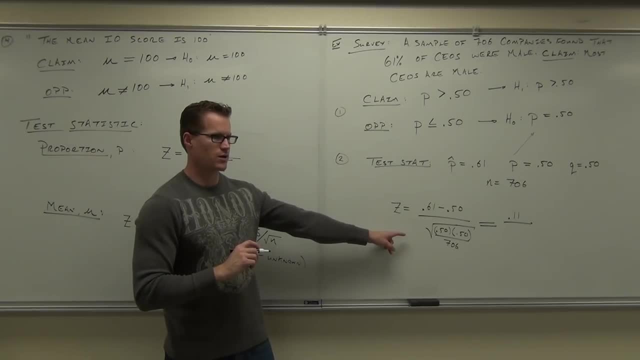 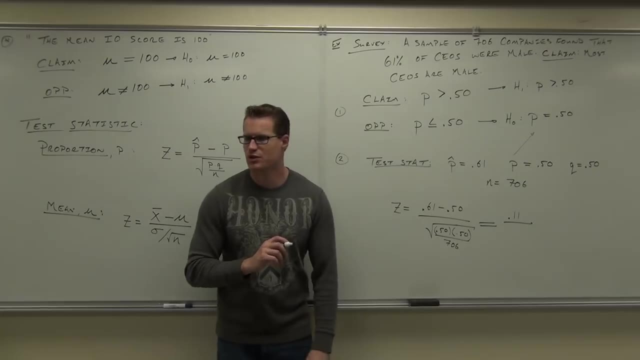 Now the bottom one. Do this on your calculator, like I tell you. You ready, Don't round anything. Take 0.50 times 0.50, press enter. You're going to get 0.25, yeah, Divide by 706, press enter. 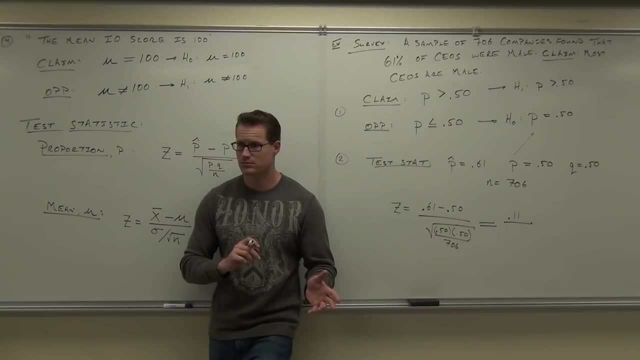 I have no idea what you're going to get, but it's going to be small. That's why you don't round. Do you have something like 0.00 stuff? Okay, Now take a square root of that. All you got to do is press square root and then press answer. 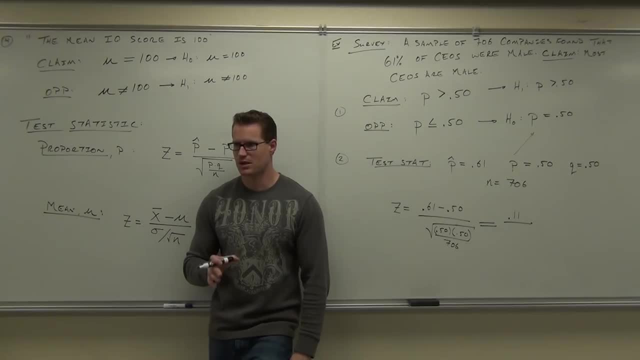 Wherever your answer button is. Usually you have to press a second or a shift button to get there. Press enter. Did I give you something like that? Now press 0.11 divided by answer. It will give you five point something. 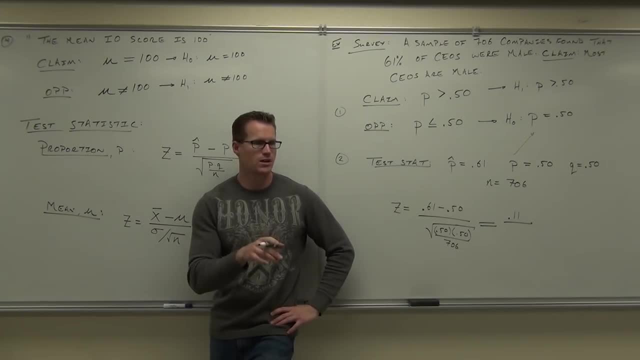 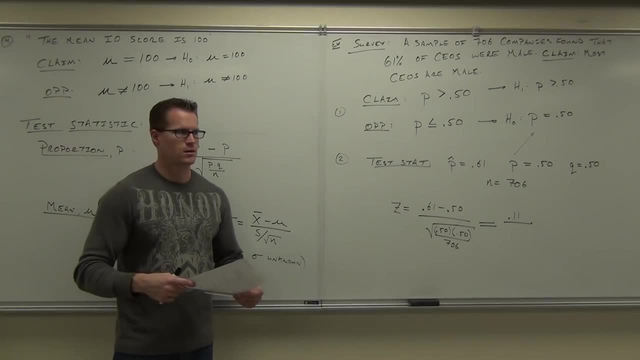 5.8.. 5.8.. 5.8., 5.8.. Did you get 5.83?, 5.84.. 5.84?? Oh, my math is wrong. Five point, so this is same stuff. 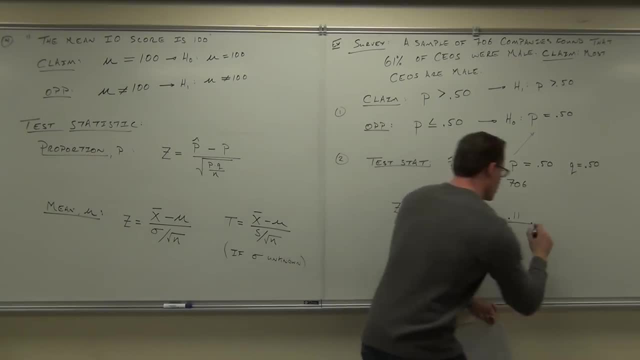 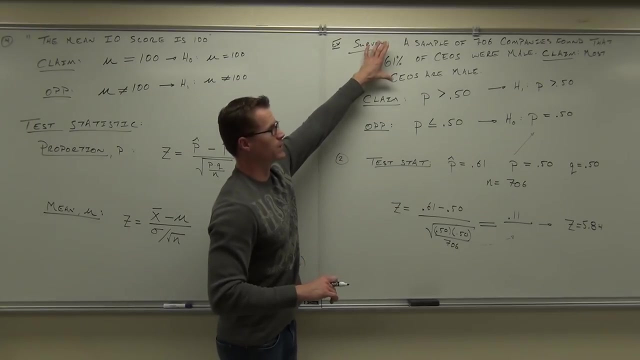 You rounded correctly: 5.84? 5.84. 5.84.. Okay, so very short recap. We have a claim, We have some statement. We write it as the claim and the opposite. We translate both into symbolic notation. 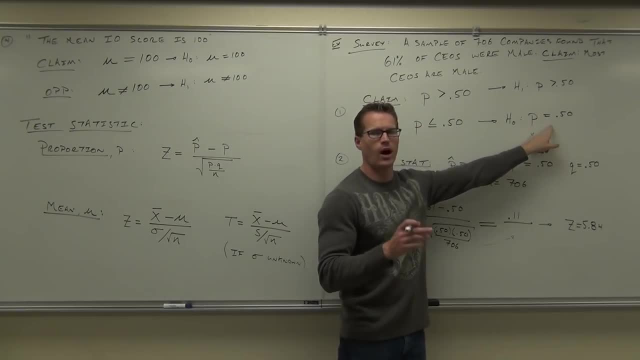 We write one as h sub zero. if it includes equal sign, We just write equals. Why do we write equals? It gives us an equality we can use in just a second. The other one we don't change at all. This is going to tell us right here. I'll give you a little precursor on whether you 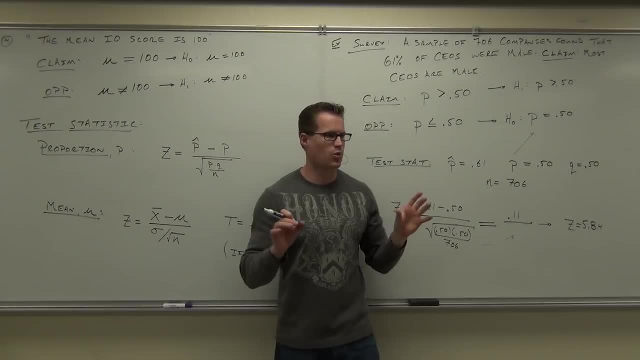 have a right tail, a left tail or a two-tailed test. That's going to be very important for us in a little while. After that, we use all that information to find a test statistic, What this does. this is a very important test. 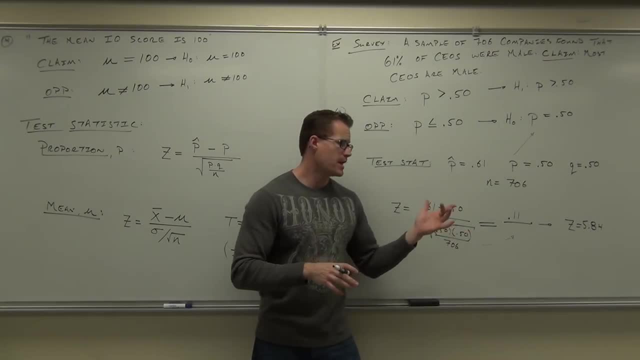 This is a very important piece for us- is tests our claim. Now you have to know whether 5.84 is a usual value or an unusual value. Is 5.84 usual or unusual for a z-score? Do you remember the range of usual values for z-scores? 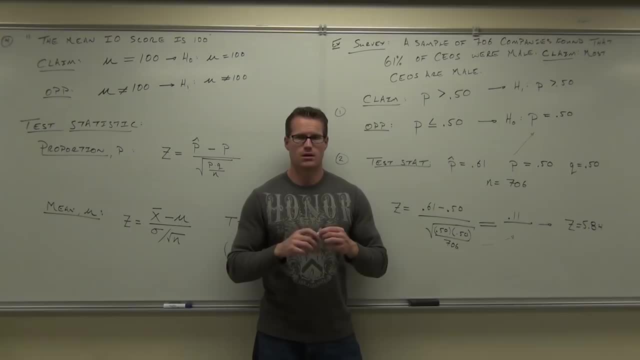 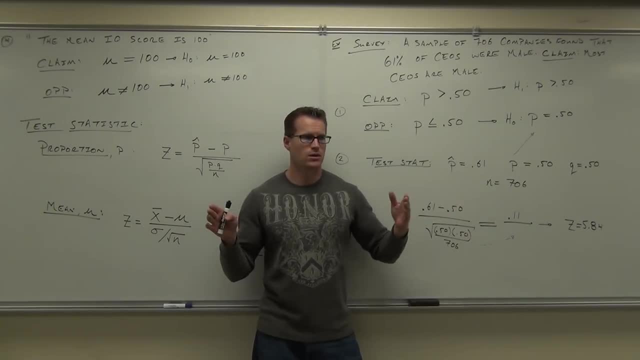 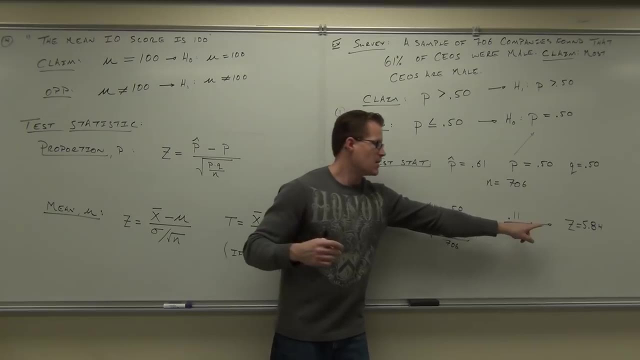 If it's in that range, it's unusual. That's the rule of thumb. Is that usual? That's way out there, Right, Listen, here's the whole idea. If this is rare enough, please watch on the board here real quick. 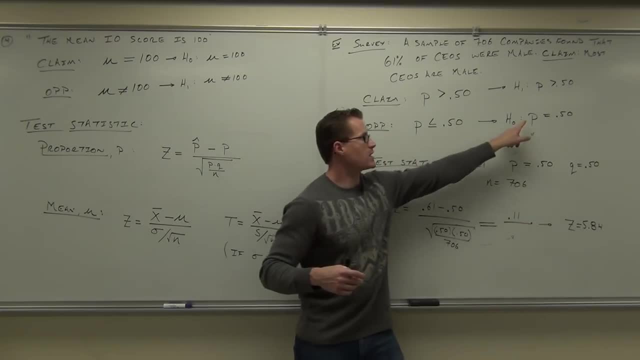 If this is rare enough, it means that our H sub zero is wrong. If our H sub zero is wrong, it means our H sub one is right, and we just proved our claim. Does that make sense to you? Now, the problem is, we don't know what rare enough means. 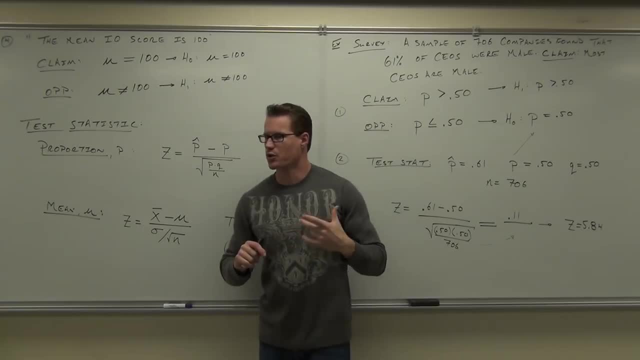 Is this rare enough? Is it not rare enough? We don't know. We're now going to incorporate the idea of significance level. That was the chapter seven idea. Remember significance level? It was like you were. 95%. confident meant the significance level is .05,. 99% meant .01 for. 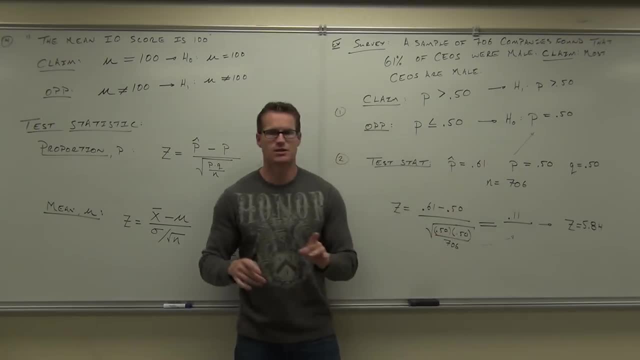 significance level. We're going to incorporate that into that idea. That's going to tell us: well, if you only need to be 90% certain of it, no problem, You can test certain hypotheses and get away with it. But if you need 99%, well, we're going to tell now how certain we are about our hypothesis. 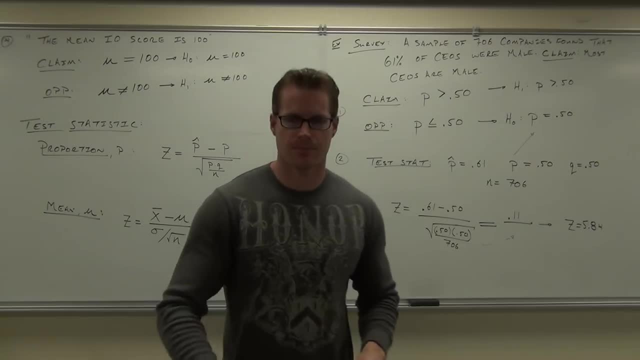 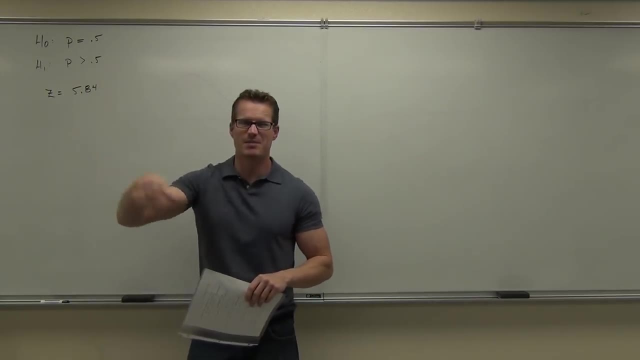 test That's going to be there, Okay, so from last time, we have already stated our claim. We stated the opposite of the claim. That's always your first step. We made one of them H sub zero and one of them H sub one. 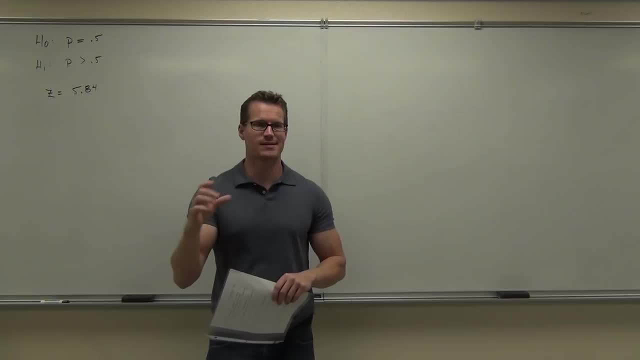 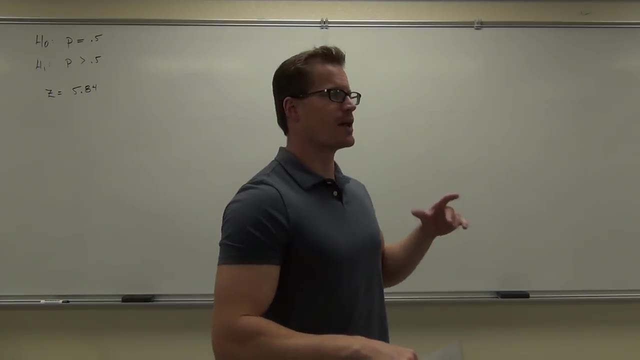 Of course the H sub zero has the equality. The H sub one doesn't. It has this thing that doesn't have the equality. It could be either the claim or the opposite, depending on how the statement is worded. After that we went and made our test statistic. 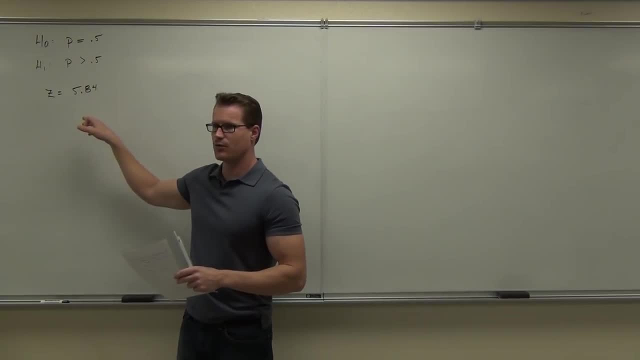 It's for proportions, a Z score, which is why we get that Z equal 5.84, but we were trying to make a decision on whether this was a positive or a negative. We were trying to make a decision on whether this was a positive or a negative. 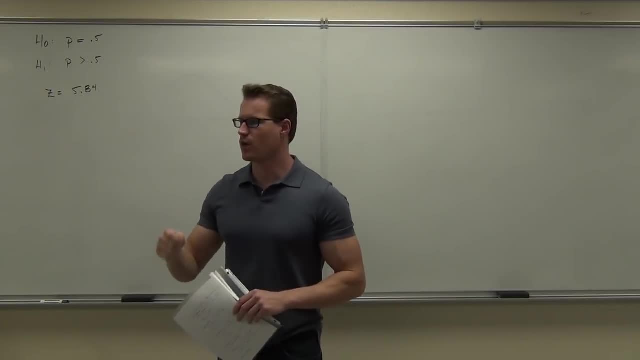 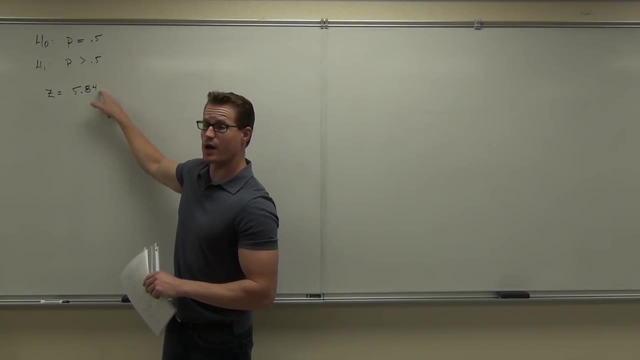 We were trying to make a decision on whether this was a positive or a negative. There was good enough evidence to reject our null hypothesis. whether this made this one false and therefore this one true, or whether this wasn't good enough, wasn't rare. 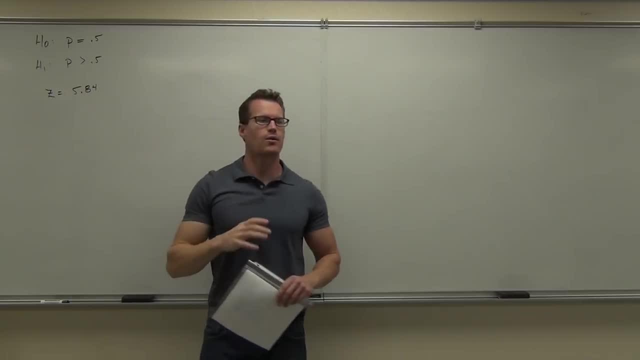 enough, and therefore we couldn't say anything about that one. That's where we're at right now. In order to do that, we've got to learn how to make a decision. That's where we're going to start today. 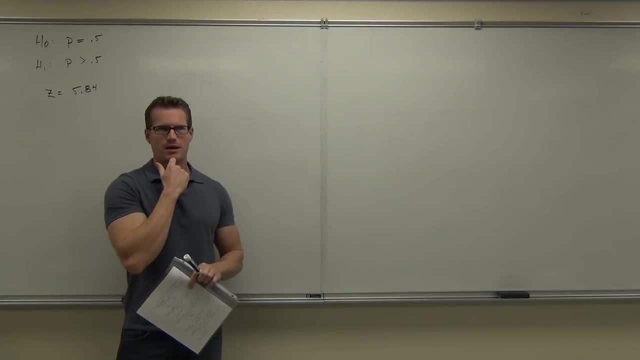 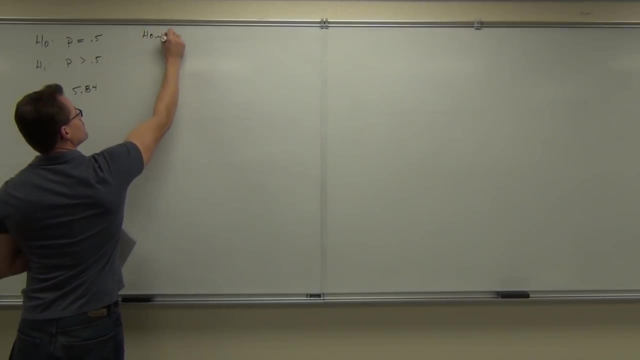 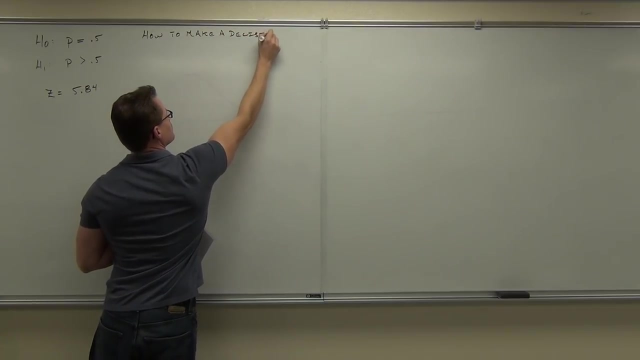 How to make a decision, and I don't mean: should I have pumpkin pie or peach pie? Not that type of decision. a decision based on your evidence and your statistics, Any of you. So I guess what I was trying to say by that is a decision is not a judgment call. 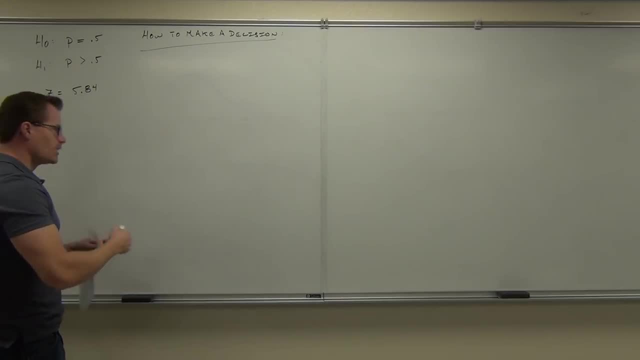 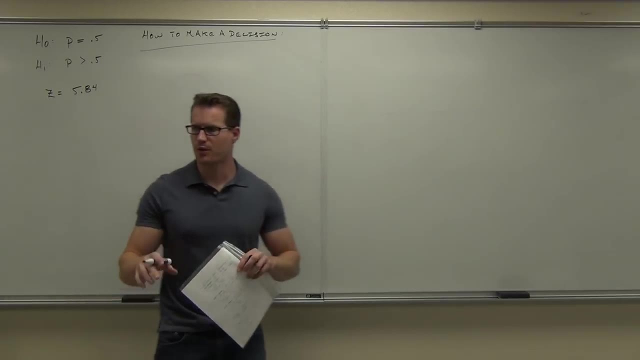 It's based on math. It's a math decision. Now, in order to make a decision, you've got to know what the significance level is. Now, that should be familiar, because we've already talked about significance level. It went back to the confidence intervals. 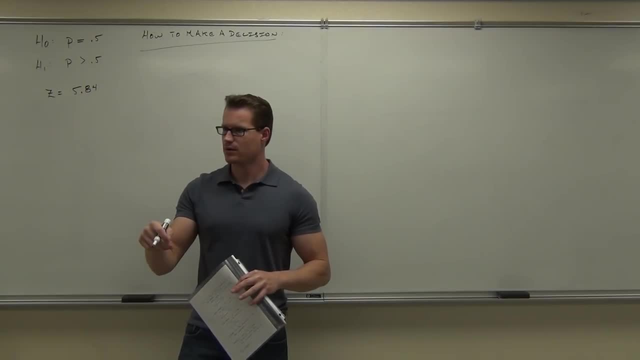 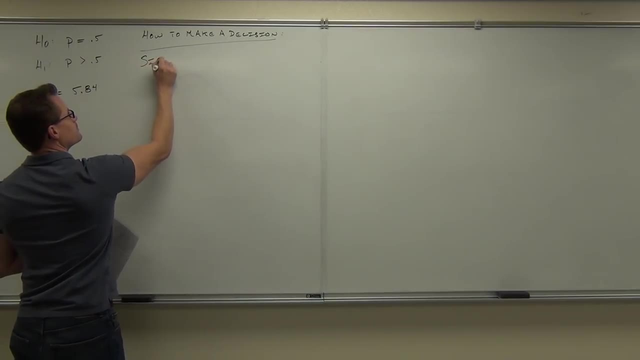 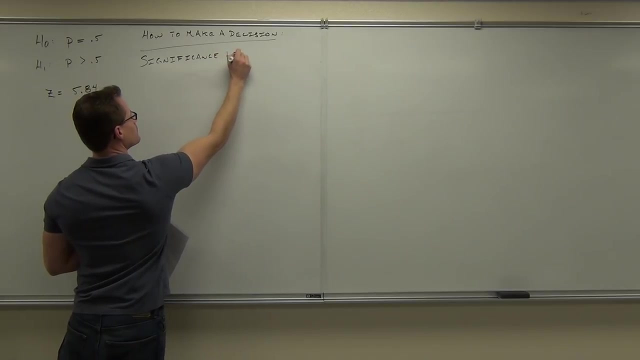 Remember confidence intervals? We had the alpha. Do you remember the alpha? Yeah, I hope you do. It was a compliment to your confidence level. It was called the significance level. So we're going to have a significance level, Just like before. it's given by alpha. 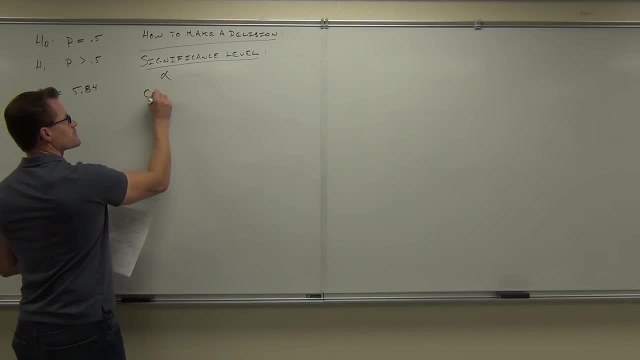 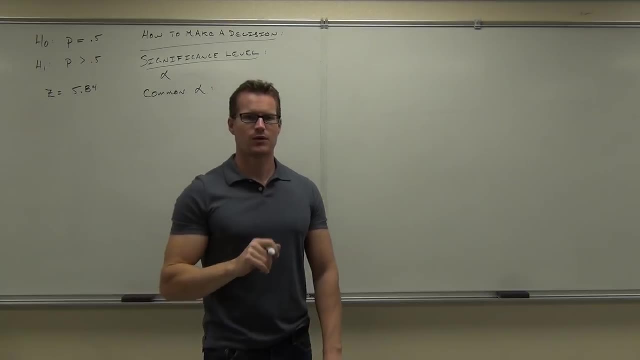 Now, do you remember the common alphas? Yeah, The common alphas: .10.. No, Those would be the critical values, Those would be the Zs. I'm not talking about the Zs, I'm talking about the alpha. 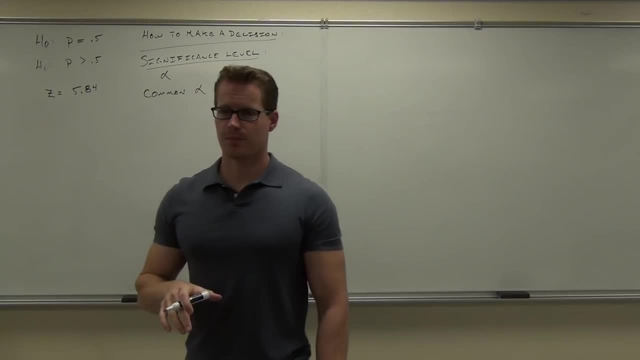 .1.. .1 was a common one, Right? That had to do with the 90.. .95.. Yeah, So .10 is an alpha. Remember, these are the compliments to your confidence levels from chapter seven. What's another one? 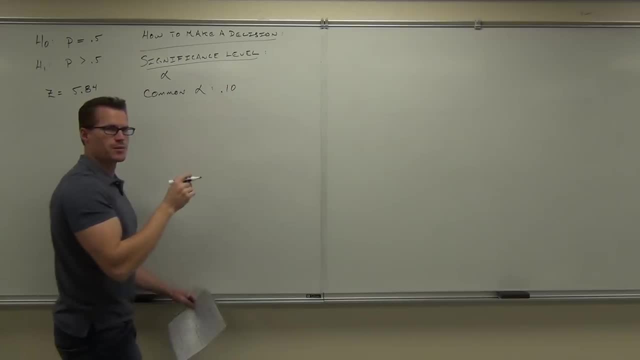 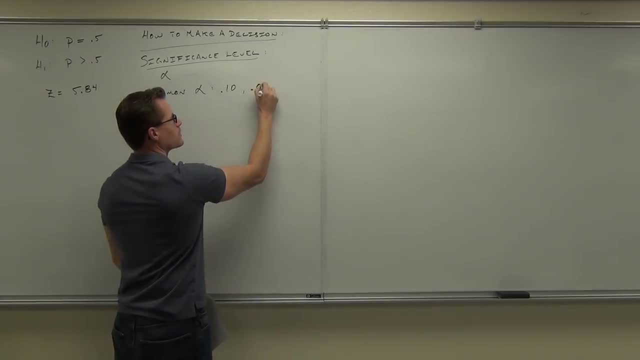 Remember doing that. So .05 was another one. What was the last one? .05.. Now do they have to be .1,, .05, or .01? No, They can be anything you want. These are going to be the most common ones, though. 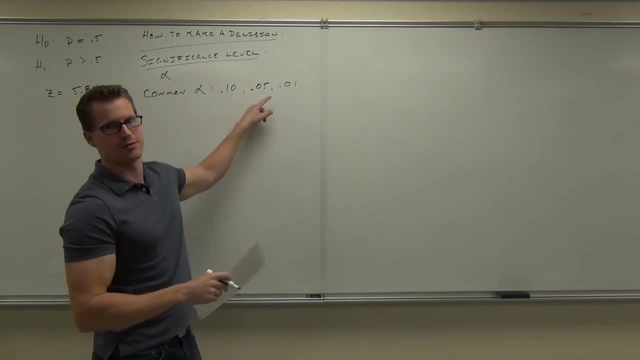 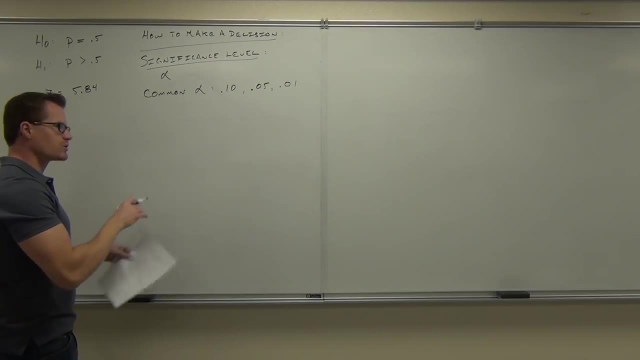 Those are typically what you see. This one is by far the most common that you have. You usually deal with a 5% confidence level or significance level Usually. Now we're still going to have critical values. Critical values were from chapter seven as well. 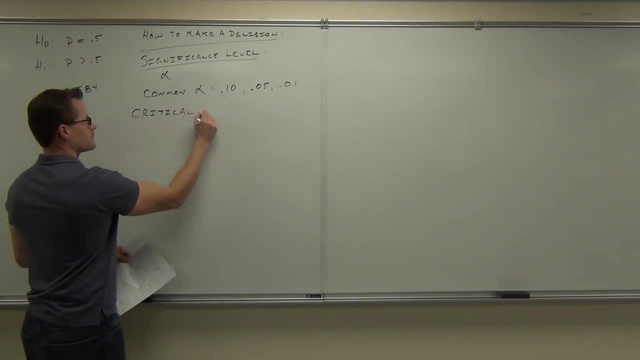 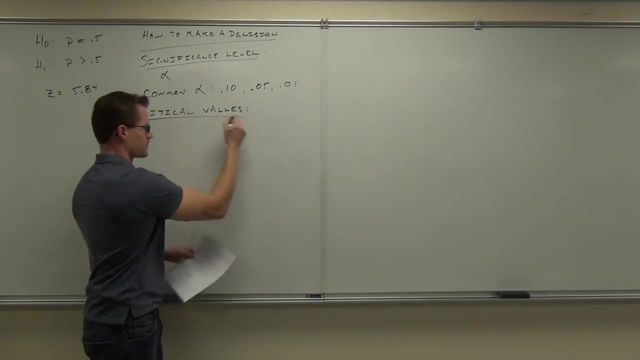 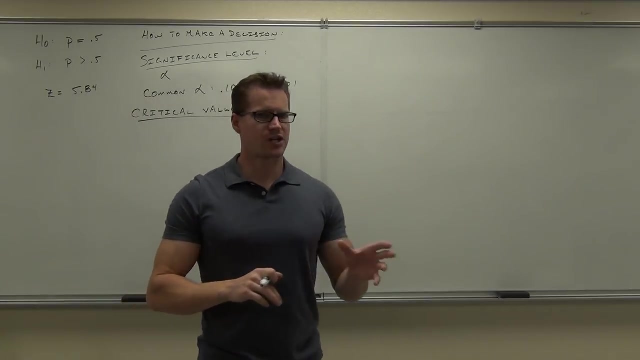 So we still have that. So critical values. Only this time the critical values are going to separate what we're going to call the rejection region from the fail to reject region. I might have mentioned that before, but it didn't make a whole lot of sense back in chapter. 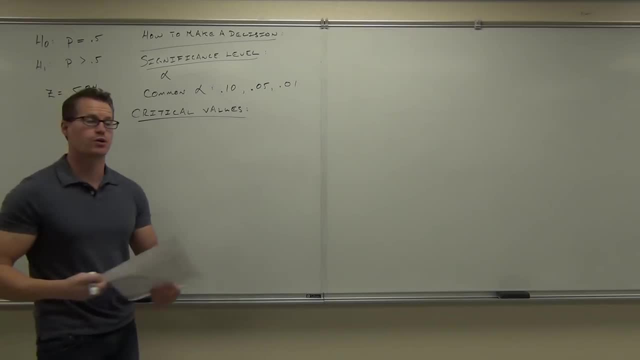 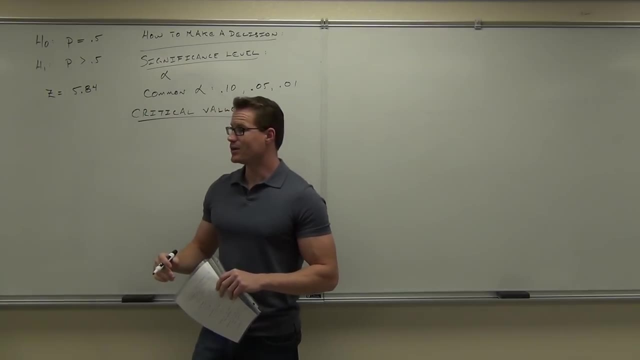 seven, because we never really worked with it. Now we get to work with it. So a critical value separates what we're going to call the rejection region from the fail to reject region. Why is it important now? Hey, we're trying to reject a claim, now right. 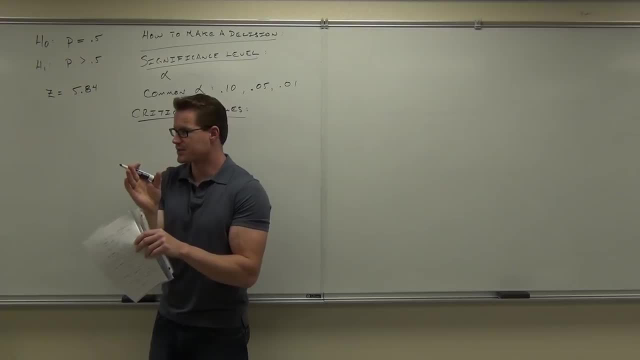 We're trying to reject H sub zero. So if it falls at the Z score, our test statistic falls in the rejection region. we reject. If it doesn't, we fail to reject. That's it. That's a decision that's based on mathematics. 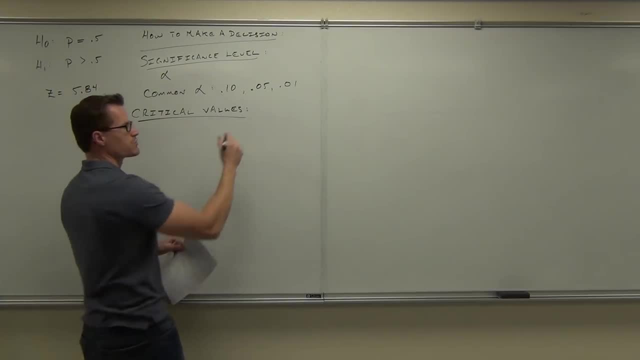 So critical values are pretty important for us. They're going to separate the rejection region from the fail to reject region. Okay, So those are critical values And what we're going to do next there We're going to write down this: groups今天的 summary from 216.. 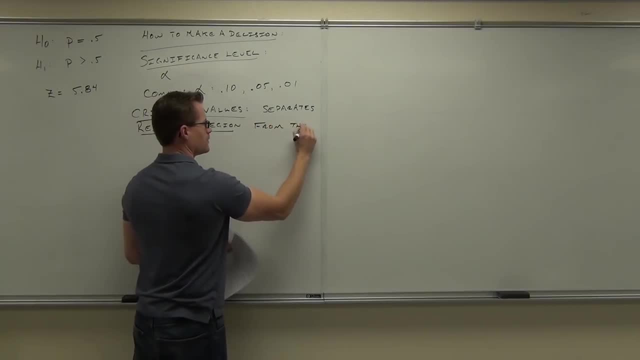 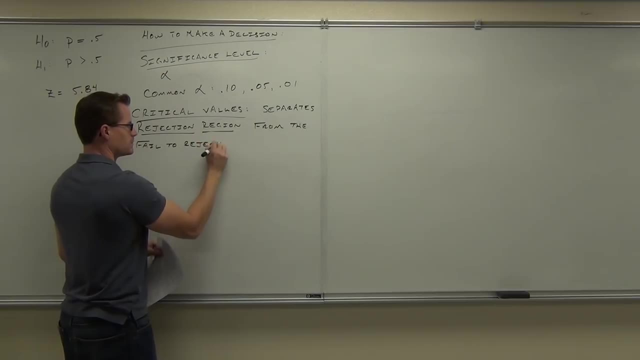 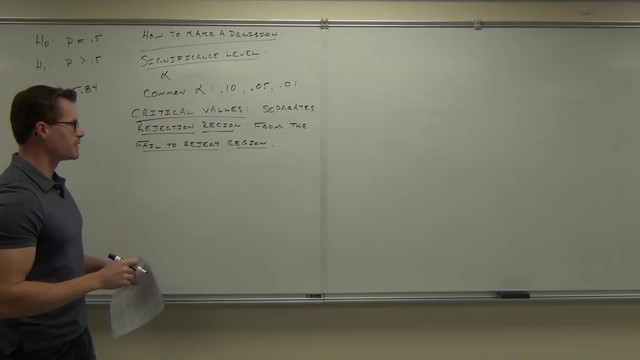 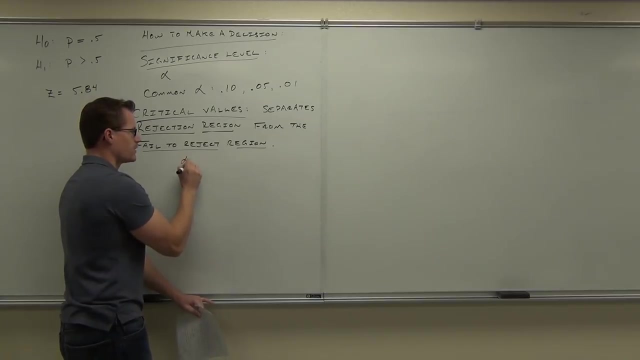 It fold out two points that fall in our task list. We'll come back with the series in a different form in just a minute. Also, we're going to be finding our critical values the same way that we would before. So if you have an alpha of .05, if we're talking about a right tail, test your z critical value. 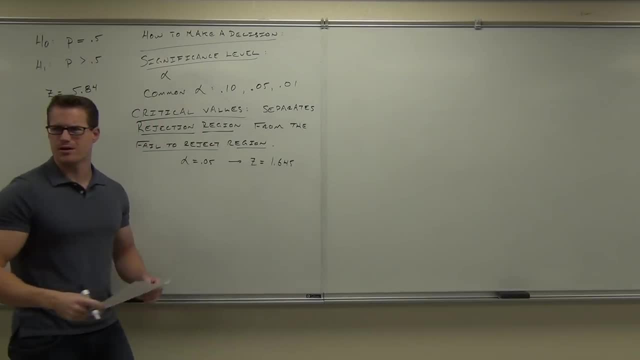 is 1.645.. Do you remember how to find those? We look at the .05 on the table. it's going to give us 1.645.. Actually it would give you a negative, but we're talking about a right tail test. 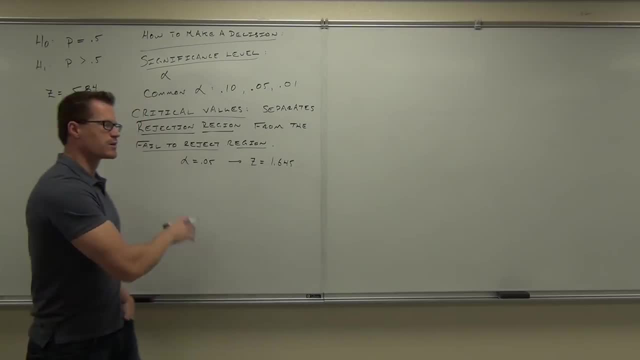 We'll talk about right, left and two tail tests in just a minute, but for right now, stick with me. These are found in the same way. Now here's what the rejection region does. We just spoke about the value, the critical value that separates the rejection region. 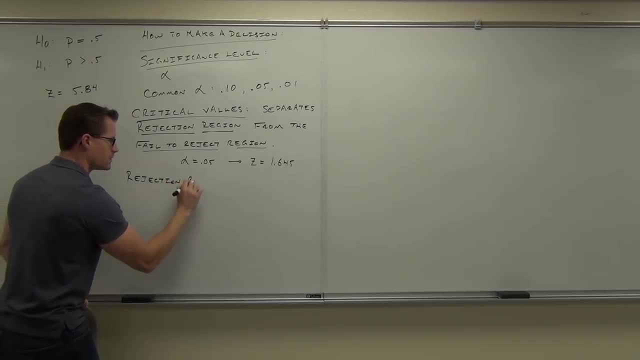 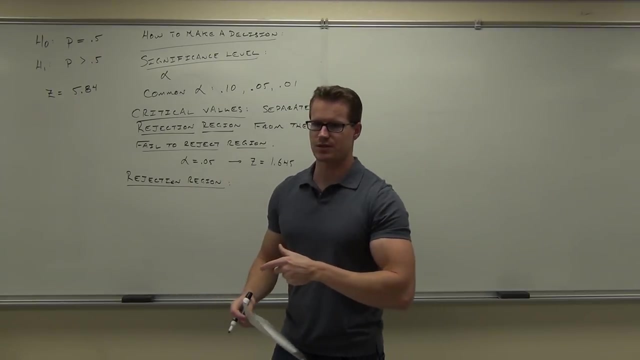 from the failed rejection region. It's the region that, if our test statistic falls in that area, we get to reject the null hypothesis. That's called the rejection region. If you fall in the fail to reject region, well then your test statistic's in that area. 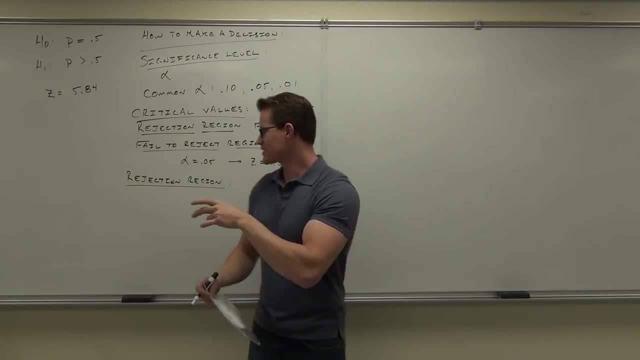 saying you don't have enough evidence to reject the null hypothesis. The rejection region is actually. it sounds bad, right, you don't want to be in the rejection region. That's like high school. High school for me is in the date. rejection region- off in high school. 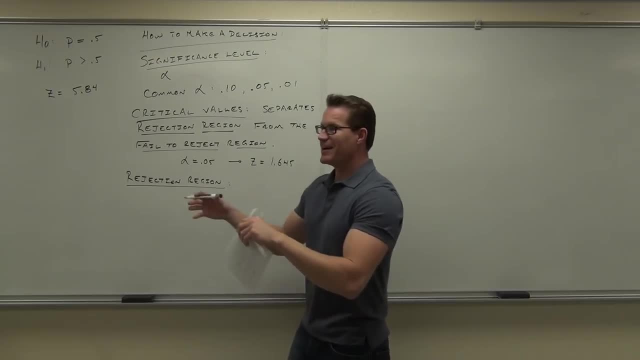 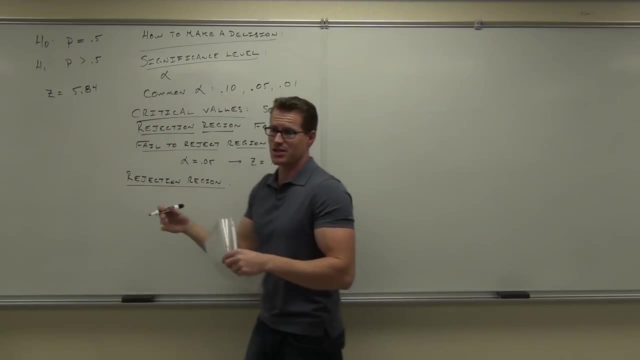 That's okay. But now it's good to be in the rejection region, because that means you have enough evidence to overturn your null hypothesis and prove the other one right. So the rejection region here is not a bad thing. it could be a good thing. 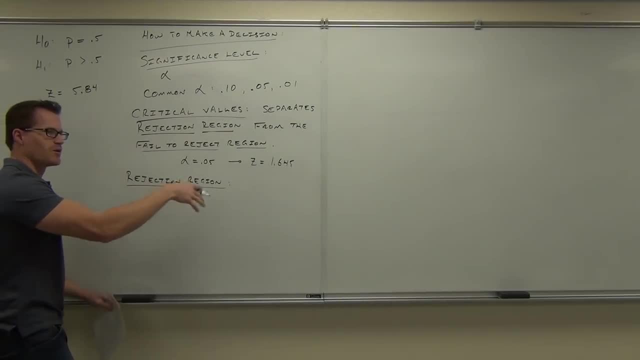 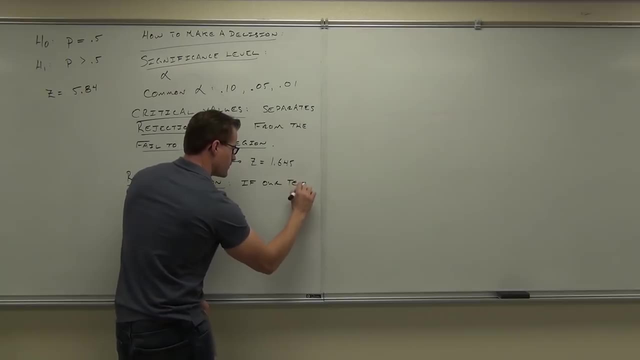 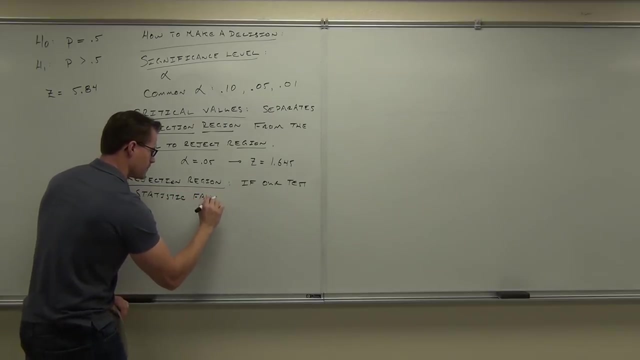 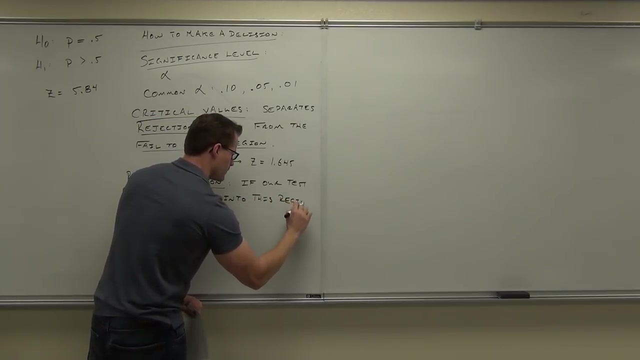 Prove your statements. So this is the region that, if our test statistic falls into, we get to reject the null hypothesis. If the test statistic falls into this region, you reject H sub zero and get a null hypothesis. Why would you reject H sub zero and get a null hypothesis? 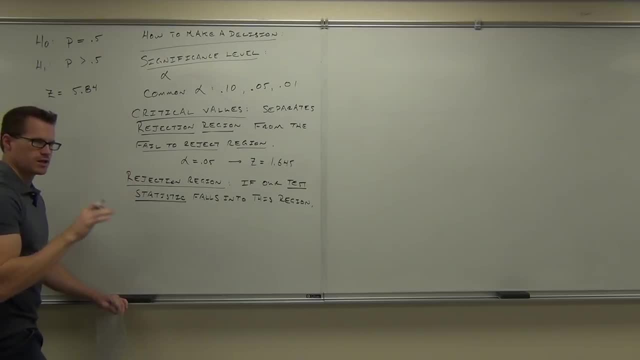 Because if you reject H sub zero and get a null hypothesis, you reject H sub zero. Okay, Okay, That's neatly thought, Okay, Okay, Okay, Okay. let me show you how this is going to work. Now, you're not going to be able to get this this far yet, but I'm going to show you how. 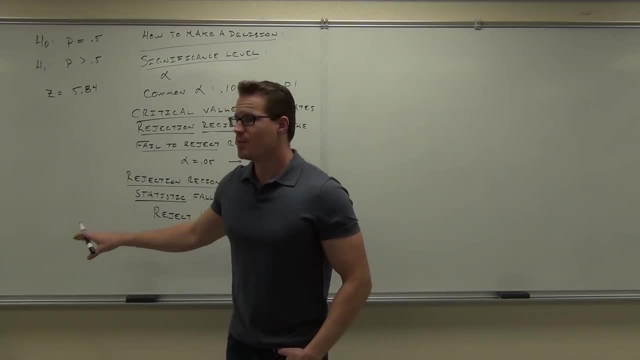 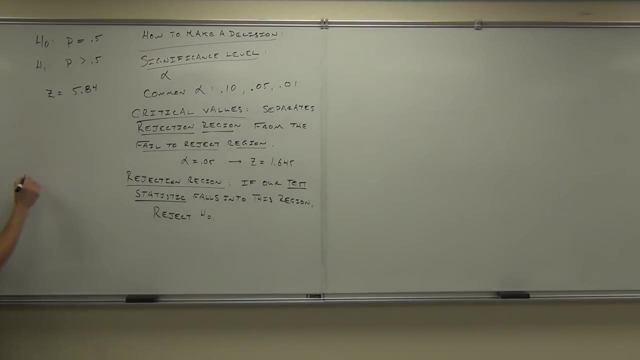 to figure out the type of picture I'm going to draw here in just a moment. But here's how this particular problem- remember the problem we were dealing with last time, right? This is a continuation of that. It was this information. Here's how this would look. 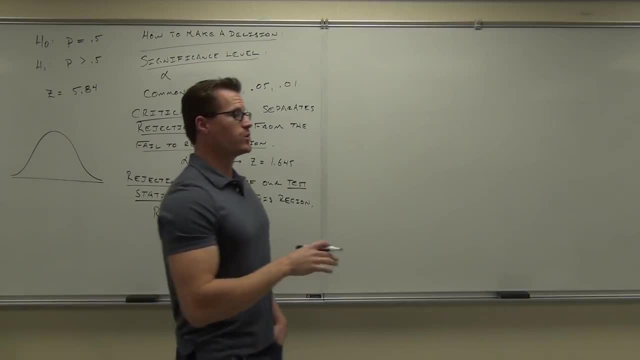 You're still going to be drawing this picture. it's the same picture all the time. I'm going to show you in a moment how to determine that this is a right tail test. I'll prove to you in just a second that this is going to be a right tail test. 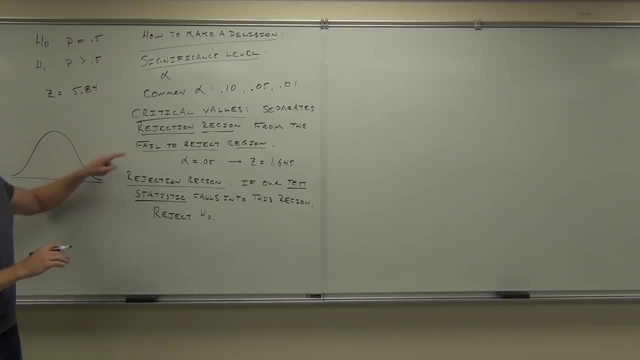 Here's how you do it. First thing you do is you look at your alpha. So let's assume that we're dealing with a .05 significance level. That's giving me a critical value of 1.645.. So remember zero's here. 1.645 will be right there. 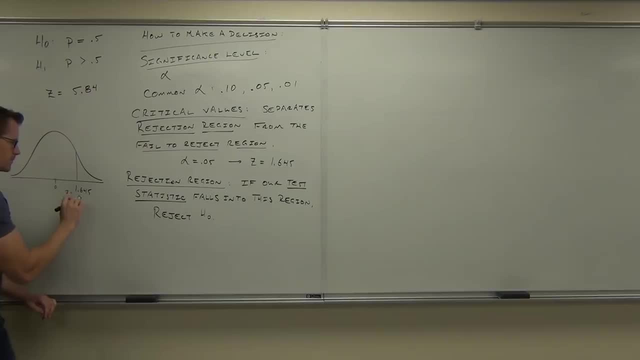 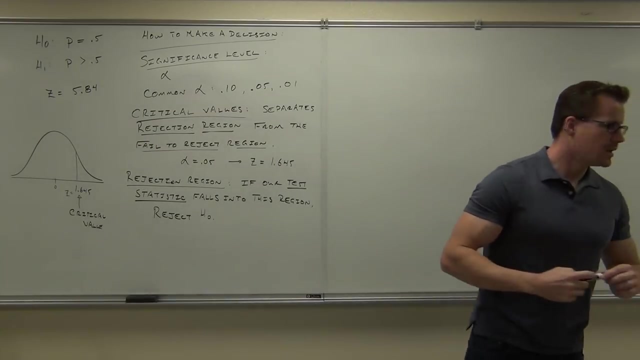 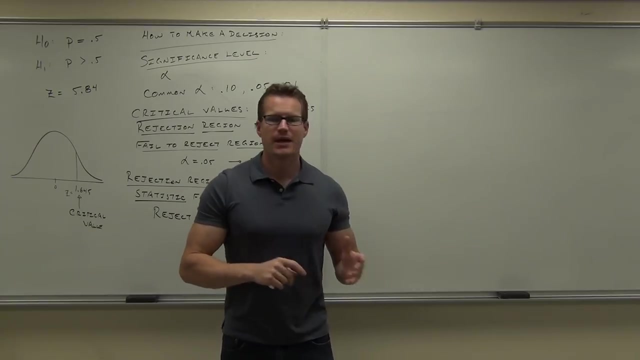 This is my critical value. Write that down in your paper, that this is a critical value. Okay, Now what that critical value does that we wrote up here. it separates the rejection region from the fail to reject region. Here's the separation. 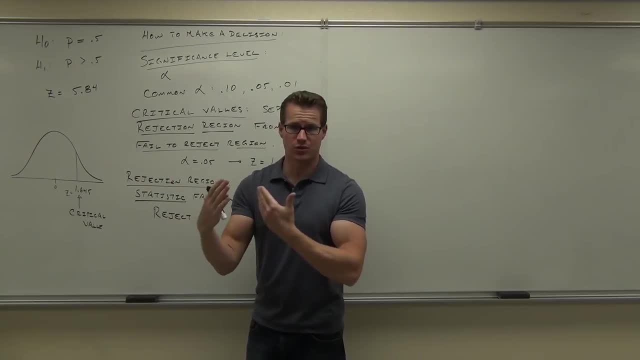 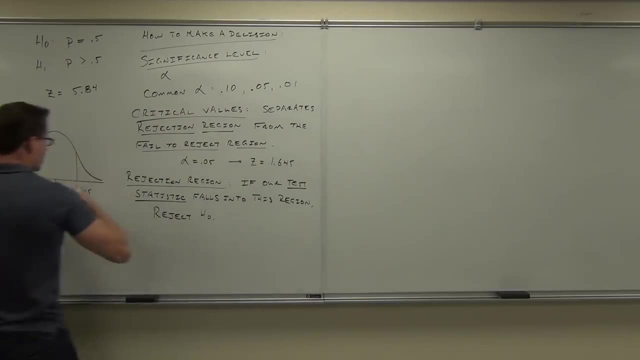 The area in the tails is the area that is your rejection region. So in here, this is the fail to reject region. Here the tail. that's your rejection region. So this is the tail. This tail right here represents .05 as a proportion of your area right here. 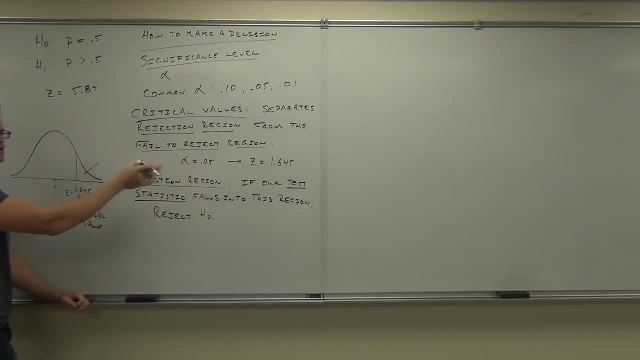 That's how we found our 1.645.. We would look up the .05.. It's going to give us a critical value of 1.645.. We put that on our paper. This is the rejection region. This would be the fail to reject region. 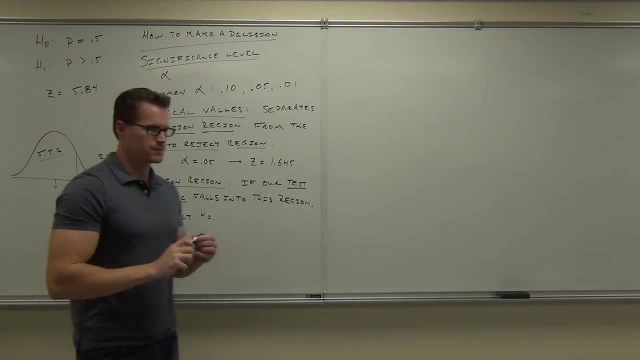 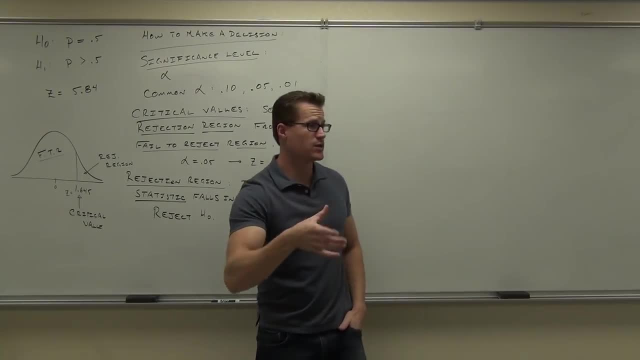 That's multiple failures. This is the failure to reject the return region. This is the failure to reject region. That's the fail to reject region. This is the failure to reject the return region. It's not because of the high latency between things. 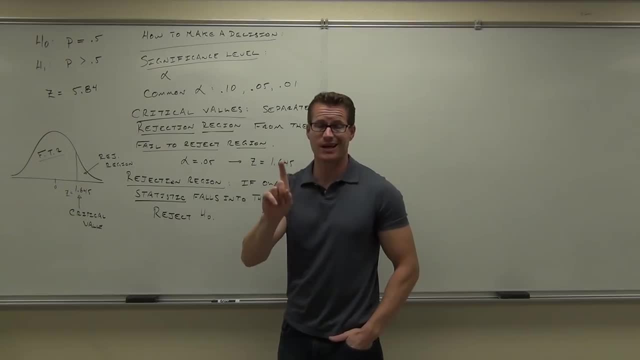 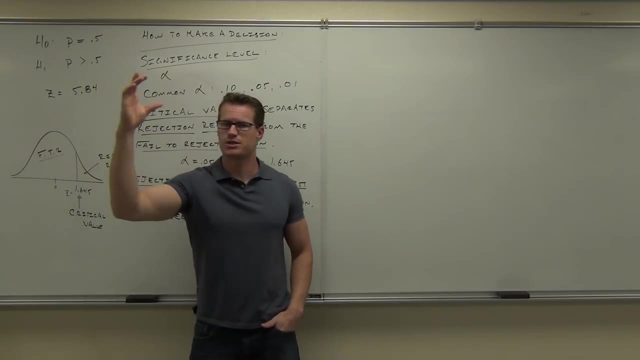 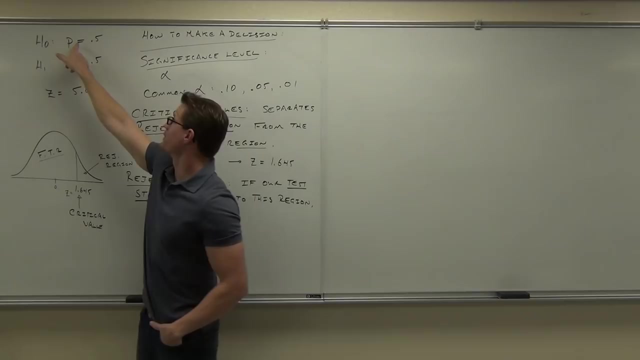 This gets just bigger and more confusing. So these are what the values are. Go ahead, One more problem and you create your z-score. Now notice that on your paper you have two z-scores, don't you? You have one. that's a critical value. 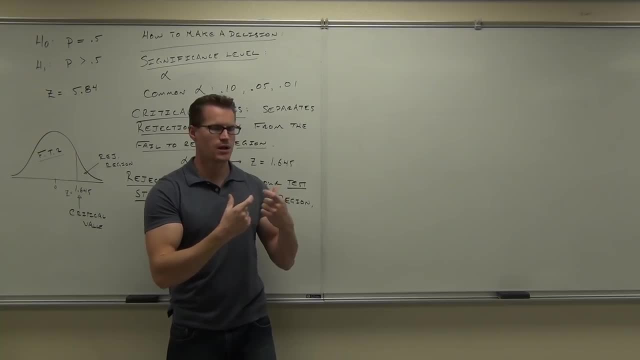 and you have one that is a test statistic. Are you following on this? Your critical value is what you put on your paper. Your critical value- it's called the traditional method- is put on your paper That separates the rejection region from the failed to reject region. 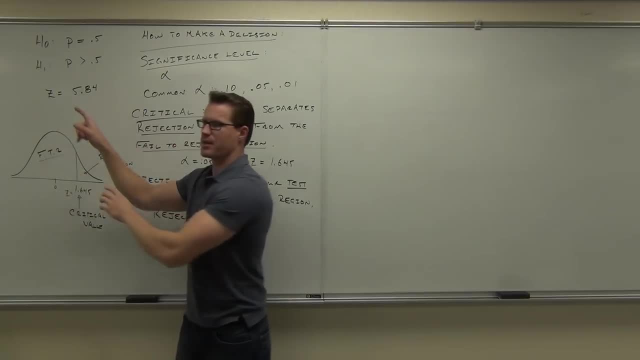 Your test statistic. that number that you created, that's based on your comparison between your samples data and your population hypothesis, gives you that number. This is what you test. Well, it's called a test statistic. It's what you're testing against your critical value. 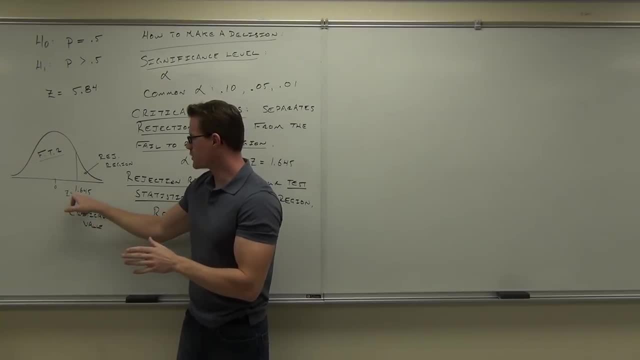 So you compare these two numbers, You compare the 1.645, and you compare the 5.84.. You look where the 5.84 is in relation to the 1.645.. Does it fall in the failed to reject region? 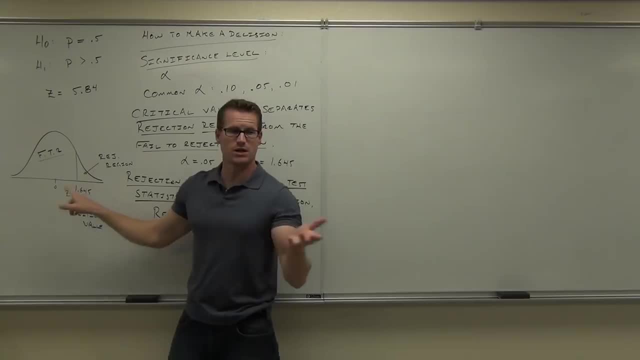 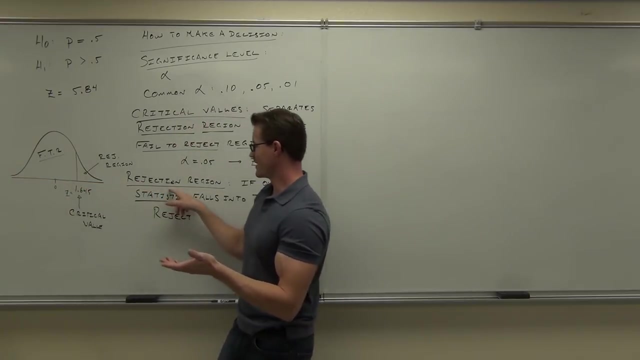 or the rejection region: Rejection. Can you tell It's a number line? Where's 5?? Is it here? This is negative. Where's 5?? Is it here? It's like here. It's like here actually. 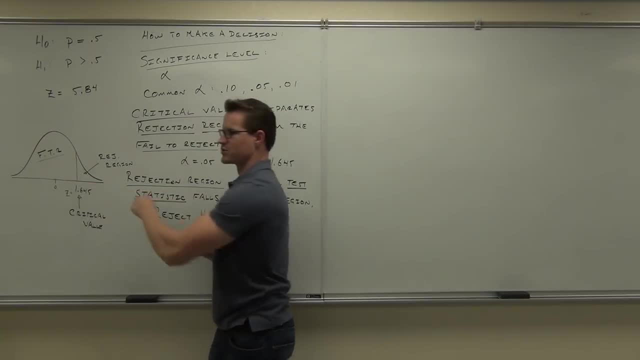 It's way over there Is that in the failed to reject region or the rejection region- Rejection Definitely rejection region That tells you you are going to reject your null hypothesis- You say: this one's wrong, this one's right. 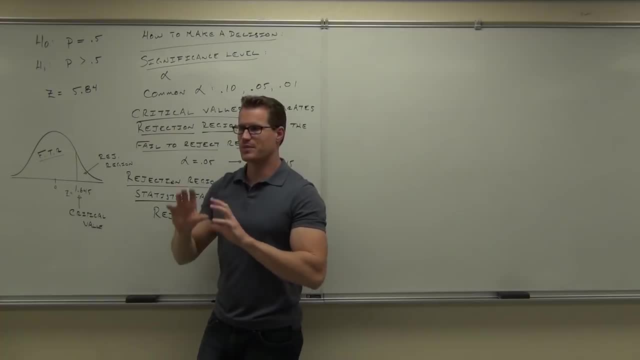 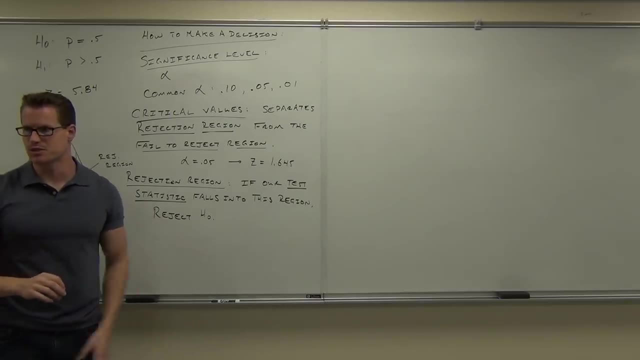 Booyah just proved my claim. That's how you make a decision, So it's based on lots of information. It's an involved process. Problems don't go quickly. They go slowly. You have to really work at it. There's seven steps to doing it. 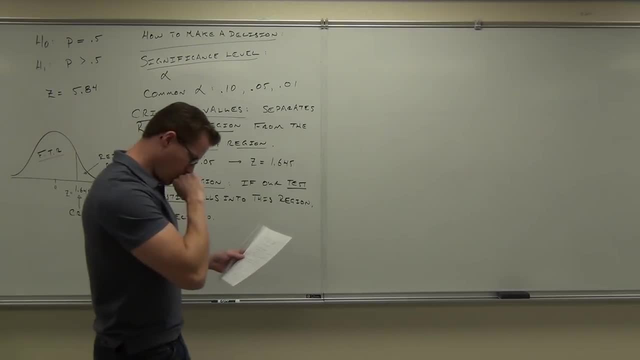 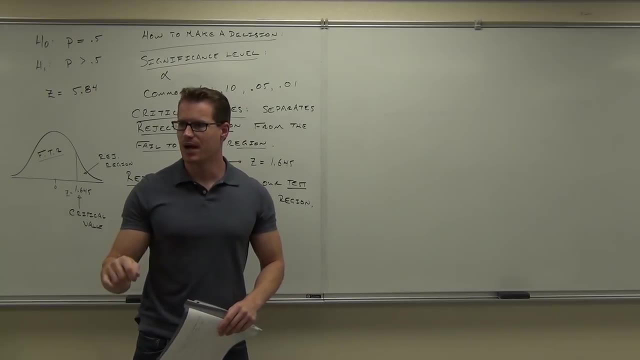 I'll show you all those seven steps as we keep going. Now, what you also need to know is that your critical value will change depending on whether you have a left tail, a right tail or a two-tail test. We'll be focusing on this. 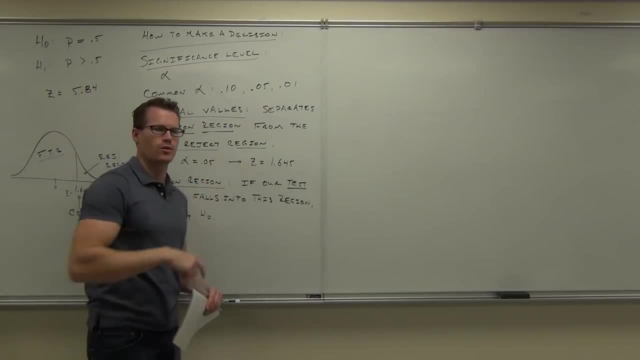 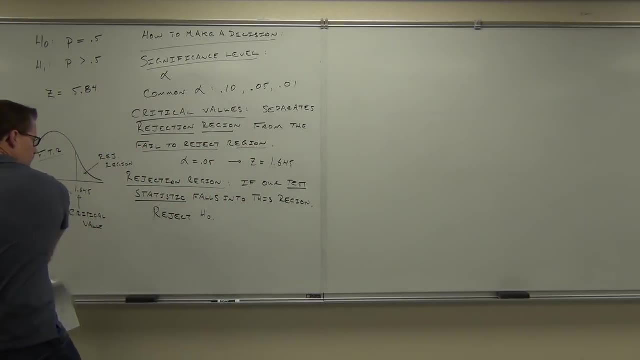 This is an important part for you. OK, You can't just memorize these numbers anymore. They're going to change sporadically as you talk about a different situation. So let's go ahead, Let's see if we can. Let's see if we can figure out one of these examples. 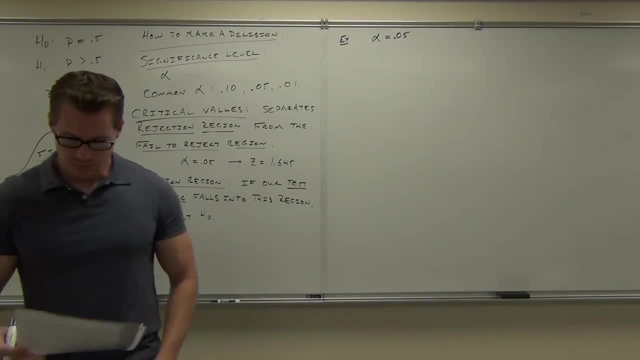 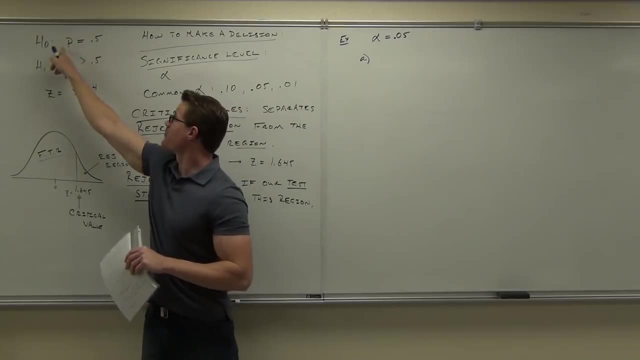 So let's say my alpha is 0.05.. That's my significance level. I'll give you three cases. I'm going to change this a bit, but it's coming from here. Let's suppose that I have a right tail. 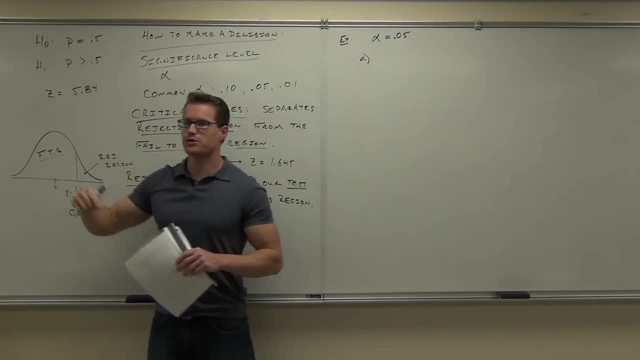 I have different h sub 1s, different alternative hypotheses. These are the ones that tell you whether you're going to be a left tail, a right tail or a two-tail test. I'll make it very explicit in a moment. 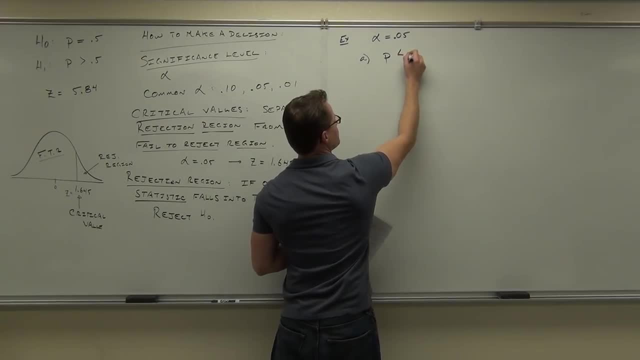 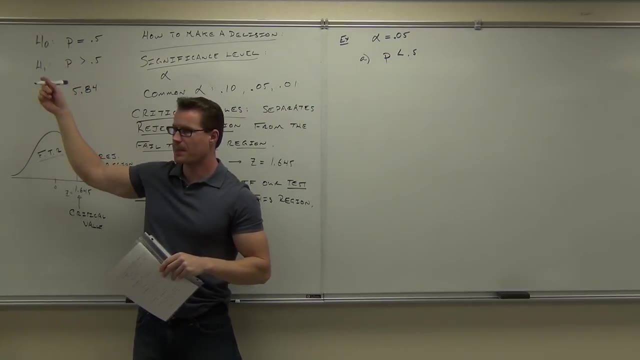 But here's our situation. Let's say that p was less than 0.5. This 0.5 is not that 0.5.. OK, I'm going back to this proportion being less than 50%. Oh, I just jumped a letter. 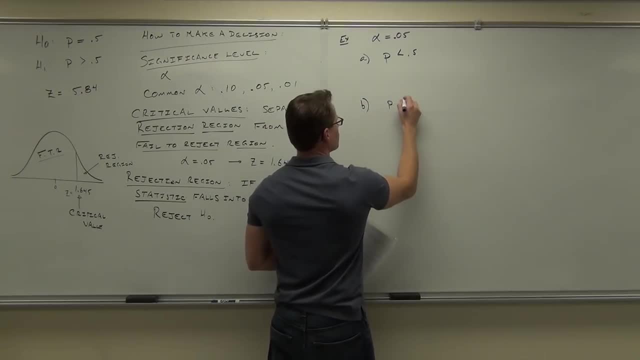 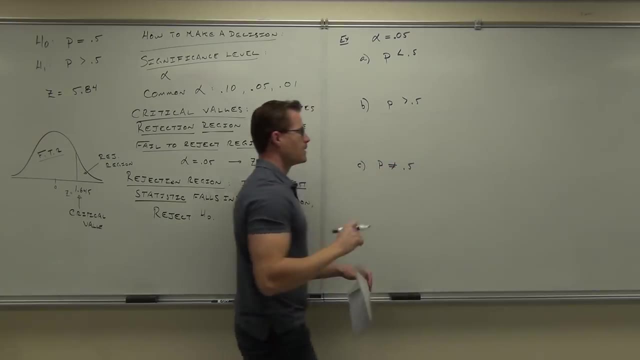 OK, I'm going to make it very explicit in a moment. So let's take h sub 1s and make them equal. These are the only cases you can possibly have for an alternative hypothesis. Remember the h sub 1s. those are the ones. 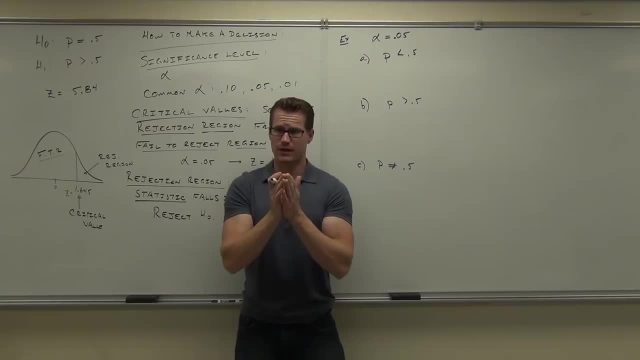 that don't have the equal sign. They're either going to be greater than, less than or not equal to, So you'd have, like h sub 1, or this h sub 1, or this one. OK, And then I'm going to go back to my equation. 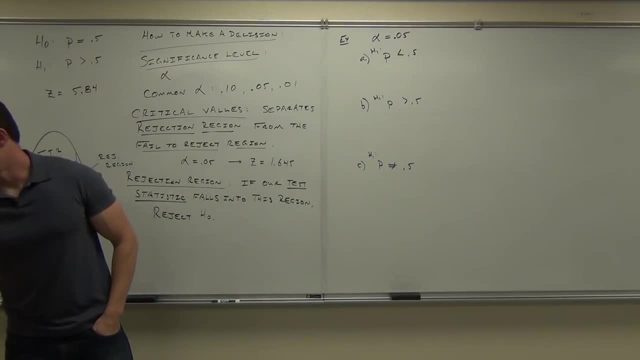 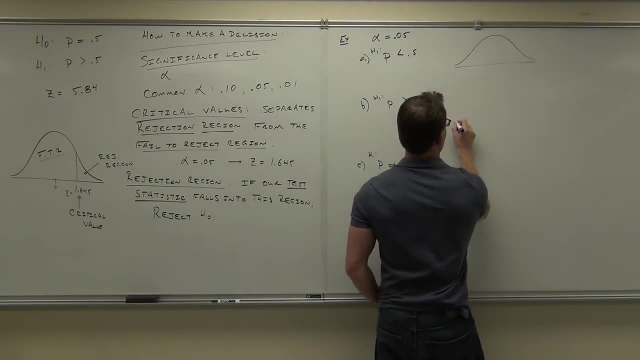 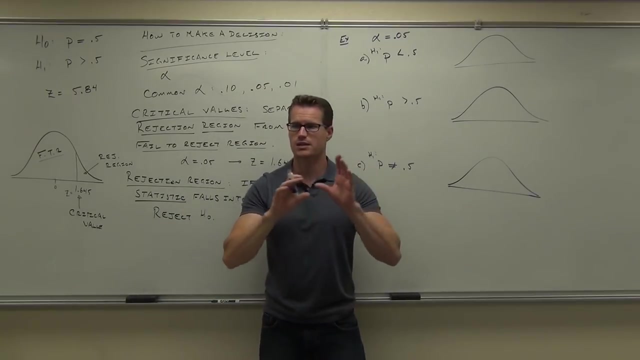 OK, Now here's how you determine what picture it is. in every single case, It's always going to be standard, normal curve and of course, we'll have zero in the middle. But you need to know whether we're talking about a right tail test, a left tail test. 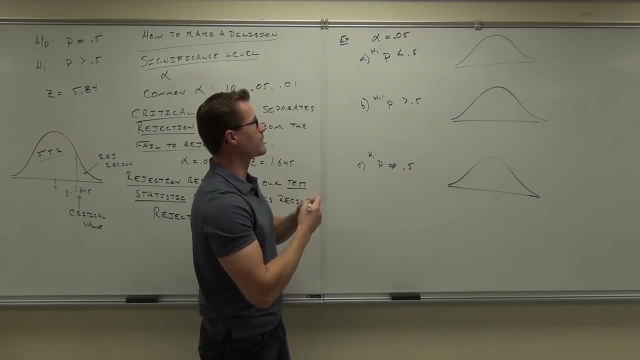 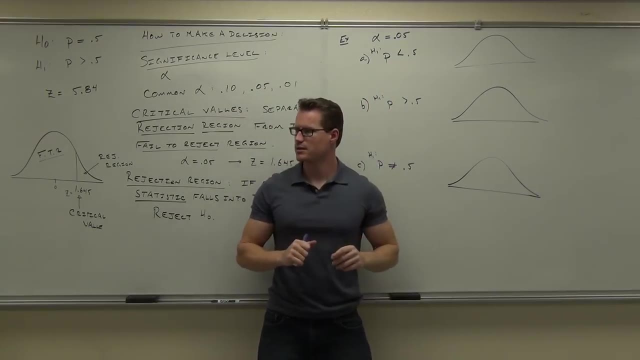 or a two tail test. it's not always the same. So, when we're looking at this thing, if you're talking about the proportion less than a certain value, where's less than? Is it to the left or to the right? Less than is to the left of something? 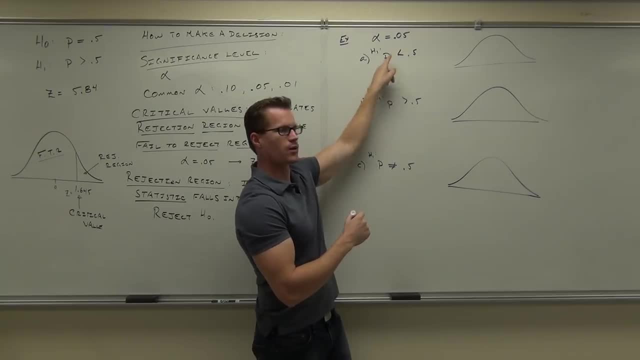 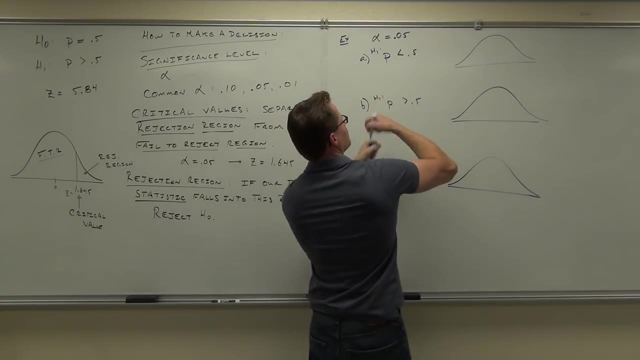 So if you have a less than see how the arrow's pointing to the left, You see that You're talking about a left tail test on that. The arrow's pointing that way, the arrow's pointing that way, isn't it? 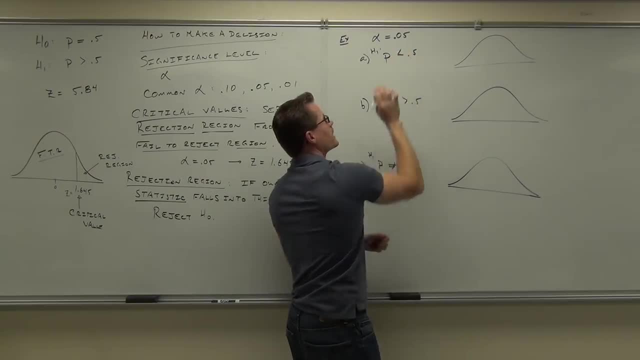 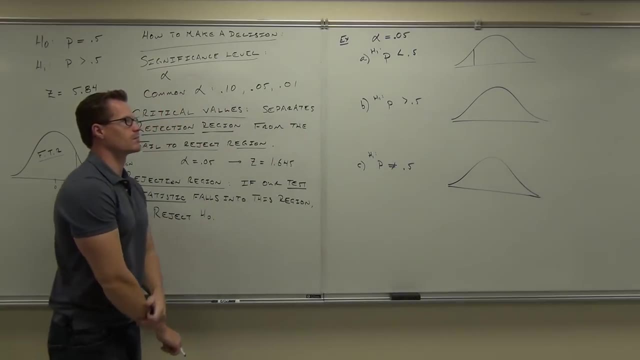 You make a little arrow out of that. If your h sub one says less than a certain value, it's less than a certain value. You will have a left tail test. This is the one we actually did over there. This was a right tail test. 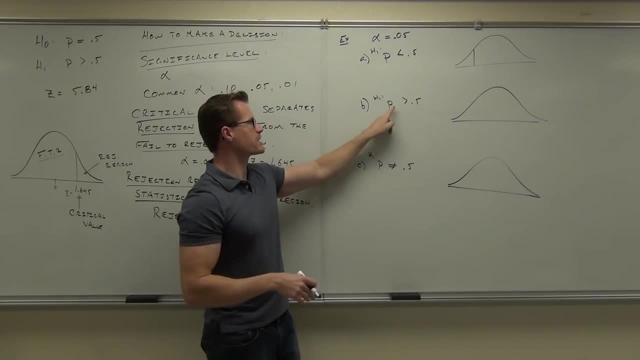 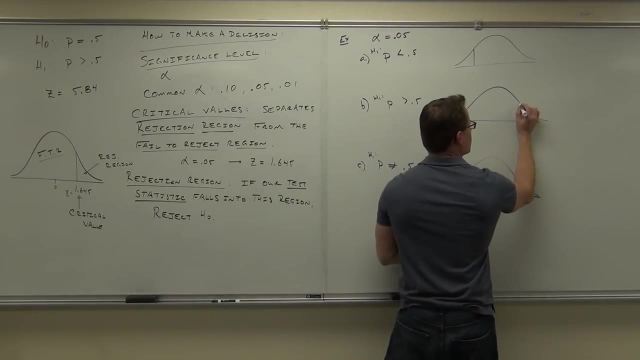 The reason why it was a right tail test, why I knew that, I said: okay, we're trying to say that proportion is bigger than a certain value. If it's big enough, it means it proved it right. So we're going to make a little stop over here for a right tail test. 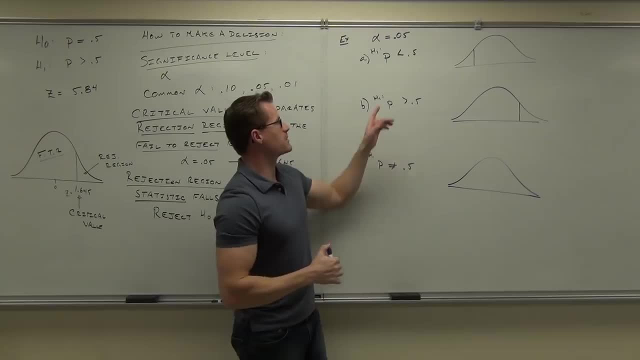 You see what this is doing is saying. is it rare enough to prove this true? Is it small enough? Is it smaller enough than 50% to say yes, this is accurate, Or in other words, h sub zero is wrong. 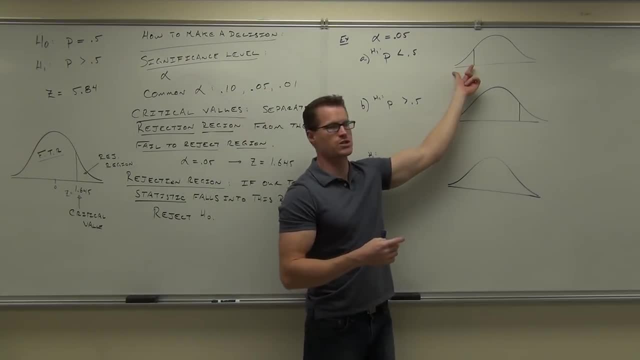 So this would be to the left of that value. This is smaller than 50%. Does that make sense to you? The right tail test says the other thing. It says: well, it has to be bigger than by a certain margin, And that margin's given to us by our significance level. 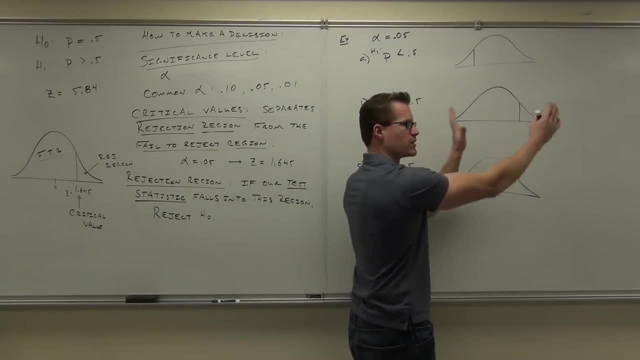 So here, left tail test- here it's pointing to the right. It says a right tail test bigger than a certain value, That's over to the right. How about this one? It says a not equal to What do you think? 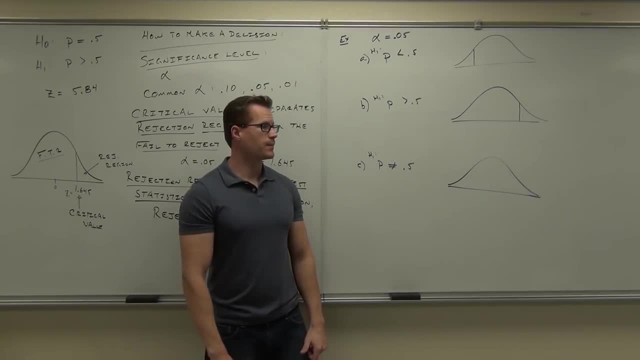 It can't be lefted, It can't be right. Hmm, Well, we've got to have a tail somewhere. Do you understand the idea of the less than and the greater than? You have to get these two before you can get this one. 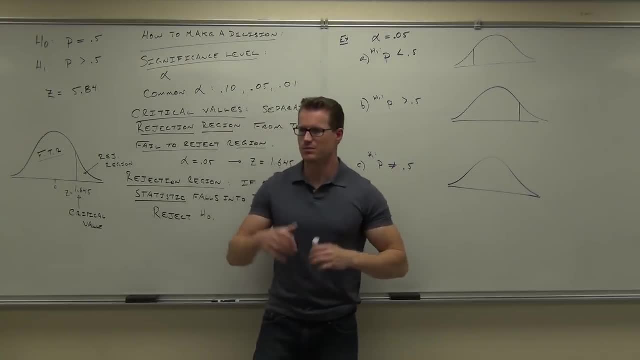 Some of you guys aren't really getting it. Let me go over it one more time. That way you really get it. You better kind of focus in on this. This is the last time we'll do it. What you're trying to do in these situations is you're trying to prove that this is not. 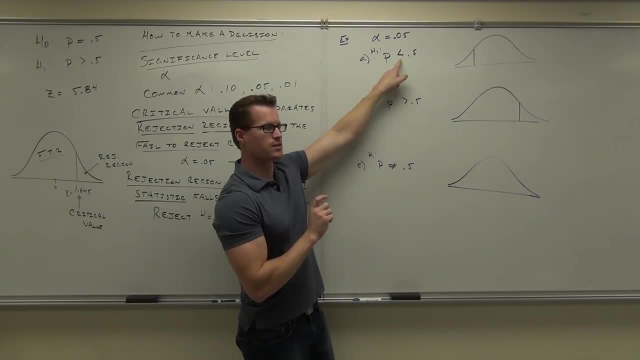 true. You're trying to prove this one right. If you have enough evidence, it would say that the proportion is less than 50 percent. It'd be farther enough to the left, farther enough, or small enough, to say that this is true. 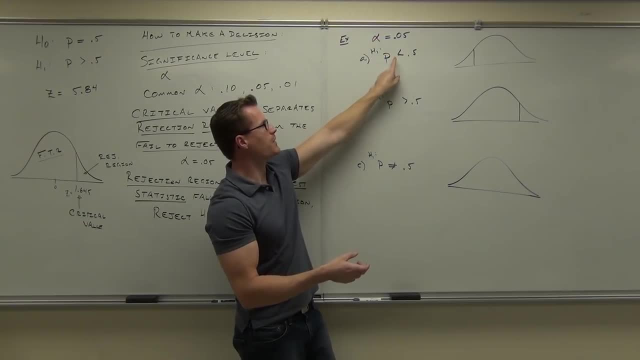 Basically, that H sub zero would be wrong is the only way you'd be able to prove that. But the to the left idea is saying: okay, we're looking for values that are smaller than some number. Here we have the opposite: We're looking for greater than. 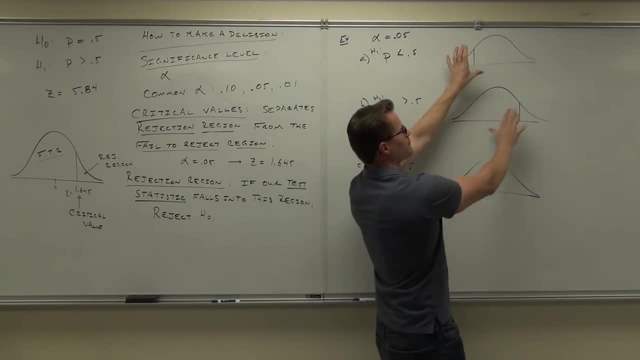 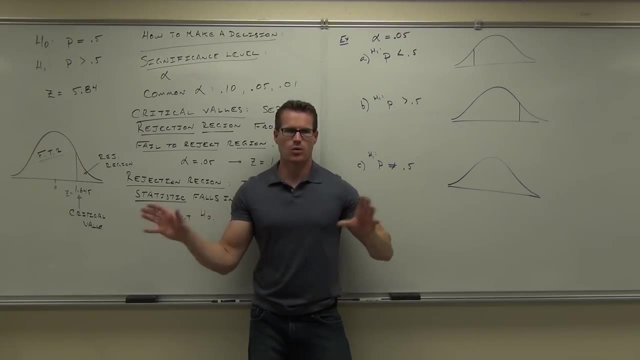 So we're looking for numbers that are smaller or numbers that are bigger. That's giving us a left or a right tail test. If we're not equal to that means it could be either smaller or bigger. Does that make sense to you? 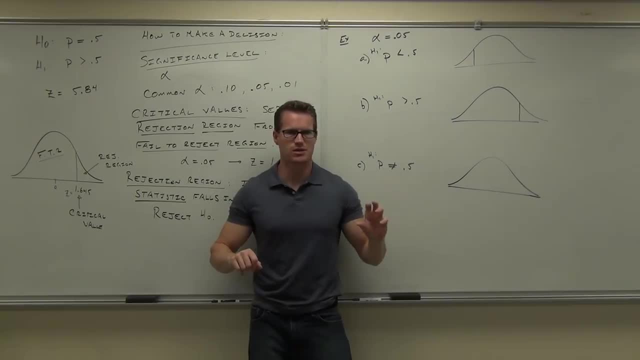 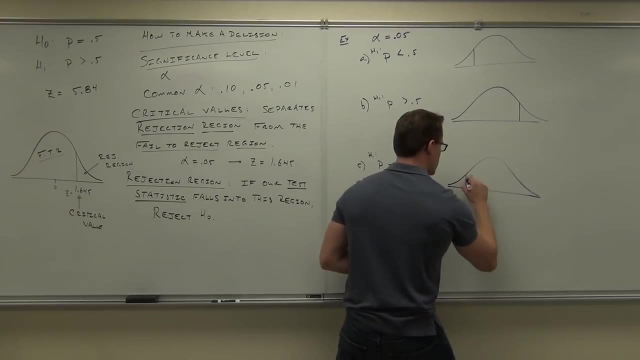 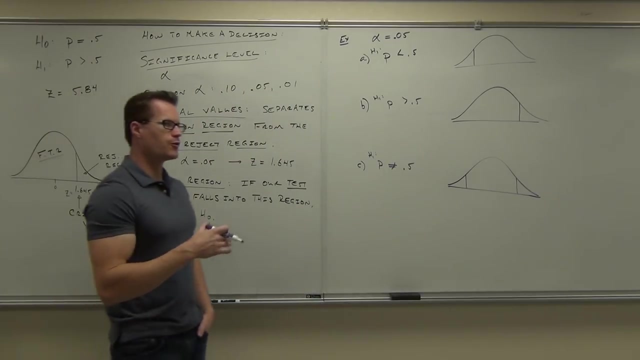 Smaller or bigger says it's not a left tail test necessarily. It's not a right tail test, necessarily. It's a two tail test. It could be either less than or greater than, So we get this Two tail test. Now, if our alpha is .05, that means the area. 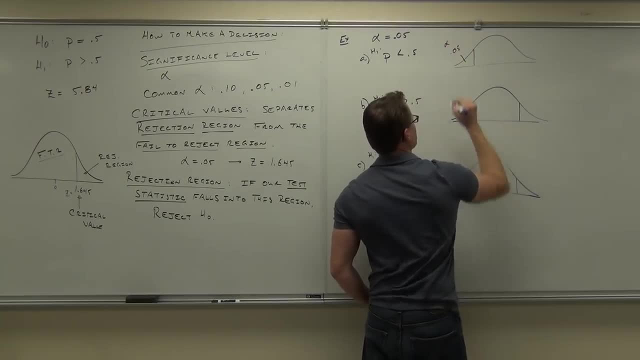 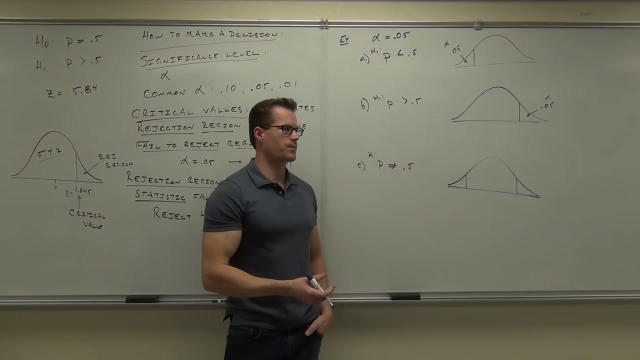 .05., .05., .05. .05.. And each tail for our two tail test is .05.. That's how you're finding your critical values. That's the way it's going to be. However, look up here at the board. 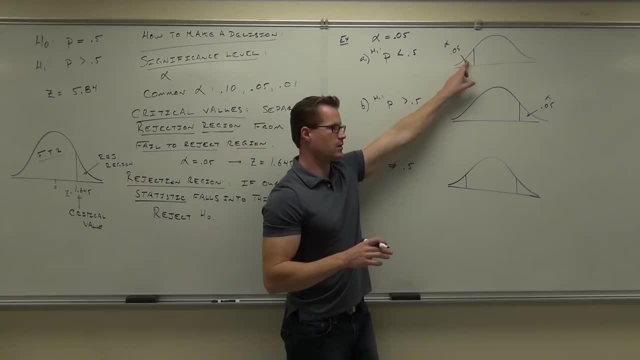 Notice that all of our alpha is in this one tail- You with me, And all of our alpha is in this one tail. How much of our alpha is going to be in this tail? 1.5. 1.5?? yeah sure, because now you're splitting it amongst two tails. this is why you. 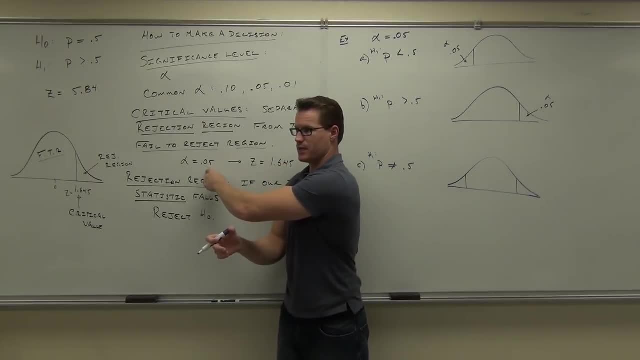 can't memorize this number for this alpha all the time, because if you have one tail, yes, that's what's gonna be, but if you have two tails, it's going to split it. do you get me? it's gonna be different. so, with two tails, well, this is. 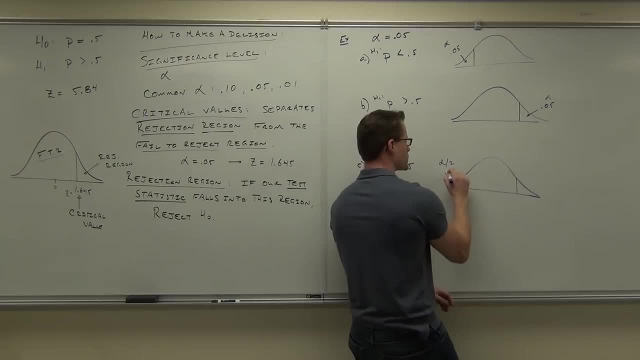 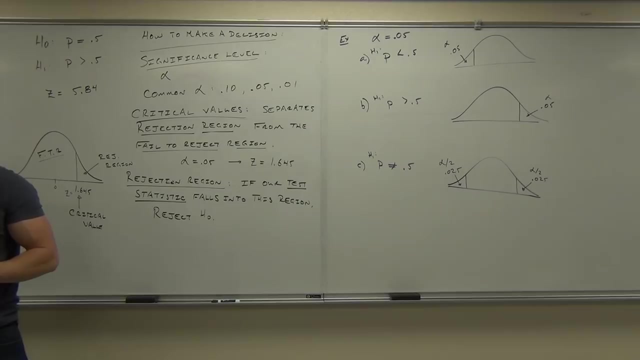 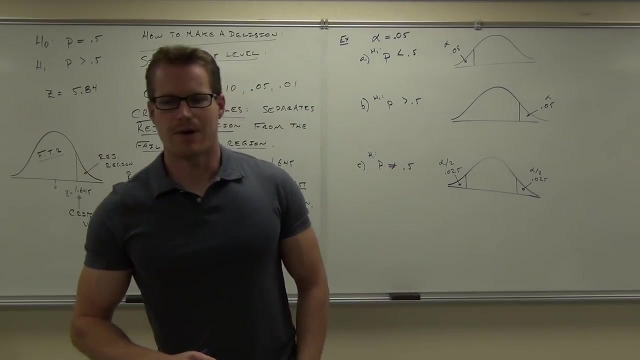 no longer 0.05. this is alpha over 2, or 0.025. this is no longer 0.05. this is alpha over 2 or 0.025. okay, go ahead and take your tables out for me. we're going to verify what these critical values are. so the idea is we're 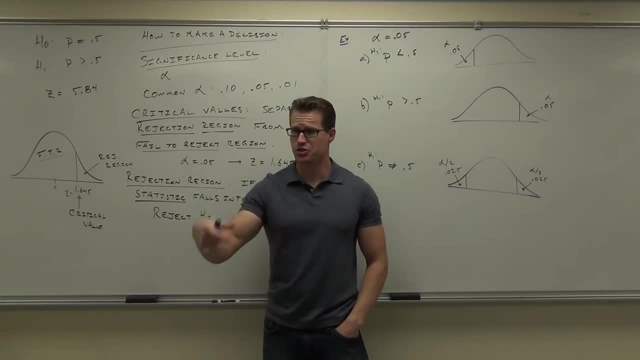 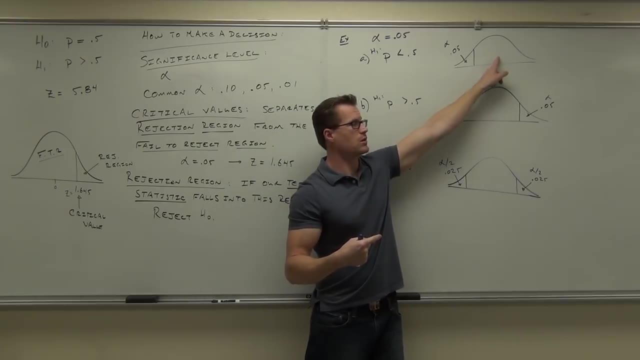 going to look for the number, the critical value that separates the rejected values from the non-rejected values. so we're going to look for the rejection region for us. by the way, can you look at the board here real quick? where's the rejection region here? rejection region- rejection region- yes. 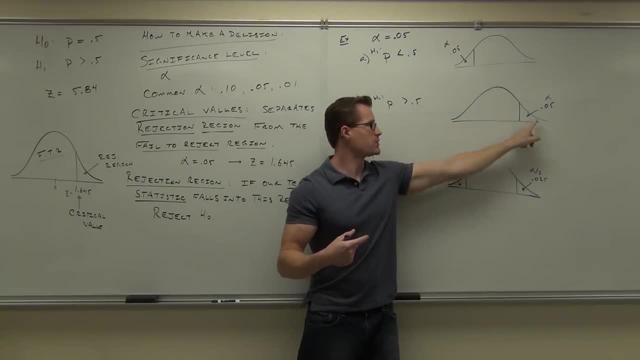 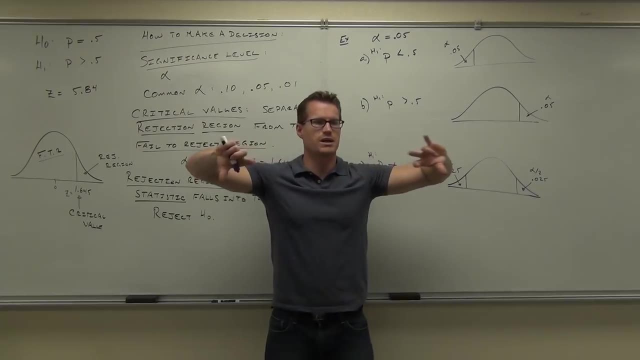 it's always the area in the tails here: rejection region, rejection, rejection region- oh, happens in either spot, because we're looking for something that's equal. so the evidence would be: it's not equal either left or right. that's how we find these out. so go ahead and look at your table, take that out, what we're looking. 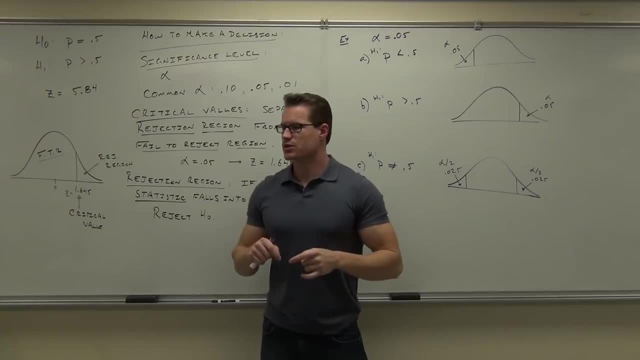 for here is the alpha in the body of your table. so look right here in the middle of your table. you'll be in a negative z-score. you'll probably be there all the time. that's okay. you just have to be smarter than your table. okay, be smarter. 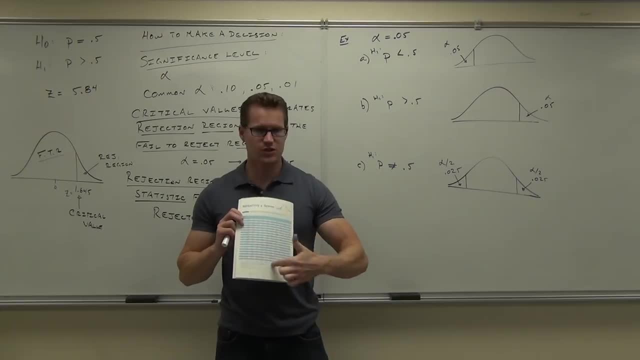 than the table. look here at your alpha. these are alphas. by the way, right here, areas, areas are alphas, alphas are areas. look for point zero five, point zero five, z-score, point zero five. did you find it? it should be one of the asterisks, right. 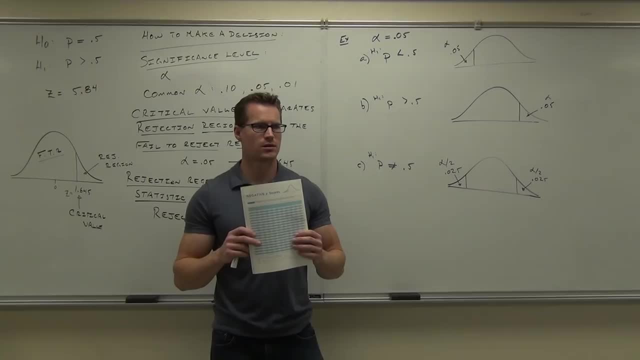 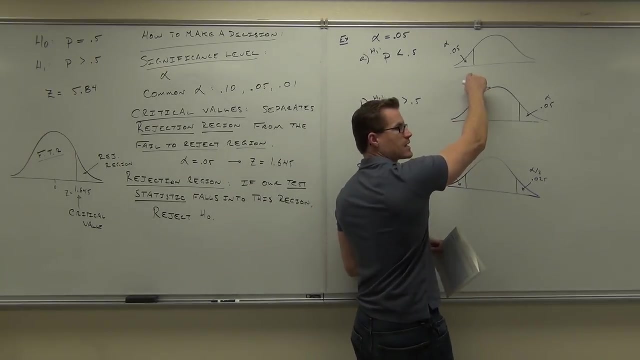 you follow it down and it tells you how much negative one point. this should be old news for you, right? you should be really clear on how to do that. negative one point. six, four, five. look up here at the board. we're talking about left tail test. left tail test will have negative z-scores. you with me on that. this is a 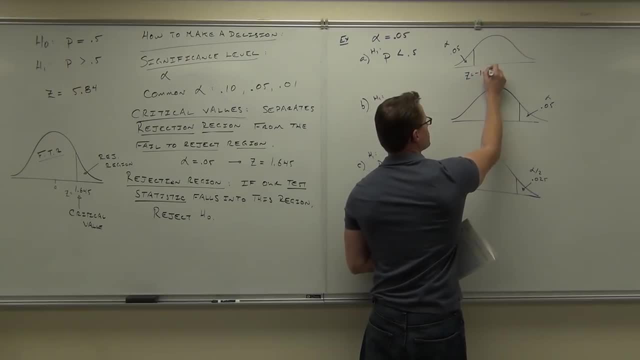 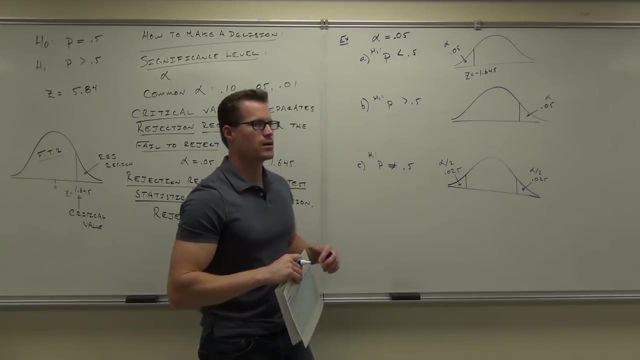 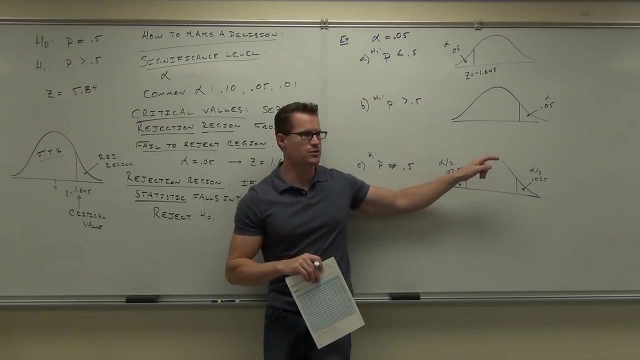 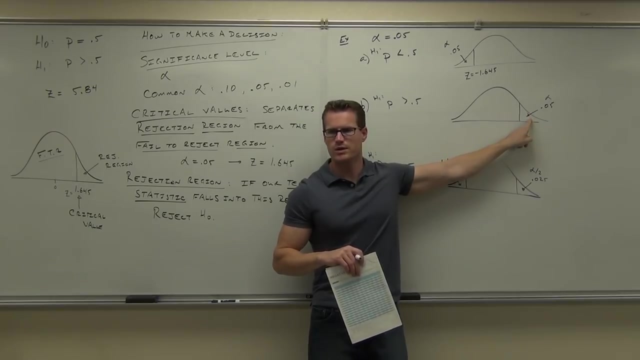 critical value of negative. one point six, four five. that's great. it's a left tail test. now here's an important piece of information. right, go to the next one. go, don't. don't look at your table. you already know the answer. if you look at point zero five here, it's going to give you negative one point six, four, five. 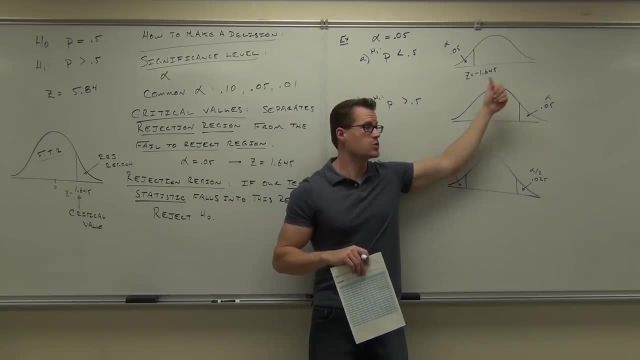 isn't it? well, I hope so, you just. you just looked up point zero five. were you all able to do that? you all got the negative one. point six, four, five. right now, if we're talking about right tail test, though, if you look up point zero five, notice this is talking about the area to the right. if you look at point 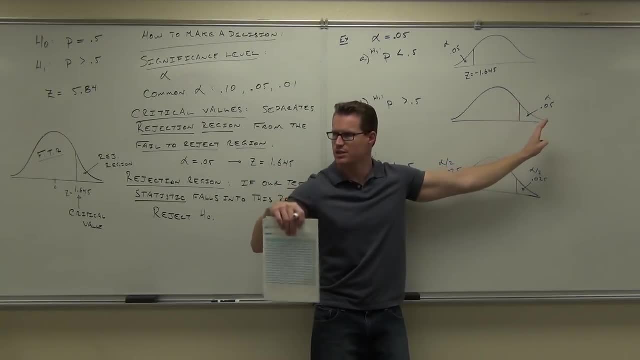 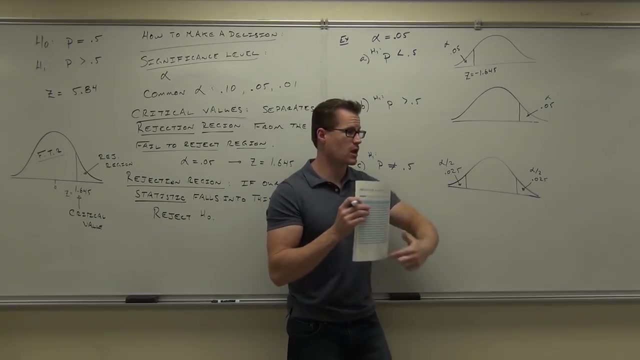 zero five. your table is still going to tell you: negative: one point six four five. is this supposed to be negative? one point six, four five. what is it supposed to be positive? why? what? we're on the opposite side now. so you can. you can do this two ways. your table only gives you the area to the left. it will only look. 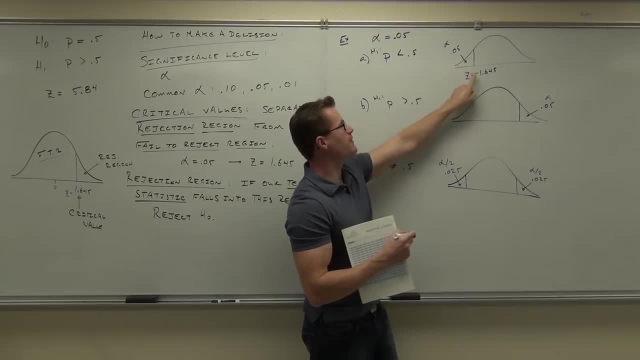 up areas to the left. so you can either look up point zero five, get negative one point six four five. that's the correct way to do it- or you can look at point zero five. you're still going to give you negative one point six five and then change it to a positive, or you could. 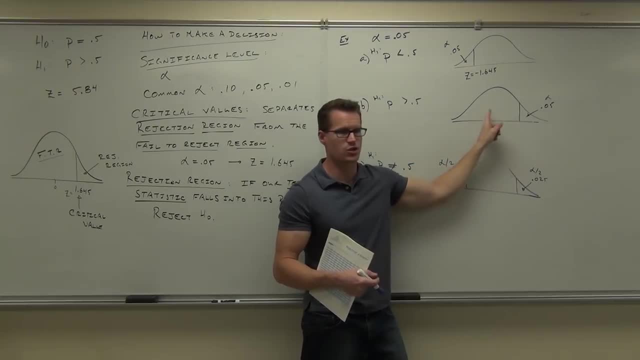 look at point nine five. that's the area to the left. in this situation, are you with me? I'll bet you a billion dollars if you look up point nine five on your table, it's going to give you positive one. point six, four, five you want to take? 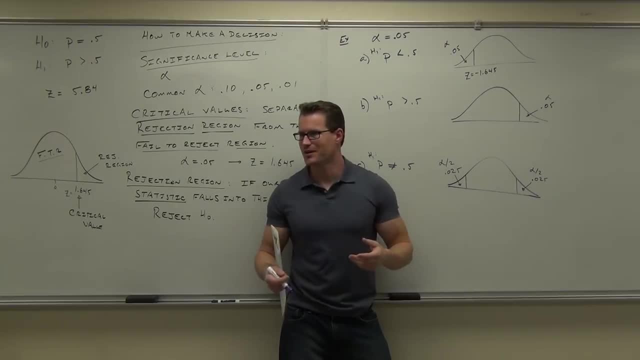 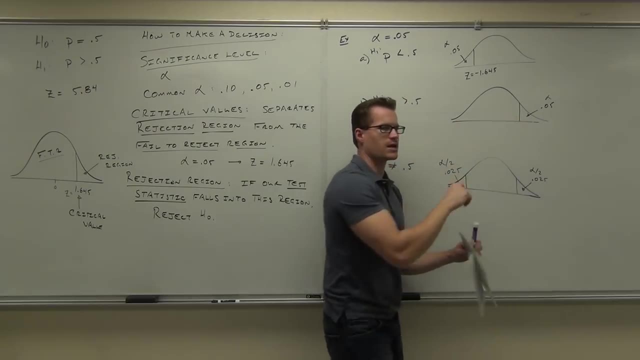 that bet because it's symmetrical. it's perfectly symmetrical. so be smarter than your table, be smarter than this, this information, and know that if I'm talking about a right tail test, even if I look up point zero five, I should have a positive value there. 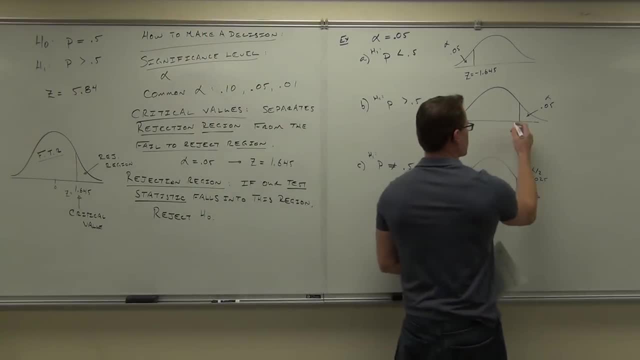 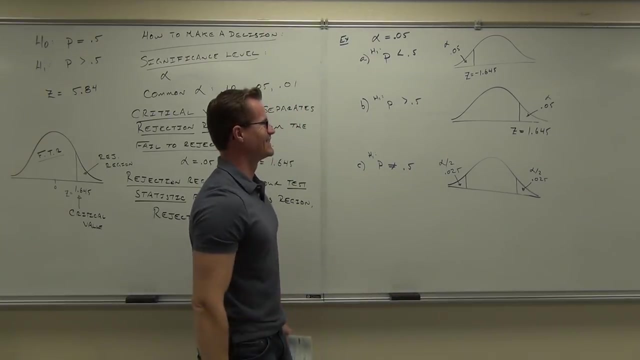 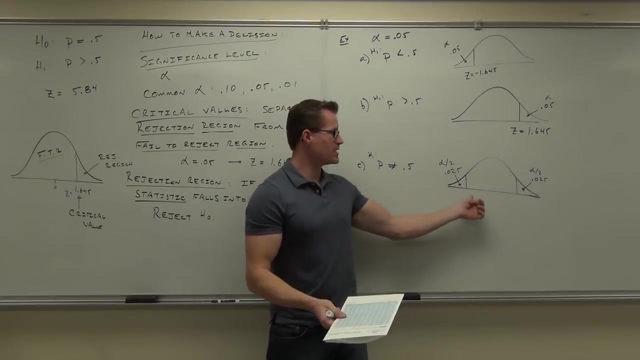 Richard had to feel okay with that. okay, so this is a critical. did you raise your table at me? you raise your? that's awesome. one point six, four, five. do you get it? I get it on table all right now. the most important question all right up here is: is this still going to be negative? one point six, four, five and one. 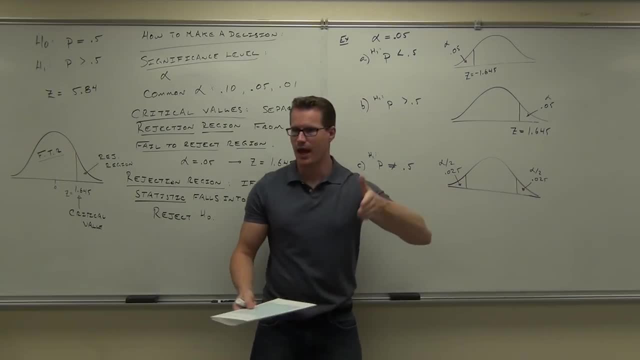 point six, four, five. no, you've essentially cut your alpha in half, so that's why you can't memorize this. you actually have to go through and do these pictures and know what you're talking about. what value are you gonna look up now? point zero, two, five. look that up for me right now. go ahead and do. 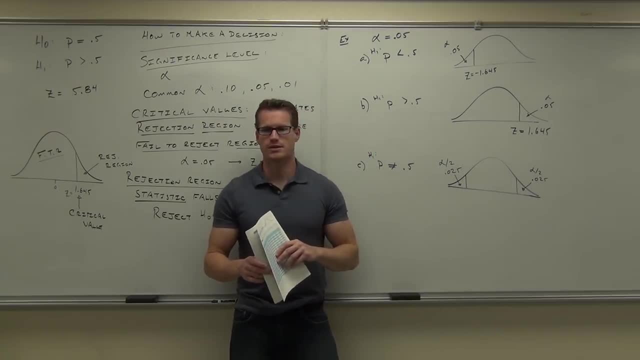 that. this, by the way, is why I put question number two in your last test, seeing if you were able to look up point one: zero, most of you weren't, so this would be a good time to remedy that situation. so you can't do that, you're. 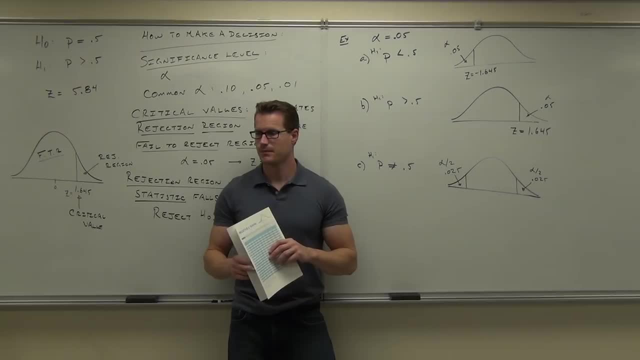 not going to pass this class. you can't do that. you're not going to pass this class. were you able to find it, you should be looking up point zero, two, five, zero. these are all four decimal numbers. so point zero, two, five is not going to be exactly on your paper point. 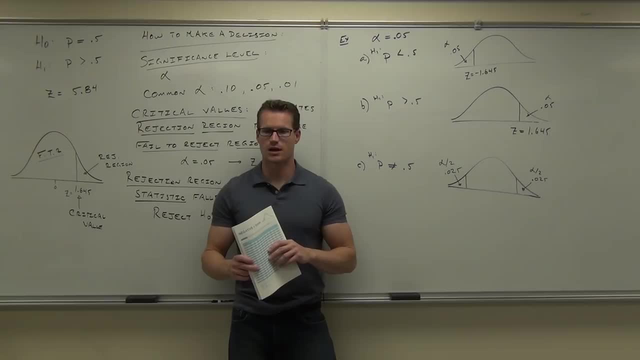 zero, two five zero might be, or if it's not, it's probably has an asterisk- is a very common value. what did it give you? one point nine. let me see one point nine, six, okay, so I'm looking, I'm looking for point zero. oh, there it is. point zero: two five zero. it's listed right there for me. 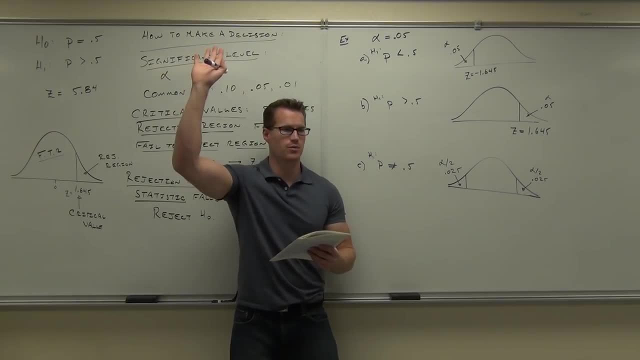 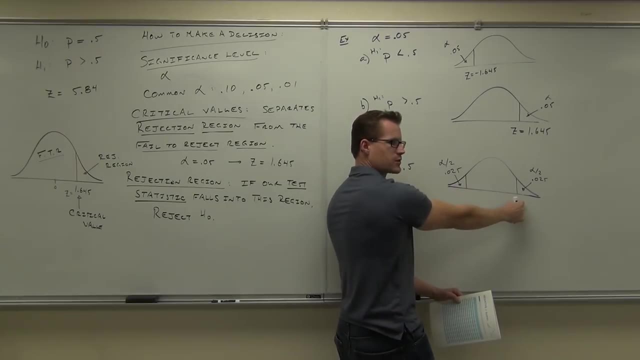 I'm seeing negative one- point nine six. how many people were able to find negative one? point nine six. good for you, that's fantastic. okay, now is this the negative one? or is this the negative one, the left or the right? so we have one critical value of negative one. 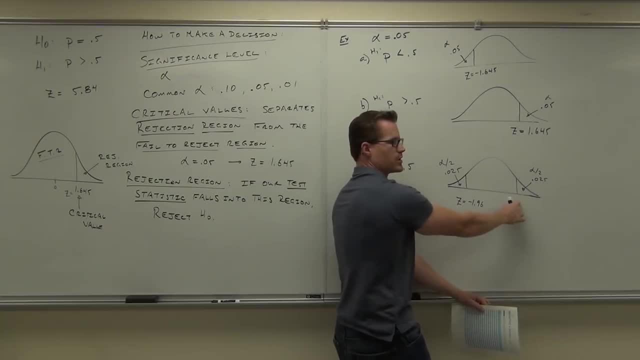 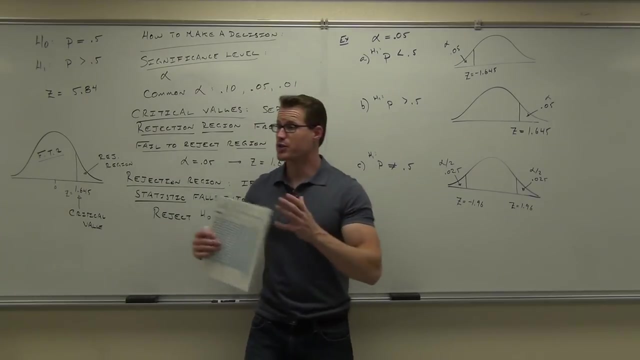 point nine, six. hey, how about this one? what do you think that one's going to be positive? yeah, it's a symmetrical chart, which is nice. so this, right here, this tells you where your rejection region is. that's why our critical values are so critical. they're critical for us to know those things. 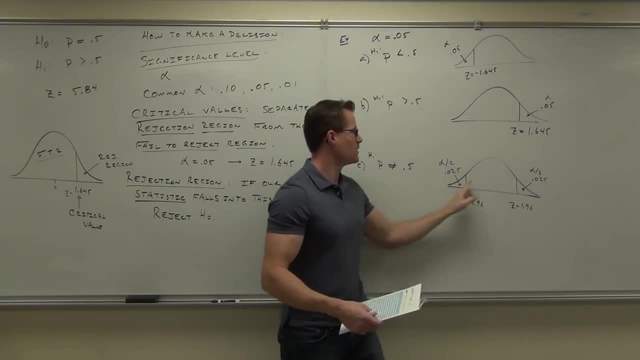 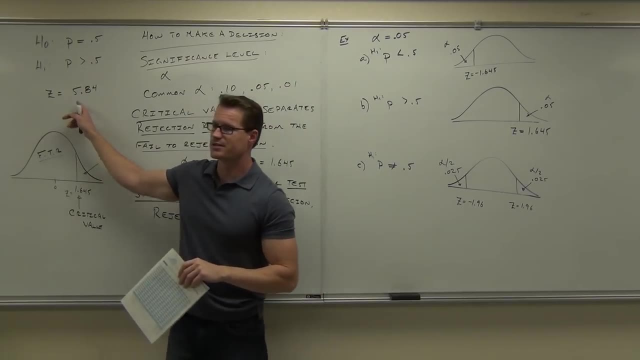 because that separated our rejection regions from the fail to reject region. and that's how you make decisions with hypothesis testing. you look to see where this number falls, your test statistic. if it falls in your rejection regions, you reject. if it doesn't cool, then you don't. so let's go N ngày. rất có lịch. 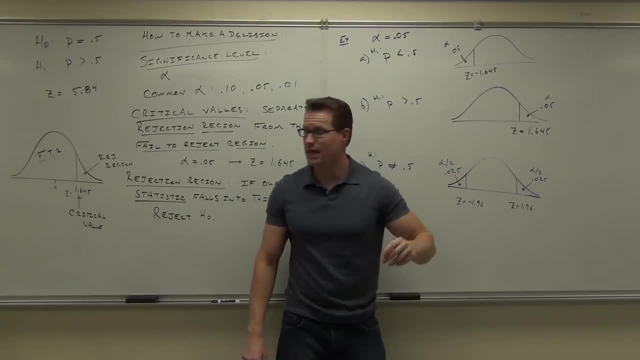 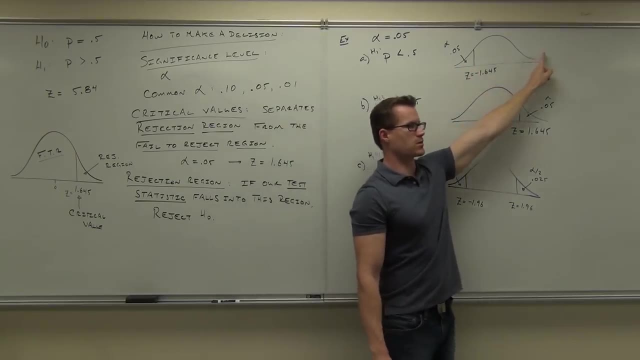 page và để nhớ, Metro padding rained five point n notable 五偏. Is it in the rejection region or the fail-to-reject region? for this Fail-to-reject It's way over here, correct, And this is my rejection region. 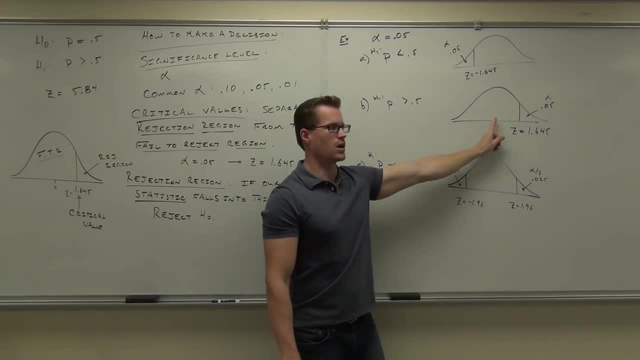 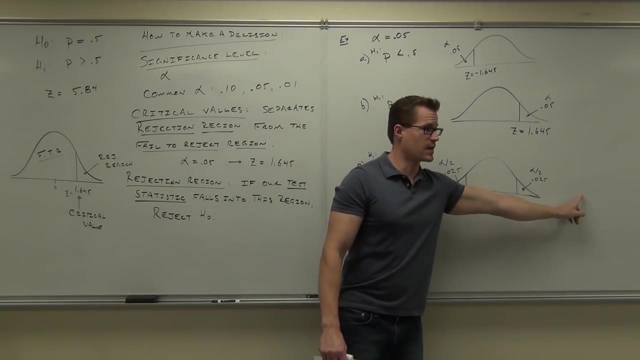 You would fail to reject in this case. How about this one- reject or not Reject, Definitely reject, It's in the tail. How about this one- reject or not Reject, Definitely reject, It's in one of the tails. 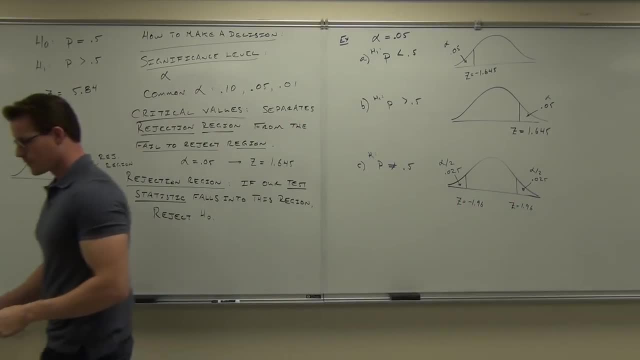 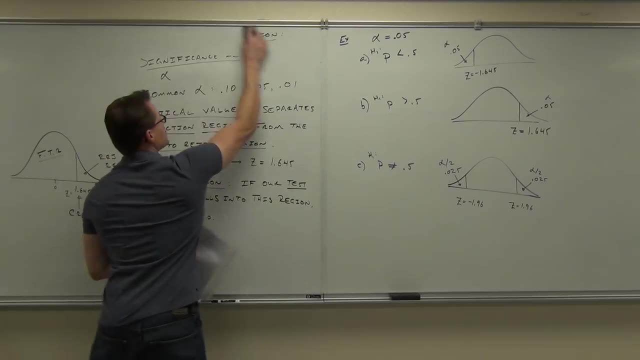 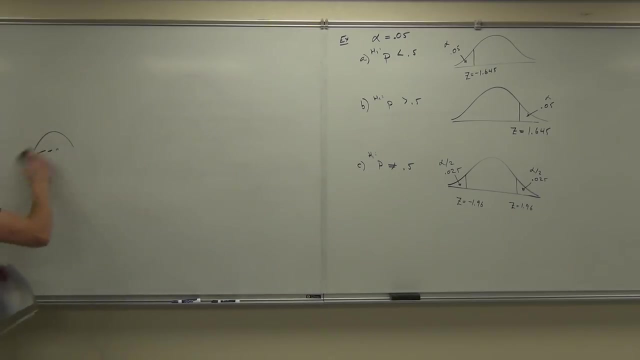 This one doesn't matter which tail you're in, as long as you're in a tail, Okay. so there's three situations that we have. I'll write this out in general so you can have not just a specific case, but something that you can follow up each time. 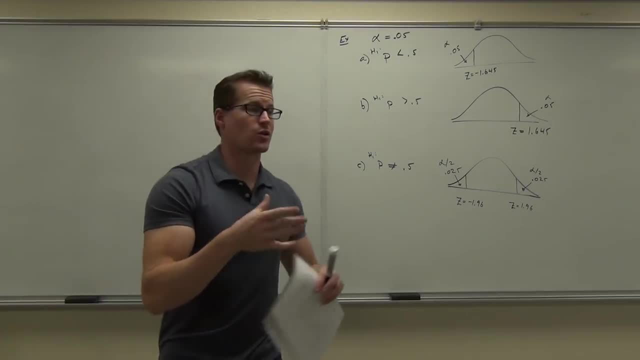 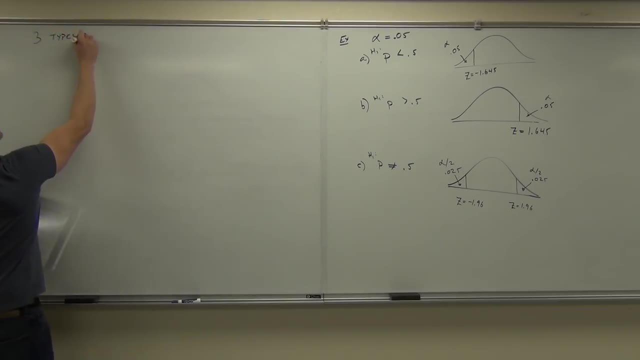 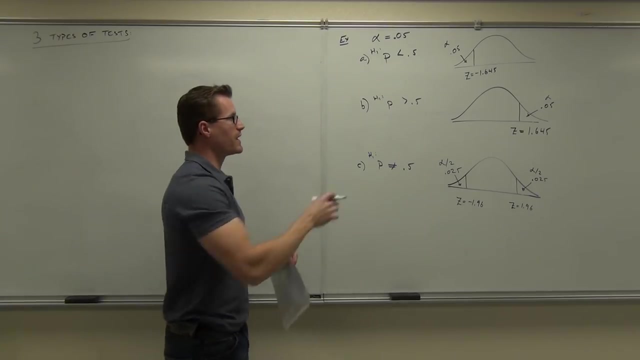 There are three types of tests. They're all determined by H sub 1, your alternative hypothesis: Three types of tests. every single one of them is determined by H sub 1.. That's where you're looking, here and here and here. 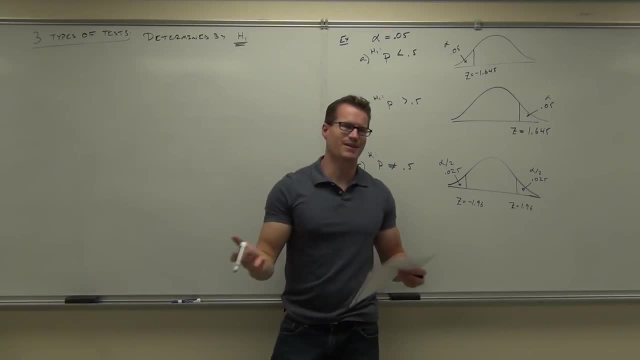 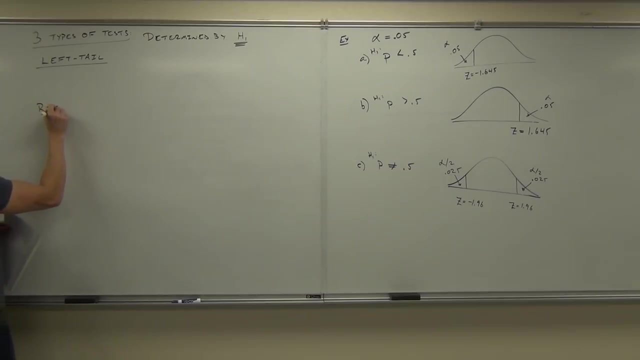 It can't be determined by H sub 0, because H sub 0 always has an equal sign. That doesn't help us out at all. It's always determined by H sub 1.. There's an option for a left tail, A right tail or a two-tailed test. 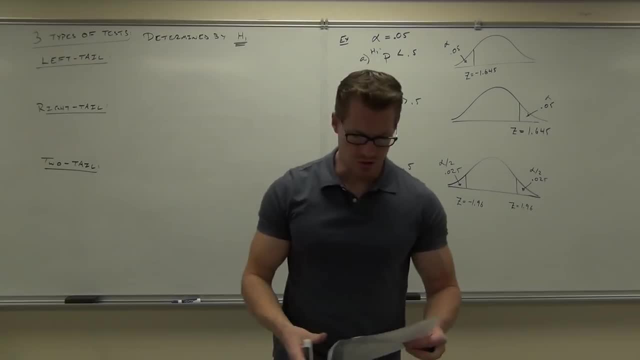 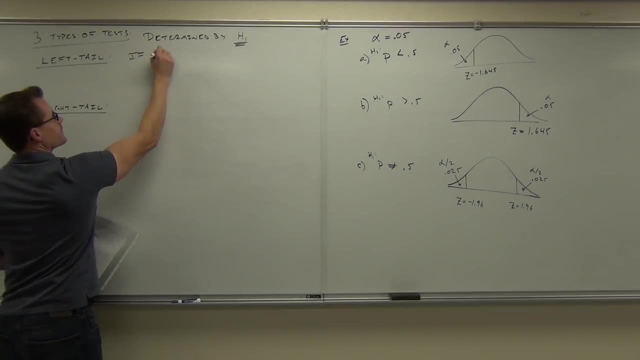 It's going to look exactly like what I have on the board. I'm just writing it out in general so you see it every time. So a left-tailed test. If H sub 1 has this sign that less than If H sub 1 has less than, it will be a left-tailed test. 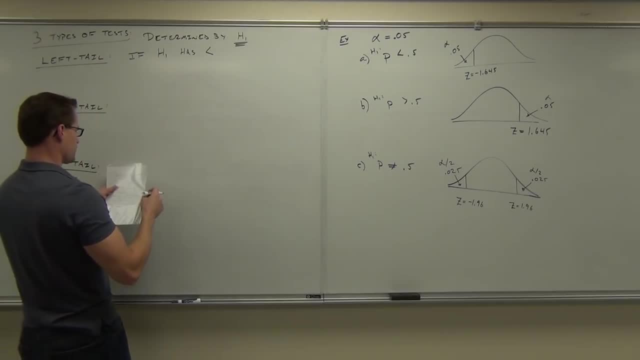 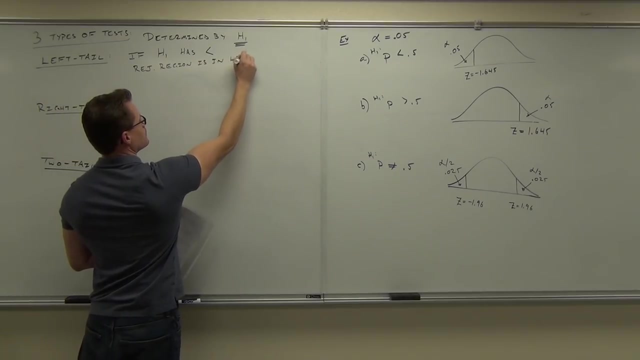 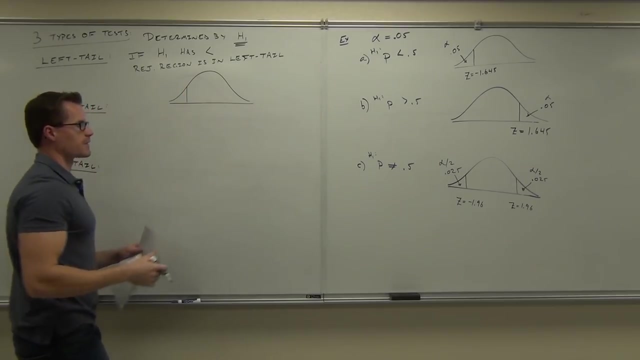 Left, less, less left. So it has that less than The rejection region is in the left tail Depression region The rejection region is. with that point I'll try to do an� shower So this goes away And then we go over it again. 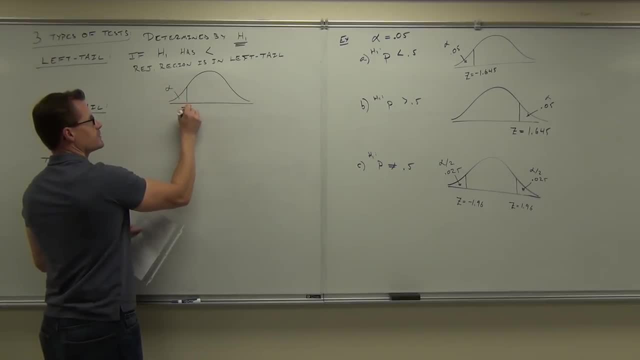 It's still not. It has to go. This would be alpha. this would be negative z. A negative critical value is what that stands for. That's where we're going to fill out this form So it won't show up in the table. You can move it over and all you need to do- what we're going to do- is look at it So straight You would stop watching. It's actually going to be something like a negative. I don't have a specific stop. It's not there. 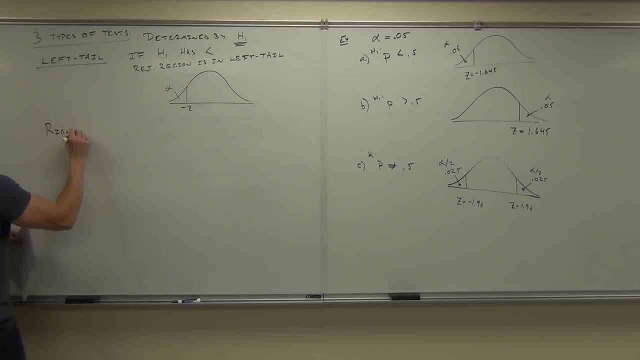 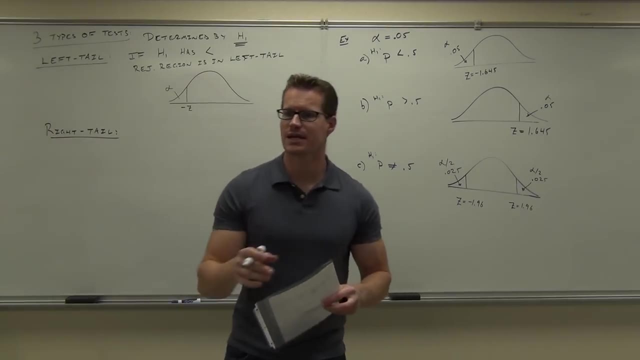 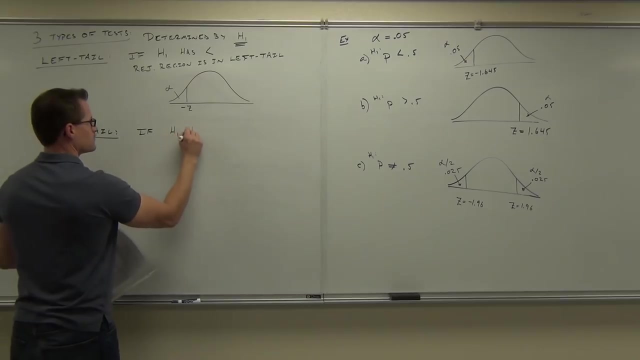 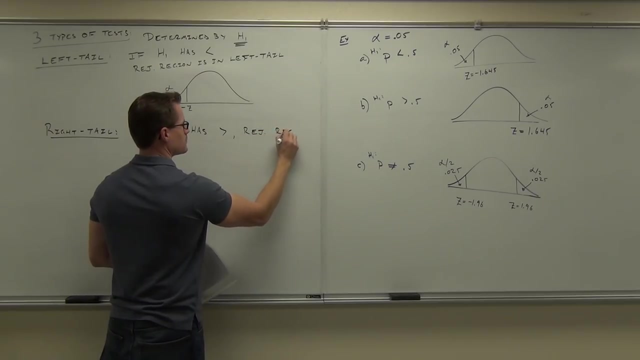 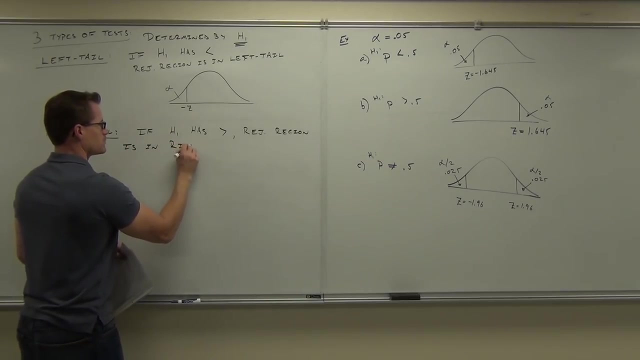 It's not there. If we have the other case, if H1 has a greater than, that's going to be a right tail test saying that the rejection region is in the right tail- It would say: okay, the rejection region is in the right tail. 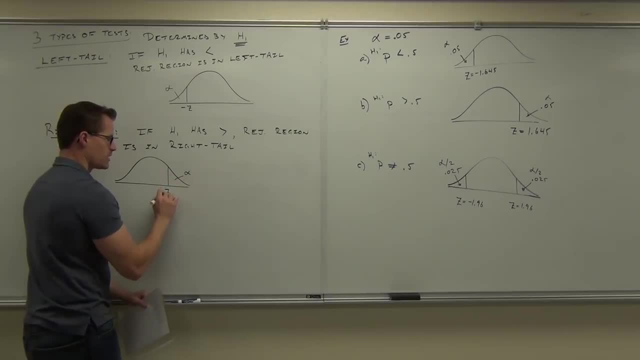 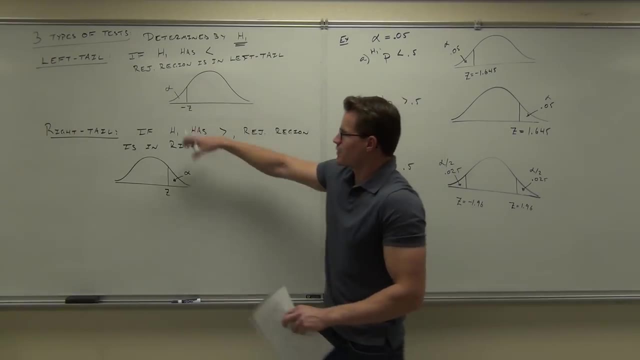 The rejection region is over here. That's given by our alpha and this will be a positive critical value, a positive Z. So for either case, you look up your alpha right. You look up your alpha all the time. So if you look up your alpha and you know it's a left tail test, you keep it negative. 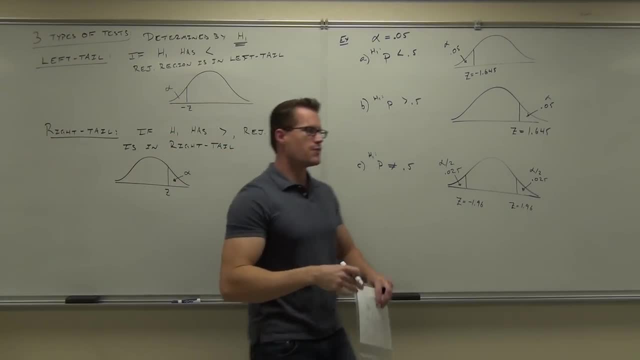 If you look up your alpha and you know it's a right tail test, you just make it positive. If you look up alpha when it's split in two, you take the negative and the positive, because that's a two-tail test and that's our last one. 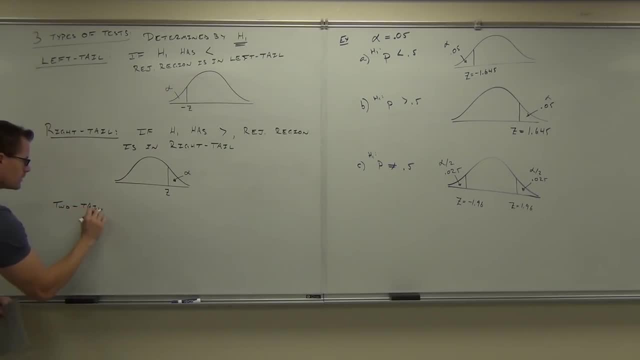 If H1,, our alternative hypothesis, has a not equal to. those are the only three options. the rejection region is in both tails. that gives us a two-tail test. Okay, However, the alpha is split amongst them, so you have half your alpha to the left. 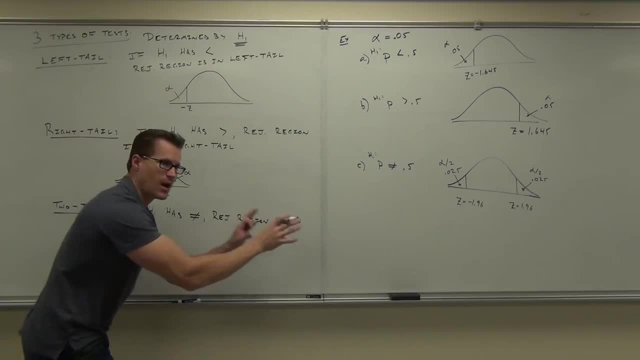 and half your alpha to the right, And that's really important that we get that down. It's not the same alpha that you would have in a left and a right tail test for the same significance level. So you've got two now, two critical values separating your rejection region. 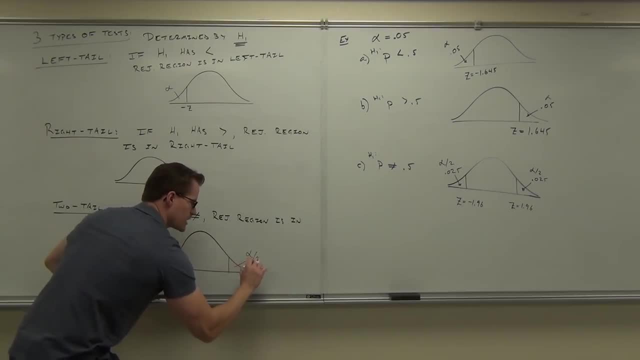 which is in both tails. so since it's split amongst both tails, you have your alpha divided by two for the right And same for the left. This will be a negative Z and a positive Z, but this is based on alpha over two. 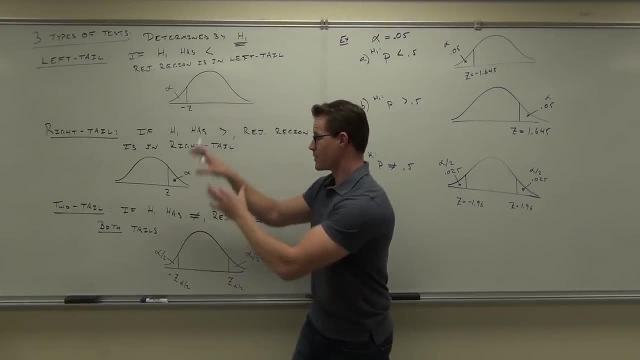 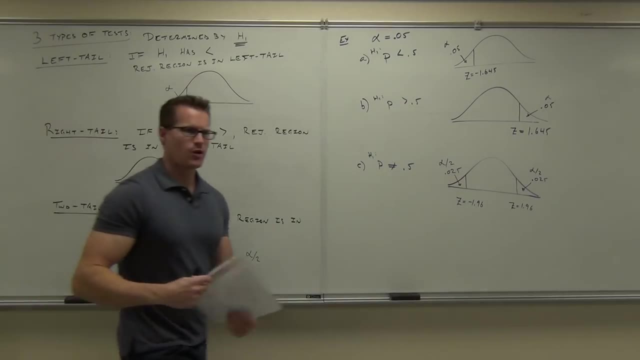 not the alpha that you had at the very beginning. It's not the significance level from the problem, but the significance level split in half. That's where that's coming from. Would you raise your hand if you feel okay with these examples? I'm trying to make this real clear for you so you understand where this is coming from. 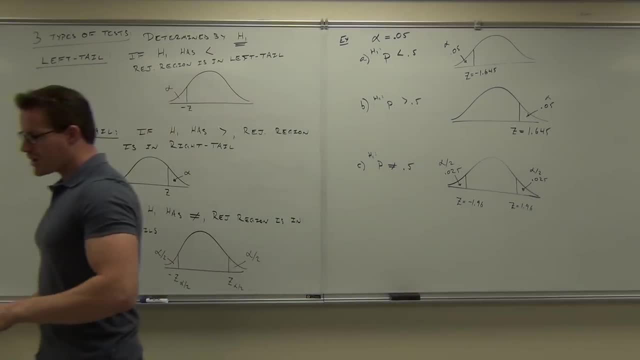 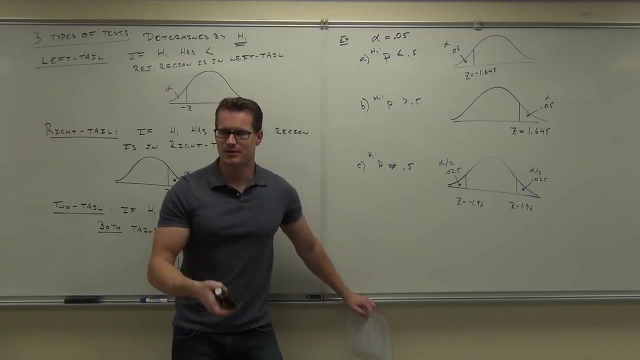 That's why we did that one as a specific example. first, There's one more definition that I've got to show you before we, before we do any sort of anything extra. This can be very confusing for people, because I'm going to use another letter: P. 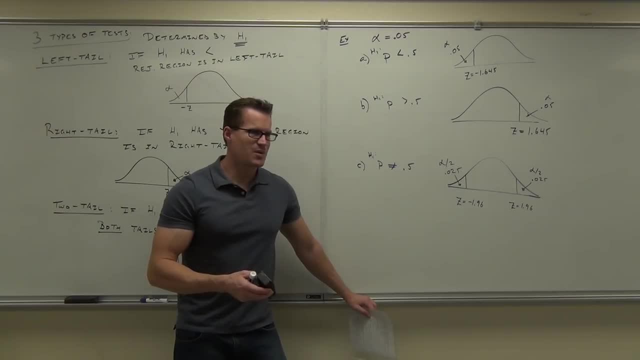 I know I've used lots of letter P's in this class. all right, The letter P- I'm about to use it- called a P value. It's an uppercase P. It stands for the probability. It is not based on a proportion. 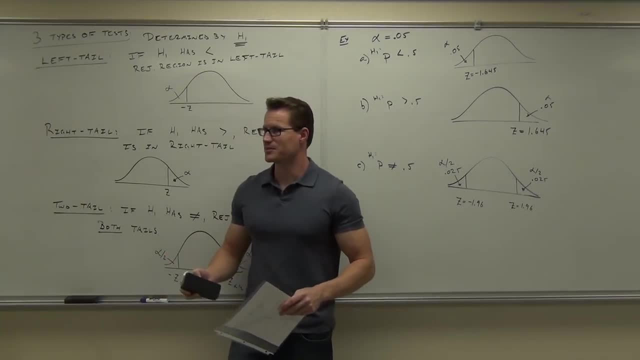 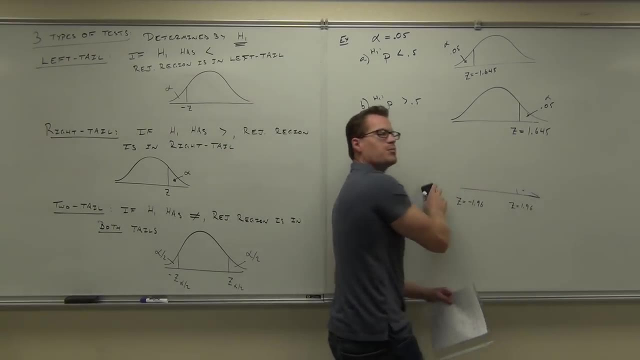 So this letter P is not the same as this letter P. I know that's confusing, because letter P's can stand for lots of different things. all right, This P is not a proportion. It's not based on a proportion. A P value is a probability value. 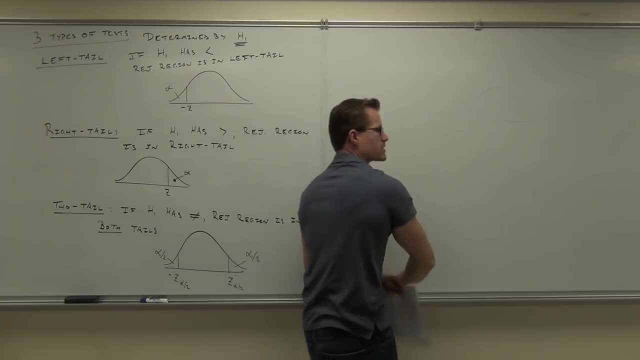 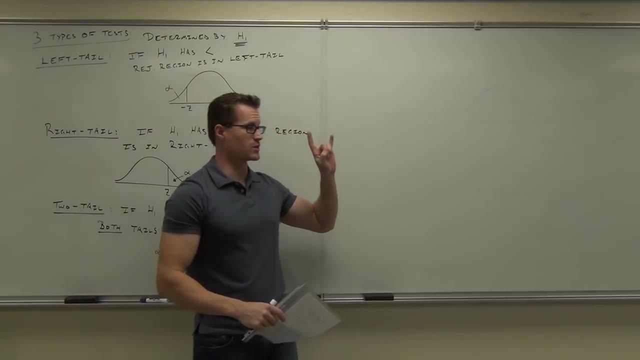 So what we're talking about right now is not a proportion. You can use a P value type of test to do what we're talking about. You see, we're going to talk about two methods for hypothesis testing: The traditional, which is what I just showed you, and the P value method. 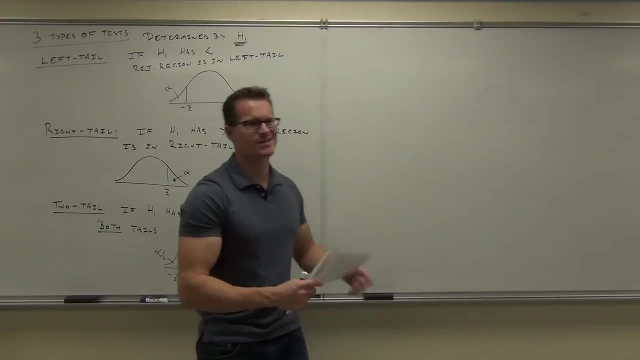 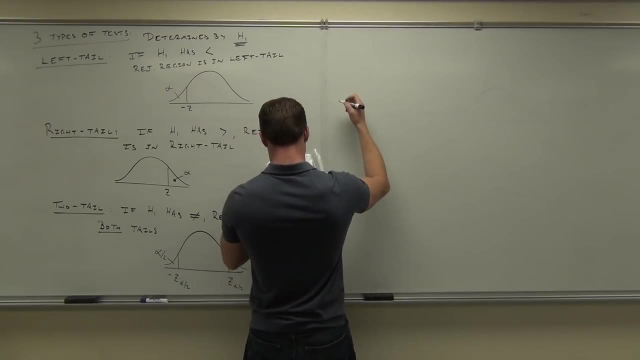 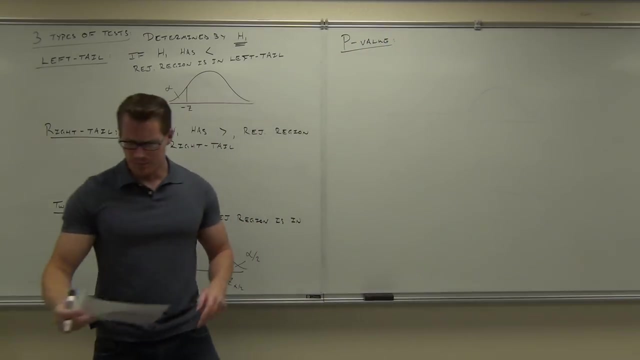 which is a slightly different way to approach it. It's becoming more and more popular. Statistics changes over time. This is becoming a more popular way to do things, So I'm going to show you both. So capital P value stands for probability value. 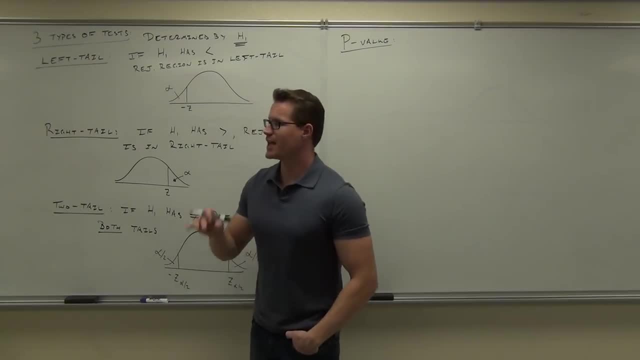 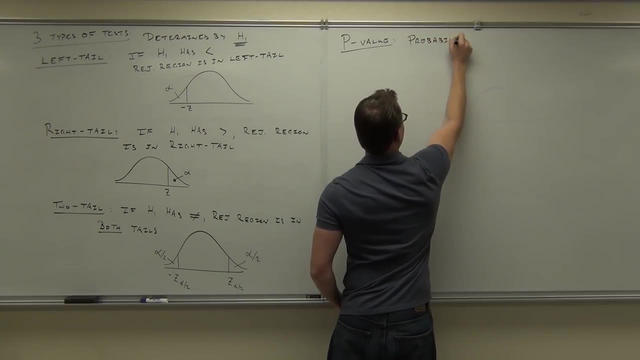 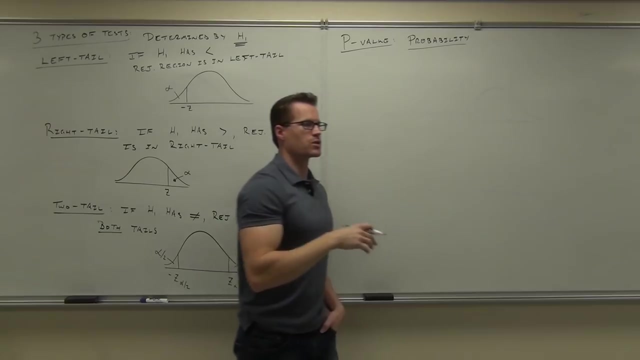 And what it is. it's the probability that's associated with your test statistic. Is it a proportion? No, No, no, no, it's a probability And it's associated with your test statistic. That was the 5.84 thing that we used. 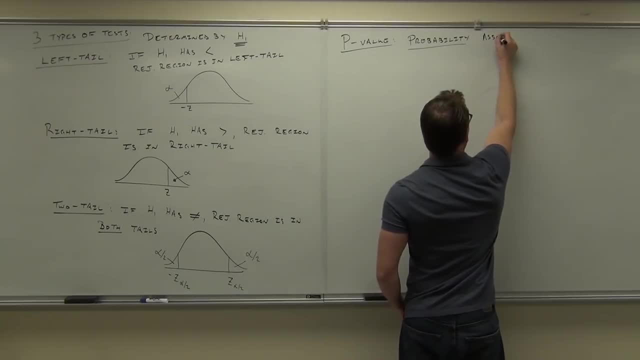 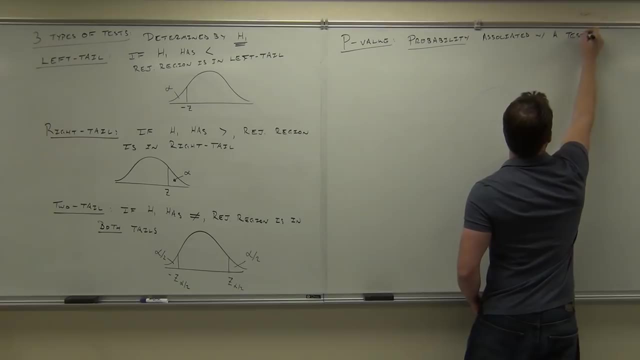 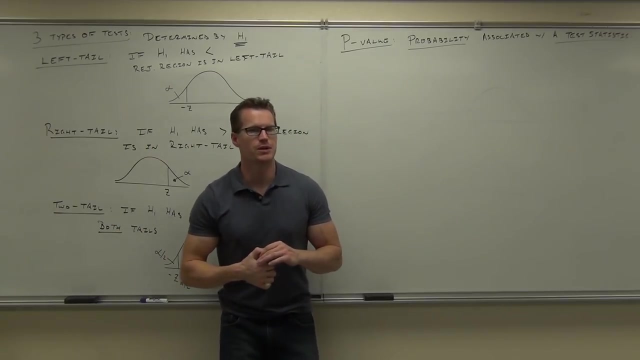 We found out. You see, I'm going to give you a little preview of what you do here. There's two ways to do hypothesis testing. The first way method, What the traditional method does, is this. Please watch carefully, I'm going to kind of explain it, give you an overview. 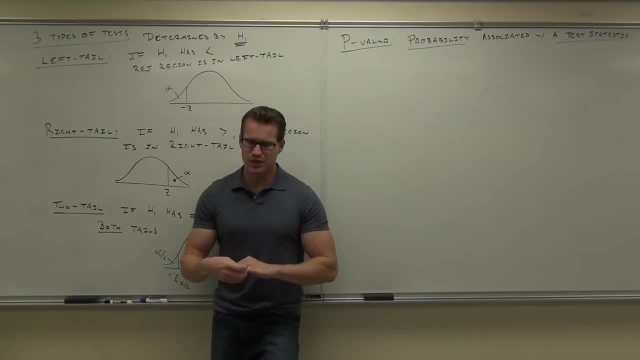 and then I'll be much more specific as we go through the next section. The traditional method does this. It says you look at your significance level and that's going to give you, based on a left tail, right tail or two tail test your critical values right. 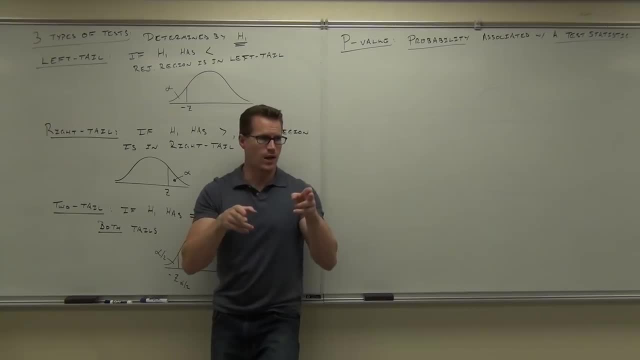 And it separates your rejection region either two or left or right tail- And then you look at your test statistic and you see where it falls. You follow me on that. This way, the P value method does something a little bit backwards. 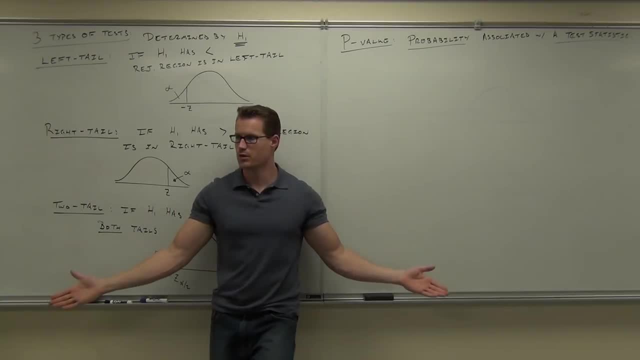 It says you're not going to worry about critical values. no critical values. It says: all you have is your test statistic and you're going to put that on your chart and you're going to find out the area in the in that particular, for that particular value. 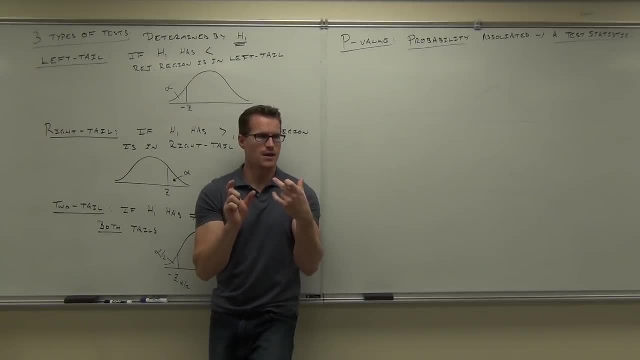 Then you compare it directly to your significance level. If it's smaller than your significance level, you know it's rare enough to reject the null hypothesis. So there's two ways of looking at it. Traditional has critical values and you look what your test statistic. 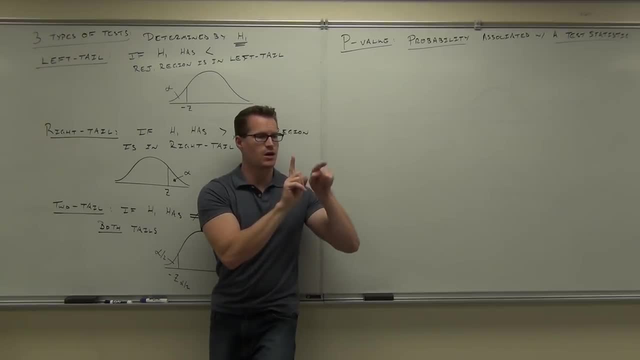 you know it's going to be false. P value says you take your test statistic, look up the area- which you guys are very comfortable doing, you've done it before- and you compare that area to the alpha. If it's smaller, you reject. 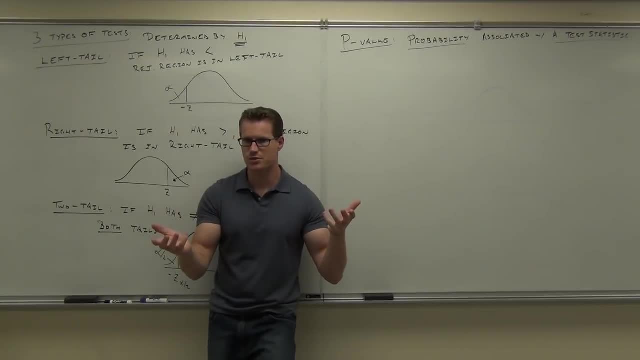 If it's not smaller, then you don't reject. That's. that's the two options you have for hypothesis testing. You need to know both, so I'll teach you both, because I'm going to ask you specifically for one method or another on your, on your test. all right? 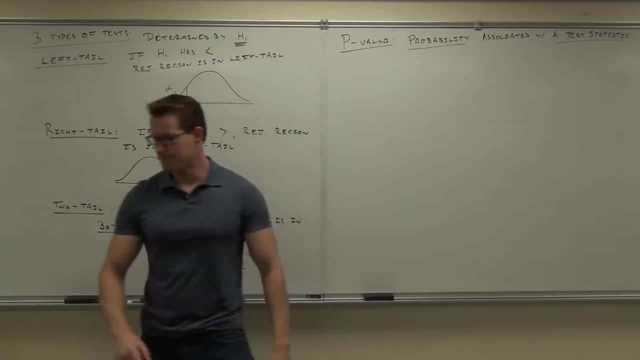 So you you do have to know both of them, So I'll let you know. there's two ways to go about it. Okay, so P value: it's a probability associated with your test statistics, and I just just talked about our decisions that we can make. 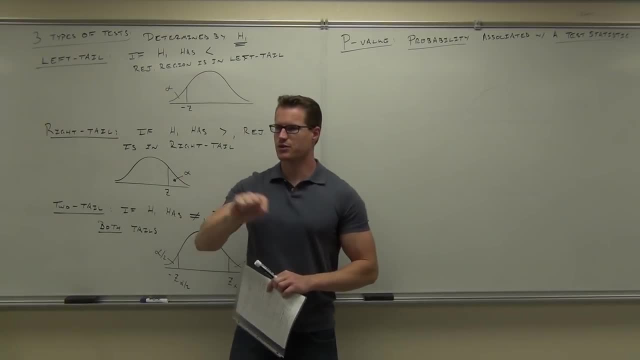 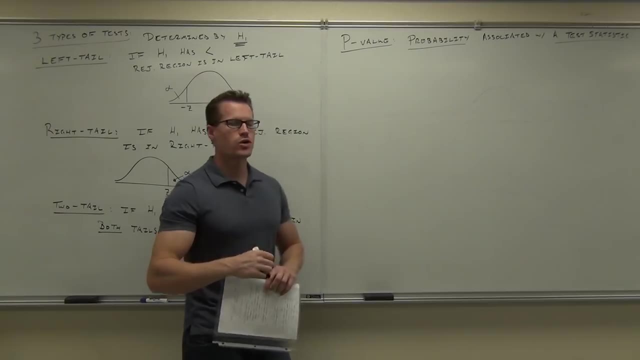 Decisions. there's only there's only two options. The decisions are: you reject the null hypothesis if it's in the rejection region for for the traditional or if the P value is less than the alpha for P value method, or you fail to reject the null hypothesis. 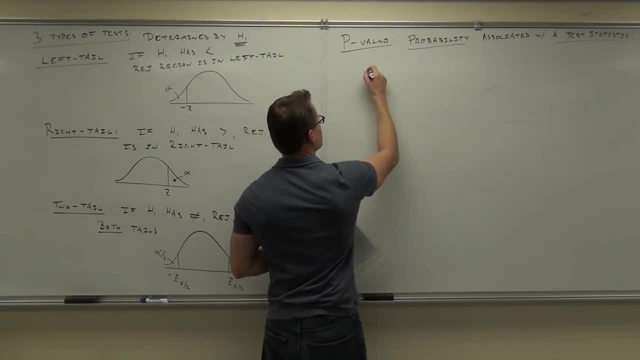 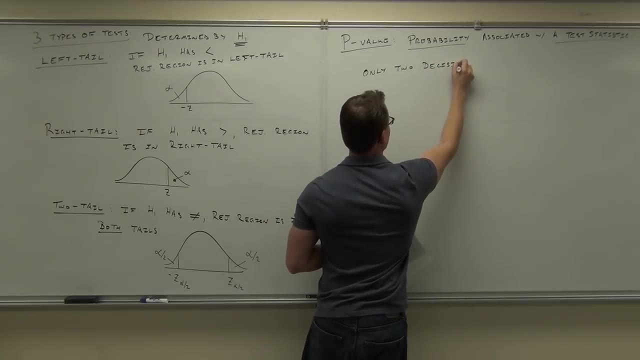 You can't ever accept it. Those are our only two options we can have. So only two decisions. they're not really decisions. you don't get to decide, so I'll decide for you based on the math. You just have to be able to do the math correctly. 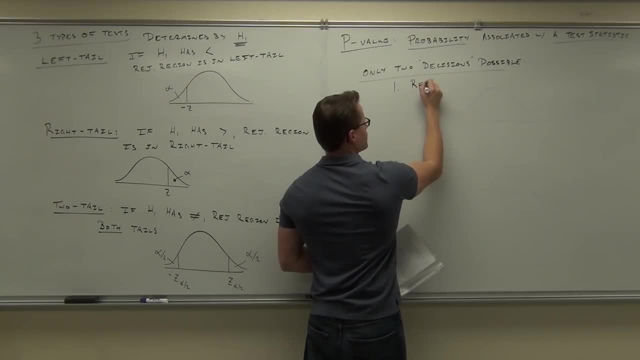 One: if it's in the rejection region, you are going to reject H of zero, the null hypothesis. Two: if it doesn't, if it's in the fail to reject region for traditional method, you fail to reject it, Okay. 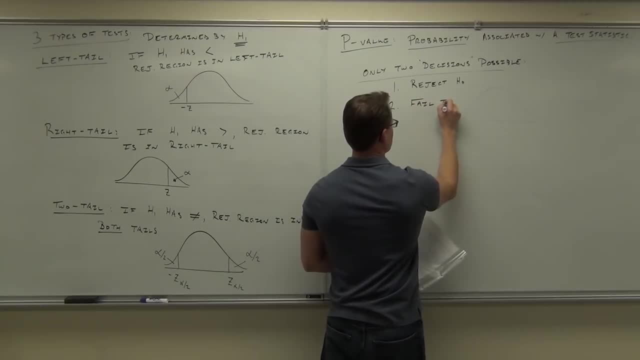 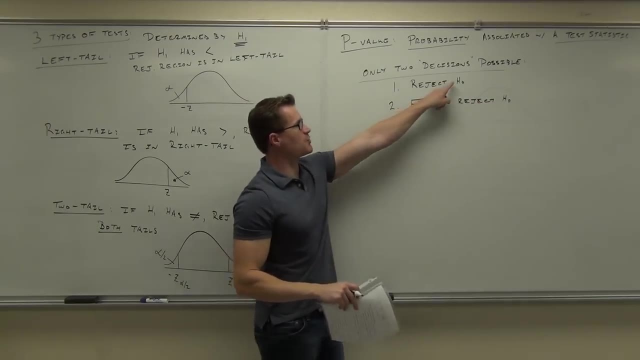 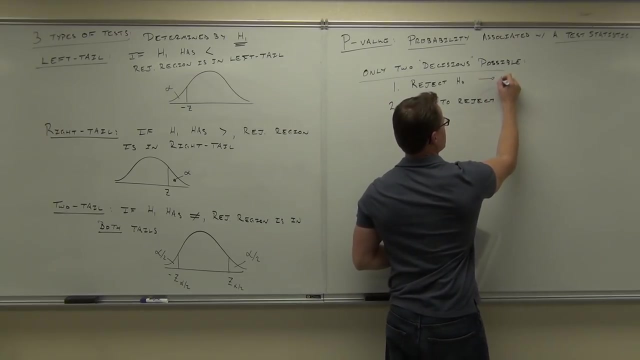 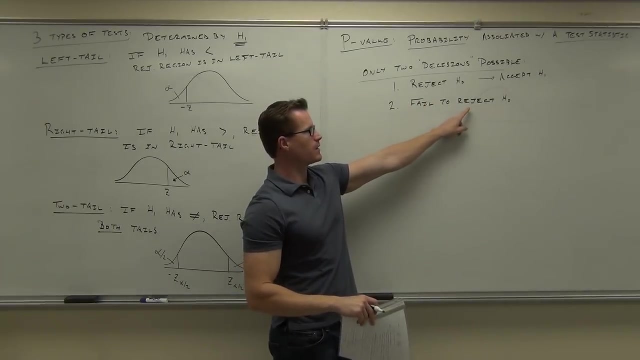 So you're going to have to do it In this case. if you reject H of zero, you accept H of one, This one. if you fail to reject H of zero, can you accept H of one? still Remember these statements that I said? 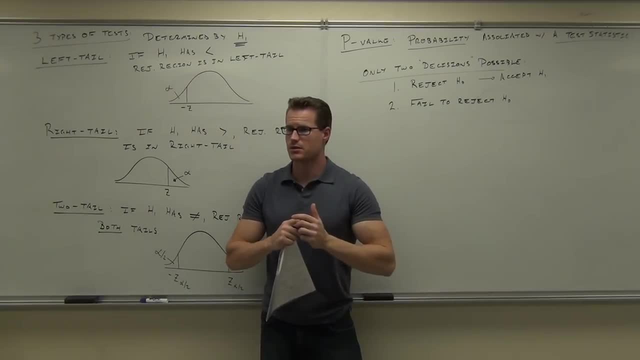 that I had up on the board: the H of zero and the H of one. they're opposites. They're opposite statements. right, It means that if this one is, if you reject H of zero, it means it's clearly false. 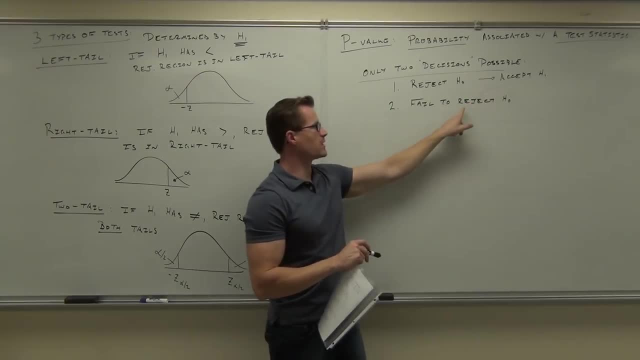 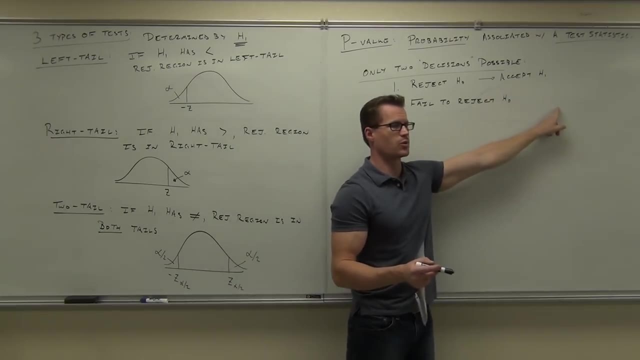 If it's clearly false, it means this one's clearly true. If you fail to reject H of zero, it means it's not necessarily false, but it's definitely not necessarily true. Can you say anything about H of one, Then you can't say anything about anything, then you're done. 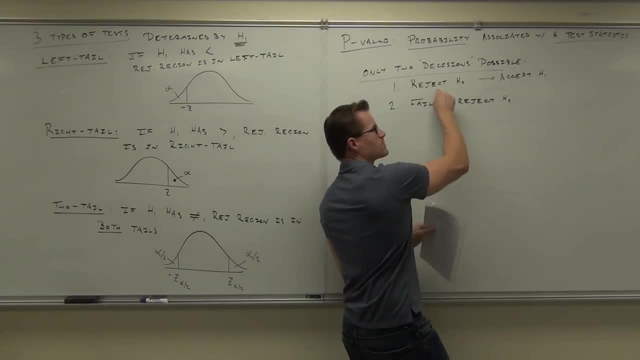 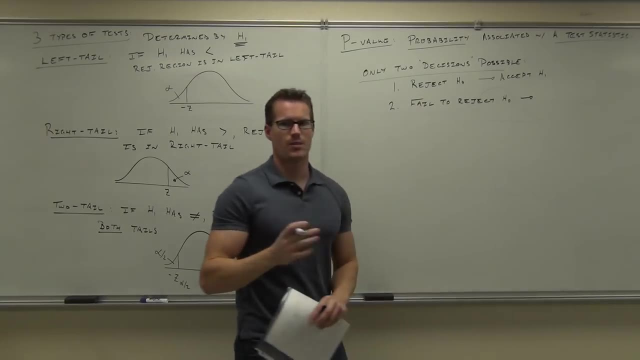 There's no decision on this. So if you reject H of zero, you do accept H of one. If you fail to reject H of zero, you do accept H of one. If you reject H of zero, you don't know anything about your statement whatsoever. 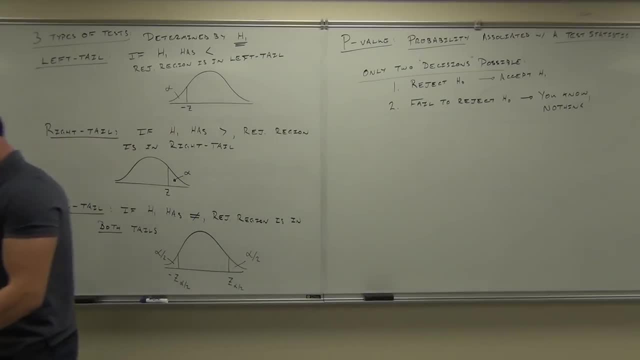 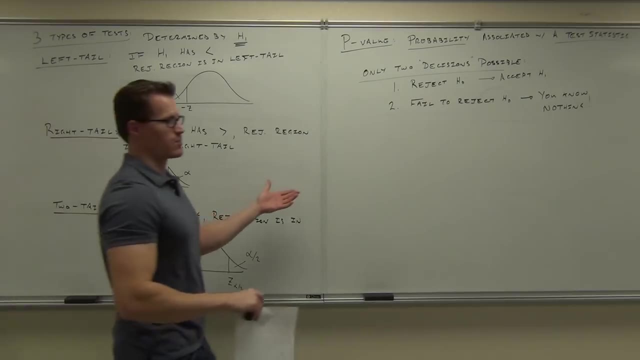 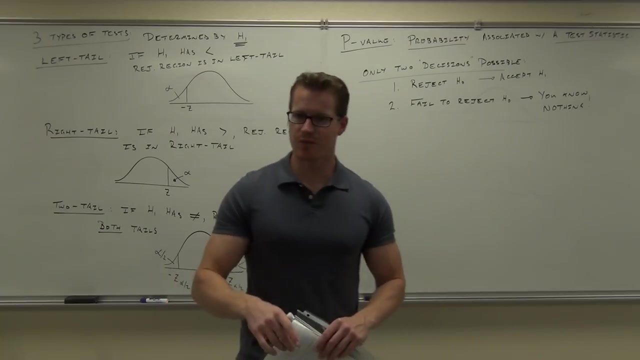 You know nothing. Love that one Can't prove it right, can't prove it wrong. you're stuck. Now I'm going to put on the board what I was talking about just a minute ago: The traditional method versus the p-value method. 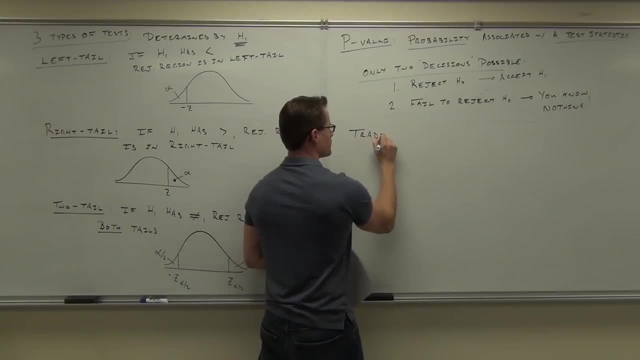 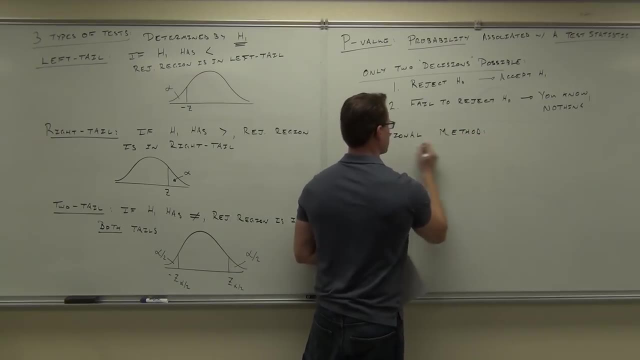 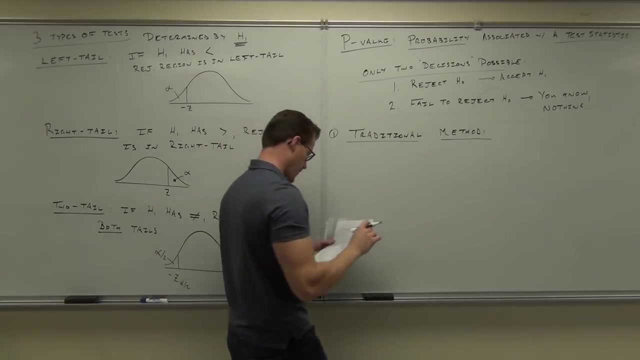 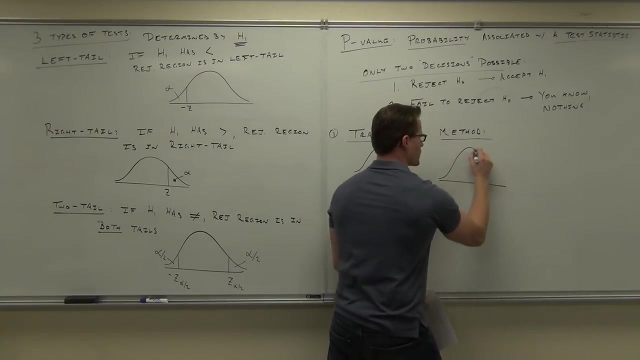 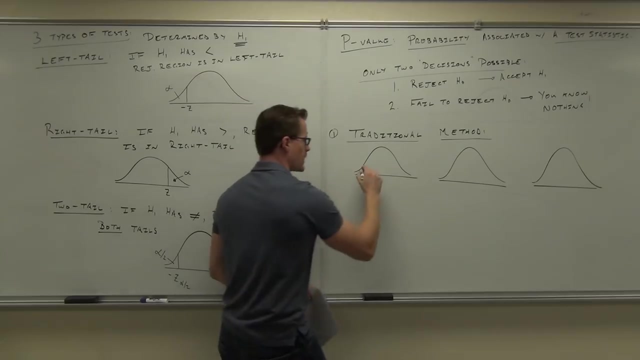 Here's the difference. if you want to see it, Traditional method does this. It will take and your three possible options here that we talked about on the left-hand side of the board. It will take your left tail or your right tail or your two-tail test. 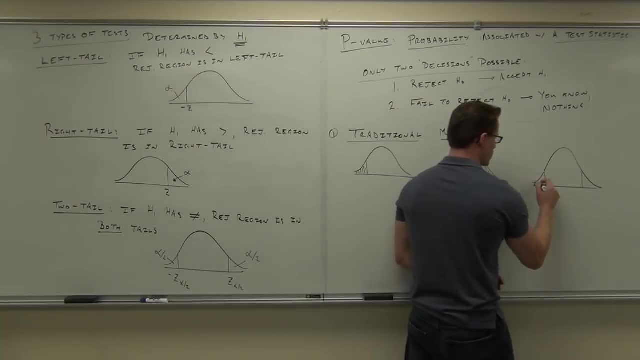 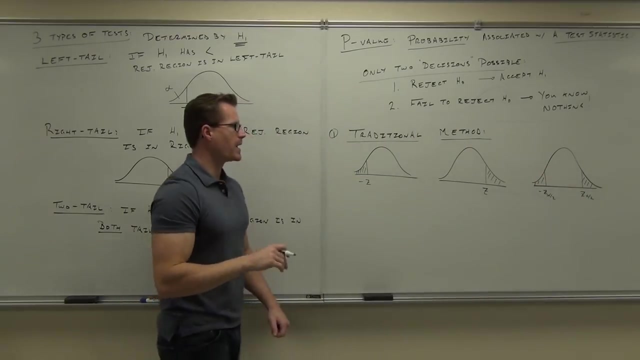 And it will give you some sort of rejection regions here, With, of course, a negative critical value or a positive critical value or two critical values, Depending on your type of test And what the traditional method says is you take your test statistic. 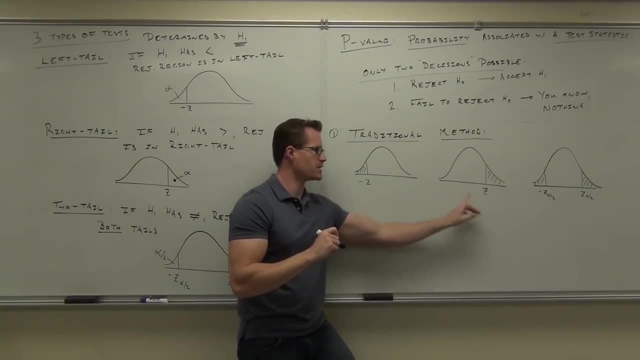 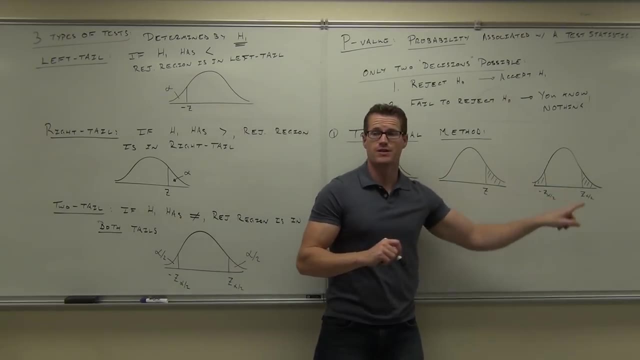 Look up here at the board with me. You take your test statistic. These things are not test statistics, they're critical values. You take your test statistic and you see if it falls in your rejection region. If it does, you reject H of zero. 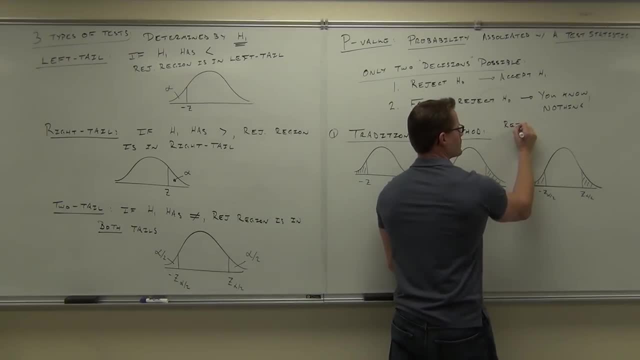 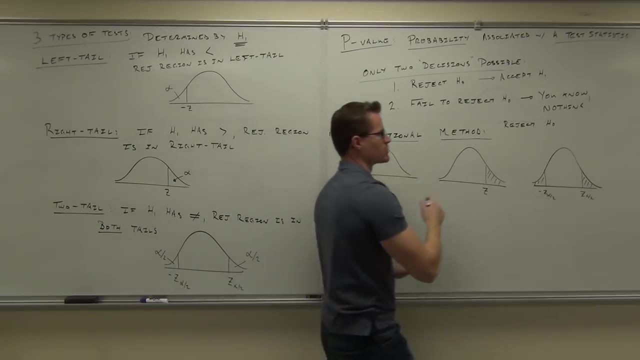 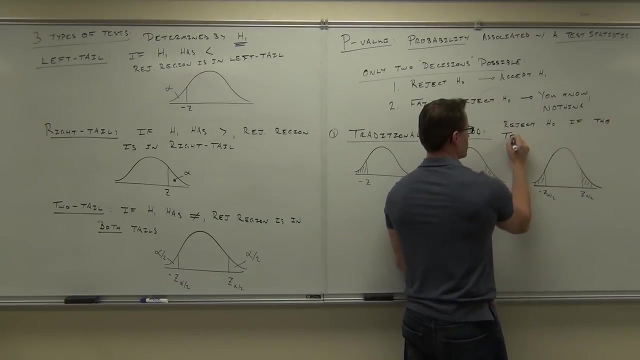 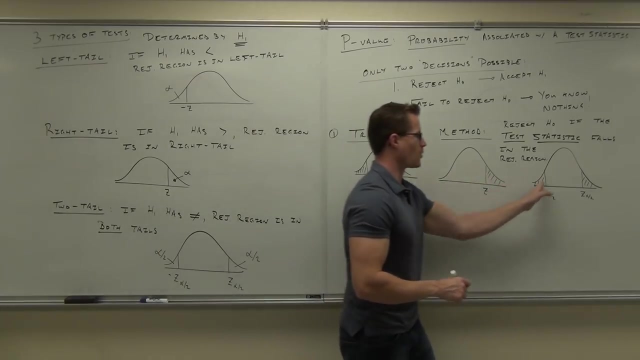 So I'll put up here What we're doing is: you are going to reject H of zero. reject H of zero if the test statistic falls in the rejection region. Thank you very much. Reject H of zero: if the test statistic falls in the rejection region, it would be here or here, or in one of those two spots respectively. 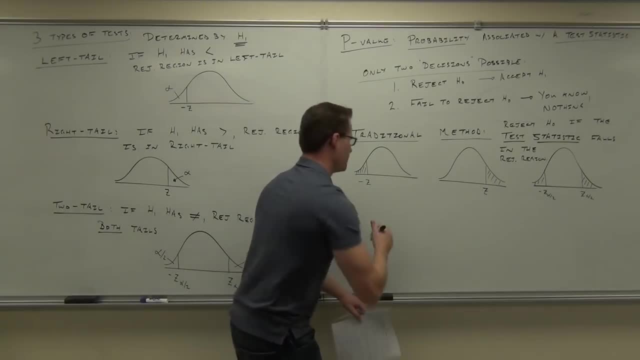 P-value method is the opposite way of looking at it. They're both equally valid. There really is not a whole lot of difference between well, there's no difference in the mathematics, it's just what you're looking up changes. P-value method says this: 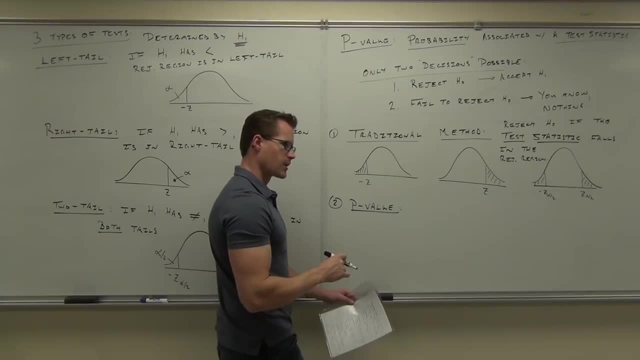 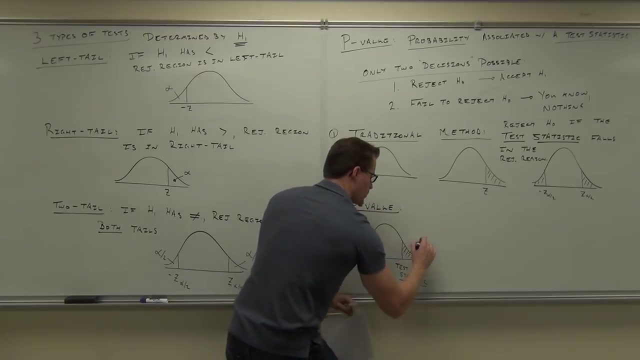 You compare the P-value to your alpha. so what you would have here, based on your left-tail, right-tail and two-tail test, you would have a test statistic And you would look up that area. This area would be your P-value. 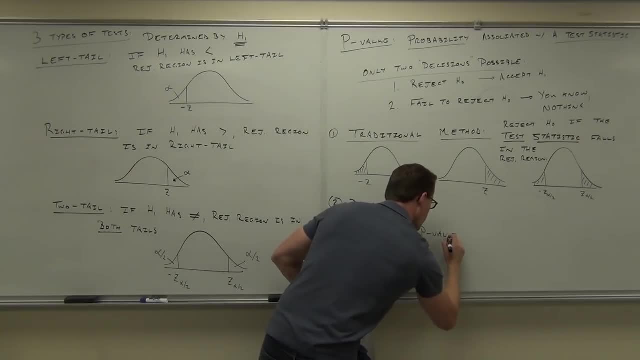 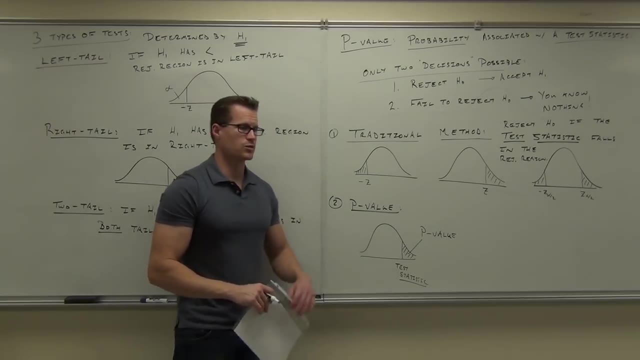 That's a weird U. That area would be your P-value, So notice how the pictures. they look very similar, don't they? Only? in your traditional method these are critical values. Here you would have a test statistic. You could still have a right-tail, a left-tail or a two-tail test. 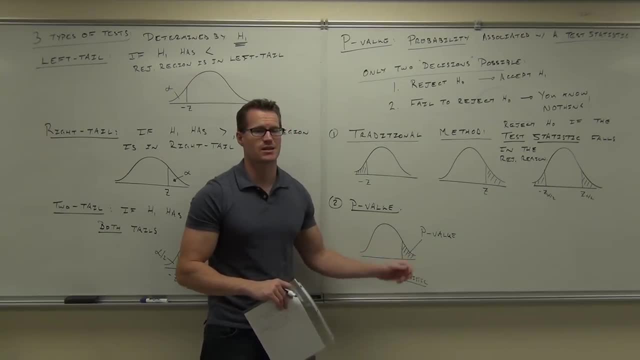 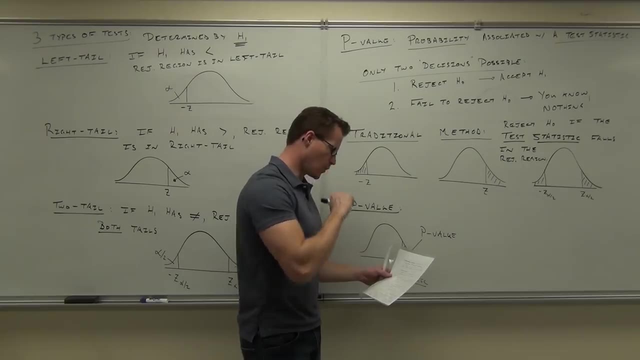 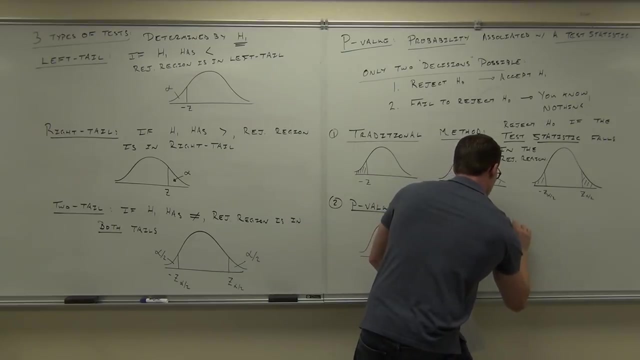 But now you're looking up the area that's associated with your test statistic, that's a P-value, And then you reject your H of zero. if the P-value is less than or equal to alpha, You fail to reject H of zero. 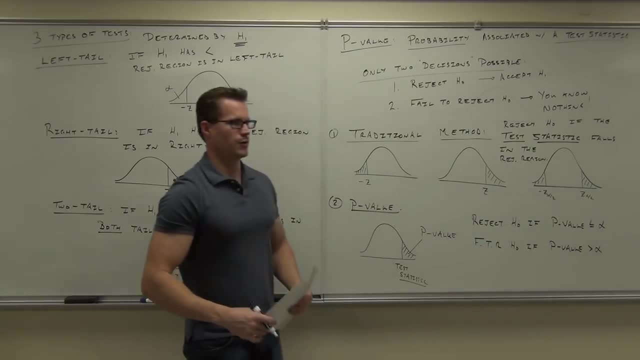 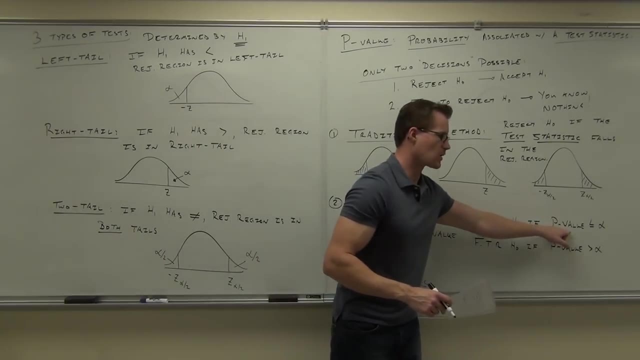 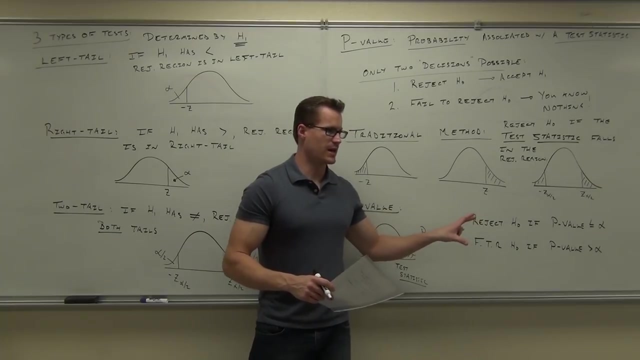 If the P-value is greater than alpha. You see, alpha is your significance, It's how sure you want to be. So if our value, if our area is less than alpha, it says, okay, it's rare enough. It's rare enough to support that with evidence. 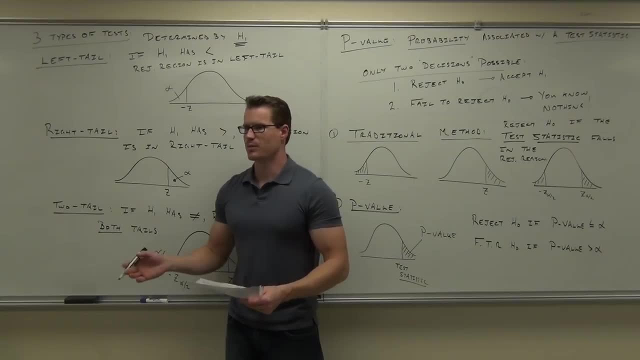 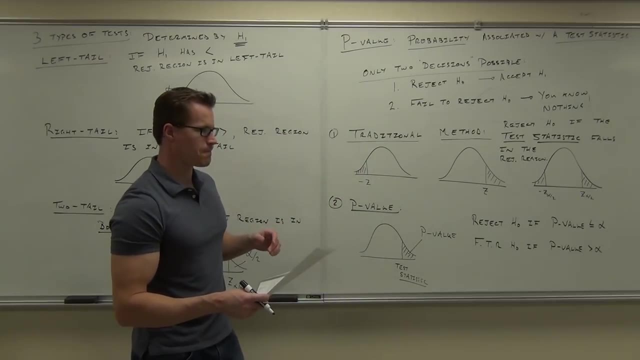 If it's not, it's bigger than alpha. it says it's not rare enough for us. May very well be true, but not according to how significant, how important we want to make this statement. Would you like to do an example of finding p-values? 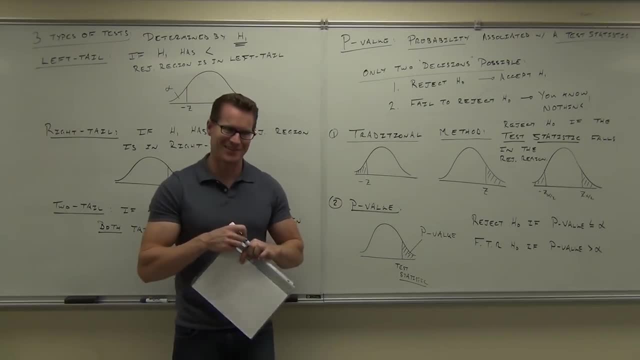 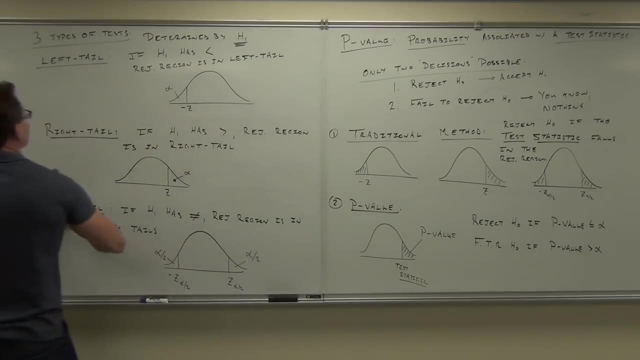 Yeah, I was hoping that you would, because I have it planned and if you didn't I would be stuck. Actually, we do it anyway, so, Okay, so hopefully you understand the traditional method right now, because we've actually done that. 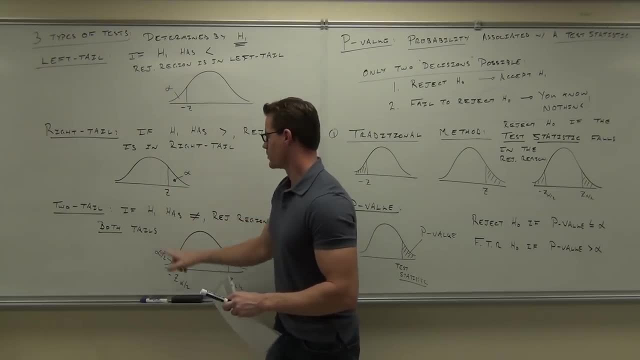 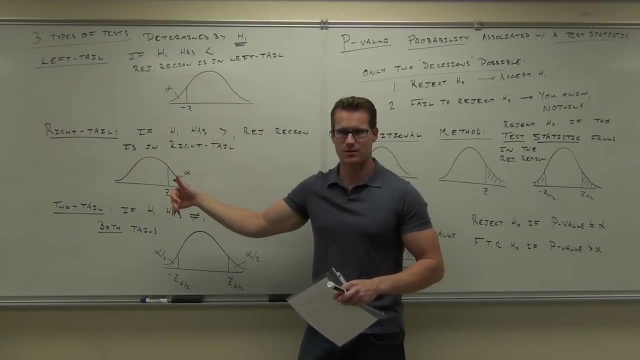 We did an example with it. Traditional method works like this: You find critical values, You already have a test statistic and you see where it falls. Do you guys have the traditional method down? You sure? Okay, here's the p-value method. 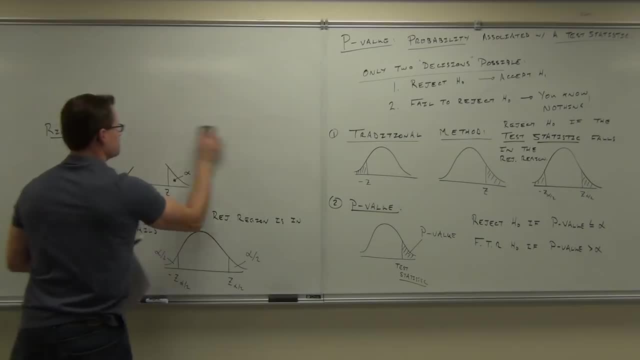 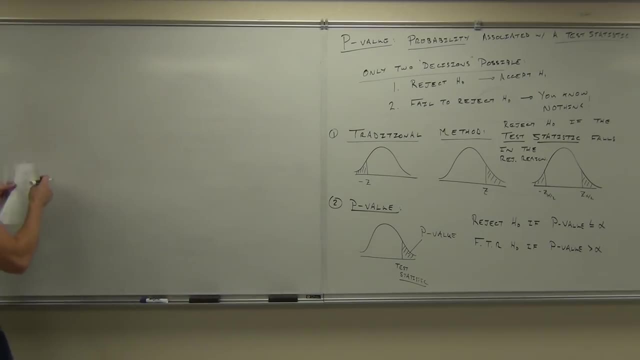 I'll just do a couple examples of finding p-value. There's really only three things you've got to do. Firstly, again, you're going to have to determine whether it's a left tail, a right tail or a two-tail test. 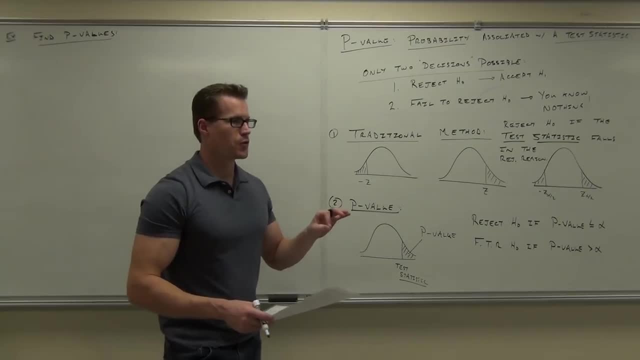 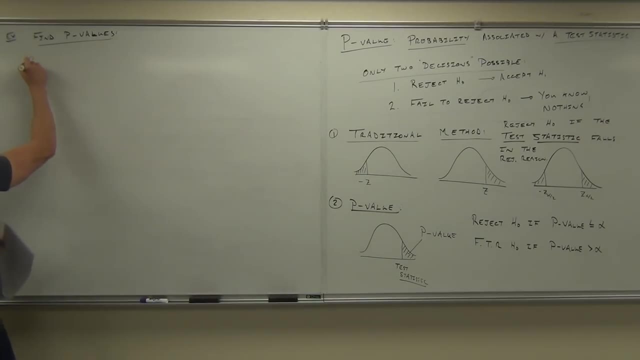 That's important. Second thing, we'll actually find the p-value. Third thing, we'll compare that p-value to alpha. That's the three things you do here. So let's do. we'll do two examples. Example number one: 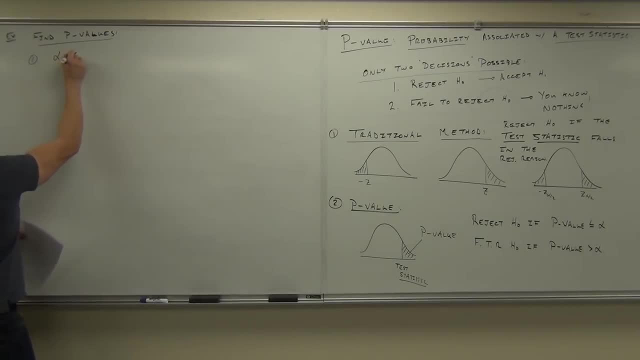 Let's say that I give you your alpha. Your alpha is 0.05.. Okay, so it's just a .05 significance level Example. I say that your H sub 1,. by the way, do I have to give you an H sub 1?? 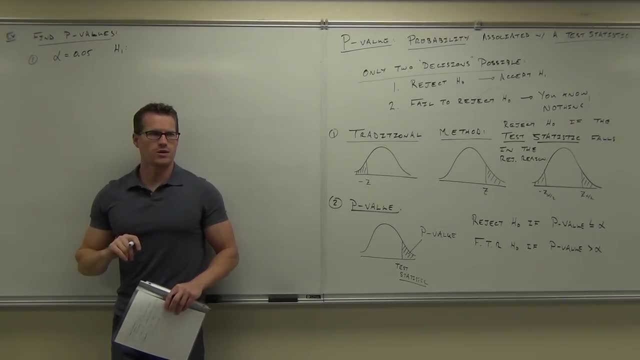 What do you think If I don't give you an H sub 1,? can you tell whether it's a left tail, two-tail or right tail test? So do I have to give you an H sub 1?? You've got to have an H sub 1.. 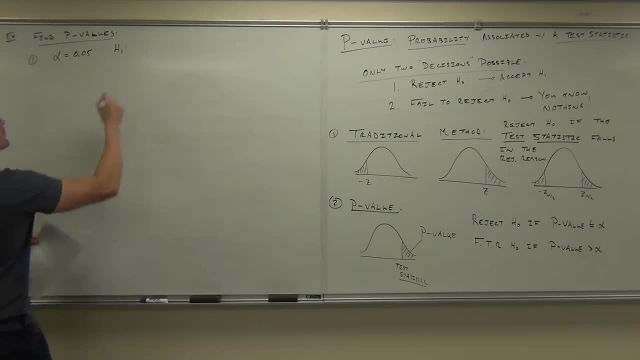 Otherwise, you're not going to be able to tell what type of test you're dealing with. Oh well, let's see how good you are. Let's see how good you are. Is this p a p-value Or is that p a proportion? 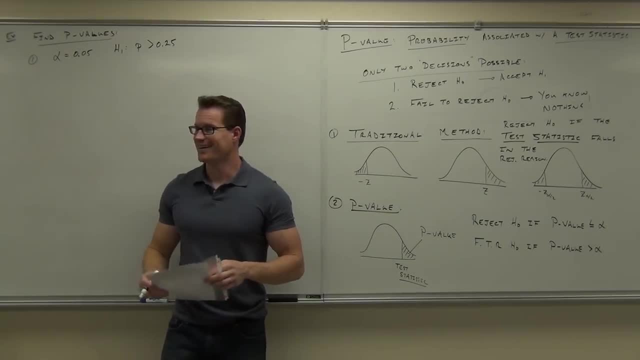 Or are they the same? Oh good, You get it. Yeah, P-value is associated with a test statistic. That right, there is a claim based on your proportion. I know that can get confusing because we have two different p's, But if it's an H sub 0 or H sub 1, it's talking about a proportion. 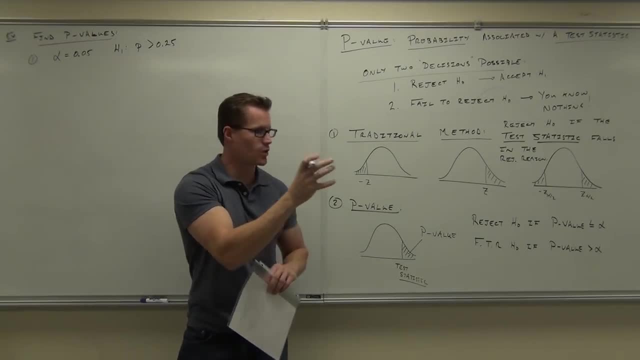 All right. If it's not, if you're looking up a z-score and you're getting an error, that's a p-value, And let's say that we're not going to do any work with this. I'm just going to give you the test statistics that I found on my own, okay? 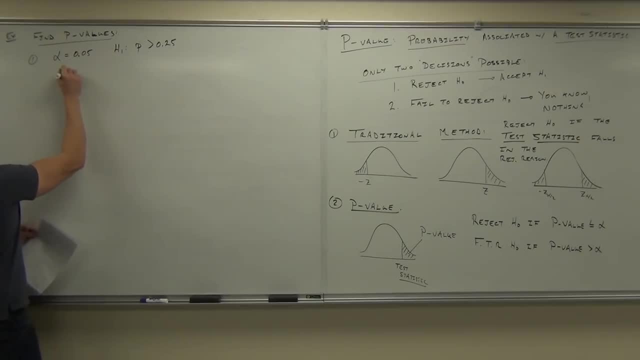 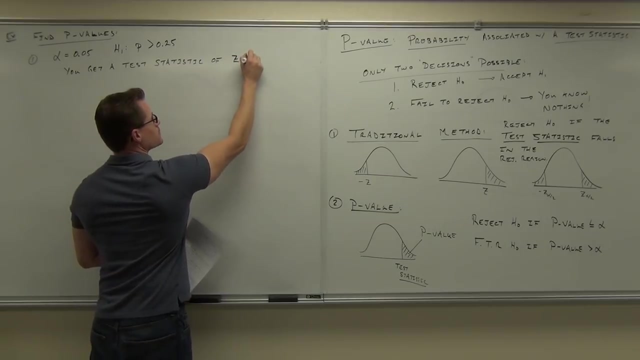 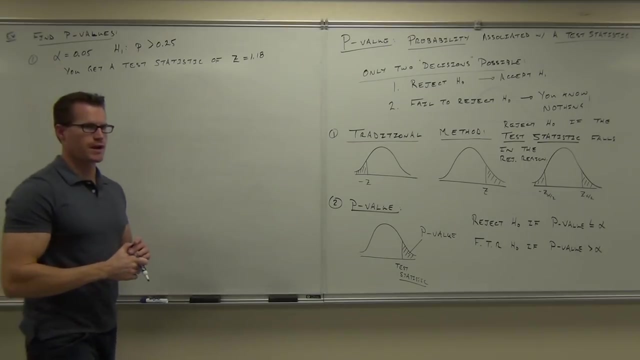 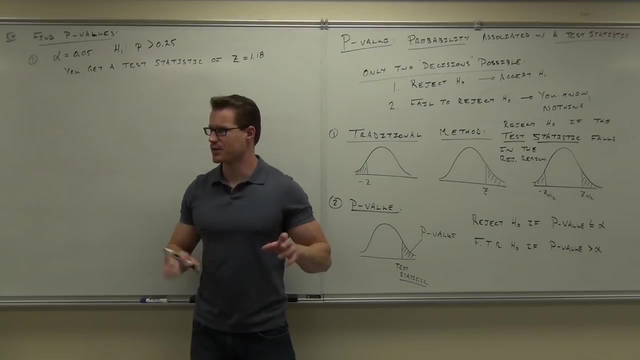 So you do all the work and you get a test statistic of z equals 1.18.. Okay, So you did the work on that. Would you like to see a comparison between the p-value method and the traditional method? Would that help you out if you saw the difference between them on this one example? 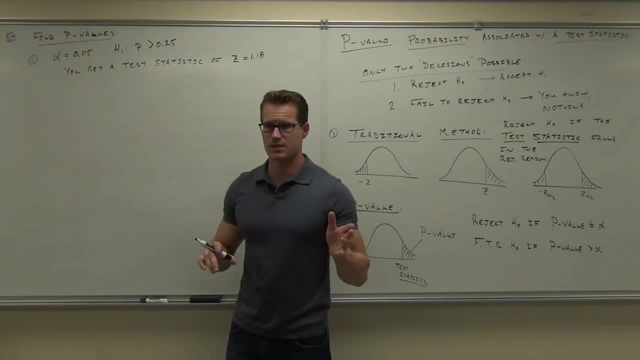 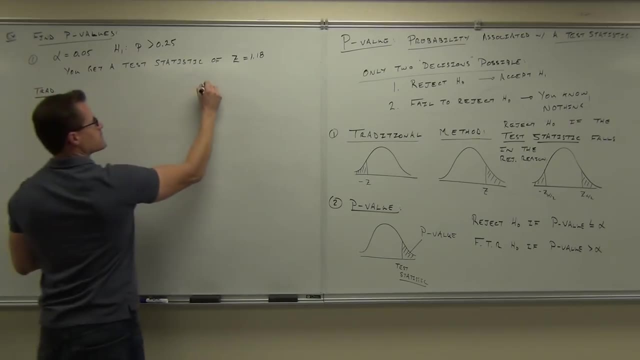 Because you could do this both ways. I'll show you both ways if you'd like. Would you like to see that? Okay, So on the left-hand side, we'll do traditional. On the right-hand side, we'll do p-val. 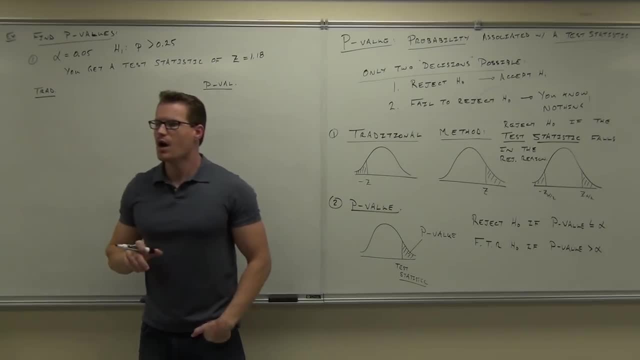 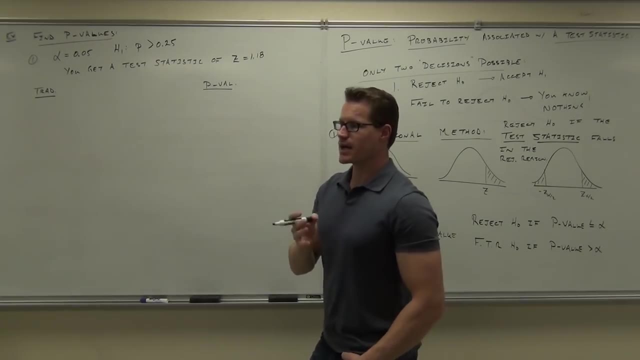 Traditional first, and then we'll do the p-value method. The first thing here is that we're going to do the p-value method, So what we need to do in each case, in each case, is determine whether you're talking about a left tail, a right tail or a two-tail test. 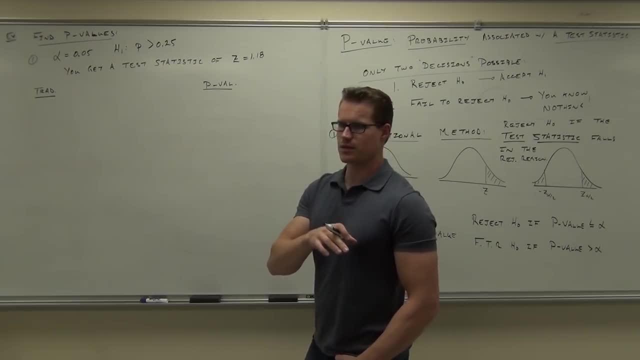 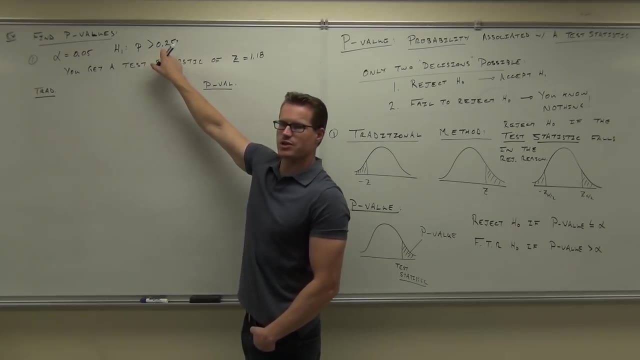 So what do you think? here Are we a two-tail test, Left-tail test, Right-tail test. How can you tell? Yeah, you just look right here. Whatever, that number doesn't matter, Doesn't matter at all. 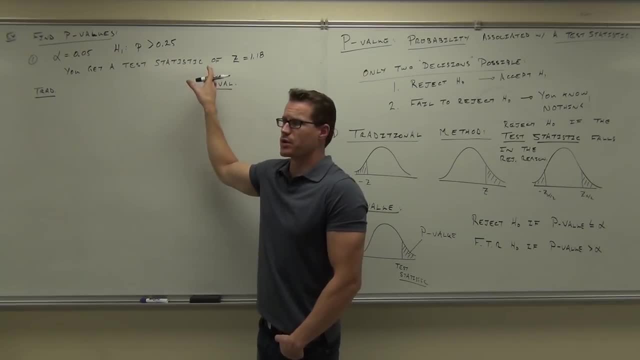 This number right here is already in your test statistic. It's already done for you, So the work's done. That doesn't matter. The only thing that matters is that That's telling you left, right Or two. You got it. 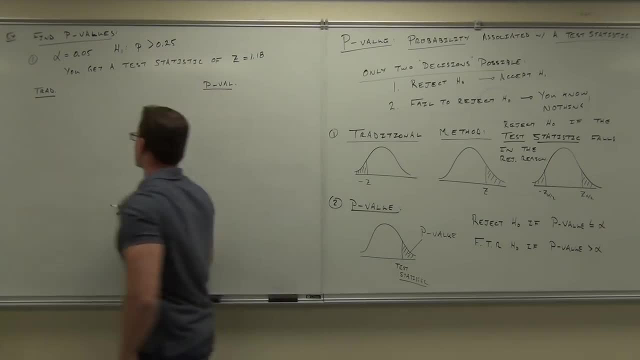 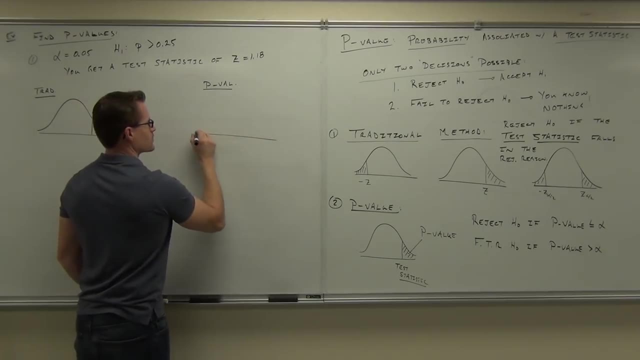 So are we dealing with a? what was it again, Right, Okay, so in each case, no matter what you're going to draw a picture for me, Both of these pictures will look identical right now. The difference is the way you go about it. 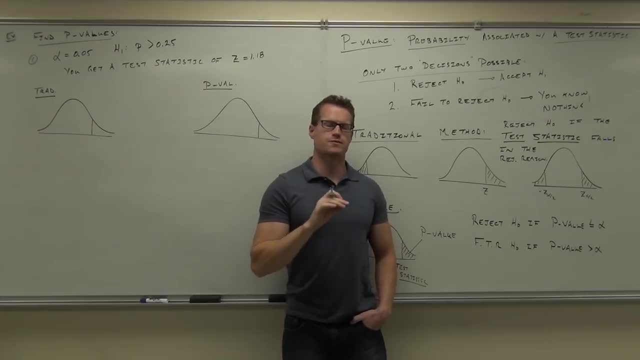 In the traditional method. here is what you do. Please watch very carefully on the board, because I'm going to ask you for both methods on your final exam. Here's the traditional method. Traditional method: It says you're going to take your alpha. you're going to look that up in the chart, which I had you do just a little bit ago, right? 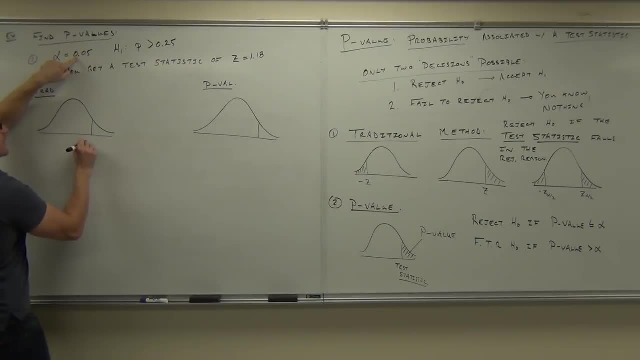 And you're going to say that this is a critical value of 1.645.. Remember that number. Are you okay on where that number comes from? Yeah, Okay, Because this alpha is 0.05.. Remember that this is a critical value. 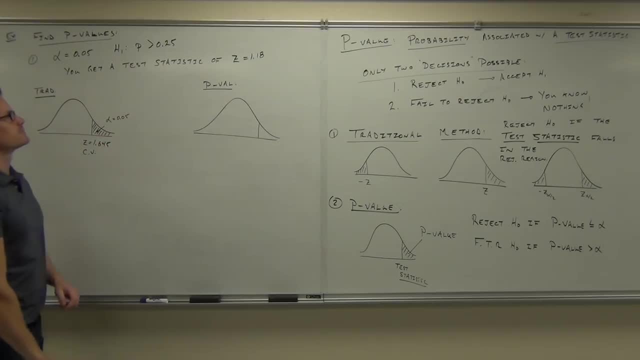 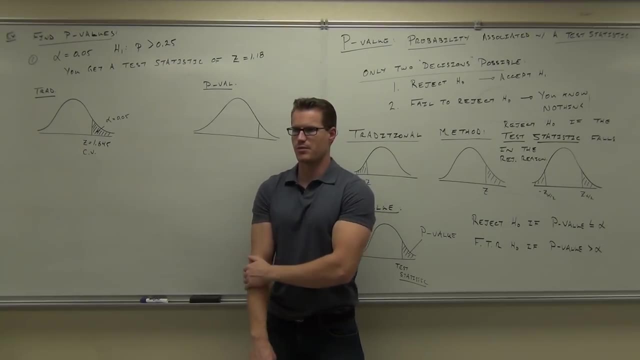 This right here is our rejection region. Did you get me so far on the traditional method? This is old stuff. We've already done that before. Now you'd go ahead and you would compare your test statistic. What's the test statistic in this case? 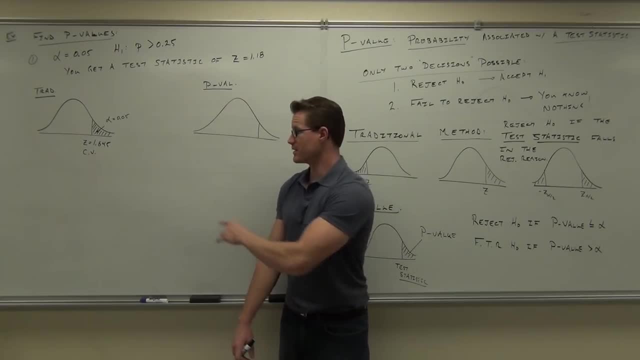 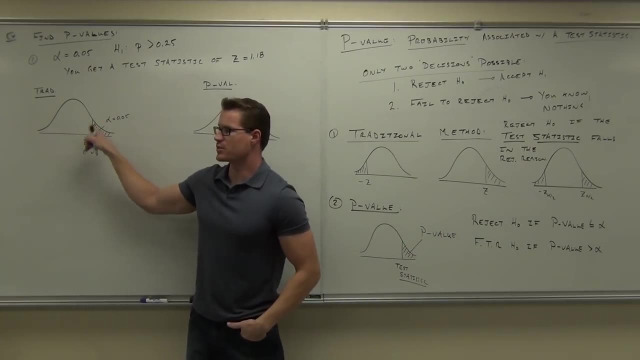 Great, 1.18.. It says test statistic: right, It's got a z-score, even though that's not a z-score. yet You're comparing two z's here. Compare 1.18 to your picture. now Is it in the rejection region? 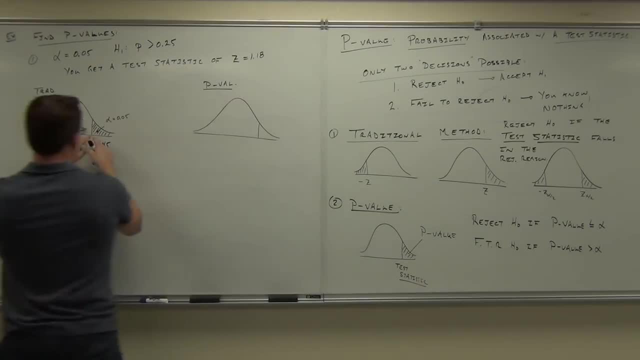 Or the fail-to-reject region 1.18 is. it's over here. That's the fail-to-reject fail-to-reject. So your decision would be fail-to-reject. H of 0.. In English, we'll deal with the interpretation in just a bit. 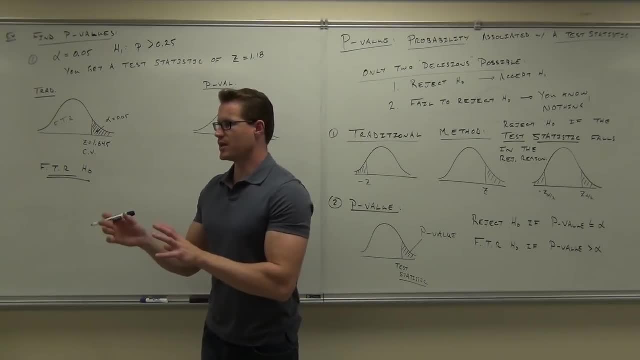 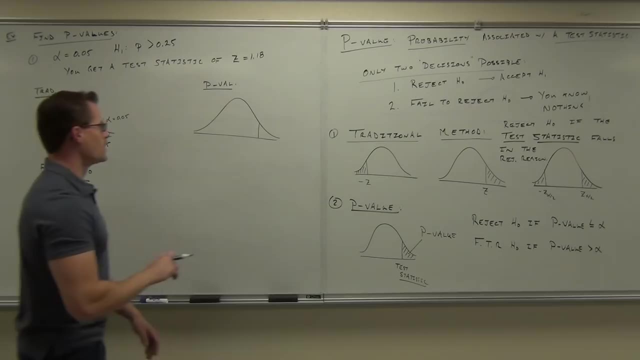 It would be. there's not enough evidence to support the claim that, whatever we're talking about, okay, There's not enough evidence You fail to reject. Right now, we're just seeing if we reject or not. Now. we should absolutely have the same decision here. 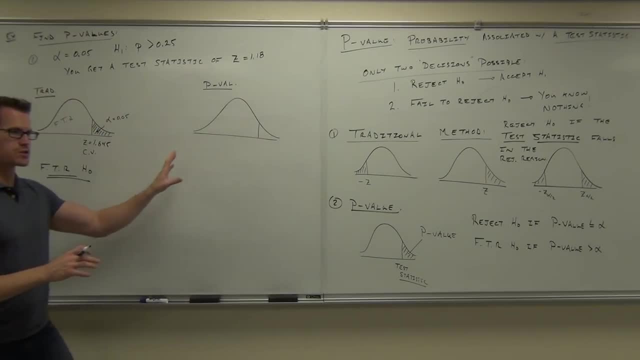 If we don't, then something's wrong. So let's go ahead. let's look at p-value First. raise your hand. if you're okay with traditional, Are you okay with that, what we just did? If you're not, raise your hand. 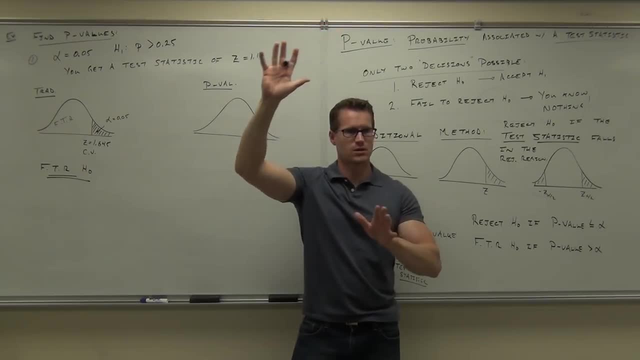 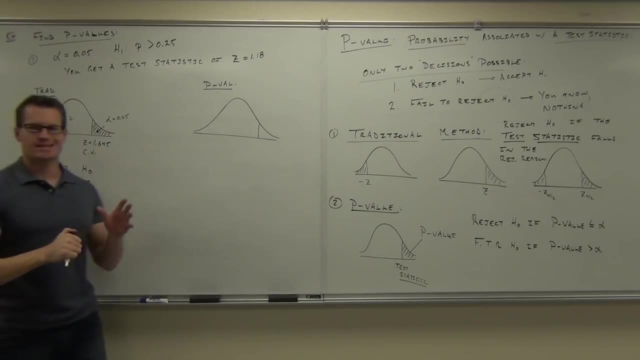 I'm assuming we're not. Let's see if we are or not. Yes, no, Good. okay, that's everybody. Now the p-value method works differently. There's no such thing as a critical value when you're dealing with a p-value method. 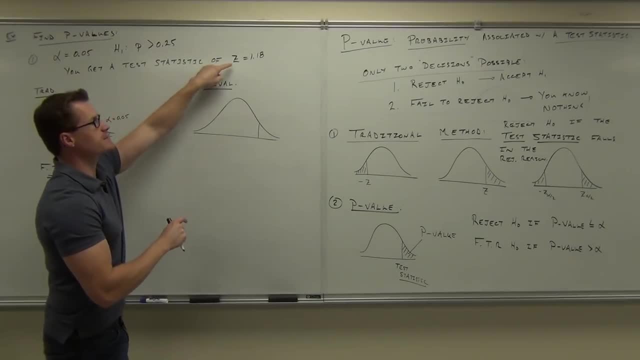 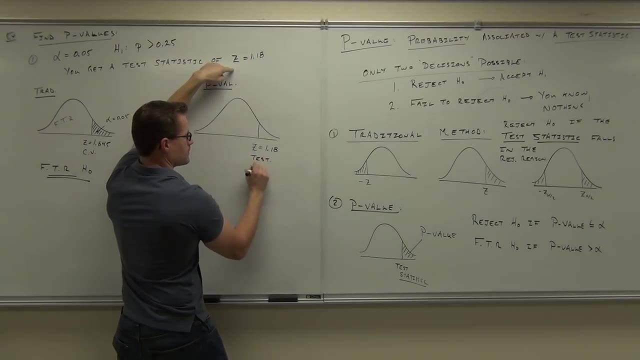 What the p-value method does is. it says: you take your test statistic and that's what you put right here And you find the area that's associated with that, That's known as a p-value. Now this is all going to come back to you. 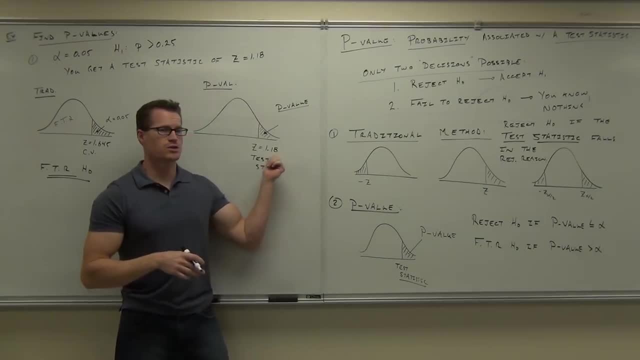 Chapter 6 is going to smash you in the face right now. Do you remember how to look up areas associated with z-scores? Do you? On your calculator, you'd put in normal CDF from 1.18 to 10.. 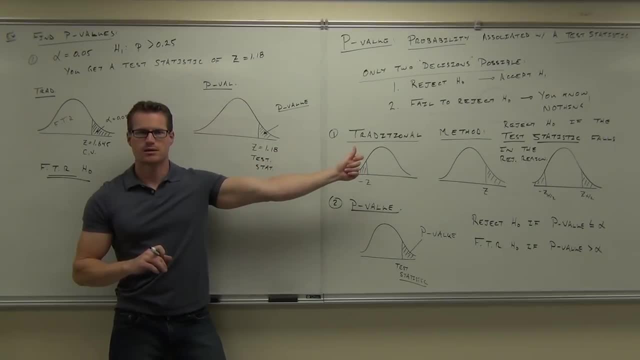 Remember doing that On your table? you'd look up 1.18.. So go ahead and do that. now Look up 1.18.. You're looking at z-scores. now Look up 1.18.. Say that one more time, Chris. 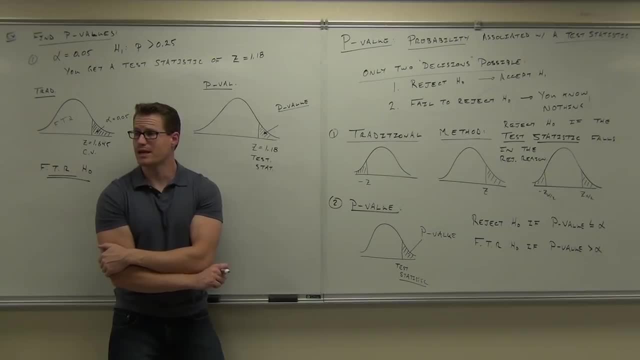 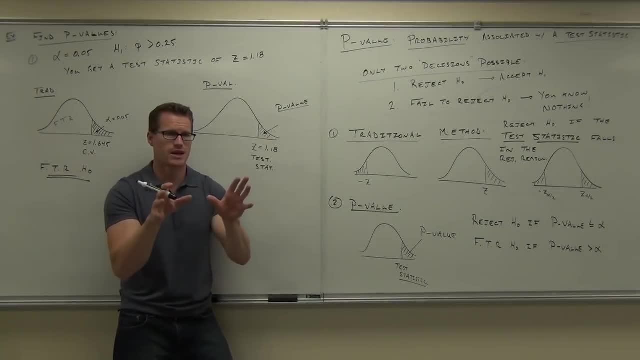 No, No. Now here's the big thing where some of you guys have not really kind of conquered this yet, even up to this date. If you do .8810, look at the board. Is this .8810?? You've got to be smarter than your table. 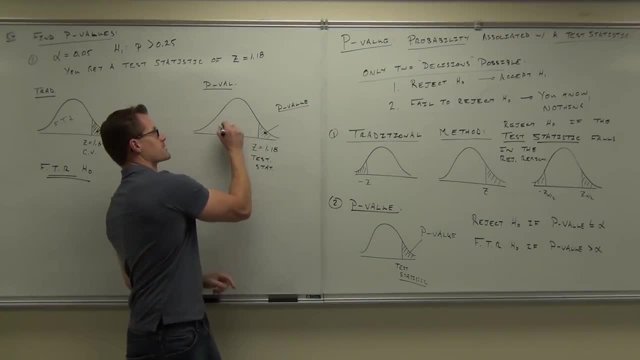 What's your table give you? Did it give you the right or the left? It gave you this: This is .8810.. Well, how do you find that one? The p-value, therefore, is .119.. How many of you guys are okay with .190?? 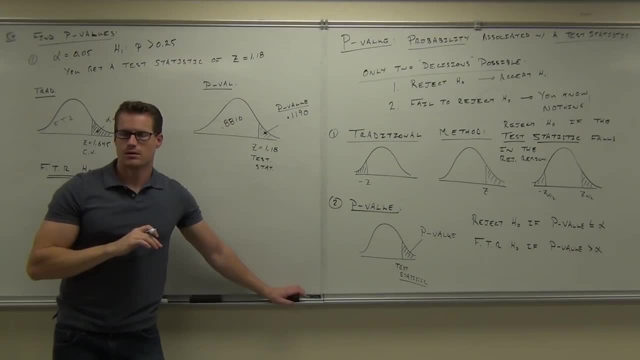 Are you okay with that? How many of you feel okay with finding the p-value? Now here's what you do with it. You compare now your p-value to your alpha. What's your alpha? What's your alpha? It should be on the board. 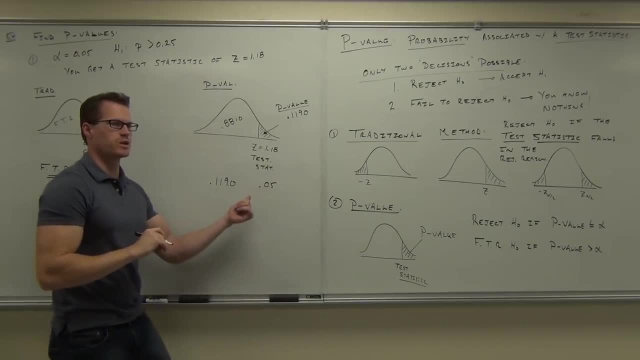 All you've got to do is put the right symbol. What I'm gonna do is put the right symbol between them. This is your p-value, this is your alpha. Which one's bigger? So do I have this greater than, or do I have this less than? 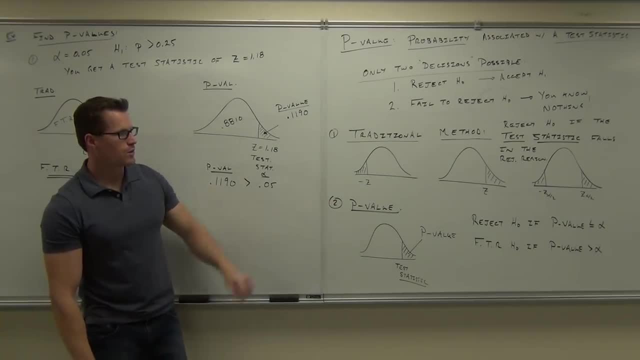 I have greater than. If your p-value is bigger than your alpha, you reject your null. you fail to reject h sub zero. If your p-value's less than alpha, it says it's rare enough to reject it. So what do we do here? 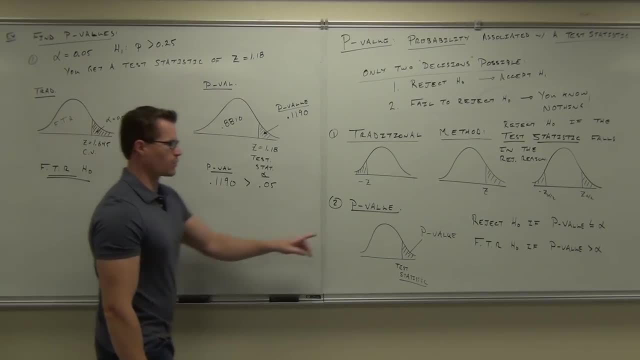 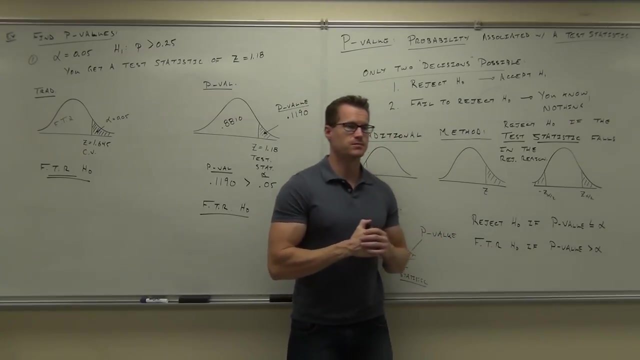 Do we reject or do we fail to reject? We're, in this case, right: P-value's bigger than alpha. we fail to reject h sub zero. Same exact situation as before, just a different way of looking at it. So which one has a critical value, traditional or p-value? 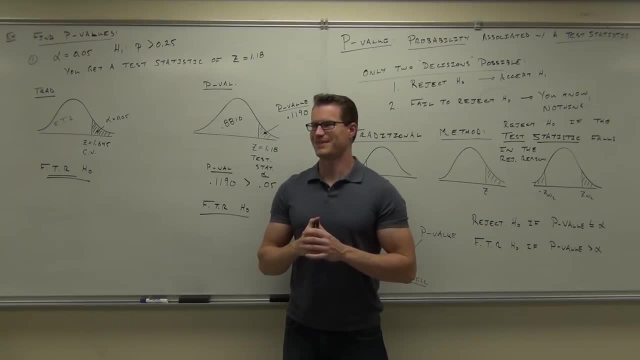 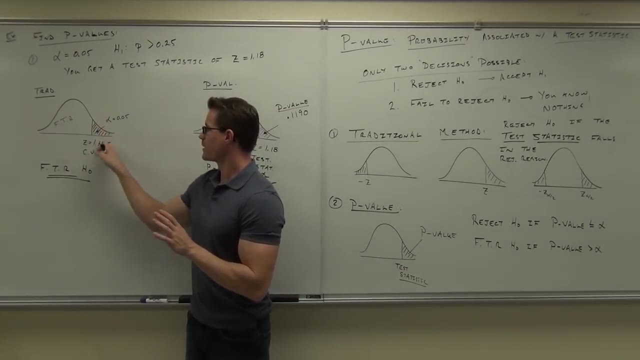 Traditional, Which one has a p-value. well, clearly, p-value In each case. you still have a test statistic, though, right, It's just whether you're comparing a test statistic to the critical value or whether you're finding the area. 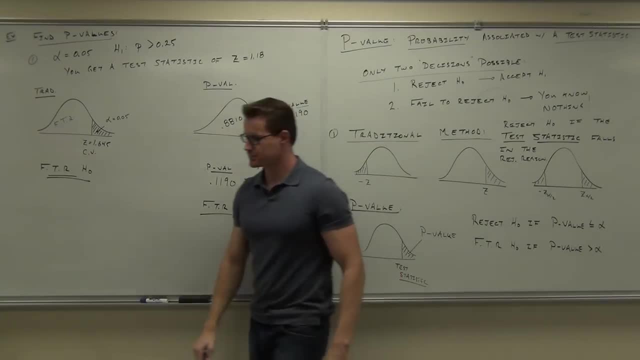 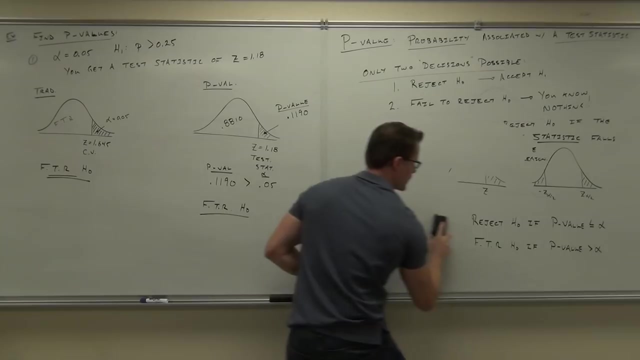 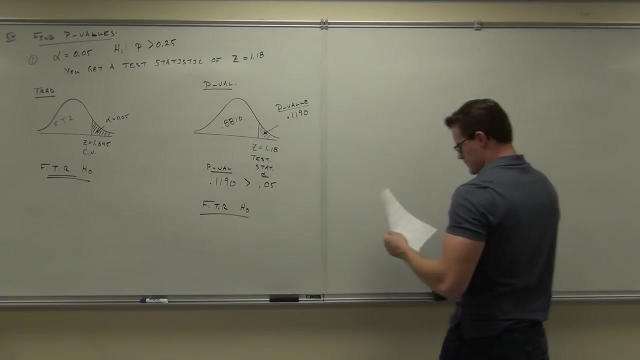 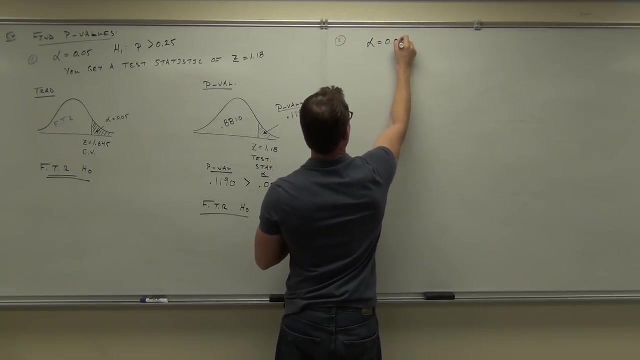 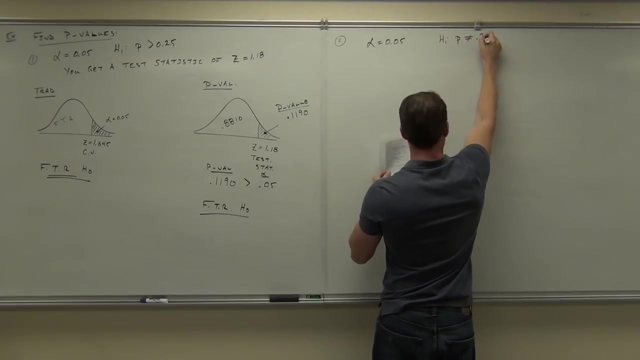 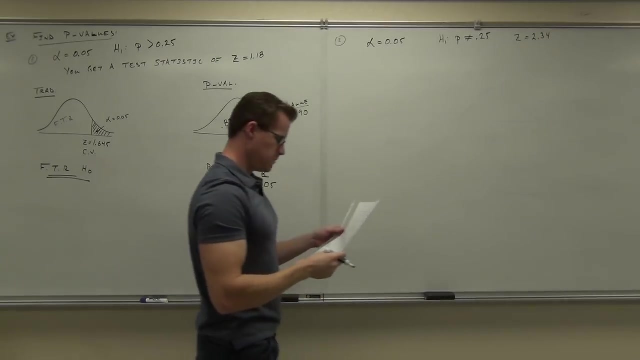 out from your test statistic and comparing it to your alpha. Okay, we've got about 30 more seconds here. I want to show you one more and then we'll be done. All right, here we go. Firstly, I deal with a one-tail, two-tail test. 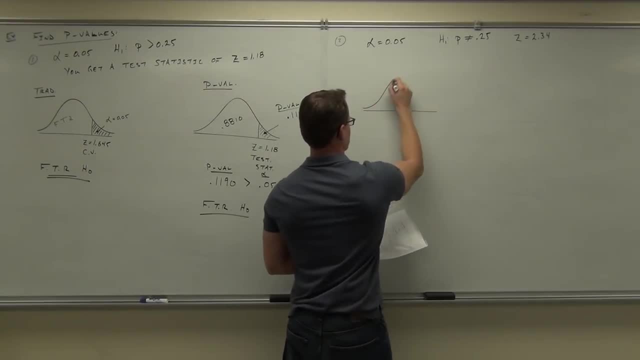 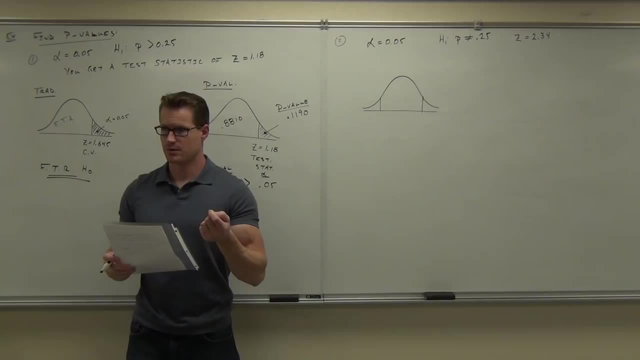 Two-tail, So you would have this shape, but now you'd have two tails. If I'm talking about the traditional method, here's how it would look. Look at the board with me, please. If I talk about traditional method, this is 0.2,. 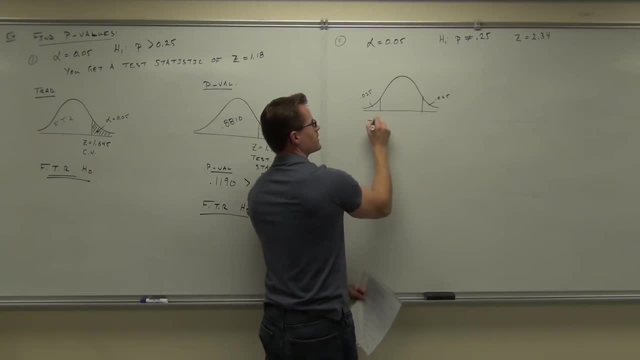 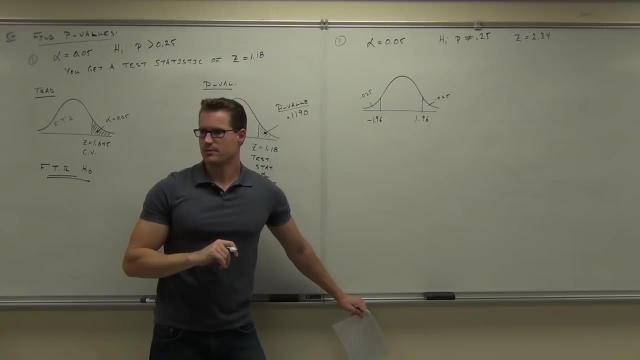 0.025, and this is 0.025,, making this negative 1.96 and 1.96.. Do you follow me on that? Would you reject or not? You should be able to make that determination right now. Would you reject or not? 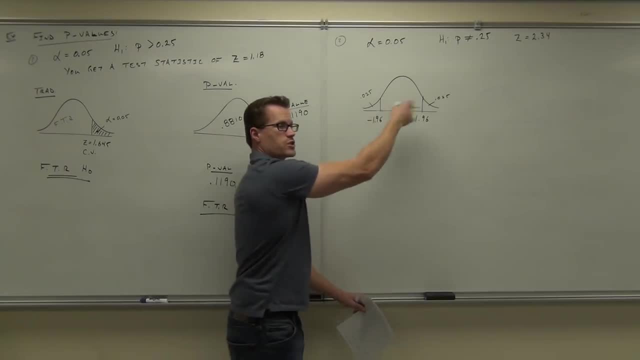 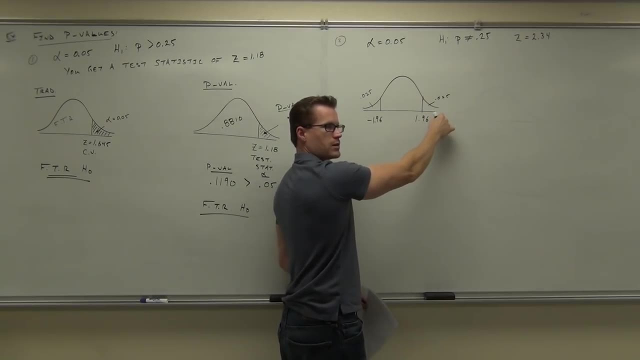 What's your test statistic? Does it fall in the rejection region? Where's 2.34? It's over here, right? This says 2.34 falls here. You would reject H0.. Does that make sense to you? P-value method does something a little bit different. 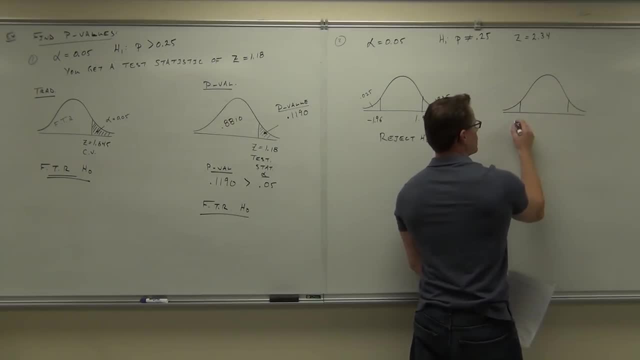 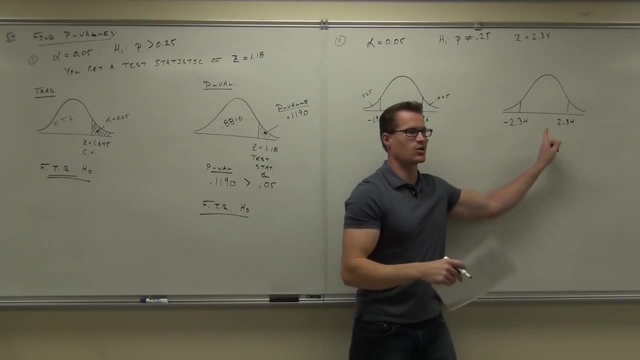 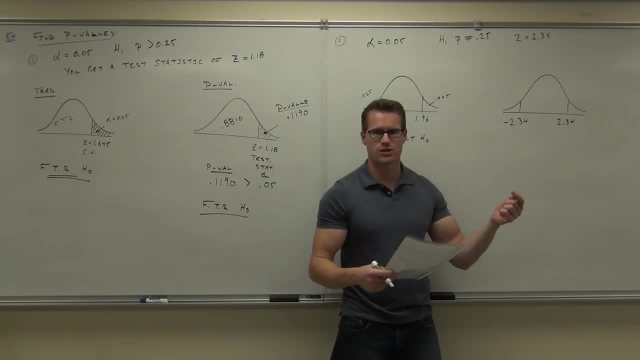 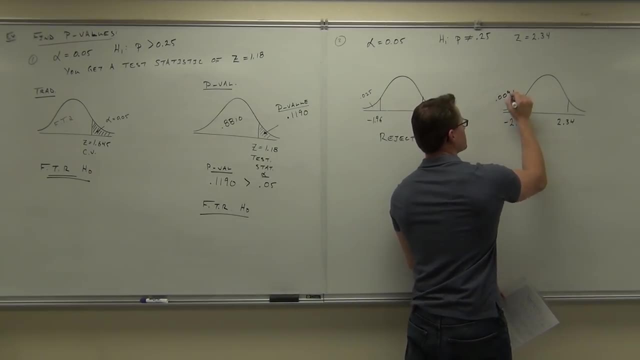 Just watch carefully. I'm going to do the math for you. You all know how to look up negative 2.34 on your distribution, right? That's going to give you 0.0096.. And of course, this is symmetrical.